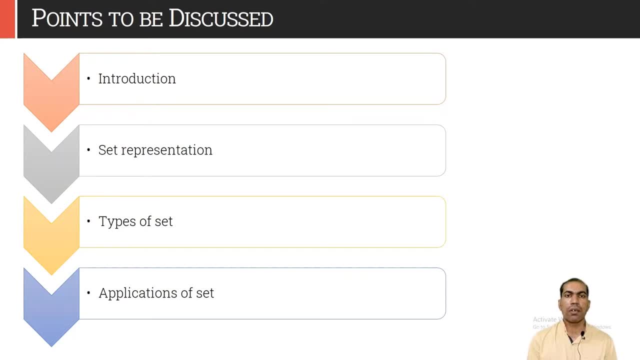 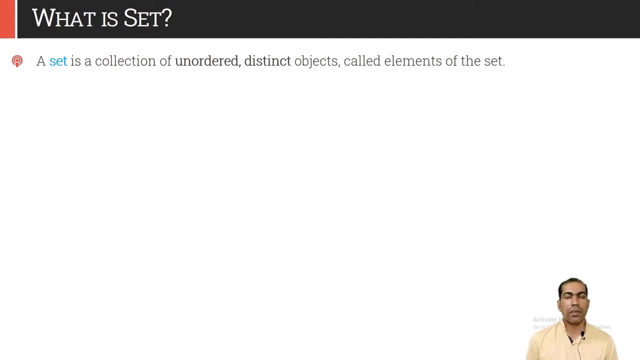 will talk about different types of set and we will state out what are the applications of sets. So basically, we can say that set is a collection of unordered distinct objects. These objects could be anything and they are known as a member or the elements of the set. 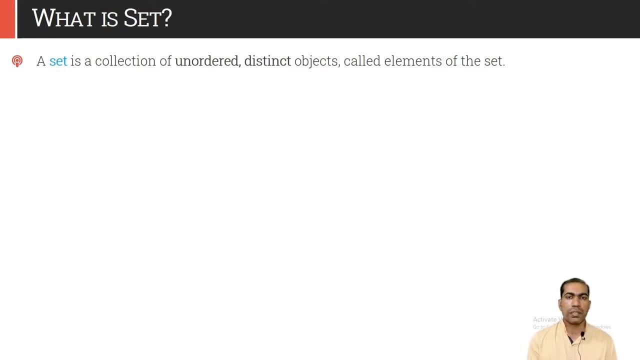 So these elements are random. It could be students, it could be CPA of the student, maybe age of the person, maybe salary, maybe position, color, fruits, it could be anything. Two properties are important. The elements are unordered into the set, So if you write, 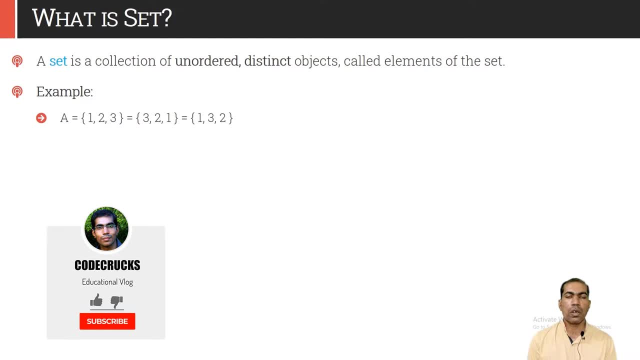 a is equal to 1,, 2,, 3 or 3, 2, 1 or 1,, 3, 2,, all corresponds to same set, because order in set does not matter. So if you write a is equal to 1,, 2,, 3 or 3,, 2, 1 or 1, 3, 2,, all corresponds to same set. 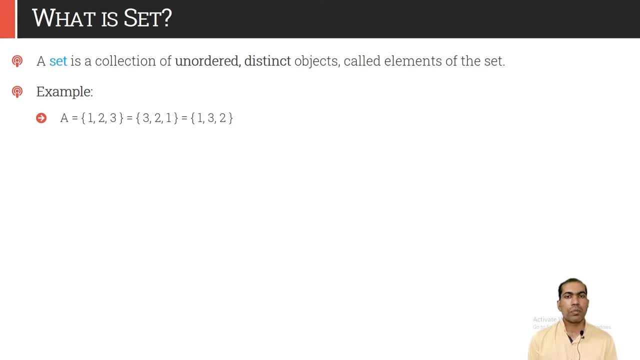 because order in set does not matter And all the elements in set should be distinct. So if your set is like 1, 2, 2, 3, 1. So it is not considered as a set because elements are having multiple. 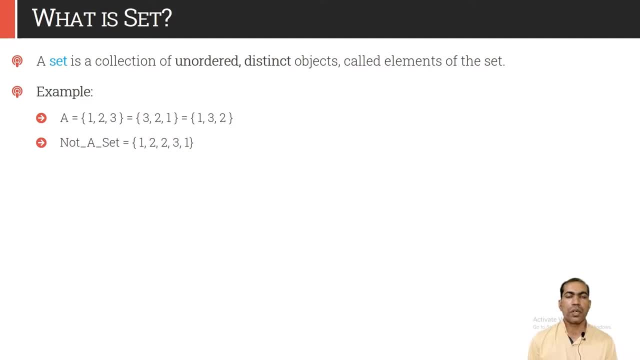 entries. So 1 and 1,, 2 and 2.. So this is not a set. However, you can call it as a multi-set, but it is not a set. We can classify sets in two categories. The finite set is a set in which we 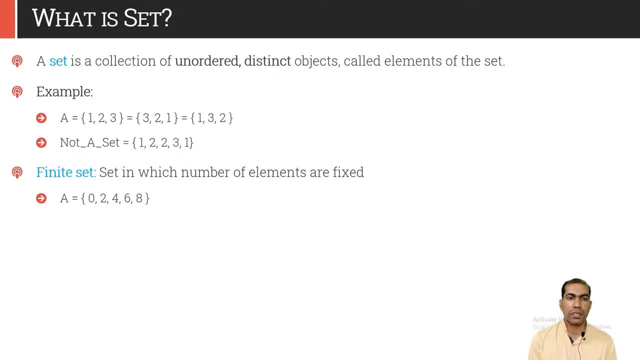 can count number of elements, That is, number of elements are fixed. For example, set A- B is equal to 0,, 2,, 4,, 6,, 8.. So this is the set of even numbers less than 10.. The number of 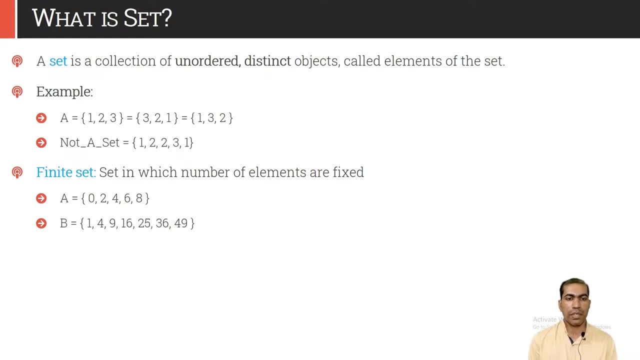 elements are here 5.. So we can count the number of elements. Similarly, set B represents elements which are perfect square, as well as they are less than 49.. So again, set B contains only 7 elements. So these are the countable sets. So we will call it as a finite set In infinite set. 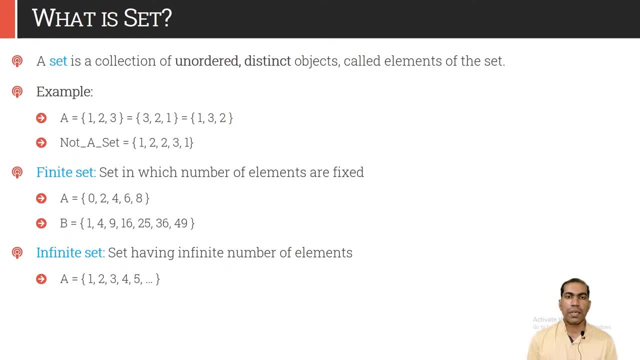 we cannot count number of elements. We know the elements but we cannot count them. For example, set A is a set of natural numbers. A is equal to 1,, 2,, 3,, 4,, 5, up to. 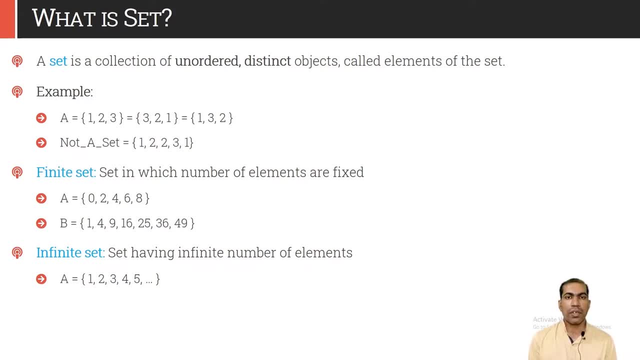 infinity. So we cannot count actually how many elements are there. We know the elements but we can't count it. So this is infinite set. Again, B is set of even numbers. So we know the elements 0,, 2,, 4,, 6,, 8,, 10 and so on, But again, number of elements are infinite. So this set is 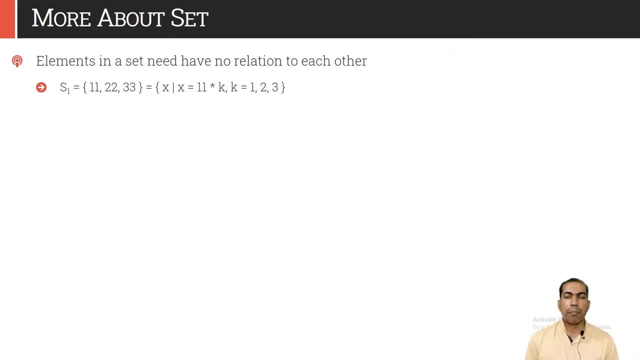 known as an infinite set. The elements in set may or may not have relations between them. If we consider set, S1 is equal to 11,, 22,, 33.. So we know that here all the elements are multiple of 11.. So we can say that there is some relationship between the elements, and we can 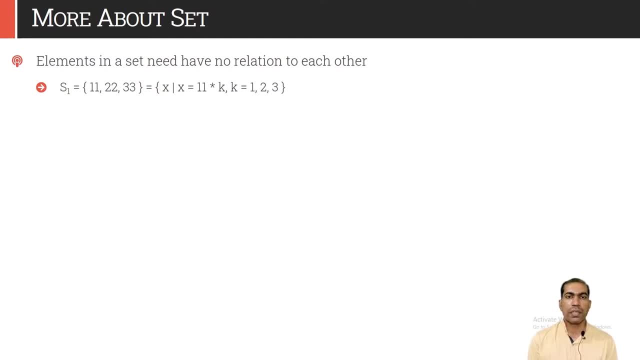 define it set S1 as, like set S1 is set of all the elements x, such that x is 11 into k and k varies from 1 to 3.. So when we put k is equal to 1 to 3, we will get 11,, 22 and 33.. But your set S2 may be. 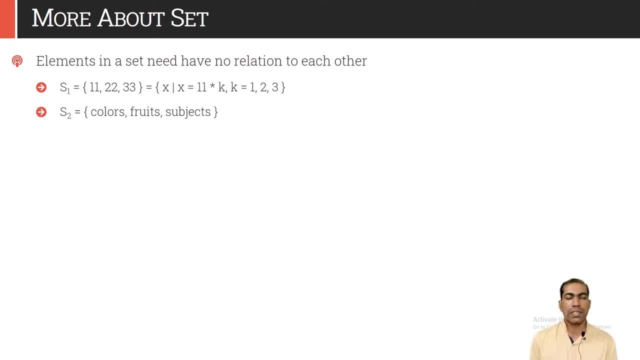 one set fruits subjects, So color itself may be. one set Fruits is another set. Subjects represent some another entity. So all these are different entities that do not have anything to do with each other. Similarly, set S3 represents red, which is color, Truck, which is vehicle. 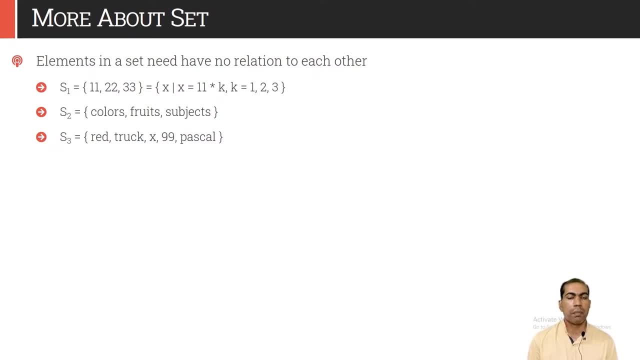 X may be some variable, 99 may be some number. Pascal is a programming language, So, as you can see from these examples, the elements may or may not have relationship between them. Set can also contain set as an element itself. So till now, whatever examples we have seen, 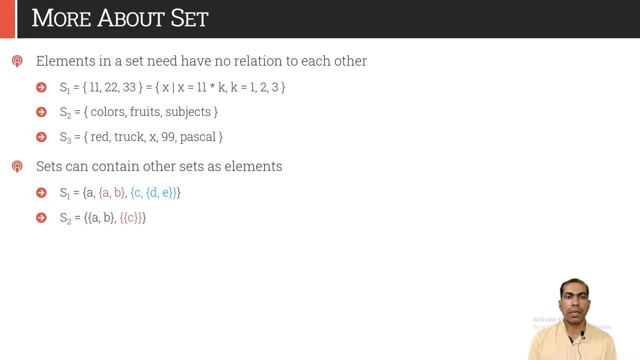 the element was only single entity. That was either a number or maybe a truck, maybe x, maybe 99,, Pascal. So they all are one element. As you can see, that set S1 is having three elements: A, that is a single element, Set AB, that is the second element And the bigger set. 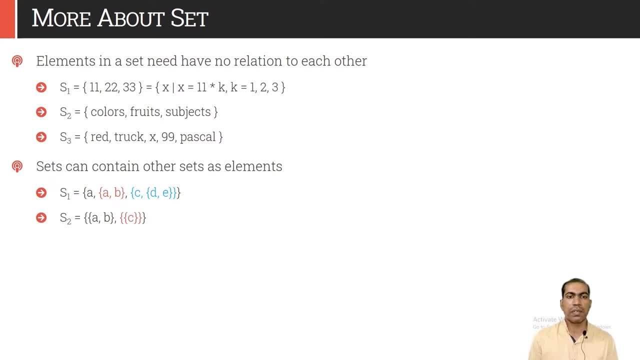 which again contains set as an element. So that is a single element And the bigger set is a single element of itself. So these three elements are shown in different color for your understanding. Similarly, set S2 is having only two elements, where first element is a set AB. 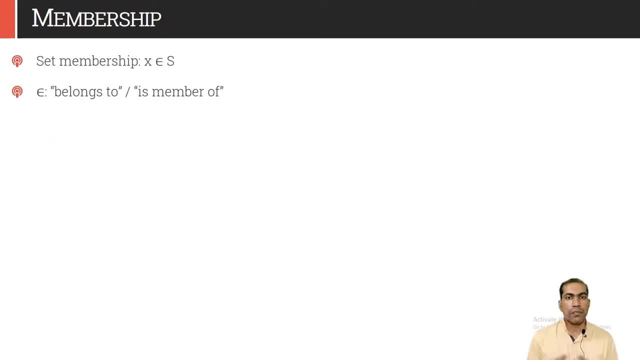 and second element is a set C. If the element is present into the set, then it is represented by this notation and it is read out as a belong to or is member of. If element X is present into the set S, then we will say that X belongs to or is member of this set. So if element X is present, 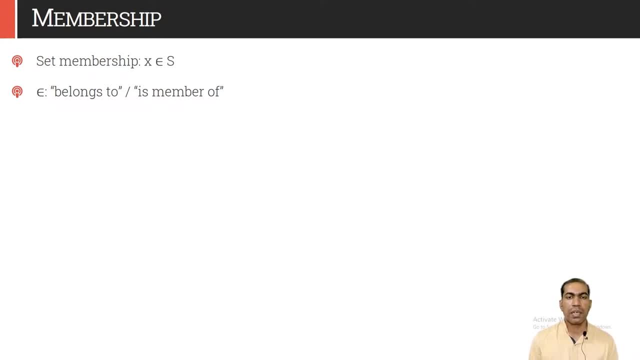 into the set S. then we will say that X belongs to or is member of this set. So we will say that to set s or x is member of s. let's see some example here. element a is not present into the set, so we will write a does not belong to set. or we will say a is not member of the set. here 3 is 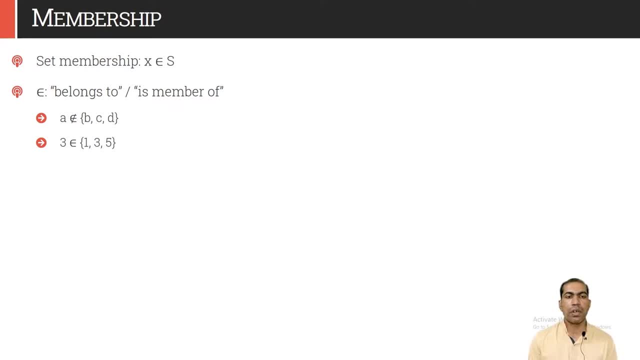 present into the set. so we will say that element 3 is member of given set. however, here the set contains two element. first one is a 1 and second one is set, again 2 comma 3. so 2 comma 3 is the entire element of the given set. so that set has only two elements, 1 and 2 comma 3, and hence we 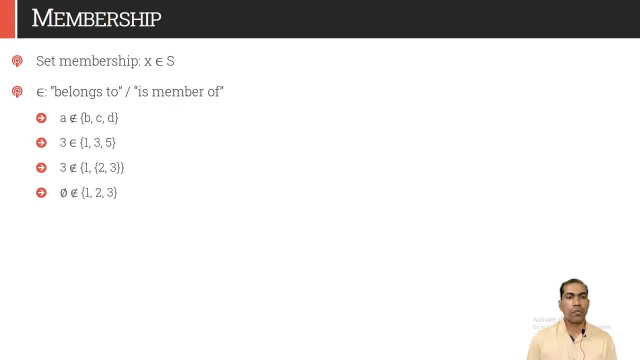 will say that 3 is not a member of given set. 5 does not belongs to 1, 2, 3. similarly, 5 is present in this set, so we will say that it is a member of set. cardinality defines how many numbers are there or how many elements are there into the set. so cardinality is what it is, simply the size of 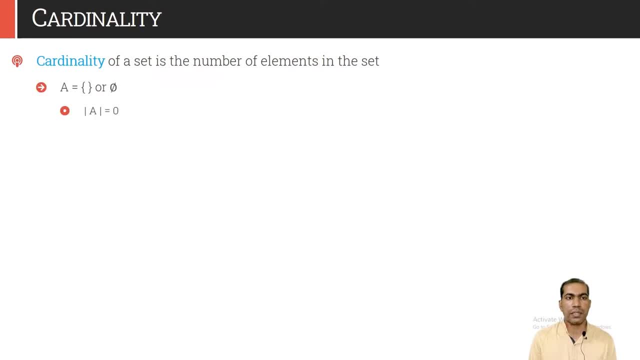 the set, or it defines the number of elements into the set. let's take the examples: set a is equal to null or the 5. you know that null set means it does not contain any element, so cardinality of set a would be 0. set b contains only one element, so cardinality. 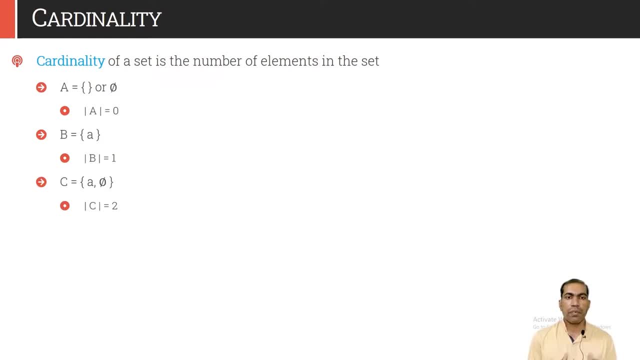 of b would be 1. c contains two element where first is a and second is a null set or the 5, but again it's an element of set. fine, so the cardinality of c should be 2 here. set d contains three distinct element: a, b and c. so cardinality of d is 3. let's move. set e contains only two element. 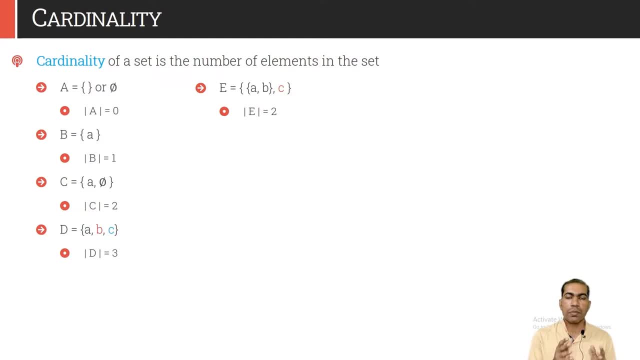 where first element is a set itself. now this set could be of size 1, 2, 3 or infinity, it doesn't matter. the set e has only two element: the set a, b that is the first element, and c that is the second element. so cardinality of e would be 2. set f is having only one element, which is 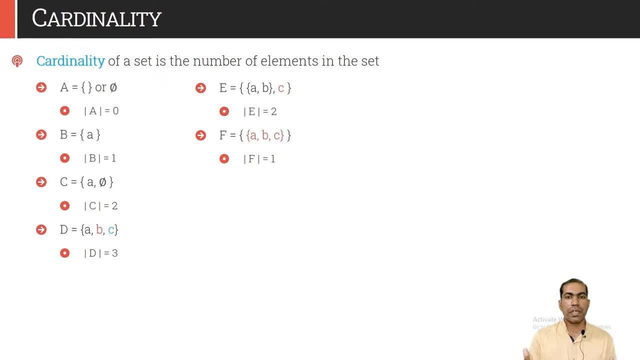 a set. now again, irrespective of size of the inner set, the number of element in set f is only one, so cardinality of f would be 1. in set g we have five elements. first, one is a second, one is a set which contains only one element, that is b. third element is again a set. within that we have a set of size. 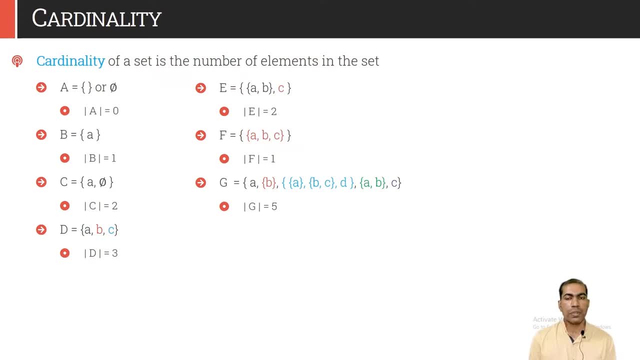 1, that is the first element, set of size 2, that is the second element and the individual element. d is the third element. the fourth element of g is set itself of size 2, that is a comma, b and the last element is c. so all elements of g are color coded for your better understanding. so the cardinality of g. 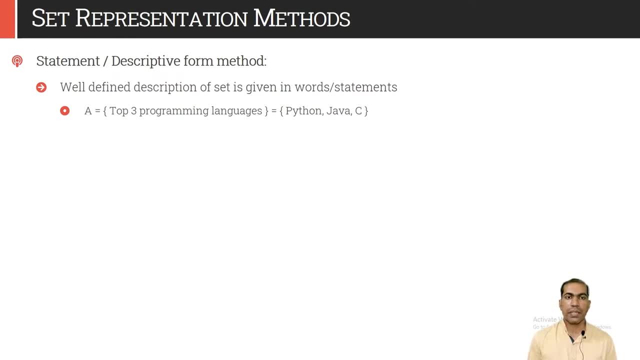 would be 5. set could be represented using different methods. we will see one by one. the first method is known as a statement, or the descriptive form method, in which we are writing the set using english-like statements. for example, a is top three programming languages, so the set, a would be python, java, c, etc. it contains three. 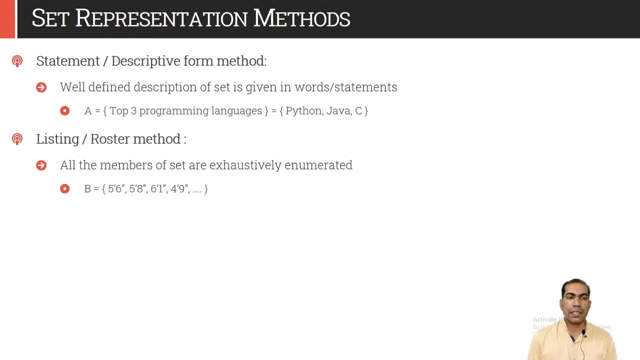 languages. the second way of writing set is using listing or the roaster method. many times it is difficult to write down the english-like statements to mention the elements of the set, for example, if you want to create a set of height of the students in the group. so we cannot write english-like. 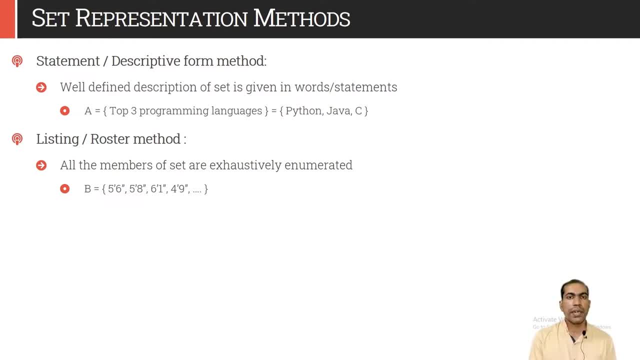 statements to represent the set. so we cannot write a set of height of the students in the group. therefore we cannot write a set of height. Potato's only set body size. we need to write down the height of individual student. so set B may be 5 feet 6 inch. that we 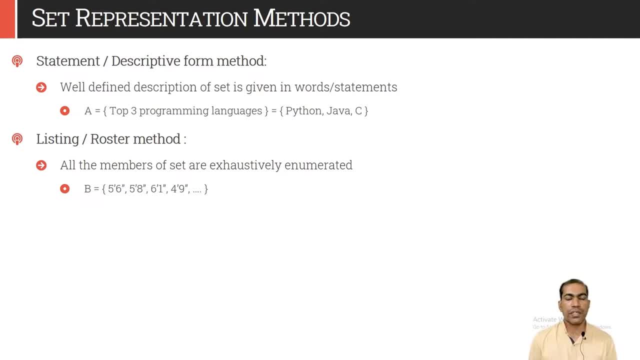 that is the height of the first student- 5 feet 80- and that is the height of the second student, and so on. so here we are enumerating all the elements exhaustively. so if size of set is bigger than it is difficult to enumerate all the elements. 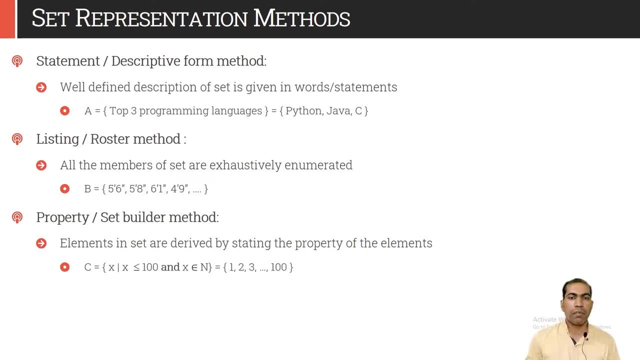 this is the most popular and most fundamental way of writing the elements. then we have to calculate Excel combined elements on two rows of two sets. this is in the top line. these are the John dentro and we have Watch your video of theicy. any item, we either just meas the word element and then you take the falling青 back in and write the first element and it is the same. 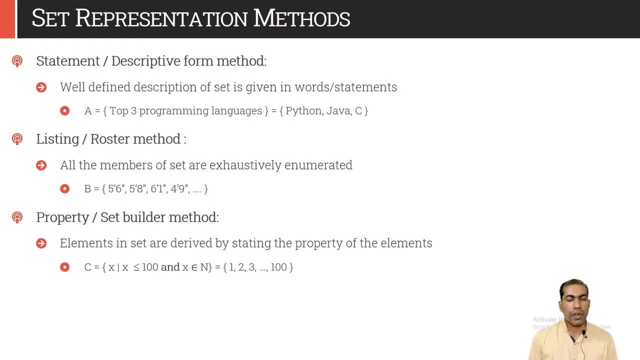 that is the property or the set builder method where we are writing set. in terms of recursive definition, that means we are finding the common property of the elements and based on that we are creating the set. so this is described as like set c is collection of elements x, such that x is less. 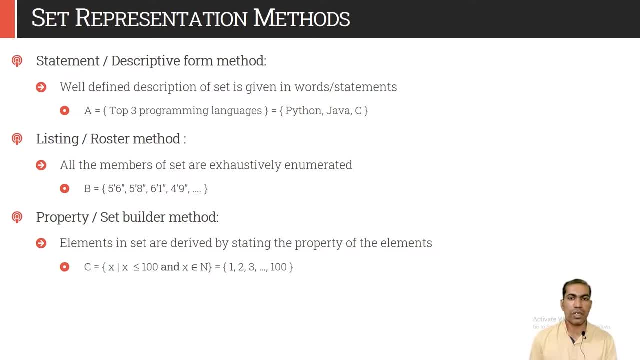 than or equal to 100, and x belongs to set of natural numbers. so you see that x belongs to set of natural number. it means x could take any value from 1, 2, 3, 4, 5, up to infinity. but again we are giving some bound on that that x must be less than or equal to 100. so now set c will take 100 values. 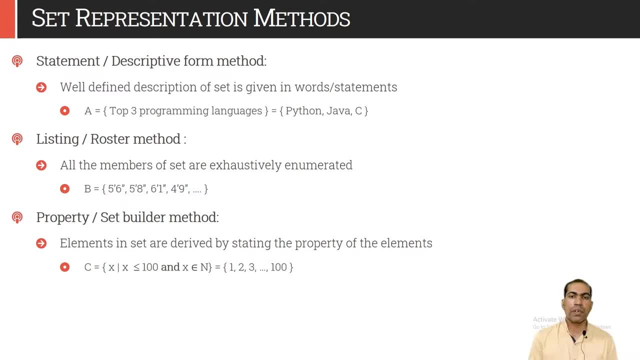 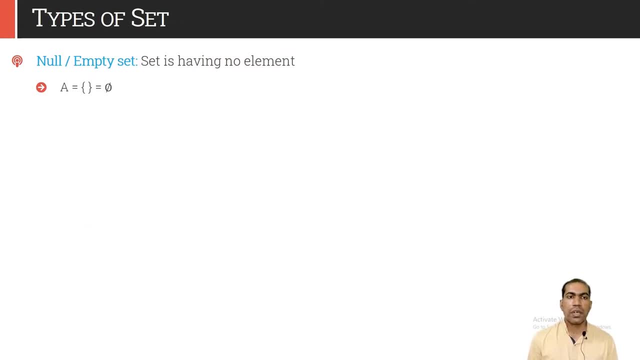 1, 2, 3 up to 100. so this is most fundamental and convincing way of writing the sets. let's talk on different types of set. so set is called a null set or the empty set if it does not contain any element. for example, if you. 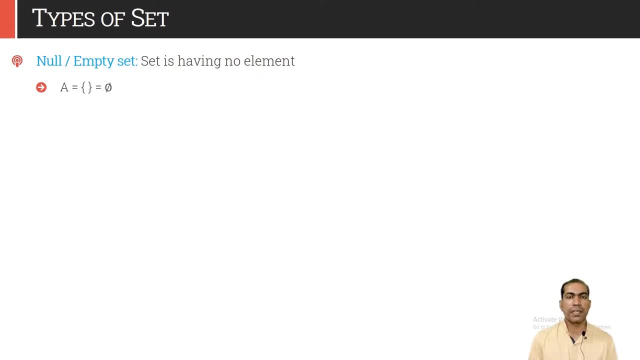 want to create a set of students whose height is greater than 7 feet. so there may not be any student of that height. so that set contains zero element: okay. or this is known as a null set, or the empty set set is known as a singleton set. if it contains only one element: okay. if it is having. 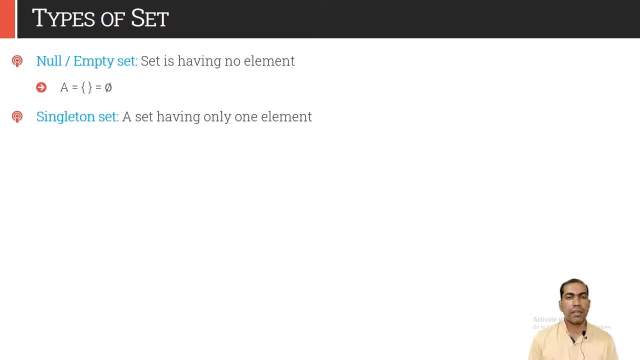 zero element, it is known as a null set or the empty set, and if it is having exactly one element, it is known as a singleton set. so obviously, phi is not a singleton set because it does not have any element within this. this is singleton set because it contains phi as the only element. 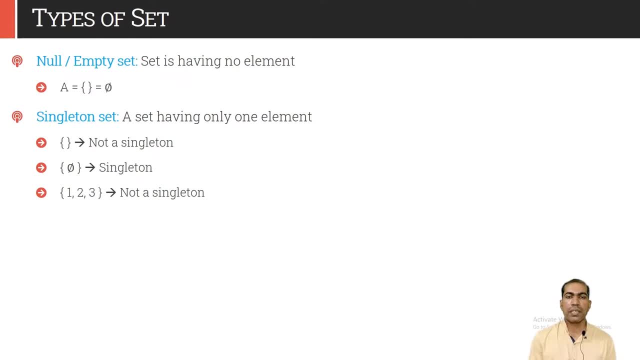 this is not a singleton because it is having three elements: one, two and three. but this is a singleton because the set has only one element, which is set. now, this set could have size one, two, three or infinity, does not matter. the outer set has only one element, which is the inner set. that's why this. 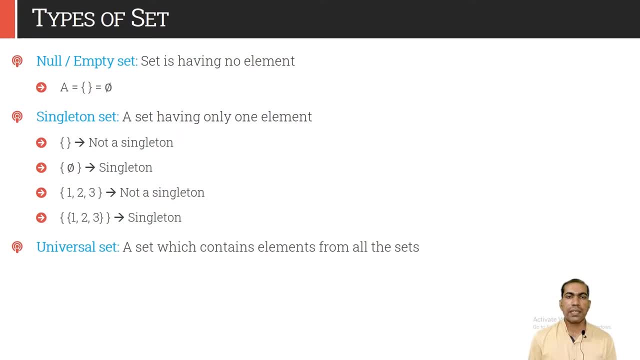 is known as a singleton set. universal set contains element from the all the sets. so many times universal set may be stated explicitly, or many times only sets are given. so to compute the universal set we should take union of elements of all the sets. universal set is typically represented by capital u or capital x. 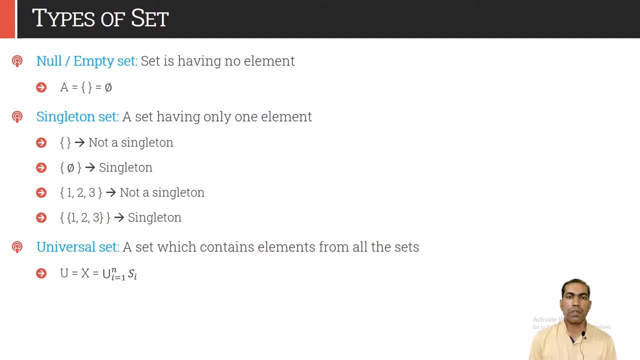 that is nothing, but it's a union over i is equal to one to n si, where si represent ith set. so if there are n sets in the domain we should take union of all the sets: s1 union, s2 union, s3 union up to x, s, n. that will give us the 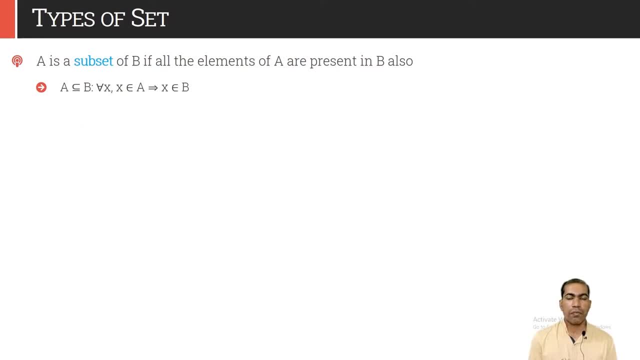 universal set a is subset of b. if all the elements of a are present in set b also, it is represented by a subset b notation and mathematically we can say that for all the elements x which are member of a should be also member of b. then we can say that a is subset of b. 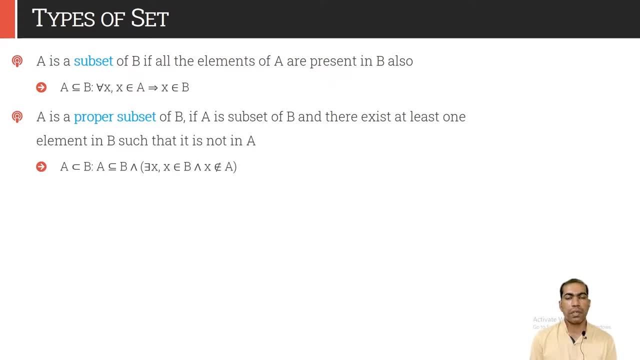 a is proper subset of set b if the first condition a is subset of b as well, as there should exist at least one element in b which is not in a. so in case of subset a and b could be identical set. but for proper subset a and b will not be equal. b will be larger set which contains all the element. 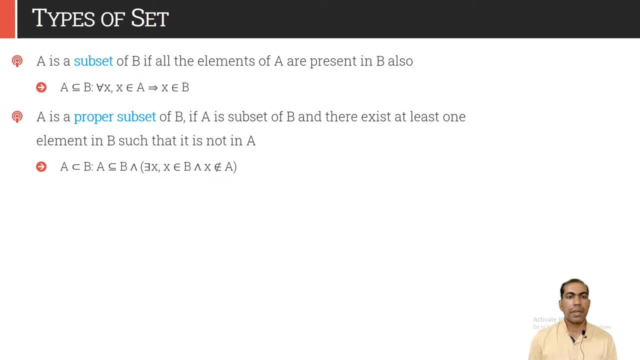 of a as well as it is having some additional element. mathematically a proper subset is like a proper subset b. it means a is subset of b and there should be at least one x in b such that it is not in a. phi is always subset of any set. it is subset of itself also, as well as set itself is. 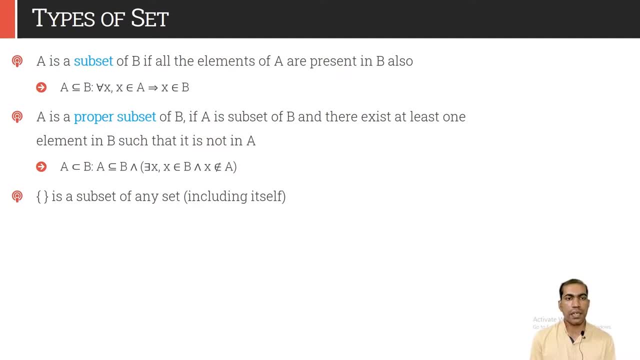 always a subset of itself. okay, so phi and set itself will be always part of subset of any set, and for phi cannot have proper subset. for finding the proper subset we need a smaller set compared to the given set. but phi itself is a set without any element, so it is not possible to derive set less than that, or 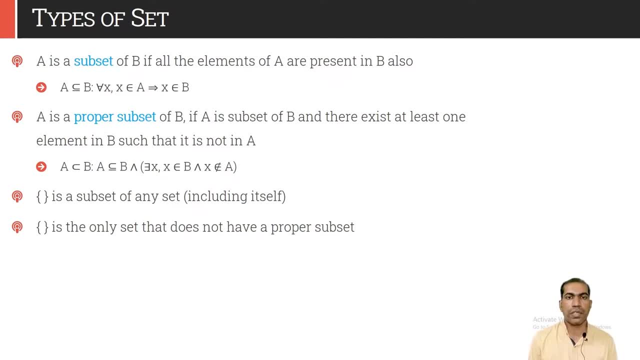 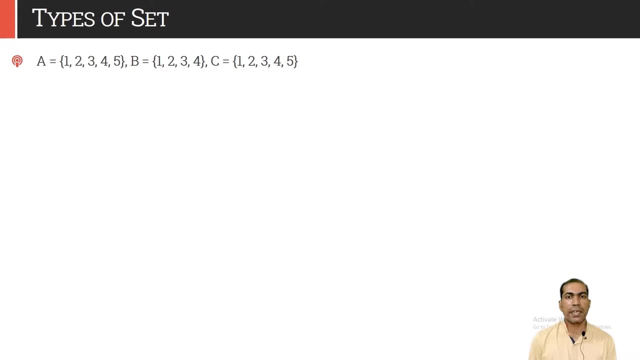 smaller than that. so phi cannot have a proper subset. let's try to understand it with the example. uh, set a, b and c are given like this, where a and c are identical sets with element 1, 2, 3, 4, 5 and b is. 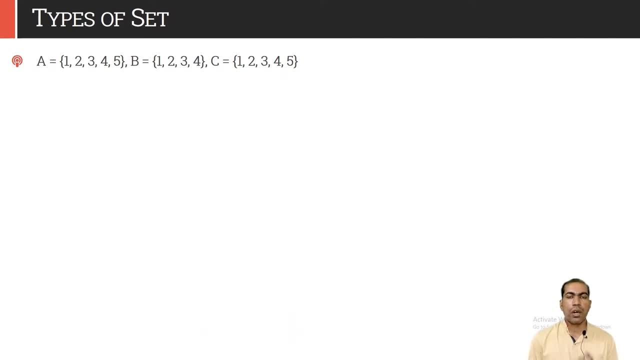 in somelikable. the general one's set below the limit seems to be. similar section to c in a to the sum of all the elements of a to c is also relate to a. c is subset of b as they are attached to all elements of b. 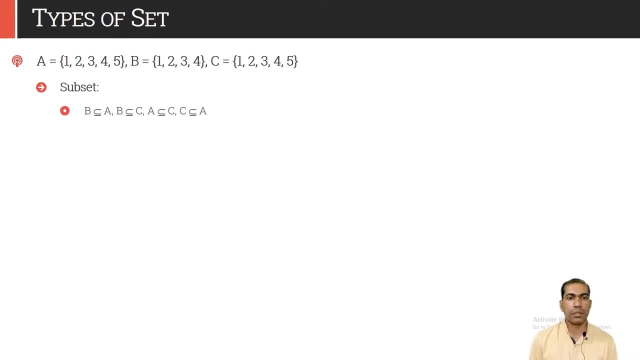 now let's study a friendly. Så the daqui demás house's. each element comes from a to a and a is also a. so as we canано say that all the elements of b is in a as well as in c, so we can say that b is a subset of a and b is c and all the elements of a are present, C. 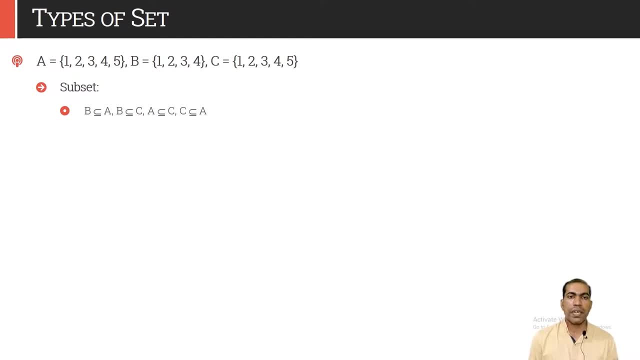 for proper subset there should be at least one additional element in the set. fine, So B is proper subset of A as well as C, because A and C is having a one extra element compared to B. So we can say that B is proper subset of B and C, but A is not a proper subset of C and C is not a proper subset. 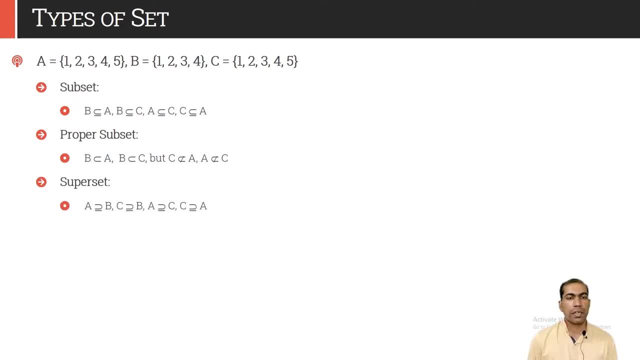 of A because they are identical. Similarly, if we talk about a superset, we can say that A is superset of B and C is superset of B, because all the elements of B are present in them. Similarly, A and C are identical sets. So all the elements of A are in C, as well as all the elements of C are in. 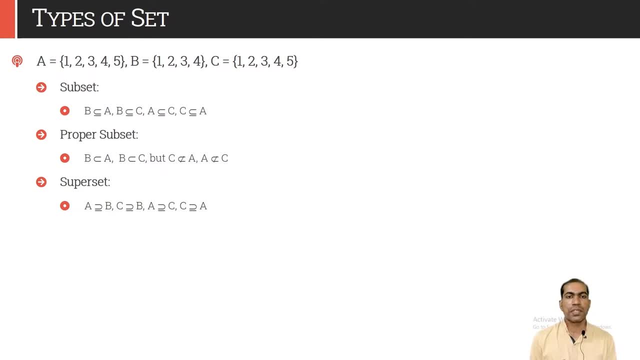 A. So we can say that A is superset of C and C is superset of A. But if we talk about a proper superset, then superset must have some additional element compared to the given set. So A is proper superset of B and C is not a proper superset of A. So we can say that A is proper superset of B and C is. 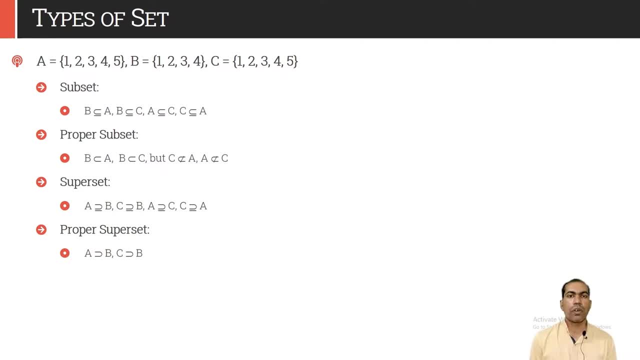 also proper superset of B. but that is not true for A and C because there is no additional element either in A or in C. Power set is collection of all the subsets of given set and typically it is represented by P of A or 2 power A: The cardinality of the power set: A is same as 2 power cardinality. 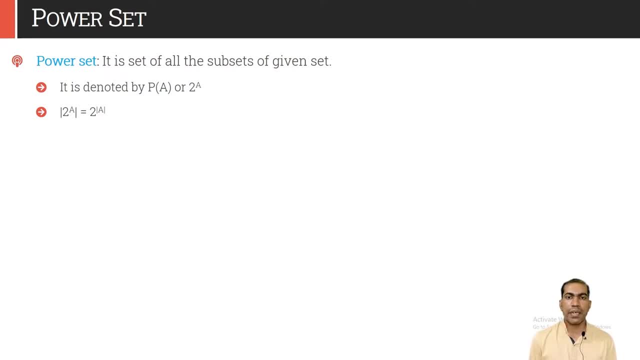 of set A itself. So if set contains an element, then power set will contain 2 raised to n elements. Let's consider set A is equal to A, B, C. It has 3 elements, So its power set would contain 2 raised to 3,. 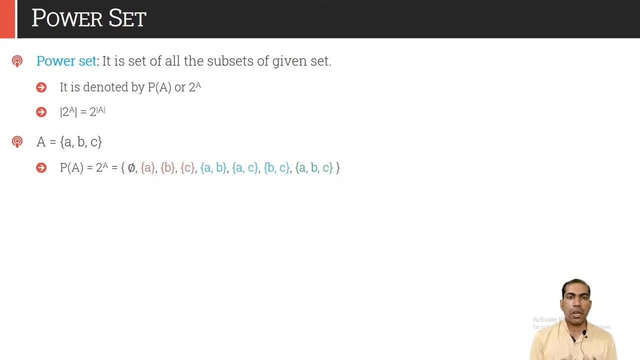 that is, 8 elements. So we will start forming all possible subsets of A. By definition we know that null set, or the phi, is always going to be subset of any set. So that is the set of size 0. Then we will create all the possible subsets of size 1.. So as there are 3 elements- A, B and C- the possible- 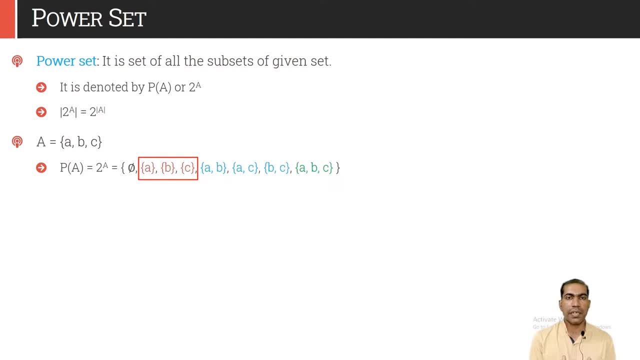 subsets of size 1 would be 3, that is, set A, B and C. So we will create all the possible subsets of size 1.: Set A, set B and set C, shown in red. Then we will form all the possible subsets of size 2.. So first we will create a subset A- B, then A C, then B C, shown in blue. 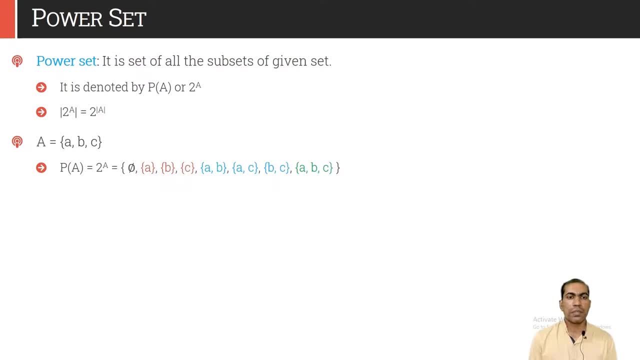 And finally, we will create all the possible subsets of size 3, but set itself is of size 3.. So we can create only one subset of that. that is A, B, C itself B is empty set, It does not contain any element. So its power set would contain 2, raised to 0. 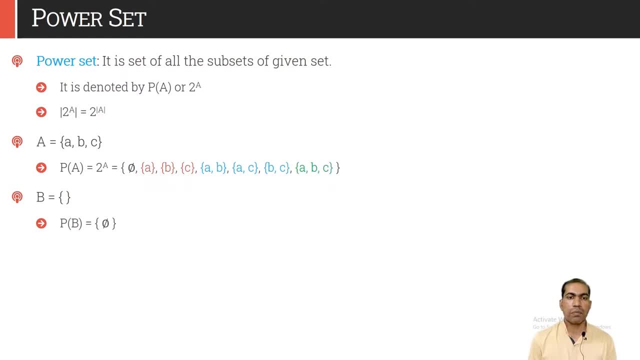 That is one element And by definition the phi is always the member of subset of any set or the power set of any set. Here C contains exactly one element, which is phi, So its power set will contain 2 raised to 1, that is 2 element. 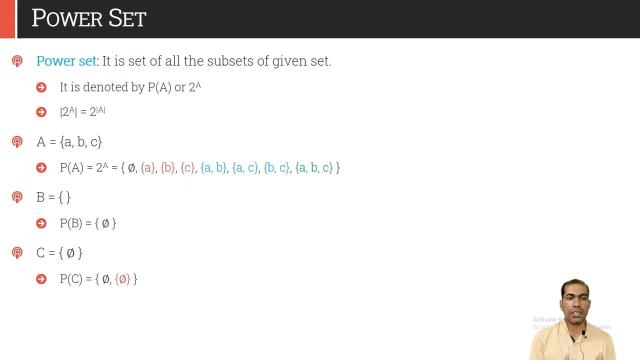 The first one will be phi itself and second one will be the subset of set C. But C contains only one element, phi, So the subset of that would be set phi. D contains 2 element, phi and set phi, So the power set of D will have 2 elements. 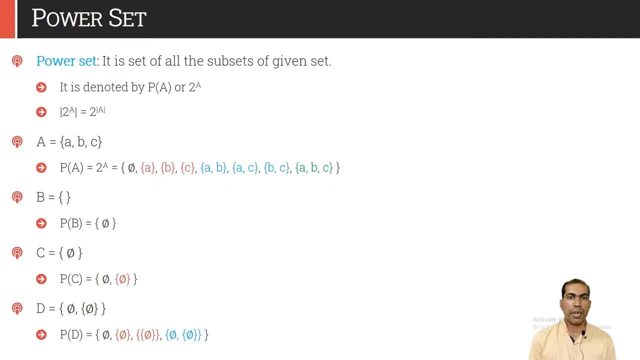 So we will have 2 raised to 2, that is 4 element, So that would be phi by definition. Then we will create 2 subsets, each of size 1, because size of D is 2.. So first one will be set phi, Second one will be set of set phi. 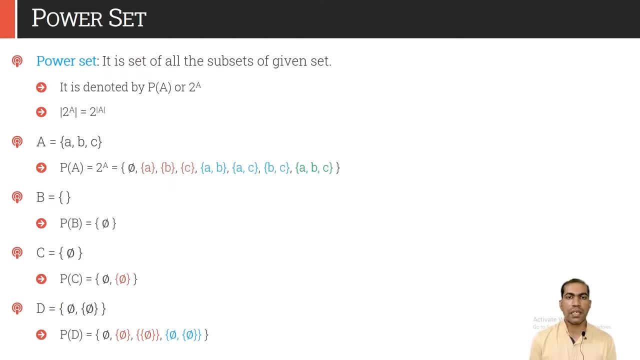 And finally, we will create a subset of size 2, that is the set itself. So set D will be the member of the power set. Let us compute 2 raised to 2, raised to A- B. That is, we are computing power set of power set of A- B. 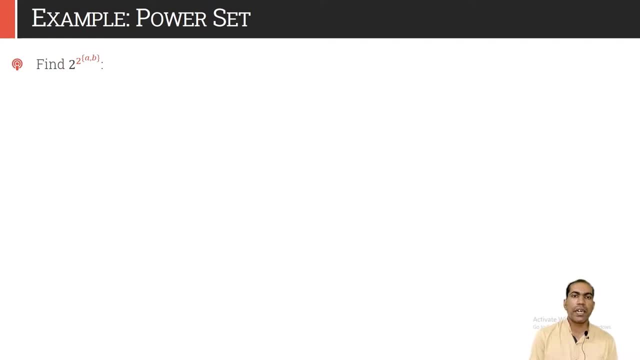 So first we will calculate power set of A- B, And then we have to again find power set of that. So by now we know that power set of A B would be phi A B and A- B, And now we have to take the power set of that. 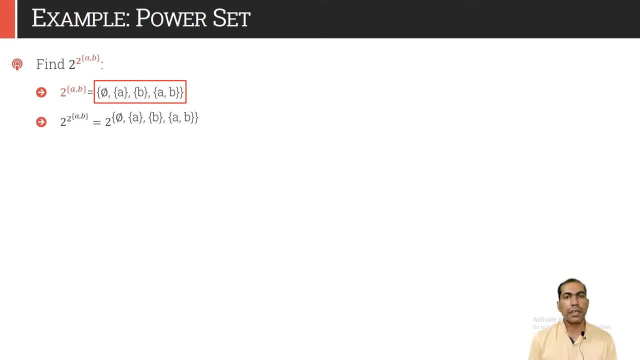 So this set contains 4 elements. So power set would have 2 raised to 4, that is 16 element. So first we'll list out all the elements of size 0. So that is phi only. Then we'll create subsets of size 1, as there are 4 elements into the set. 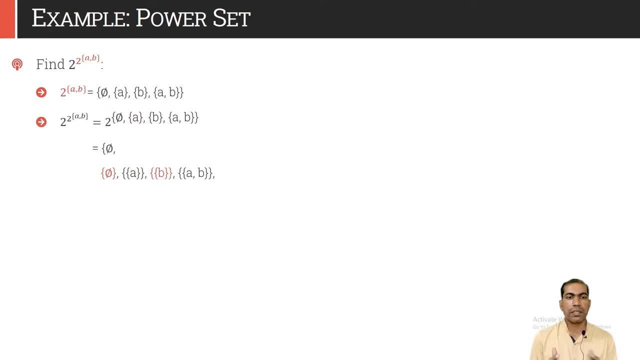 We can create 4 subsets each of size 1, that is, phi, A, B and A, B. Then we'll create subsets of size 2.. So first phi and A, phi and B, phi and A, B and A and B, A and A, B and B and A B. 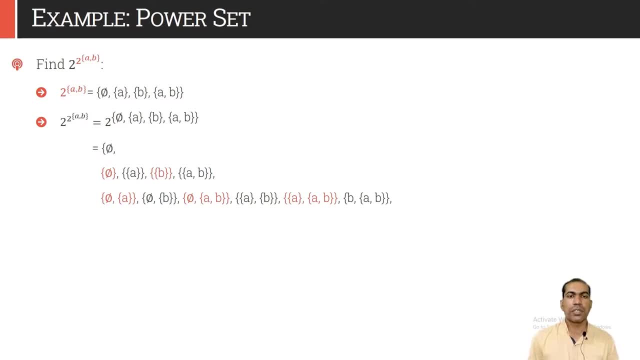 So all these possible combinations are of size 2. Then we'll create all the subsets of size 3. So we'll take phi A and B, That will be the first element, Then phi A and A B, That will be the second element. 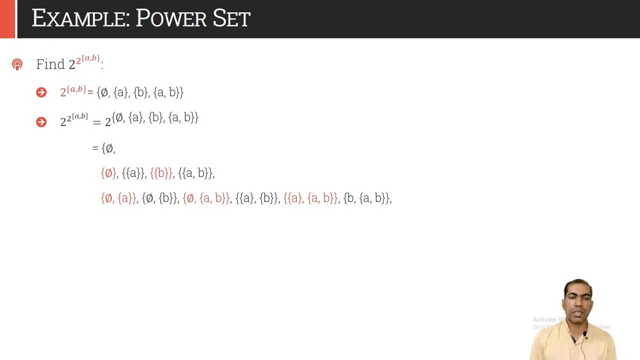 Phi B and A B. That would be the third subset. And A B, A B, That would be the last element of size 3.. And finally, subset of size 4.. That would be the set itself. 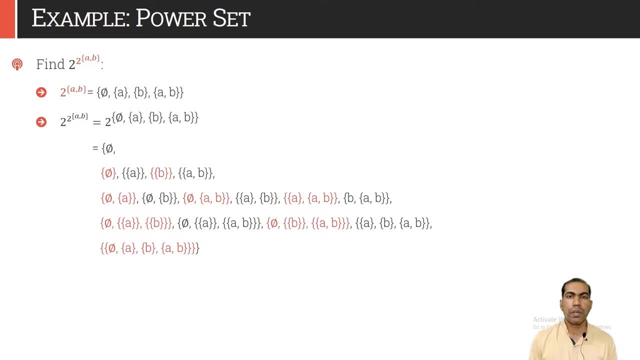 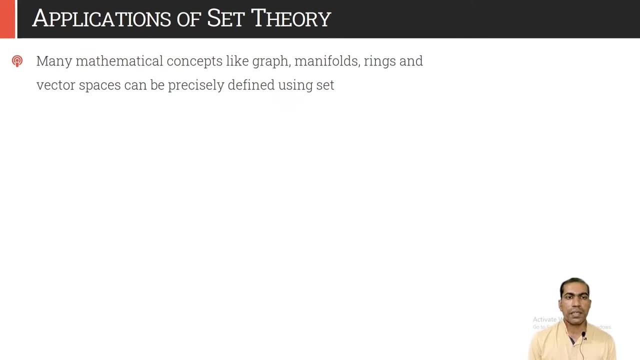 So, as you can see that we have 16 elements into 2 power, 2 power A B. That is the power set of power set of A B. Let us talk about few applications of set theory. So many mathematical concepts like graphs, manifolds, ring. 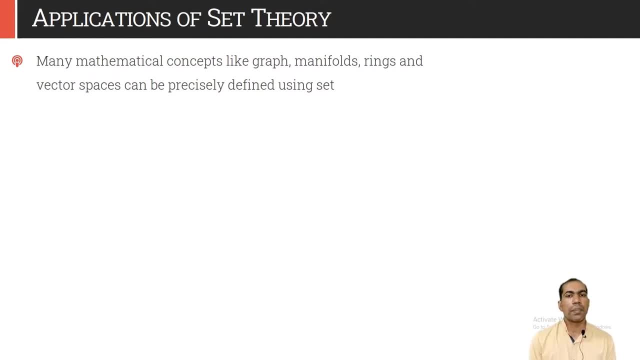 metoids, vector space, etc. are precisely defined using the set. So set is fundamental representation in all these concepts. Even many data structures are also using set as the basic notation. Many computer science problems are also using set. very frequently All the number systems are using set as their basic representation, like set of natural numbers. 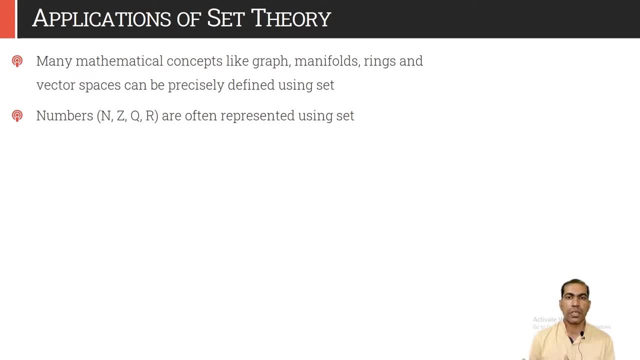 So that is enclosed within set. So that is enclosed within set. So that is enclosed within set, So you can get set as the default in curly bricket: one, two, three and so on, Set of complex numbers etc. Set theory is foundation of discrete mathematics and set theory is also used in many abstract. 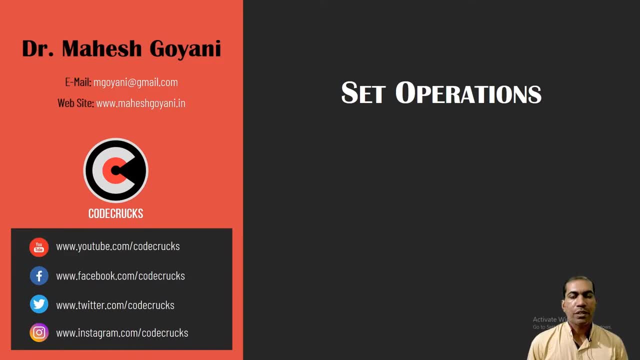 algebra problems. Hello folks, welcome to Code Cracks. This is Dr Mahesh Gujrani and in this video I will be talking about set operations. In previous video we have talked about set representation. We have introduced set and we have seen how we can represent the set. 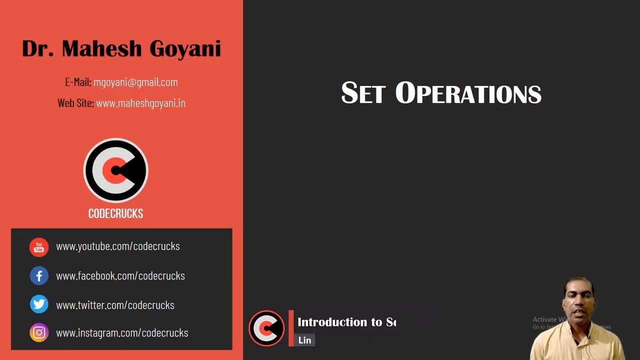 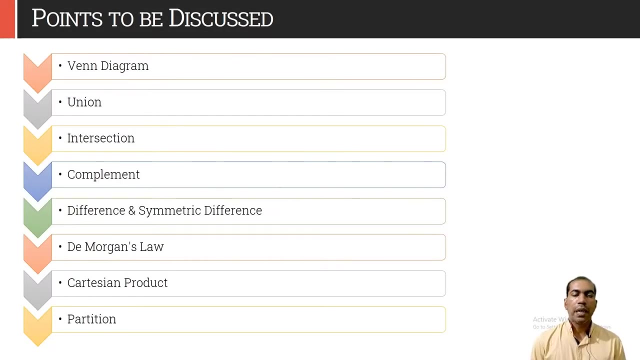 we have also discussed various types of sets. as we know, that set is very important from the perspective of mathematics as well as from the computer science, so it is very important to understand that, what type of operations we can perform on the sets. in this video i'll introduce 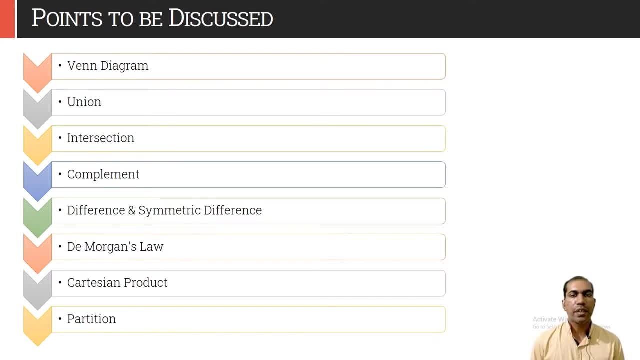 what venn diagram is, and then we'll discuss various set operations like union, intersection, complement. we will be also talking about difference and symmetric difference operation on the set. that will be followed by de morgan's law, cartesian product and at last i'll talk on partition of the set. mostly we are writing sets in curly bracket notations. we are writing the. 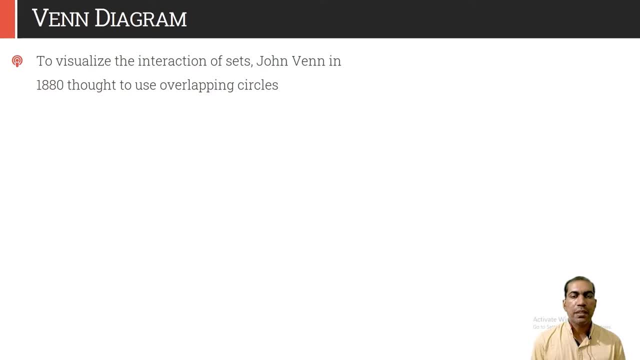 elements within the set. so when we have multiple sets, it is difficult to understand the relationship between the sets if they are written in form of curly brackets or they are written in form of conventional way. so what is the interaction between the set? how sets are correlated. it is 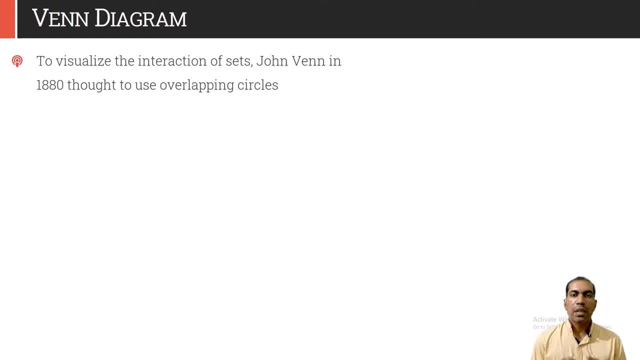 difficult to understand the relationship between the sets if they are written in form of conventional way. so what is the interaction between the set? how sets are correlated, it is difficult to understand from just textual data, but it would be better if we can represent the same thing in. 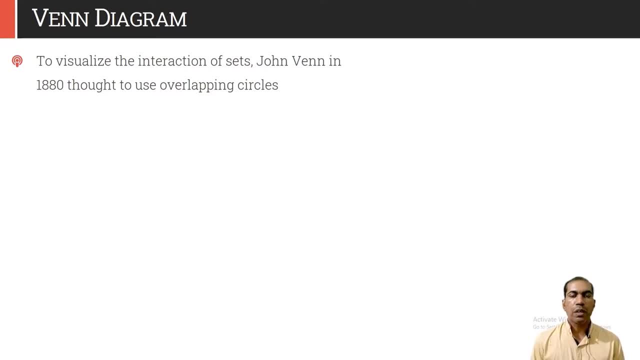 graphical way. so john venn has proposed a notation, which is known as a venn diagram in 1880s, in which each set is represented by a circle. here yellow circle represents set a, blue circle represents set b and the green part is common in both the sets. so a union b operation is given by combining. 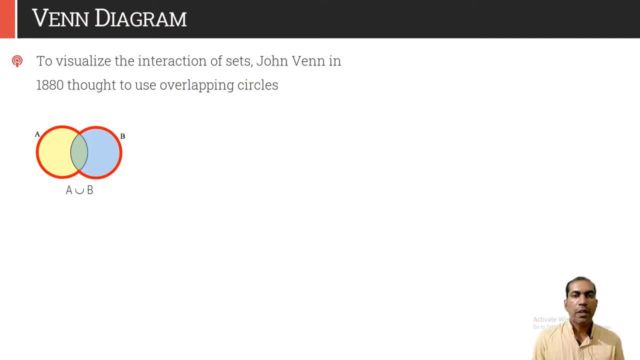 all the elements from both the sets. so the red boundary of both the circle represents union operation a intersection b is defined by common elements within two sets. so the green portion is the common one between two circles. so that particular part highlights a intersection b, operation a complement intersection b. so first we will calculate a complement. a complement means. 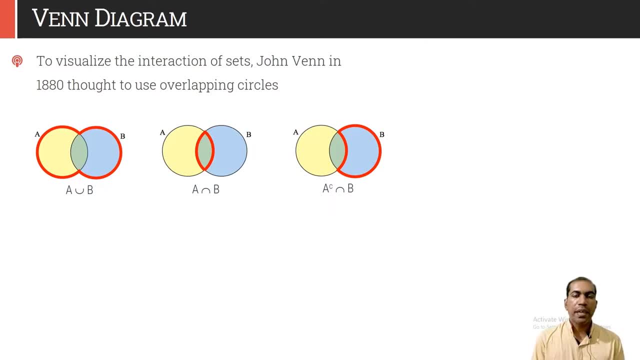 everything which is not in a, okay. and then we are taking a intersection of that with b, so we will be left with this moon shaped blue color. we will try to understand all the operations with the help of example, as well as with the help of venn diagram. 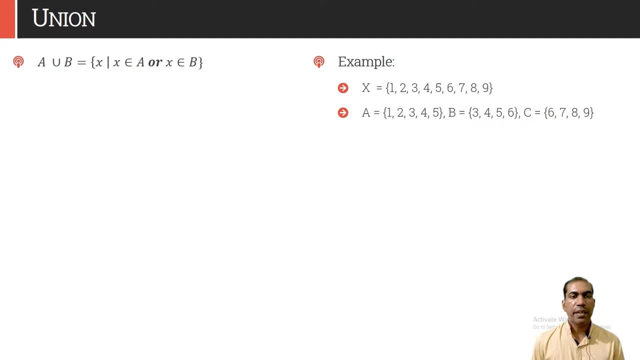 the union of two sets, a and b, is defined as a union b and mathematically it is written using property method or the set builder method as, like this: a union b is collection of all the elements of x, such that X is member of A or it is member of B. So if element is either in A or B, we will be copying. 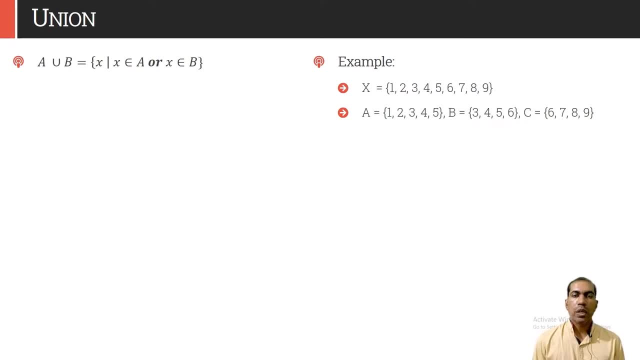 it into the A union B operation. So, as shown here, we have set A, which contains element 1,, 2,, 3,, 4, 5.. Set B contains element 3,, 4,, 5, 6.. So when we take the union of these two sets, 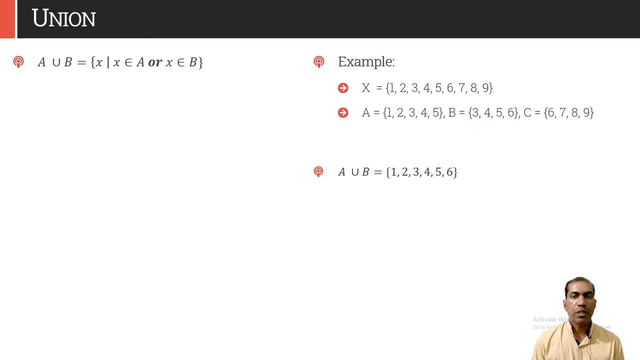 3,, 4,, 5 are common in both And, as we know, that set does not contain repeated elements, So we will be writing them only once. So A union B will be 1,, 2,, 3,, 4,, 5 and 6.. 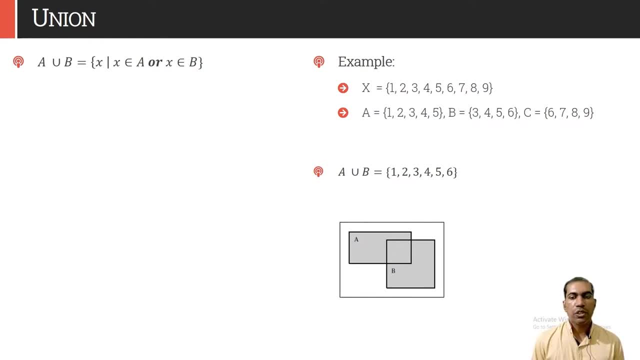 In Venn diagram, representation A union B operation is shown like this: The outer rectangle is known as a universal set, that is, capital X. Inner two rectangles represents set A and B, and the gray region represents the output of the operation. A union B contains all the elements. 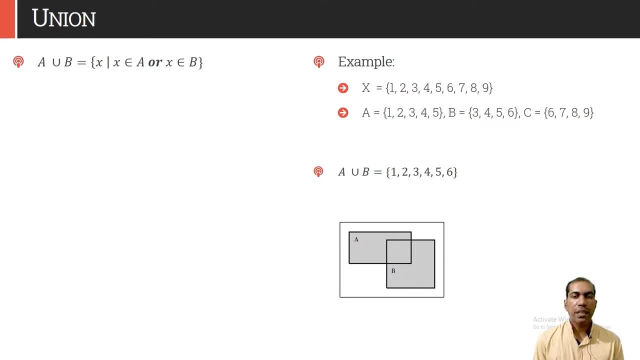 from set A as well as from set B, So we will be writing them only once. So A union B will be set B. The everything in A and B is of gray color. A intersection B is given by the common elements in both the sets. So mathematically we can denote A intersection B as collection of. 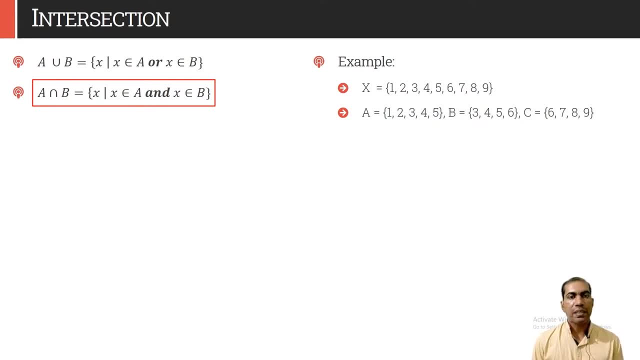 all the elements X, such that X is in A and X belongs to B. So here element must be present in both the sets A as well as B. If we talk about set A and B shown here, then elements 3,, 4, 5 are the common elements. So A intersection B would be 3, 4 and 5.. The Venn diagram representation. 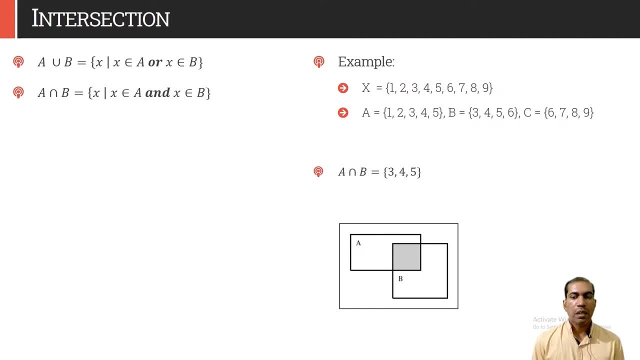 of intersection operation looks like this: The common part in A and B is highlighted into gray, which is the intersection of both the sets. Absolute complement, or often known as a complement operation, is given by omitting all the elements of set A from the universe. It is typically 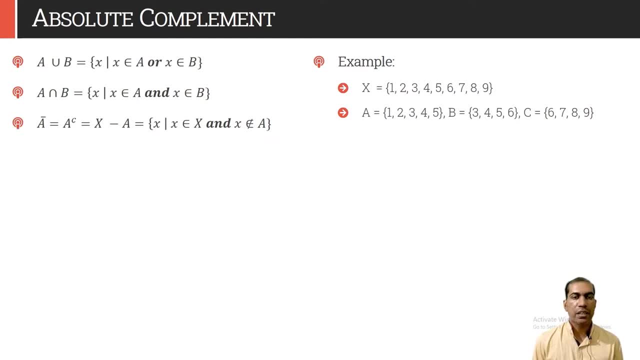 represented as A bar, A bar or A complement or A dash. Using set melter method we can write complement as collection of all the elements X, such that X is in universal set but it is not part of set A. It means we have to simply subtract all the elements of A from capital X. So 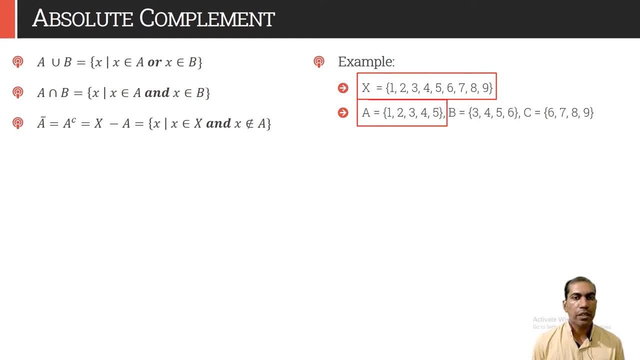 here X contains 1 to 9,, A contains 1 to 5.. So when we perform the complement operation of A, it would take only 6,, 7,, 8 and 9.. When we perform the complement operation of A, it would take only 6,, 7,, 8 and 9.. 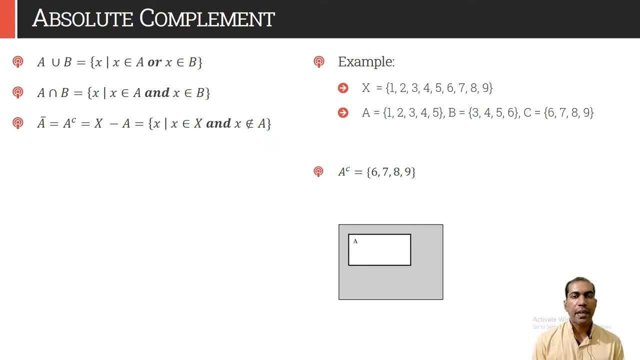 In Venn diagram we can represent complement operation like this. A complement, it means everything which is not in A but in universe. So this grayed region is the output of A complement operation, Relative complement, or it is also known as a difference Absolute. 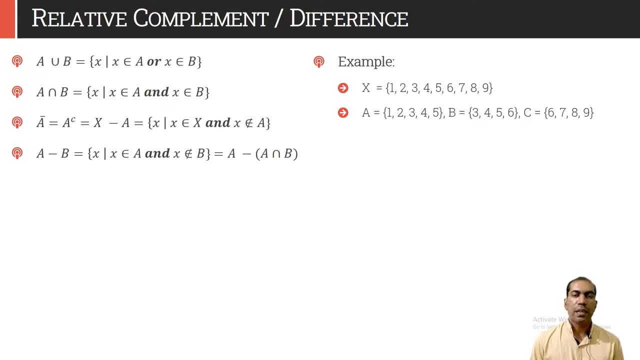 complement is taken with respect to universal set. Relative difference is computed with respect to sets. A minus B is given as collection of all the elements of X, such that X is in A but it is not in B. Fine, Or in another way. we can write it like: A minus A, intersection B. 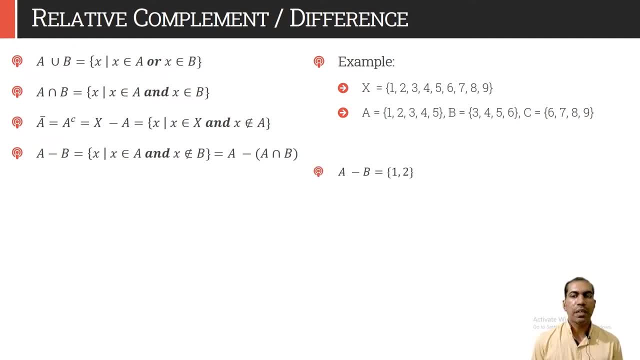 So if you would like to calculate it, A minus B would be simply 1 comma 2.. And the Venn diagram representation of that looks like this: We have to subtract all the elements of B from A. So whatever is left, that is A minus B Symmetric difference. it is actually a union of two of us. 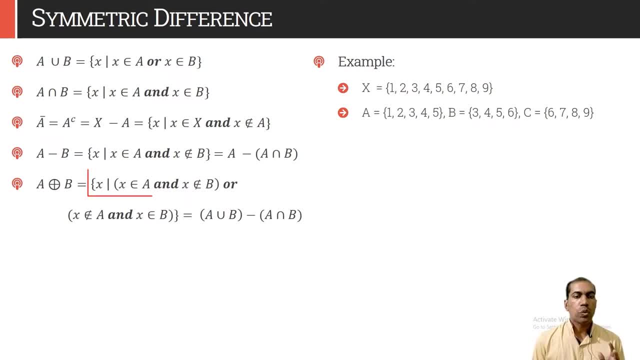 So it is a collection of all the elements X, such that X belongs to A but it does not belong to B. So this part forms A minus B And we have to take the union of that with B minus A. That is, X belongs to B but it does not belong to A, The another way of representing 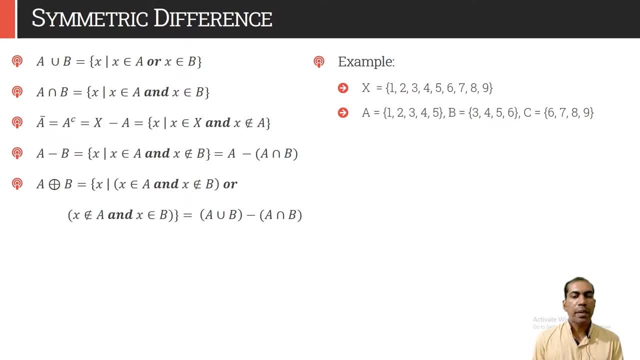 symmetric difference is A union B minus A intersection B. Let us subtract. Let us subtract to calculate for the given data. So A union B would be 1, 2, 6.. A intersection B is 3,, 4, 5.. 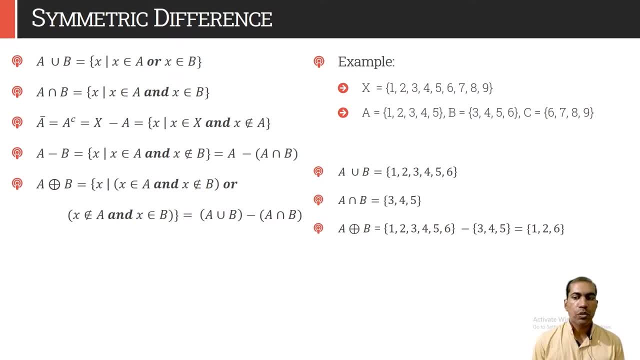 So we have to subtract this intersection from the union. So the symmetric difference of A and B would be 1, 2, 6.. The Venn diagram representation for the same looks like this: So we are subtracting the common part in both the sets from union of that De Morgan's law. it is very important and 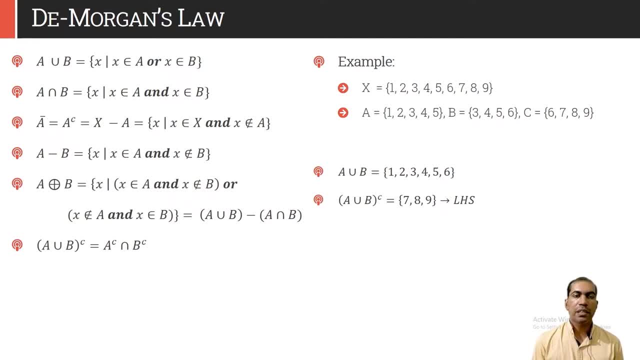 very popular law. It is very often used in reduction of set operations. The first law says: A union B whole complement is same as A complement intersection, B complement. So let us first calculate A union B whole complement. So A union B is 1,, 2, 6.. We will subtract it from the capital. 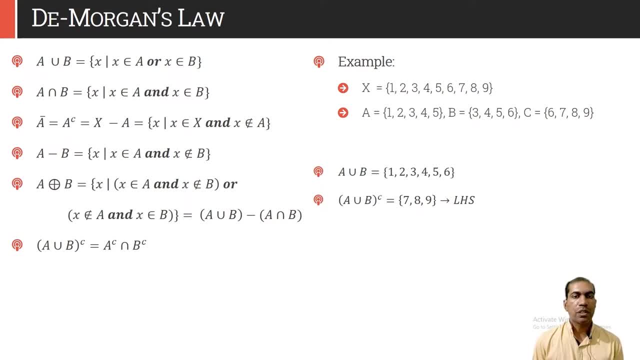 X. So we are left with 7,, 8,, 9.. So this is the output of left hand side of this equation. Let us find out A complement, B complement And intersection of that. So A complement is simply 6,, 7,, 8, 9.. B complement is 1,, 2,, 7,, 8,, 9.. 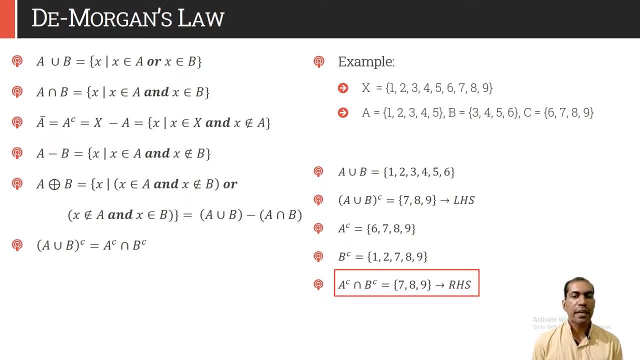 And their intersection is 7,, 8,, 9,, which is the right hand side of this operation. So as we can see that LHS and RHS are identical- Fine Hence this law is proved Graphically- we can represent: 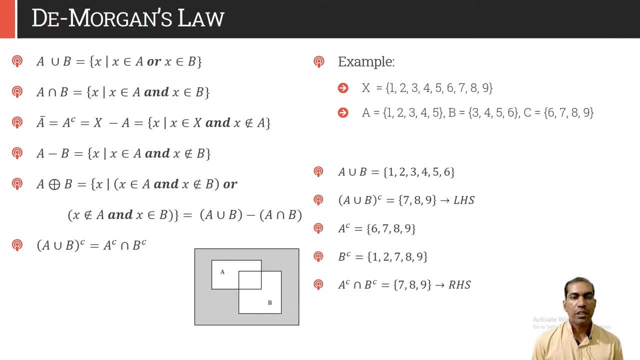 this law using this diagram. What we are doing is we are taking the A union B And then we are taking the complement of that. So everything which is neither in A nor in B will be in A union B whole complement. The another law of De Morgan is: A intersection, B whole complement is equal to. 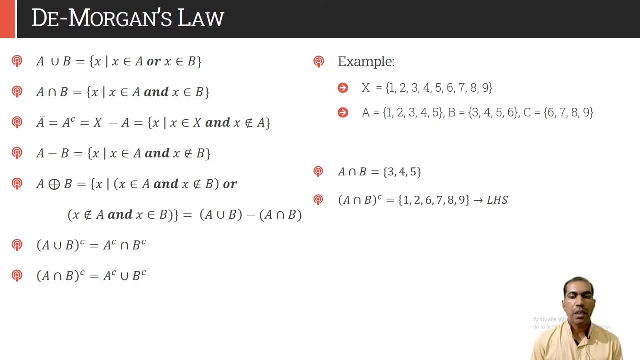 A complement, union, B complement. So as we can see that A intersection, B whole complement is 1,, 2,, 6,, 7,, 8,, 9.. Then we will calculate A complement, B complement. We will take the union of that That. 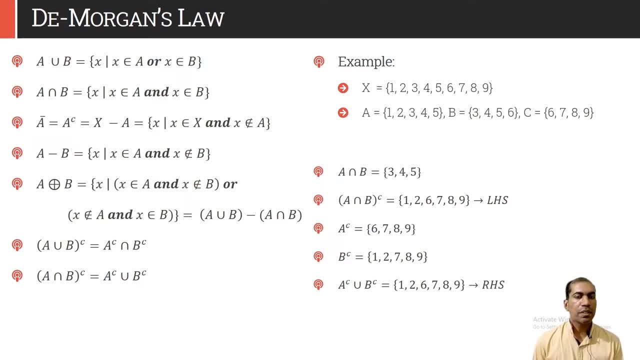 is nothing but 1,, 2,, 6,, 7,, 8,, 9.. Which is same as LHS, And hence this law is proved, And graphically we can represent it like this: What we are doing is A intersection B, So that is the common elements in both the sets, And 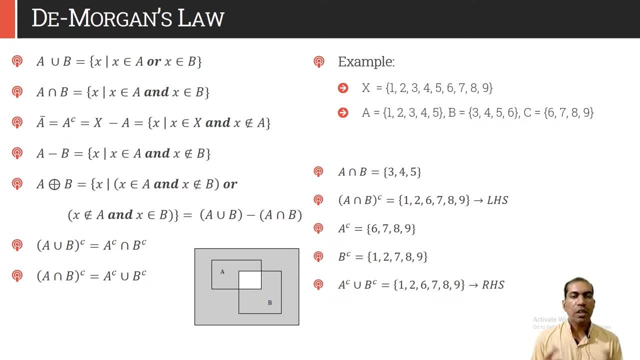 then we are taking the complement of that. So everything which is not in complement will be the part of this. So the region is shown in gray color. Cartesian product, which is represented by set of tuples rather than individual elements. So A cartesian product, B. 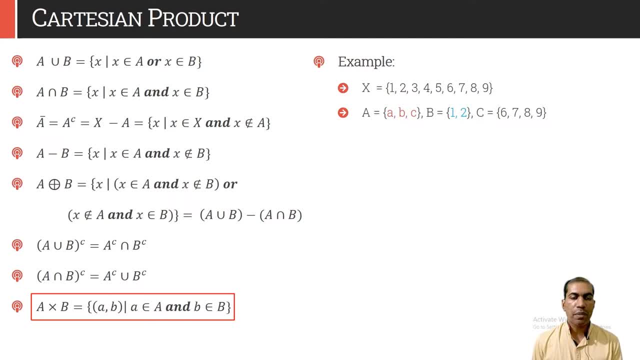 is given as collection of all the tuples A- B, such that the first element, small a, comes from set capital A and second element in tuple small b, comes from set capital B. So here order within tuple is very important. It must be A- B, First element must come from set A and second element 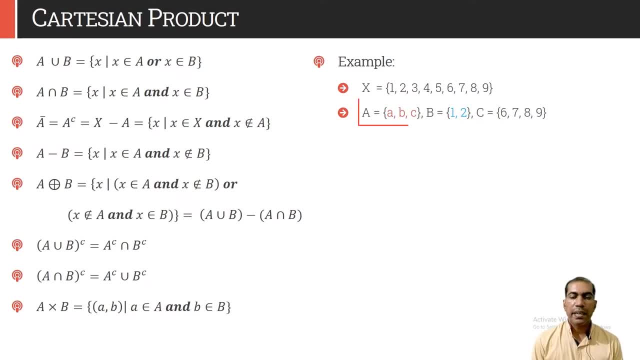 must come from set B. Let: set A is equal to A, B, C and set B is equal to 1, 2.. So to compute the cartesian product between A and B, we need to associate each element of A with every element of B. So we will relate A with 1, B with 1, C with 1.. Then A with 2, B with 2 and C. 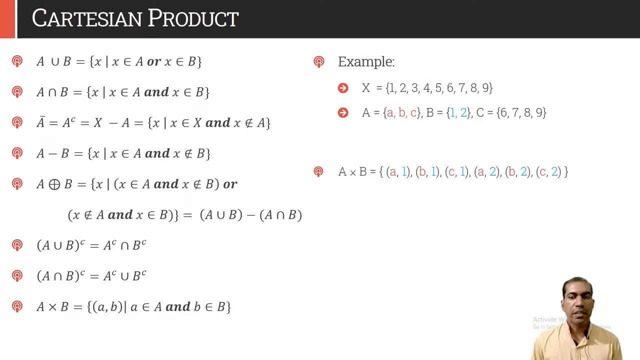 with 2.. So cartesian product between A and B is given as A comma 1, B comma 1, C comma 1, then A comma 2, B comma 2, C comma 2.. The first element in all the tuples are coming from set A. 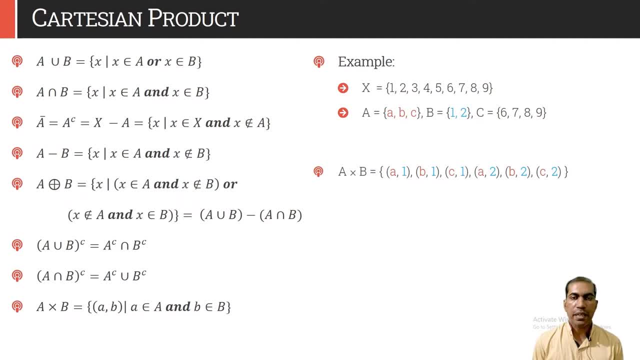 B and second elements in the tuples are coming from set B. The tuple itself is an individual element in set. So if we are writing in this way or in this way, they both are same. We can alter the order of tuple, but we cannot alter order within the tuple. So whether I will write, 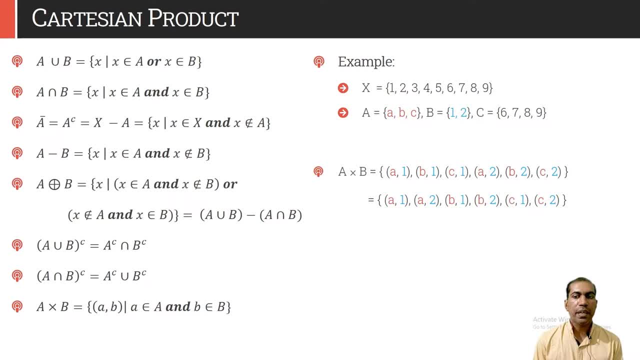 A1, B1, C1, A2, B2, C2 is same as A1, A2, B1, B2, C1, C2.. As we know, that set is unordered collection, So order does not matter. 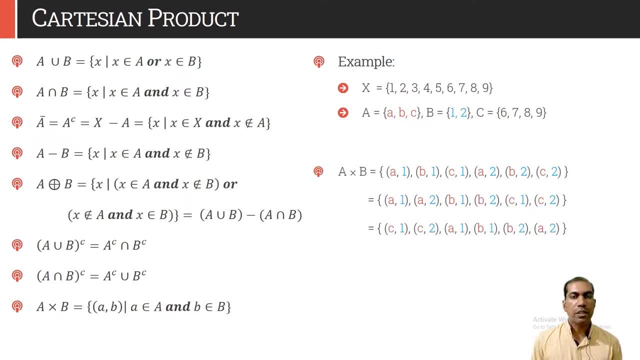 Or I can write like this also: C1, C2, A1, B1, B2, A2.. So all this corresponds to A cartesian product B, but it is not same as 1A, 2A, 1B, 2B, 1C, 2C, Because here the first element is coming. 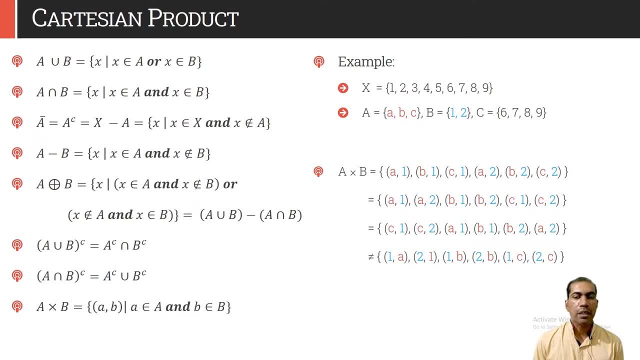 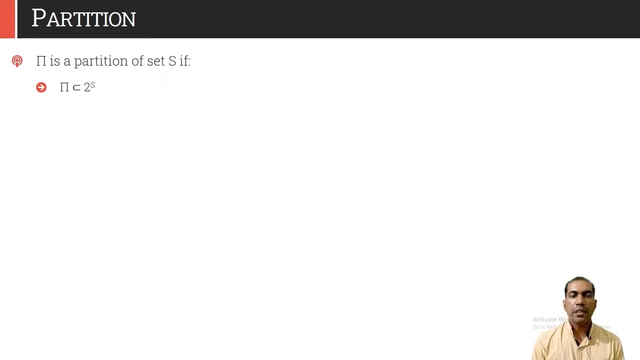 from set B and second element is coming from set A. So actually this is B cartesian product A and A cross B is not same as B cross A, the partition operation. It is represented by symbol pi, So pi is partition of set S if it satisfies following. 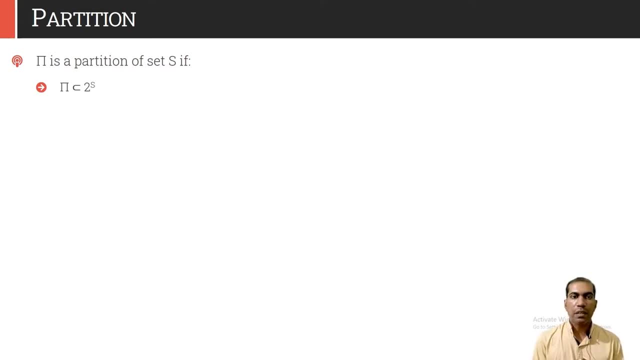 condition. The first condition is that the partition must be proper subset of power set of given set. So what we are doing is we are dividing the given set into subparts and those subparts must be subset of the power set of given set. That is the first condition. 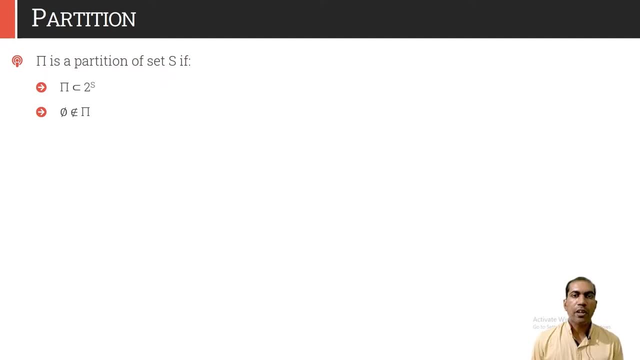 The phi must not be present into the partition. Phi cannot be member of any partition. The third one is if we select any two component of the partition and if we take the intersection, it must be null. It means whatever partition you are deriving in those subparts, element must not be common. And the final condition is that 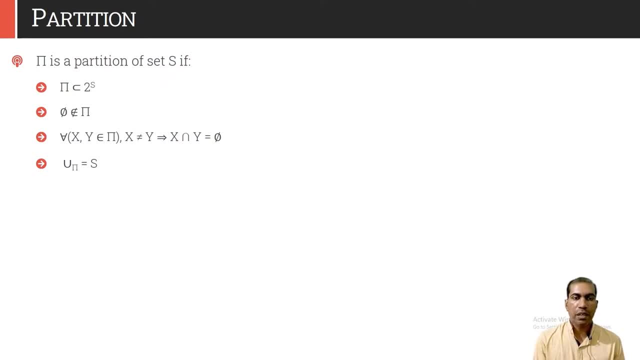 when you take the union of all those components of partition, then it should again give us, or it should be able to generate, the set itself. Consider the set A, B, C, D, E, C, D, E, C, D E, F. We can create random partitions of that. Assume that one of the possible partition 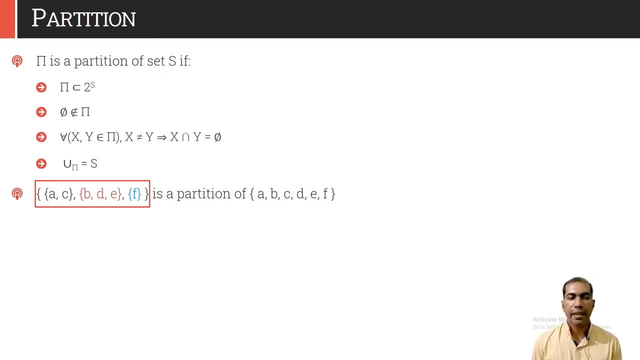 we have created is like A, C, B, D, E and F, So this partition contains three elements. Now we will check whether this is valid partition or not. So the first thing is pi. So this is partition is represented as a pi. Pi must be proper subset of power set of given set. 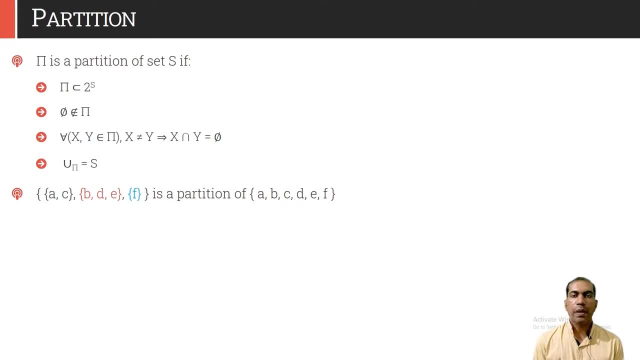 So the given set contains six elements, So its power set will have 2 raised to 6.. That is 64 elements. All the elements of this partition are definitely part of power set of S, So the first condition is satisfied. Pi is not member of this partition, So second condition is also true. If we select 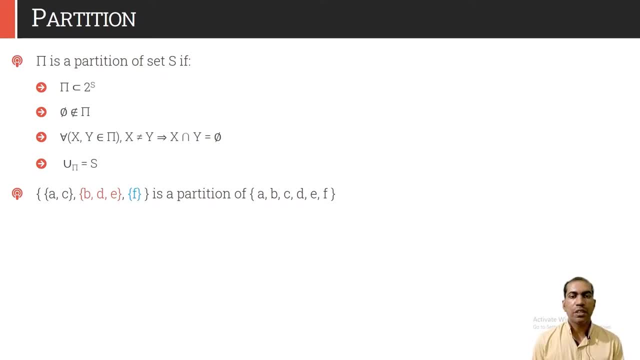 any two components from this partition, then their intersection must be null. So if I will take A, C and B, D, E, there is no common element. A, C and F, no common element. B, D, E and F, there is again no common element. It means this condition. 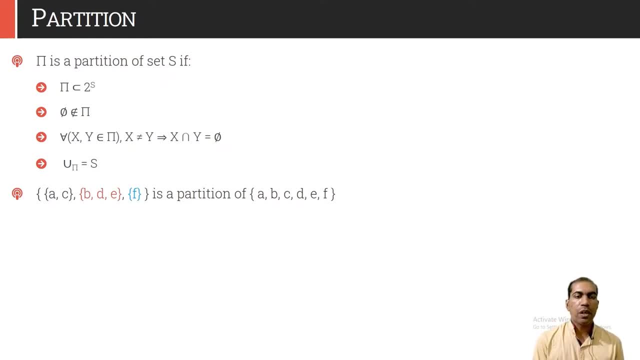 is also satisfied. If we take union of all the elements of this partition, it is generating set S, So this is a valid partition. So partition must satisfy all these four conditions. If we create partition like this, then this is not a valid partition. The reason is that 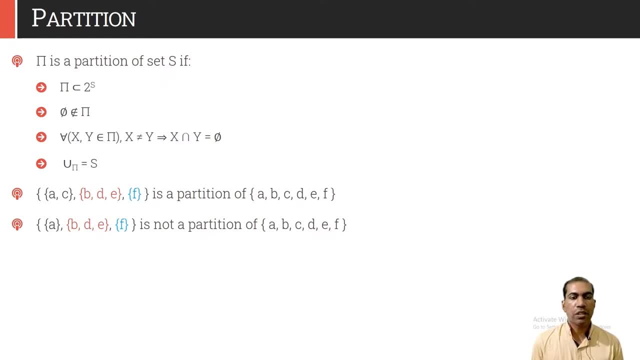 when we take the union of this, it is not generating the original set. The element C is missing. If we create partition like this, then also it is not valid, Because B is repeated in two components, A B and B D. So this is also not valid partition. 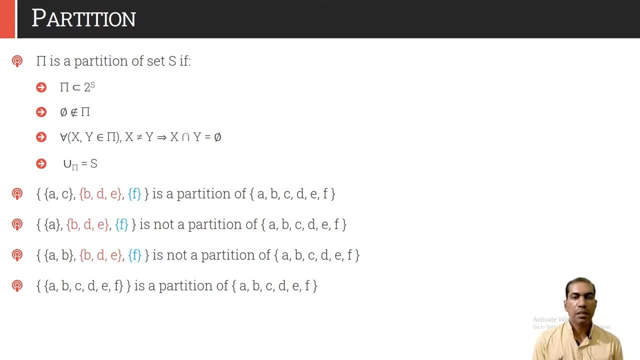 This is valid partition. We have generated only one component of the partition of the set. This is also valid partition. So there is no restriction how many elements should be there. You can create n number of elements if there are n elements in given set. So 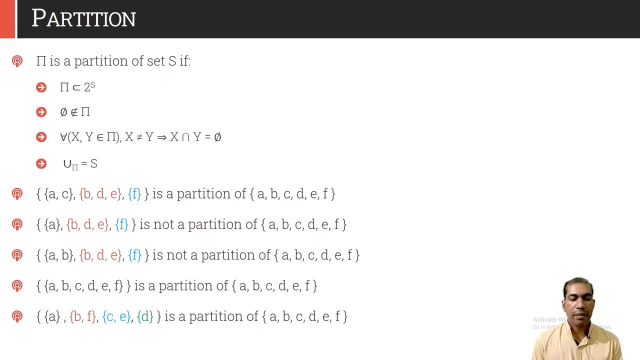 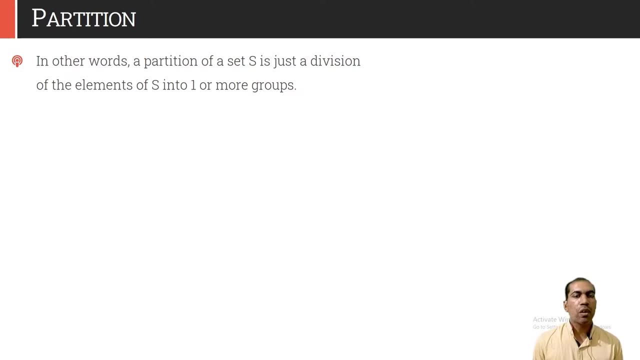 minimum you have one element, maximum you have n elements. So in other words, a partition of set is just division of elements of S into one or more groups. So if you want to compute the partition, that how many partitions are possible for this set, then what we can do 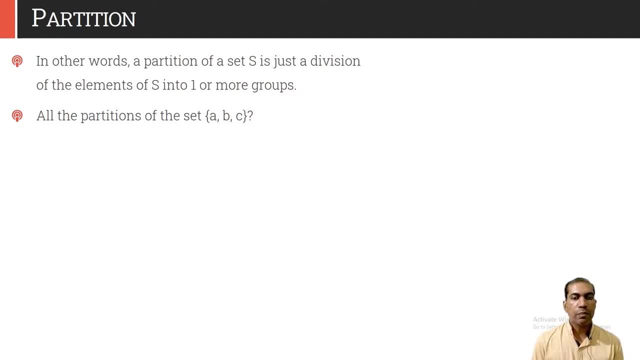 is, we can partition it into smallest possible component. As phi cannot be the member of partition, we will take the size of component as a one. So this is the valid partition, Each component is having only one element. Now, we will try. 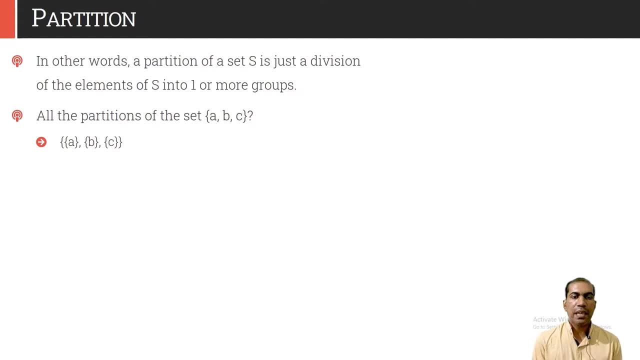 to create component of size 2.. But as the size of this set is odd, one component will be of size 1, other will be of size 2.. So A B C is a valid partition. B A C is valid. 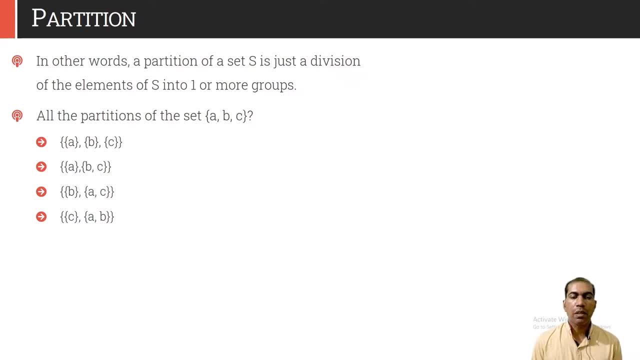 partition, and C, A, B is also valid partition. Now we will try to create a partition with component of size 3.. So only one possibility is there: A, B, C. So for given set we can create five different partitions. 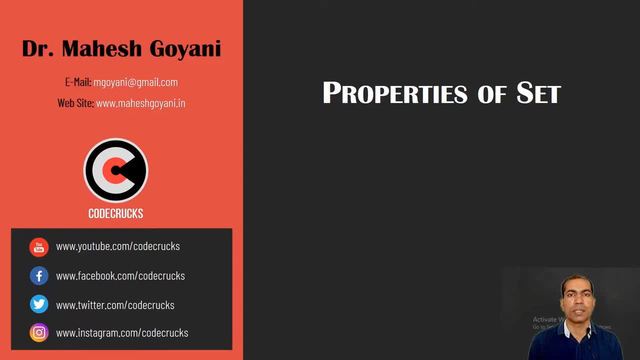 Hello folks, welcome to Codecracks. This is Mahesh Gurnani, and in this video I am going to talk about various properties of the set. In previous video we have talked about various operations on the sets. More often, we are dealing with multiple sets and we are performing. 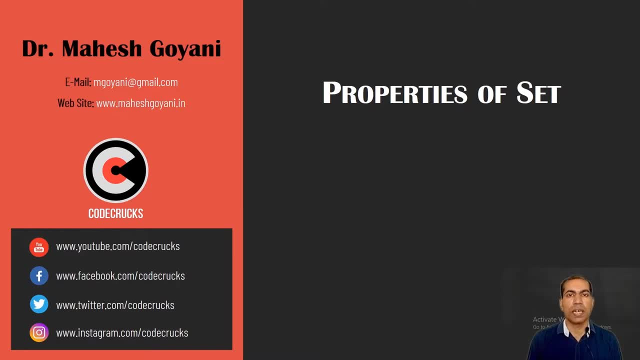 various operations across the sets. The operation can be as simple as union of two sets, or it may be as complex as series of the operations onto the sets. Whenever multiple sets and frequent operations are involved into the experiment, it would take quite a long time. 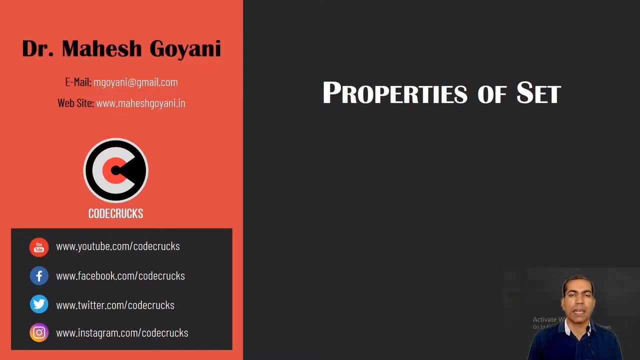 to compute the final result. But by applying the properties of the sets we can reduce those complex set operations into a simpler. So properties of set will help us to reduce the equations and that will help us to get the operations. So let us see how we can. 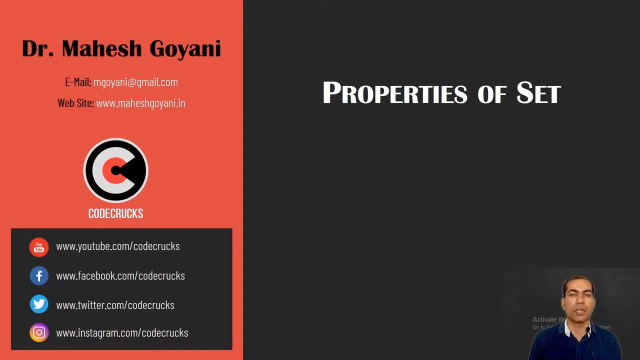 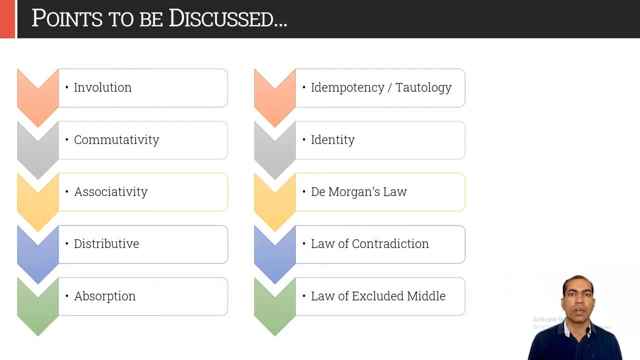 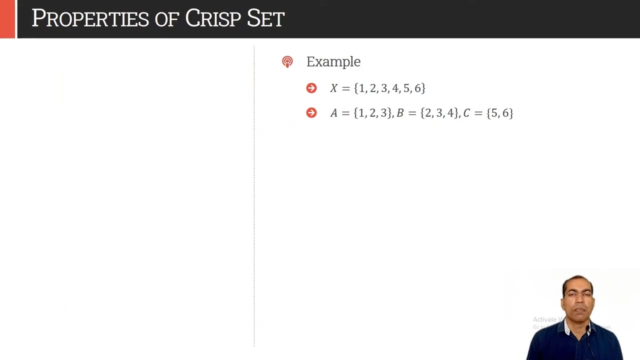 get the output quickly. So in this tutorial I will be talking on different properties of the sets which can greatly help us. In this video I will be focusing on various properties like involution, commutativity, associativity and so on. We will talk all. 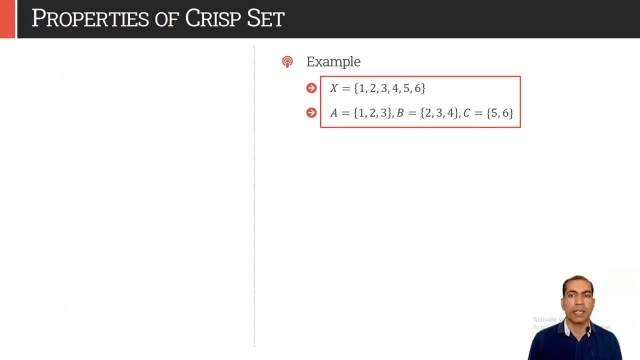 the properties in context of this data Set. A is 1, 2, 3.. B is 2, 3, 4 and C is 5 comma 6.. If we take union of all these three sets, we will get the output quickly. In this tutorial I will be talking on different properties. 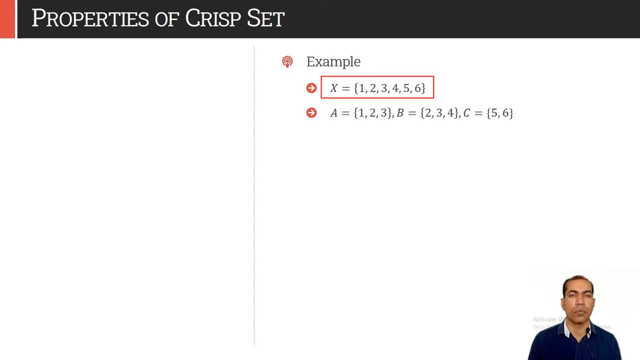 universal set for that, that is, capital. X is equal to 1, 2, 3, 4, 5 and 6. the first property is involution. a complement of complement is equal to a. we already know how to calculate a complement. if you don't know, I advise that please go and. 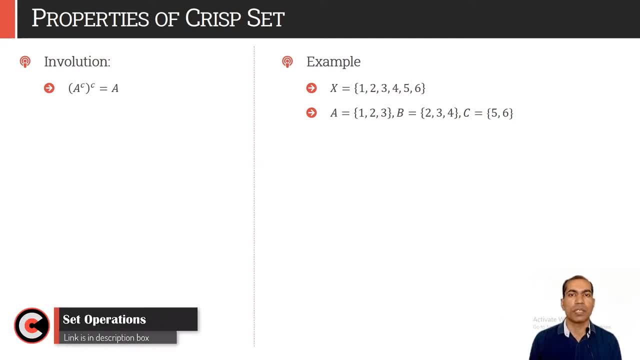 watch the previous video, that is, the various operations on to the sets. the link of that video is given in description box. a complement is computed by subtracting all the elements of a from the universal set capital, X. that is a complement is X minus a, so X is 1, 2, 3, 4, 5, 6. a is 1, 2, 3, so a complement would be. 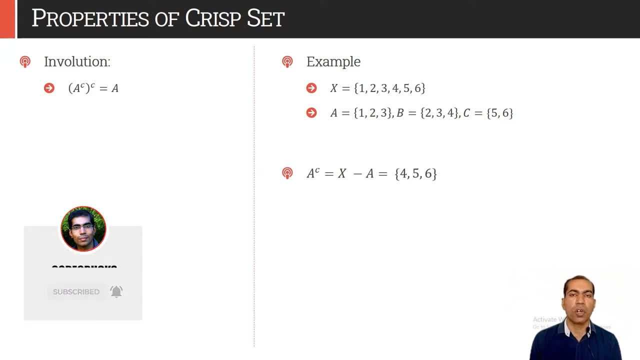 4, 5, 6. we have to take complement of this output 1. so again we have to subtract this 4, 5, 6 from the universal set capital X, and that is nothing but 1, 2, 3, which is set a itself. 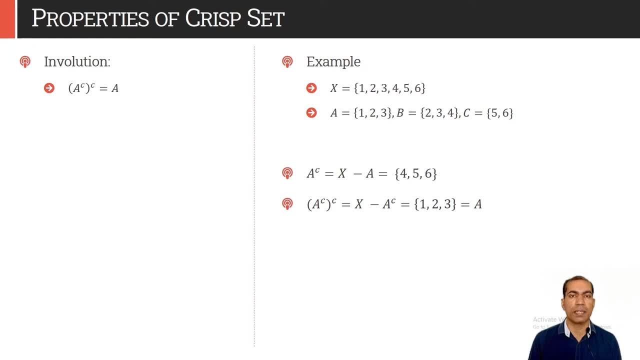 it is proved that complement of the complement of the set is set itself. commutativity: some operations are commutating, some are not. 5 plus 4 is equal to 4 plus 9. so we can say that plus operator is commutative if by: 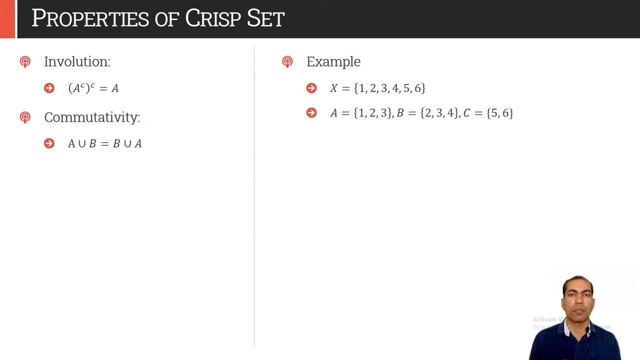 altering the order of operand output does not change. such operators are called commutative. 7 minus 10 is not same as 10 minus 7, so minus is not commutative. in case of set theory, union operator is a commutative. that is A union B is same as B union A. so if we compute A union B it will take. 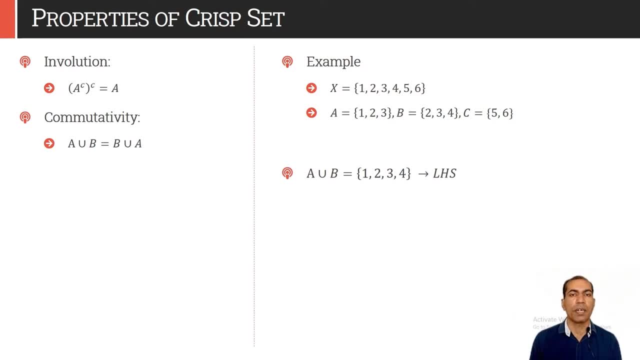 all the elements from both the sets, that is one, two, three, four. and if we take B, union A, definitely it will be same, so we can say that union is a commutative operator. A intersection B is same as the intersection A. intersection B means common elements from both the sets, that is, two and three, and in same way B. 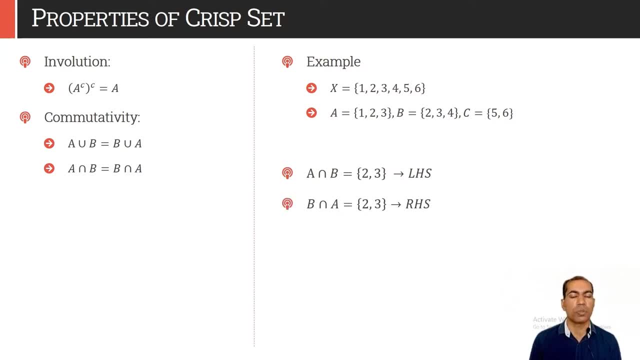 intersection A will also take the same elements, that is two comma three, and it is proved that intersection and union both are commutative, for the sets operator is called associative. if we can alter the order of operation, that is a commutative operation is 1 plus 2 plus 3, suppose this we want to compute. so if we first add 1 and 2 and the result we are 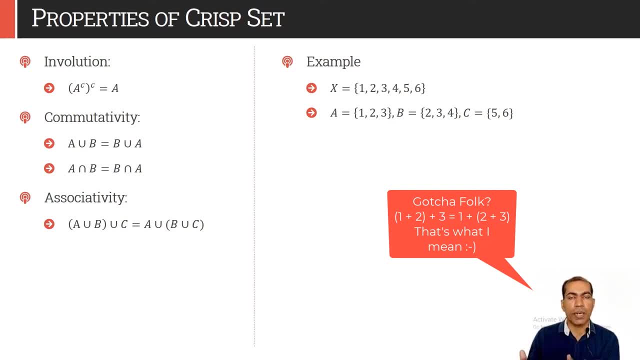 adding into 3. it will be same as first we add 2 and 3 and then we add it to the 1. so it does not matter whether you first add first two operand or you first add last two operand. result is same in this case. so plus is associative in case of set operation, union is also associative. that is first. 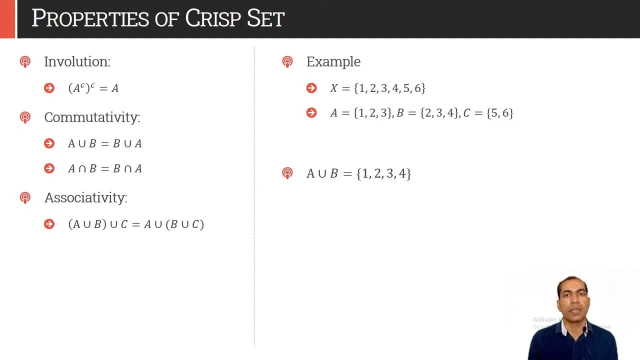 you take union of a and b and then you take the union of that with c, that will be identical if you first take union of b and c and then take union of that with a. in identical way, intersection is also associative. so if you first compute intersection of a and b and then we take 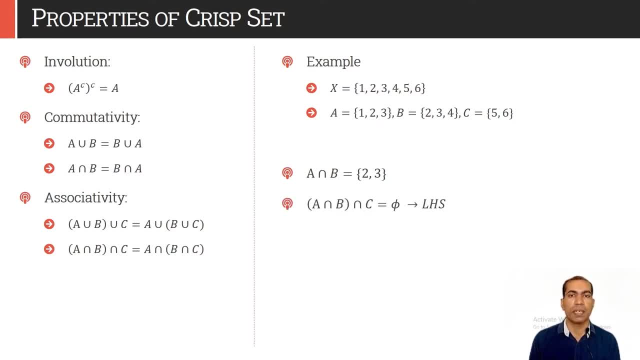 intersection of that with c will be definitely same as first we compute intersection of b and c and then we take intersection of that with a, and then we take intersection of that with c and then we take intersection of that with a with set A. So intersection is also associative operation, Distributive A, union, B intersection. 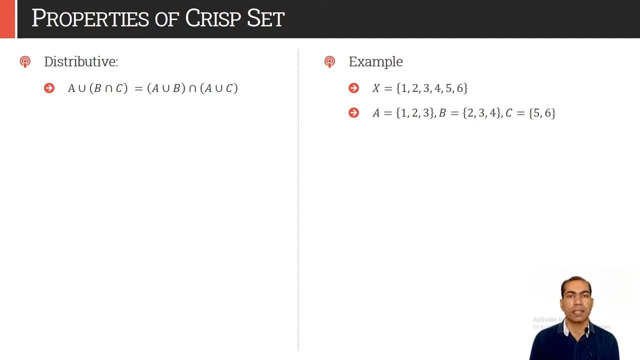 C is same as A union B intersection A union C. So to prove this we will first calculate left hand side of this equation. So let us compute B intersection C, That is 5, because there is no common element in set B and C. If we take union of that with set A, then it 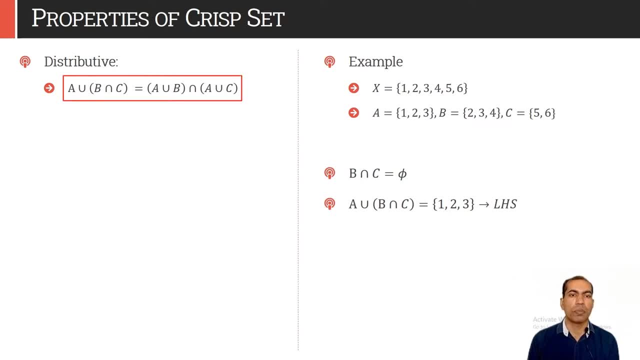 would be 1,, 2, 3.. That is the output of left hand side of this equation. Let us try to compute right hand side of this equation. So first we will calculate A union B, which is 1,, 2,, 3, 4, and we will compute A union C, which is 1,, 2,, 3,, 5, 6 and intersection. 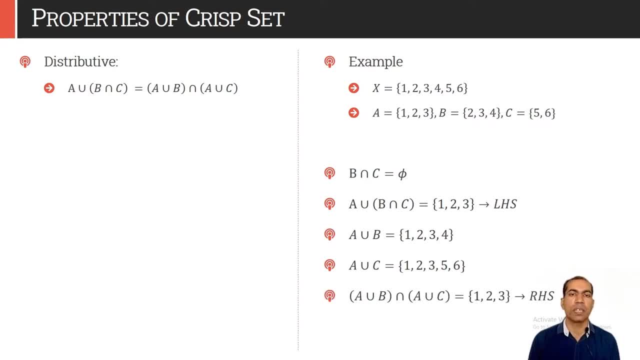 of these two set would be 1,, 2,, 3, which is same as left hand side. A intersection B union C is same as A intersection B union A intersection C. So in similar way we will first compute left hand side of this equation. So B union C would be 2,, 3,, 4, 5,. 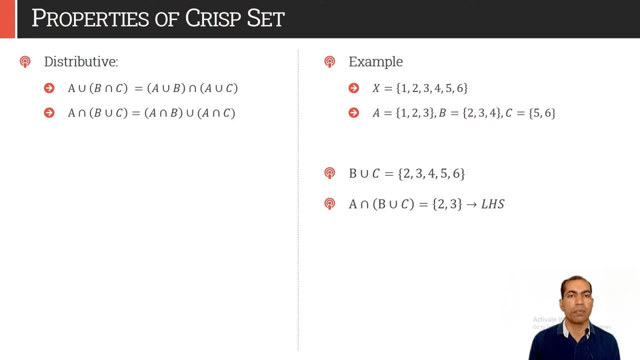 6, and intersection of that with set A would take 2, 3.. On right hand side first we will calculate A intersection B, That is 2, 3.. A intersection C, which is null, and the union of these two would be 2, 3.. 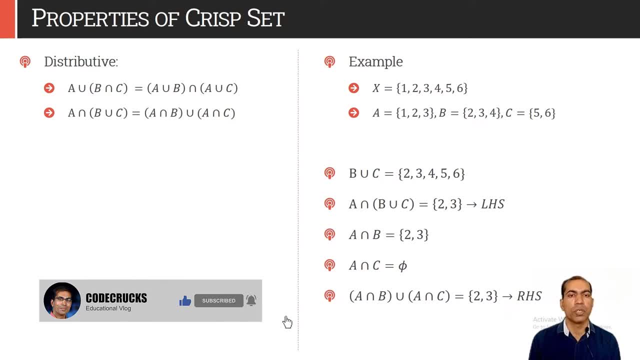 So that is identical to the left hand side of equation. So it is proved that this set operations are distributive. Absorption A, union, A intersection B is equal to A, As we know that A intersection B will take common elements which are in both the sets. 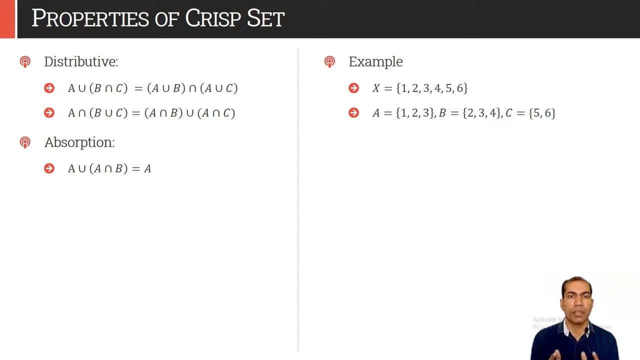 A as well as B. So definitely A intersection B will be subset of set A. So whenever we take union of set and its subset, definitely output will be the larger set. That is, the set A itself. Let us try to understand it with the data. 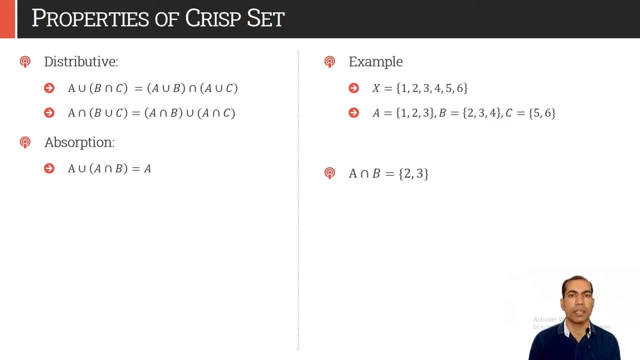 A intersection B in given case would be 2,3.. As you can see that 2,3 is subset of A as it is present in set A. So if we take the union of A and the A intersection B, definitely it will generate the set itself. 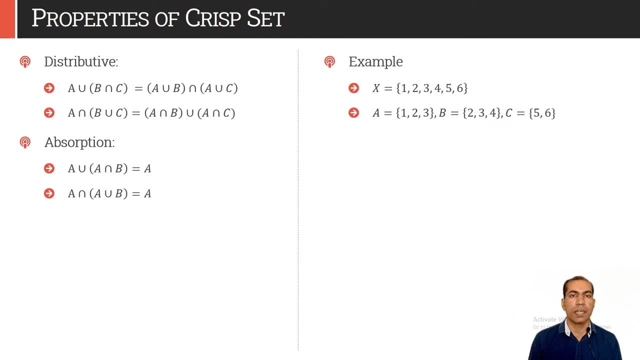 This is called absorption column. In identical way, if we take A intersection, A union B, that will also be A, Because A union B will contain all the elements of A as well as from B. So A union B will be always superset of set A as well as superset of set B. 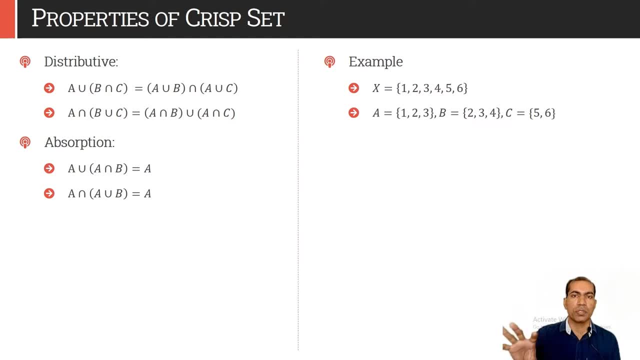 Whenever we take intersection of set with its superset, obviously it will generate set itself as an output, because that is the smaller set. So for given data, A union B would be 1,2,3,4.. And if we take the intersection of that with A, definitely it will generate the set itself. 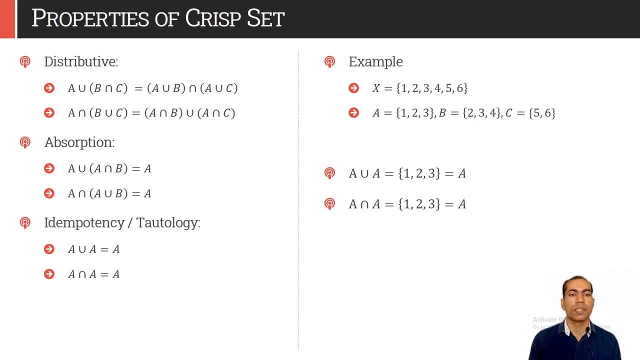 Hence absorption property of the set is proved Item potency or the tautology. If we take union of set with itself, will definitely be set itself, And if we take intersection of set with itself, then the output will be the set itself. 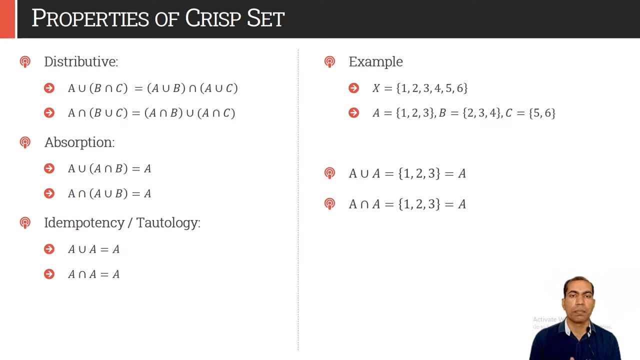 Just like 5 plus 0 is 5, 10 into 1 is equal to 1.. So 0 and 1 are tautology for addition and multiplication operation. Similarly this A union A is A and A intersection A is A in case of set theory. 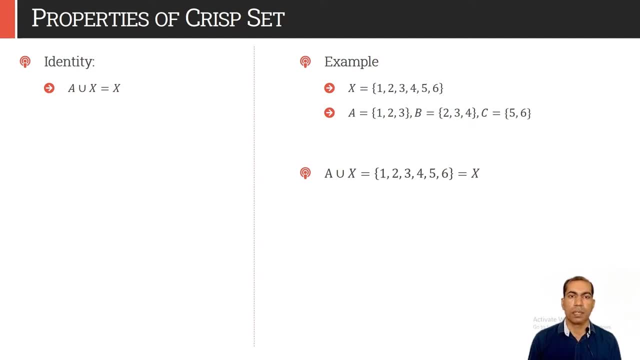 Identity property. A union X is X. Just, we discussed that X is a universal set which is always a superset of A. So when we take Intersection of set with its superset, output will be definitely superset. So A union X is X always. 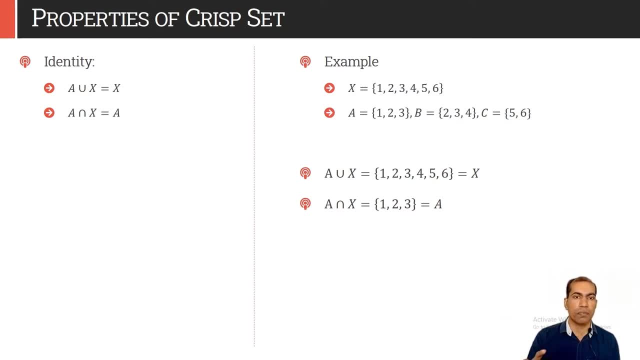 A intersection. X is A. A is subset of X. Whenever we take intersection of set with its subset, then output will be definitely subset because it is the smaller one. A union 5 is A. 5 indicates null set. So there is no element in that null set. 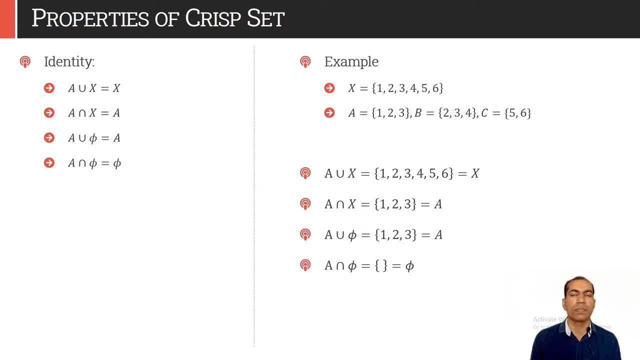 So A union null set will be set A itself. Ok, So A intersection null or A intersection 5 will be 5.. De Morgan's law It says that A union B, whole complement, is A complement, intersection B, complement A union B is 1,, 2,, 3, 4 and complement of that would be 5, 6.. 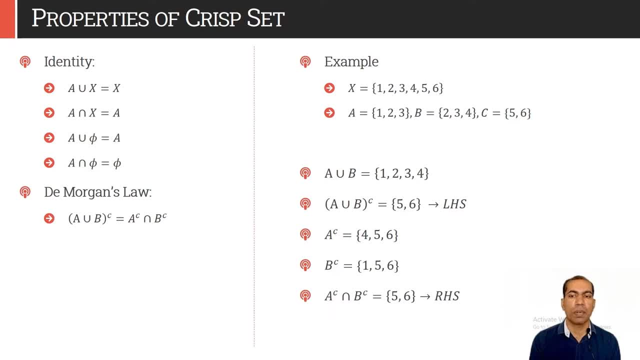 Now to compute the right hand side, we need to calculate A complement, which is 4, 5, 6.. B complement, which is 1, 5, 6.. And intersection of these two complement is 1, 5, 6.. 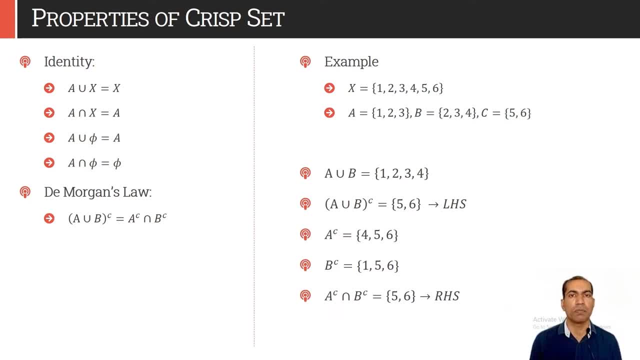 So A union B is 1,, 2,, 3,, 4.. And intersection of these two complement and set is 5, 6, which is same as left hand side. The second law of De Morgan's is A intersection, B whole complement is same as A complement. 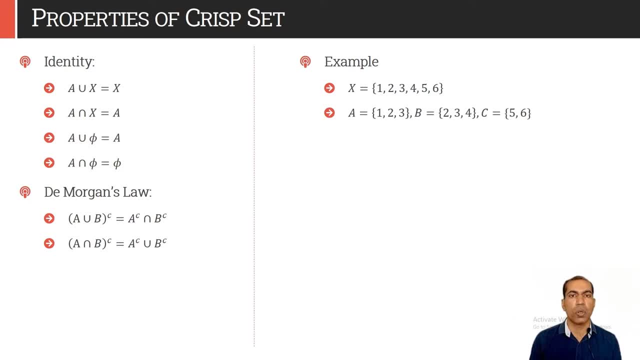 union B complement. So first we need to calculate intersection B, which is 2, 3.. Then will calculate complement of that, which is 1,, 4,, 5, 6.. To compute the right hand side, first we will compute A complement, which is 4,, 5, 6.. 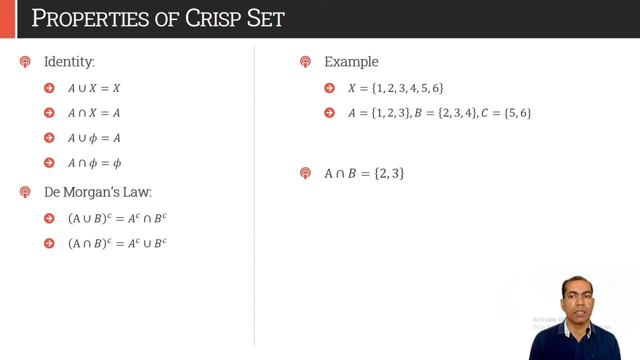 Then we will calculate Kwt W 2,, 2,, 3,, 4, and complement of that which is 1,, 2,, 4,, 5.. To compute the right hand side first were compute A complement which is 4,, 5,, 6.. 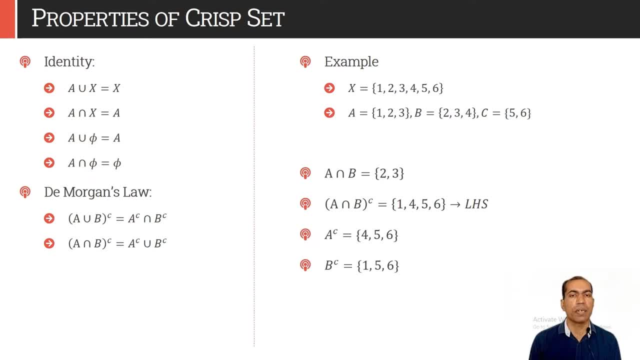 Default Ruleio of De Morgan's Thesis is 8. Regular battles are suggested by that. If A có lavoro de Armas, that means that there the other arm goes further from the other edge. B complement, which is 1, 5, 6, and union of that is 1, 4, 5, 6, and as we can verify it, 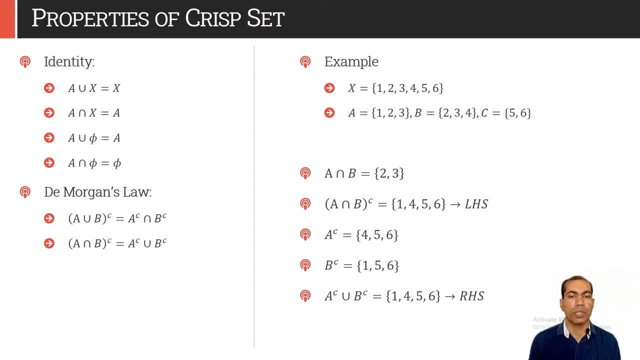 is same as left hand side. so the De Morgan's law is satisfied Law of contradiction. if we take intersection of A with its complement, that will be definitely null set, because A complement is set of all the elements which are not in A. so there will not be any common element between set A and its. 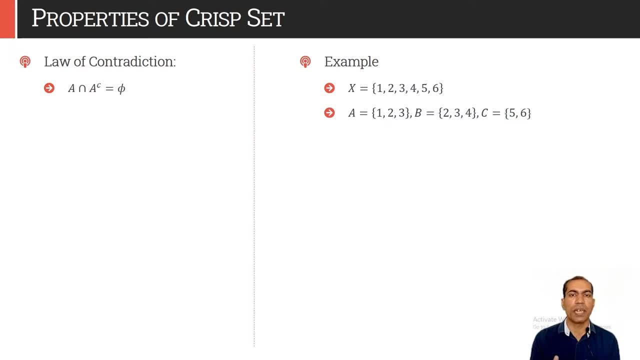 complement and hence the intersection would be definitely null set. that is A intersection. A complement is 5, so here A complement is 4, 5, 6 and if we take the intersection of that with A, as we can see, is null set. Law of excluded middle. 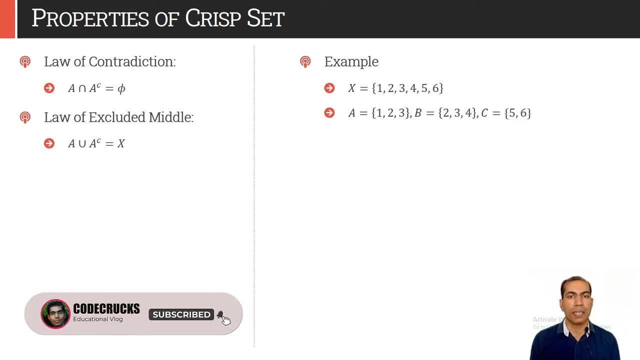 so A union A complement is X. A complement is computation of A in the middle. a union A complement is X. A complement is computation of a complement is not in A. So there will not be any common element by subtracting all the elements of a from x. so when we take the union of that two would definitely 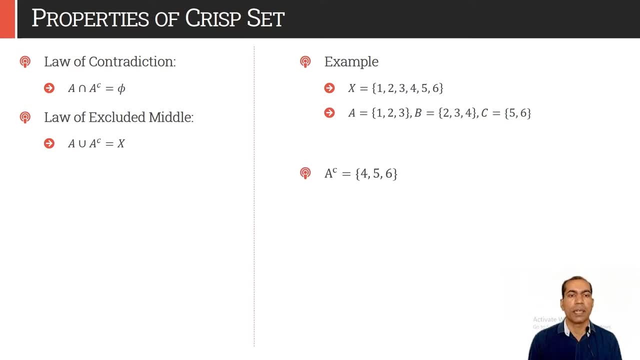 sum up to a set of universe. in our case a complement is 4, 5, 6. when we take the union of that with a itself, it will produce the entire universal set: 1, 2, 3, 4, 5, 6. hello folks, welcome to. 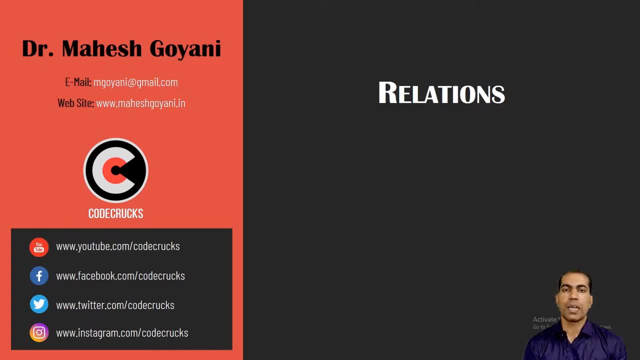 cold crux. this is mahesh gujrani, and in this video i will be talking about relations. relations are basically derived from cartesian product of two sets. we have already discussed how to compute cartesian product of two sets in previous video. link of that video is given in description box. 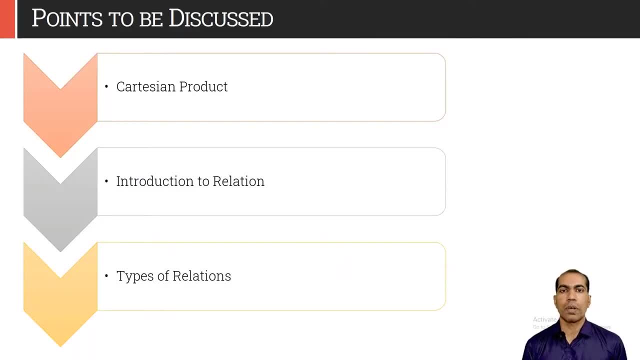 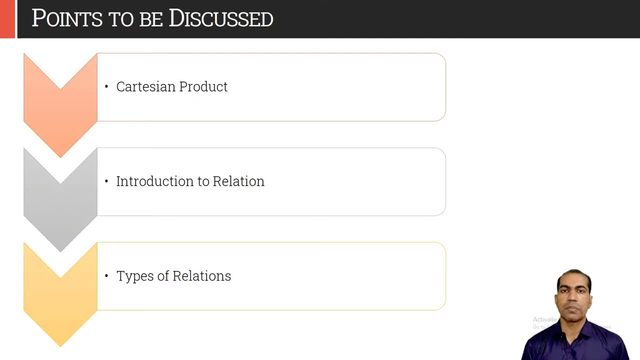 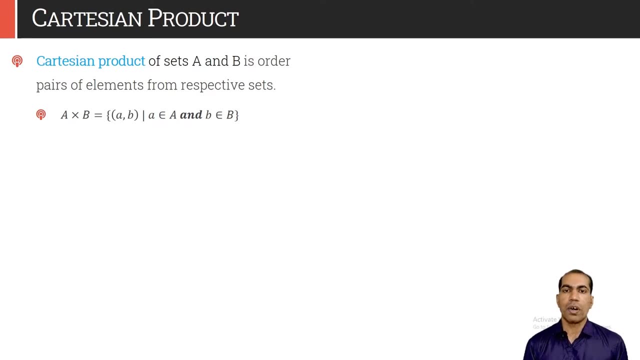 what is relation, and we will also discuss various types of relations in this video. cartesian product of two sets, a and b, is collection of ordered pairs of the elements from respective set. mathematically it is defined as a cross b, where cross is nothing but it's a cartesian product operator. so a cross b. 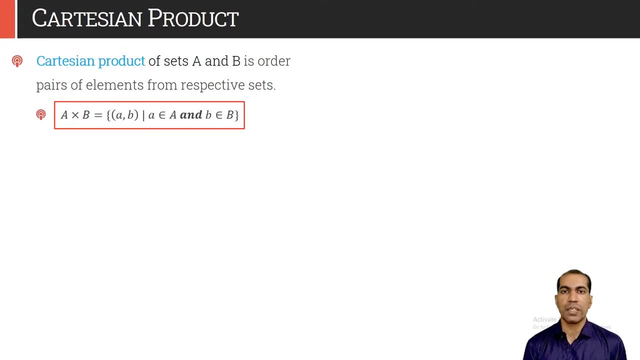 is given as collection of tuple a, comma b, such that the first element, small a, comes from set capital a and second element, small b, comes from the set capital b. so order of this element is very important. we cannot alter order of a and b within this tuple. consider that we have two sets. 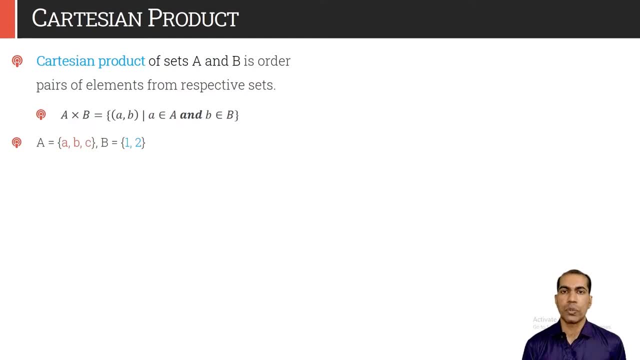 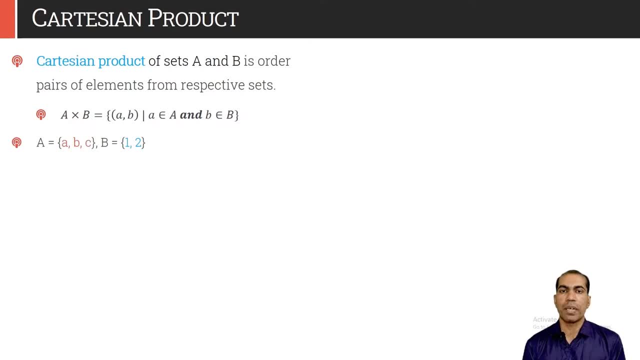 between a and one a and two b and one b and two c and one c and two and so on, and that collection of ordered pair will form the cartesian product. so we can define the cartesian product of set a and b as a: 1, b, 1 c, 1 a, 2, b, 2, c, 2. as you can see, the first element in this tuple is coming from set a. 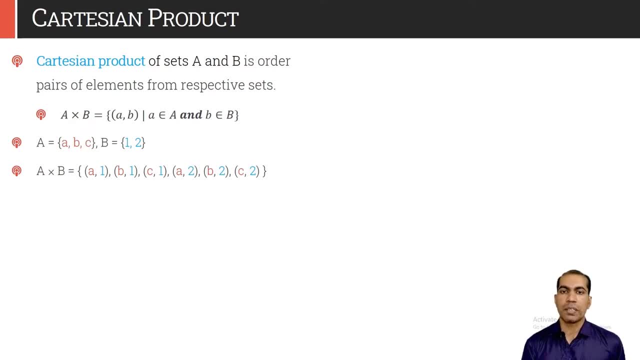 colored in red, and second element in all the tuples is coming from set b, colored in blue. Again, Cartesian product itself is a set and we know that order of elements within set is not important. It is unordered collection of elements. So we can swap or we can readjust the position of tuples. That's perfectly fine. So I can also define. 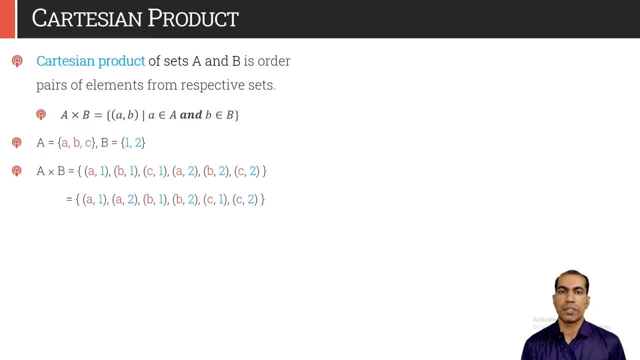 Cartesian product as a1, a2, b1, b2,, c1, c2, or even I can randomly place the tuple. However, elements inside tuple we cannot alter. That means order of a and b must not be changed. So 1a, 2a, 1b, 2b and so on is not a cross b, because here the first element belongs to. 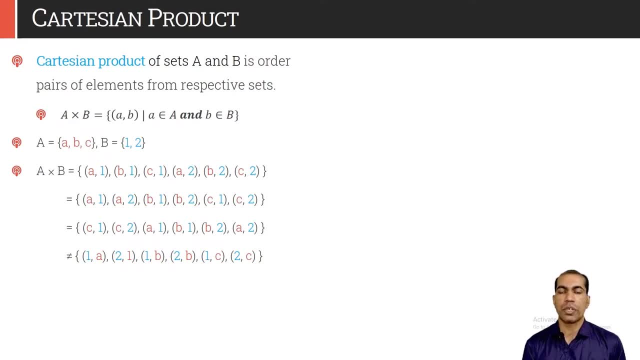 set b and second element belongs to set a. So in fact it is b cross a and in general a cross b is not same as b cross a. Let us compute 2 power, a cross b. That means we have to compute the power of a cross b. 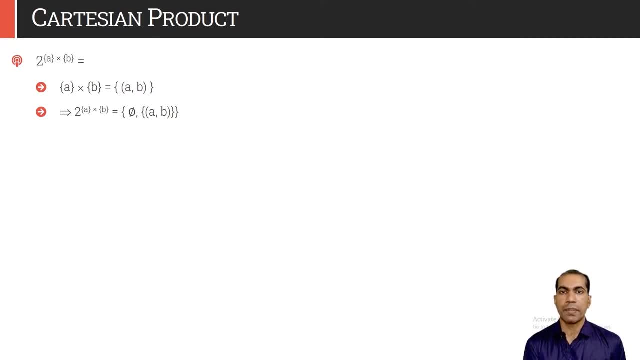 For set of Cartesian product of set a and b. both the sets contain only one element, So their Cartesian product will also contain only one tuple. By associating a with b we will get only one tuple, that is a- b. Now, power set of this set would contain two elements. 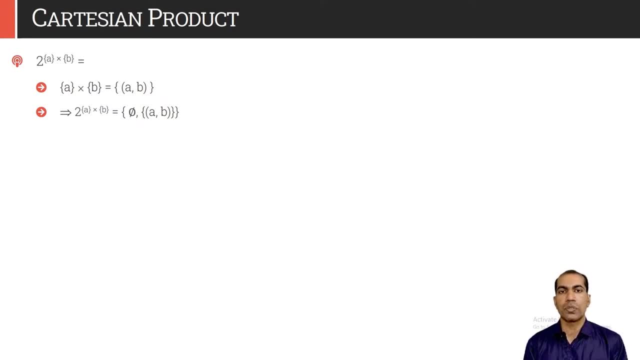 because the set contains only one element, Power set will have 2 raise to 1, that is, two elements. By definition, null will be the part of any power set and set itself will also be the member of any power set. So this power set of Cartesian product of a and b would be 5 and tuple. 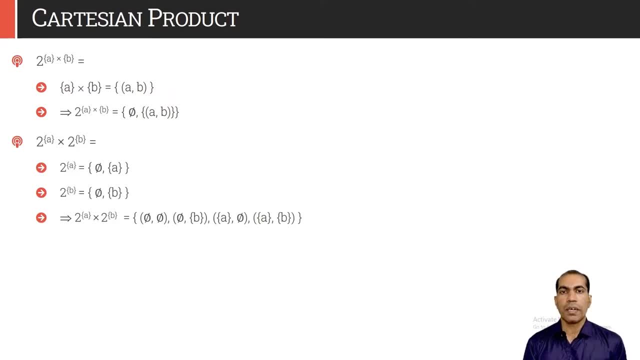 2 power a cross 2 power b. So now we are computing the Cartesian product of two power sets. In previous example we have computed first Cartesian product and we have computed the power set of that. Now we are individually computing power sets of set a and b and then 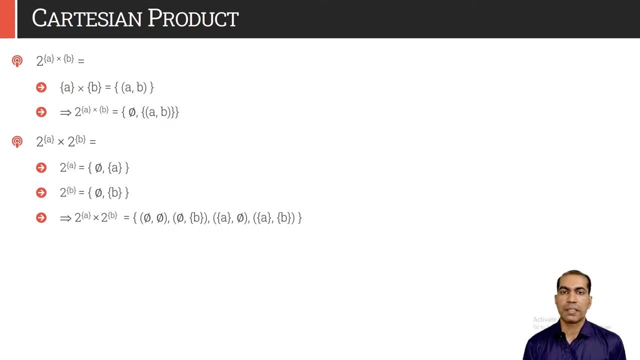 we will take the cross product of that. As each set contains only one element, their power set would contain two elements: 5 and the element itself, That is, 2. power a will be 5 and a and 2 power b would be 5 and b. 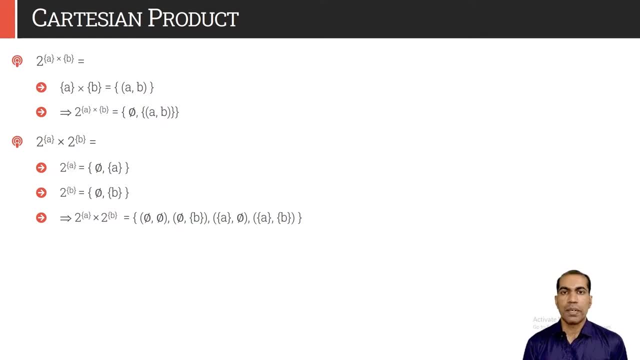 Now this: both sets contain two elements, So their Cartesian product would contain 2 into 2, that is 4 elements. We shall associate each element of 2 power a with all the elements of 2 power b, So that would be 5 comma 5.. 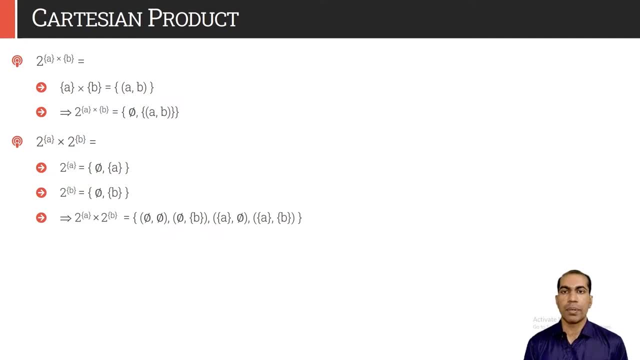 5 comma 5.. 5 comma 5.. 2 comma. 2 comma b. 3 comma a comma 5.. 3 comma a comma b. The concept of Cartesian product is not just limited to two sets. we can extend it to n. 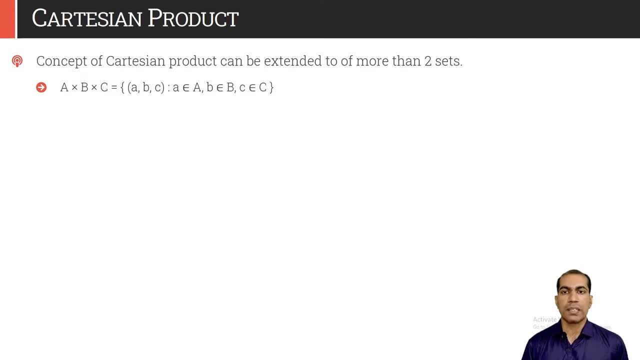 number of sets. Suppose we have three sets, A, B and C, then we can compute Cartesian product between these three sets as A cross B, cross C, And it would be collection of all the triplets small a, B and C, such that small a is coming from set a small b – belongs. 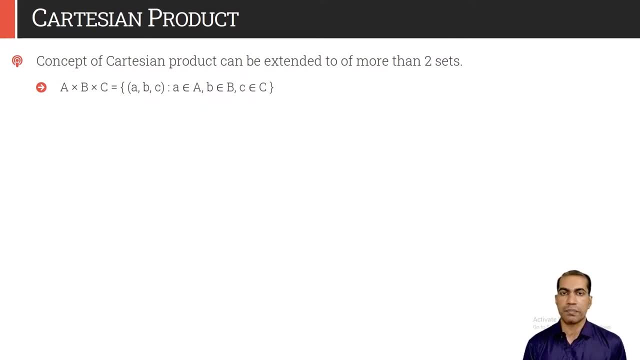 belongs to set B and small c belongs to set C, And in general we can extend it to n number of sets. Technically we can say that A cross, B cross C is same as first we compute the Cartesian product of A and B and then we will take the Cartesian product of that output. 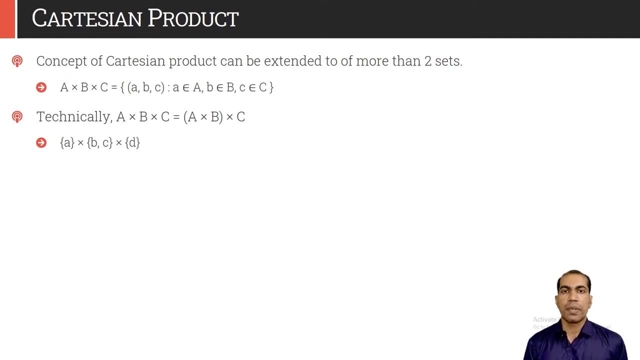 with the C. Let us consider the example. we have three sets containing element A, B comma C and D. So first we will compute the Cartesian product between first two sets, so that will be A comma B and A comma C. We will take the Cartesian product of that output with third. 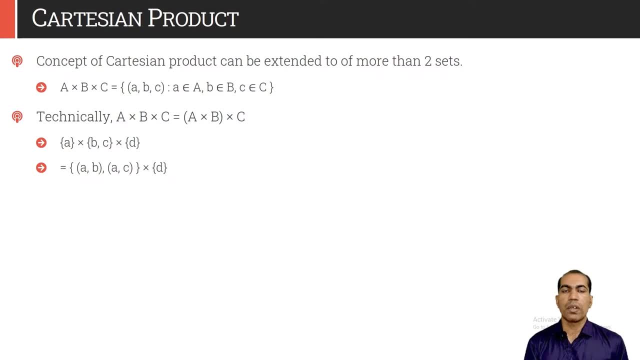 set, that is, with the D, so that would be A comma B comma D and A comma C comma D. For the simplicity, we are often orbiting this inner parenthesis so that the Cartesian product of this would be A comma B comma D and A comma C comma D. 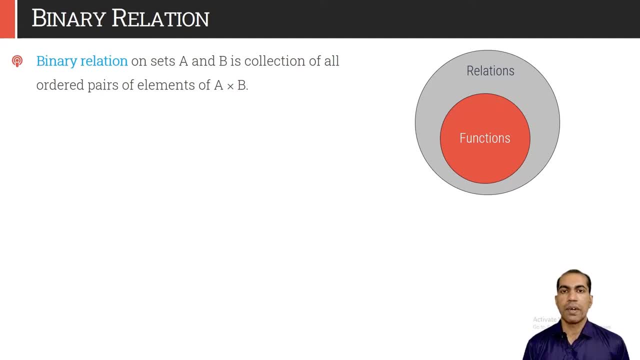 relations are always defined over the Cartesian product of given sets. So binary relations on two sets, A and B, is collection of all ordered pairs of elements of A cross B. So Cartesian product will act as a superset and relation will be the subset of that. Now, by defining the relation, 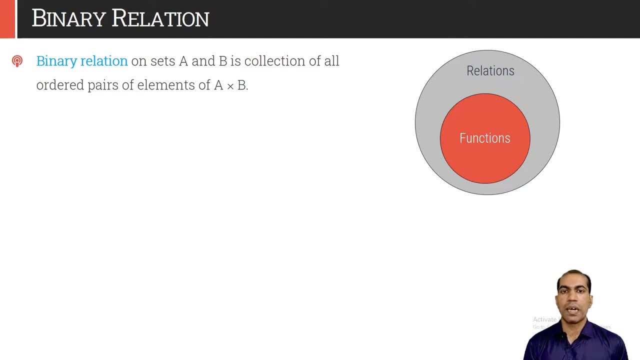 we are selecting some of the elements from the Cartesian product. Generally, relation is represented by letter R, and if tuple A comma B is satisfying the condition for relation R and if it is in R, then we can write it as a A, R B. So that is the notation for element A is: 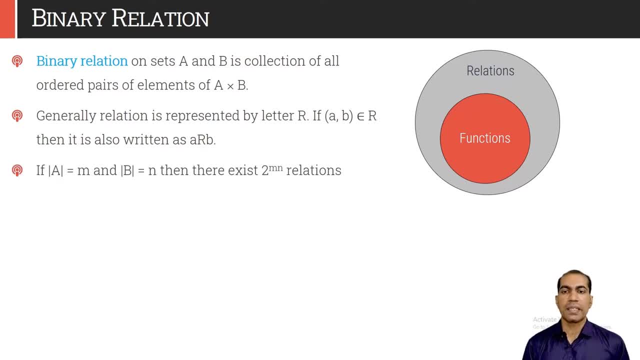 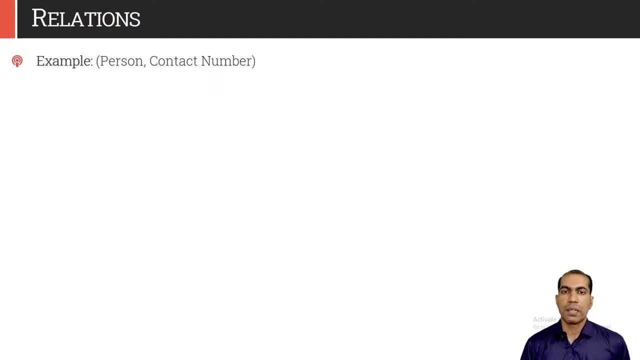 related to B by relation R. If set A has M elements and set B has N elements, then there are 2 raise to M and different relations are possible. Let us take one example: Each person is having some contact number. For simplicity, we are assuming that each person is having one contact number. 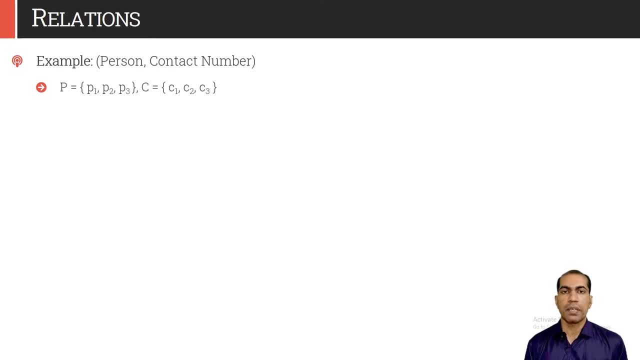 and we are considering this. set person P is having elements P1, P2, P3, 3 persons and the set of contact number, capital C, has 3 contact numbers: C1, C2, C3. If we calculate the cross product of P and C then it would have 9 different elements because each PI will be associated with. 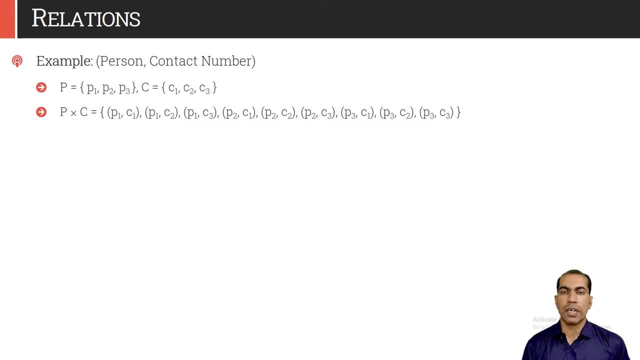 each of the CI, Each person is having only one contact number. and we are assuming that P1 has contact number C1, P2 has contact number C2 and P3 has contact number C3. So the relation person related with contact number would have only 3 tuples out of these 9 tuples. That is P1. 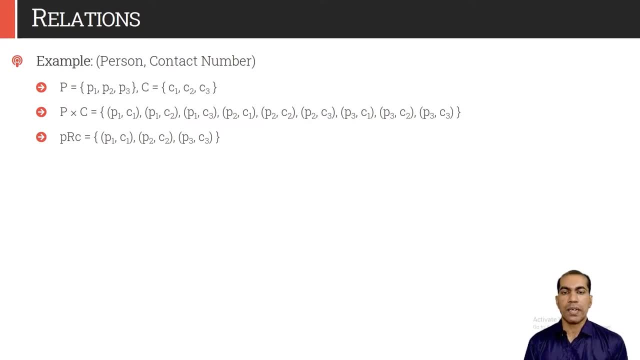 comma C1, P2 comma C2 and P3 comma C3.. If I consider P1 comma C2, then person P1 is not having a contact number C2, rather it has contact number C1. So we will not include tuple P1 comma. 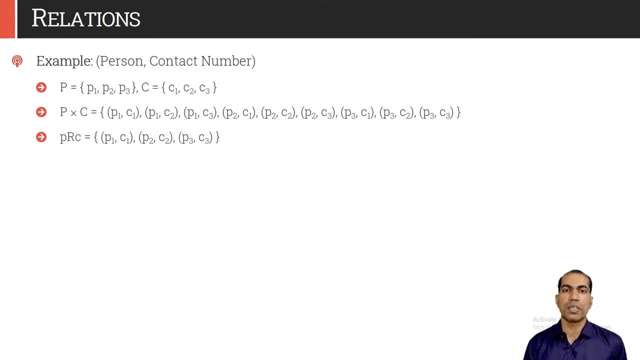 C2 or P1 comma C3 in relation R because it is not satisfying the condition of the relation. the another example: like we can define less than relation over set of natural number. set of natural number contains elements from 1, 2, 3, 4, 5 up to infinity, if i take the cartesian. 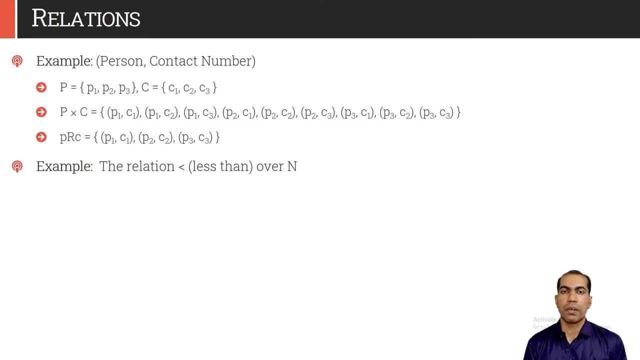 product of n with n, then it will have tuple 1: 1, 1, 2, 1, 3, 1, 4, and so on: 2 1, 2, 2, 2, 3, 2, 4, and so on: 3 1, 3, 2, 3, 3 and so on. now the relation we have defined is less than it means. a should be less. 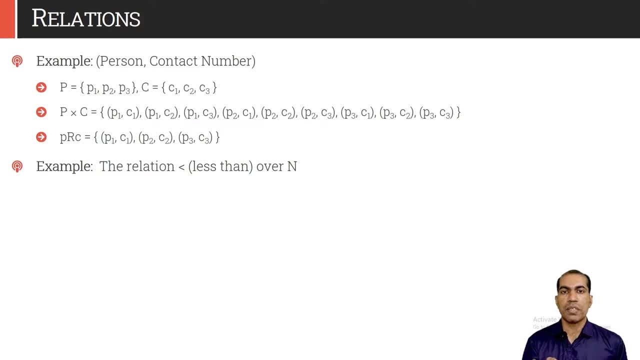 than b. that is what the relation is. so if i pick up the first tuple from cartesian product of n with itself, then that is 1 comma 1. 1 is not less than 1, so that will not be the part of relation. if i consider 1 comma 2, so 1 is less than 2. it is satisfying the condition for being less than. 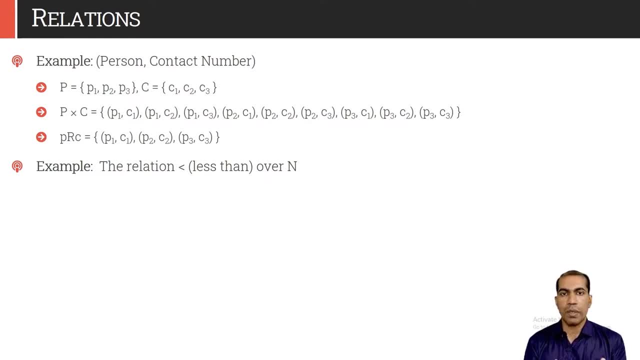 so that will be the part of relation r. 1 comma 3. so in that case 1 is less than 3, so that will be also part of relation. so Except 1 comma 1, all the pairs starting with 1 will be in relation R, because they all will. 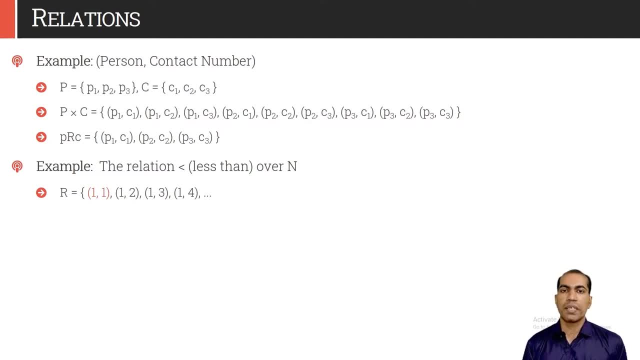 satisfy the condition a less than b. Similarly, if we consider all the tuples starting with 2, then 2 comma 1 will not be in relation, as 2 is not less than 1.. 2 comma 2 will also not be the part of relation R, but 2 comma 3, 2 comma 4 onwards, all the tuples are satisfying. 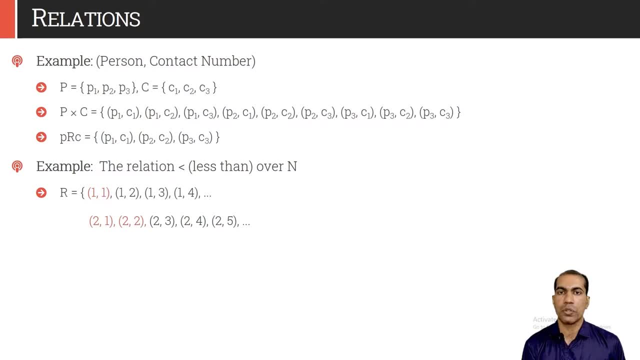 the condition 2 less than 3,, 2 less than 4,, 2 less than 5, and so on. So they all will be the part of relation and same we can observe for rest of all the tuples 3, 1, 3, 2, 3,. 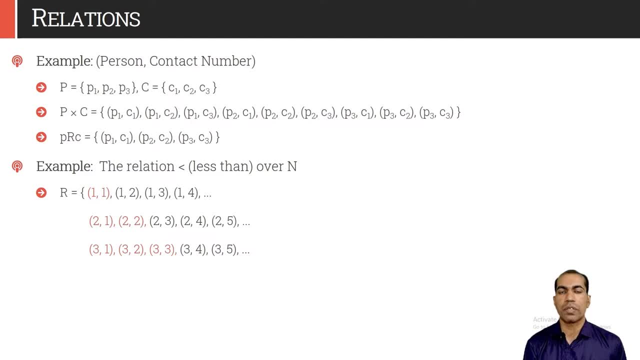 3 will not be in relation R, but then onwards 3,, 4,, 3,, 5,, 3,, 6 and all will be in relation. Often relations are described over the same set. That means R is subset of set A cross. 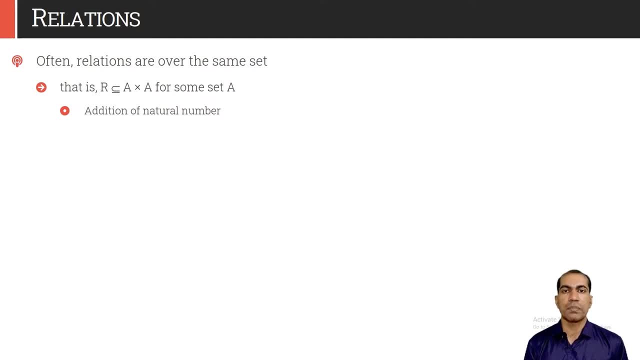 A, R is derived from the Cartesian product of same set, A cross A. The example is like addition of natural numbers, So set of natural number is having 1,, 2,, 3,, 4,, 5 and so on. infinity base. 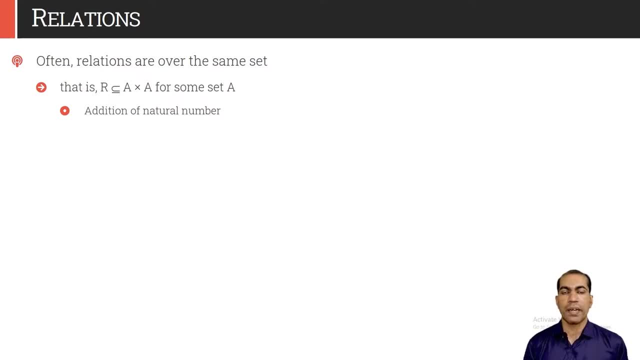 If I pick up any two numbers from that set N, and if I add it, I will again generating the natural number. So this relation is always having same set for the base. That means the relation addition over natural number is derived from the N cross N set. However many times 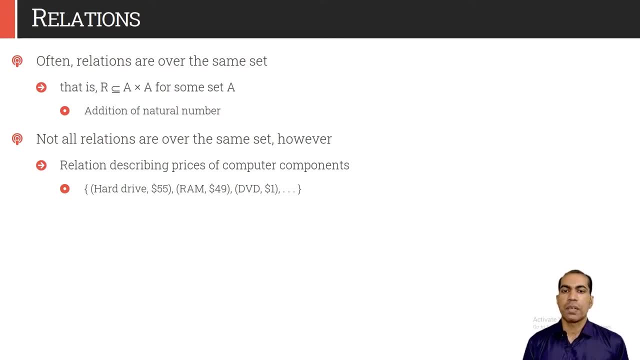 relations are described over different sets. For example, if we want to create a relation between computer components and its parts, then we have to create a relation between its parts and its price. Then it would take two different sets. One set contains computer components, another set contains the price. So hard drive is of $55,, RAM is of $49, TBD. 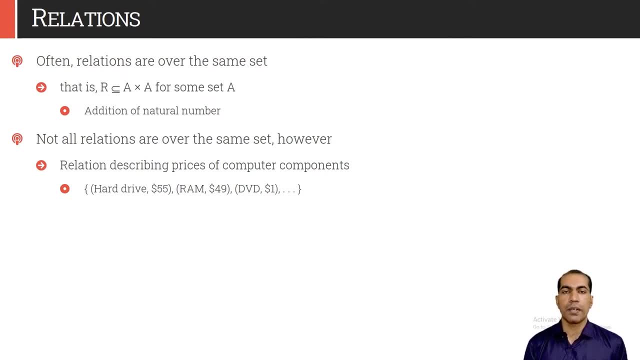 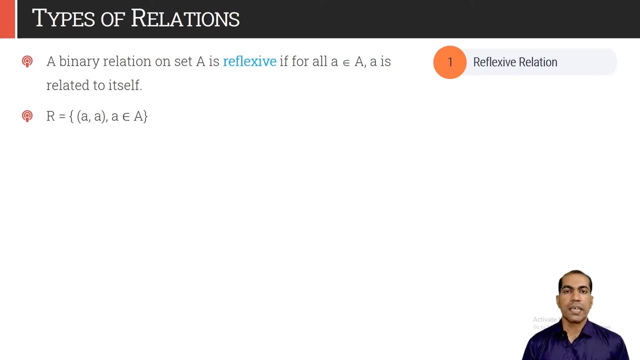 is of $1 and so on. So this is described over different sets. Let us talk about types of relations. This is quite important. A binary relation on set A is said to be reflexive if all the elements of capital A are in relation to the set A. So if we have a binary relation, 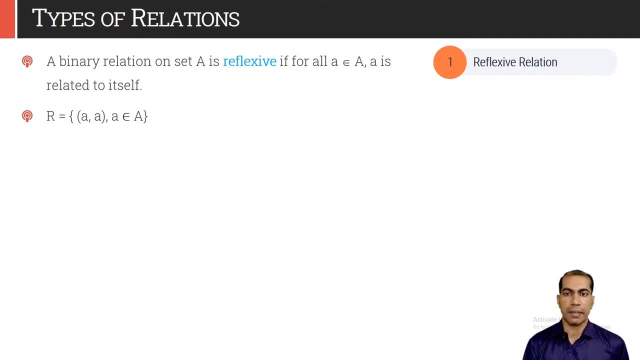 A that is related to itself. that is ARA. In other words, we can say that the couple is in R. If it is having identical elements- a comma a- then it is in relation R. Assume that set A is one comma two and the relation R over that is having some tuples: one comma. 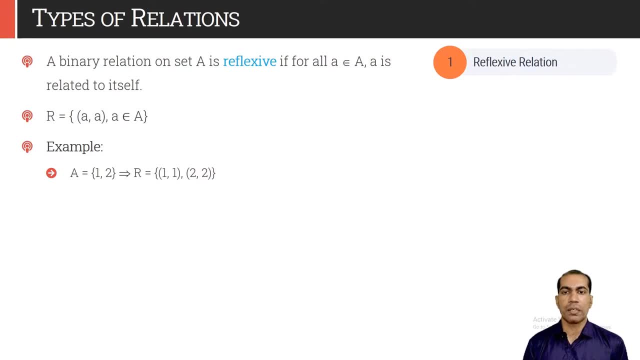 one, two comma two. So R is reflexive relation, because set A is having two elements, one and two, And for both ARA is in relation. If we have a vertex, U is in relation to the u, then definitely u is reachable from u itself, because we are already on u and u is reachable. 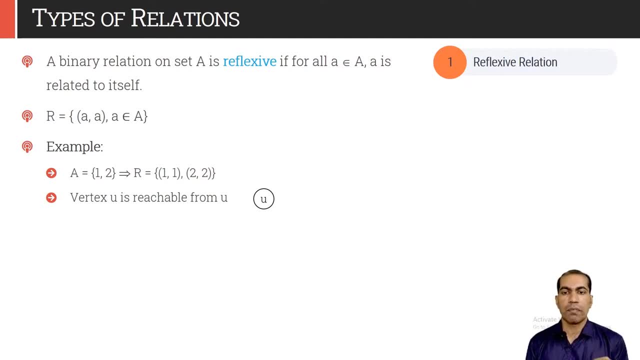 from that. So in that sense also we can say that the vertex u is reachable from u is a reflexive relation like less than or equal to is equal to, greater than or equal to all are reflexive relations. but less than and greater than are not reflexive, because 3 less than 3 is not true. 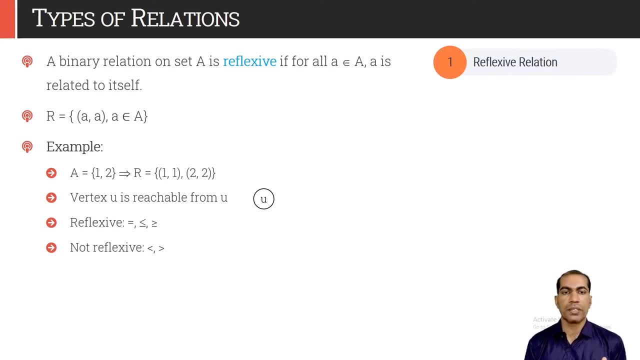 So a is not associated with a or a is not related to a. but in case of less than or equal to, greater than or equal to, I can say that phi is less than or equal to phi or tan is greater than or equal to tan. So in that case a is associated with a by less than or equal to or greater than or equal. 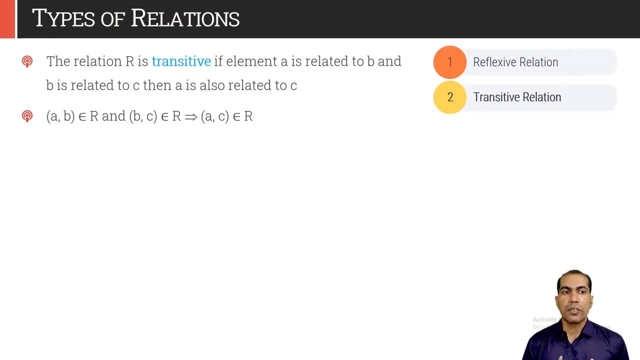 to relation, So it is reflexive. The relation R is said to be transitive if any element a is related to b and if element b is related to c, that means a must be reflected. If this is true for all the tuples in relation, then we can say that that relation is transitive. 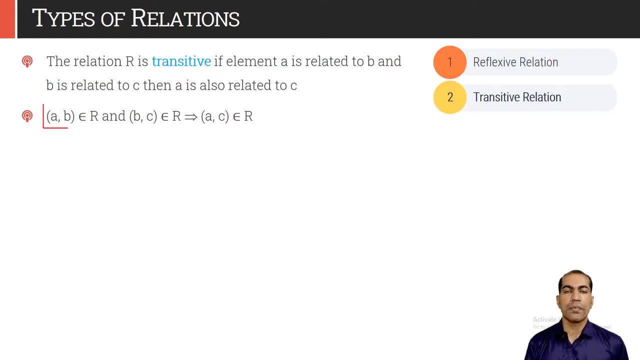 relation. Mathematically we can say that if a comma b belongs to R and b comma c belongs to R, then a comma c must be in R. Consider the set: a is equal to 1, 2, 3, b is equal to 1, 2, 3. 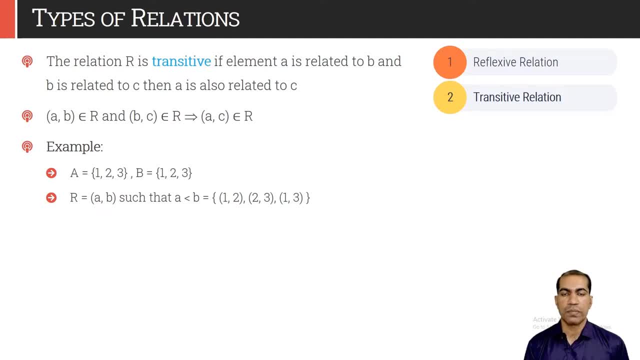 and we are describing the relation less than over these two sets. So a should be less than b. So we will pick up first element from set a b, from the set capital B, and we will check if it is less than or not. If a less than b condition. 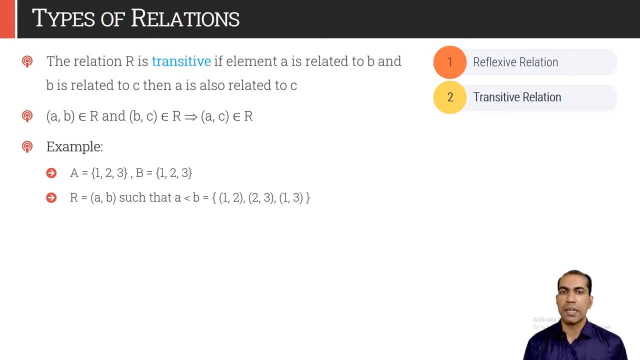 is satisfied, we will put it into relation R, else we will reject it. We will select one element from a and we will try to relate it with all the elements with in b. So 1 and 1 are not satisfying the condition, a less than b, So that 1 comma 1 tuple will not be in relation R. 1 comma 2 is. 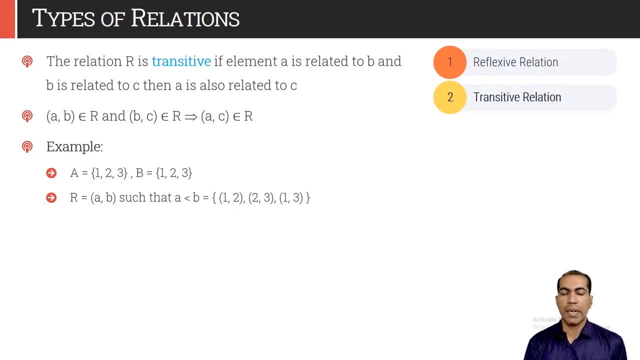 satisfying the condition because 1 is less than 2.. So that will be added into relation 1 comma 3. it is satisfying the condition of a less than b, So it is added into the relation R. Similarly, 2 comma 1 is not true. 2 comma 2 is also not true. 2 comma 3 is true, So that is added. Then 3 comma. 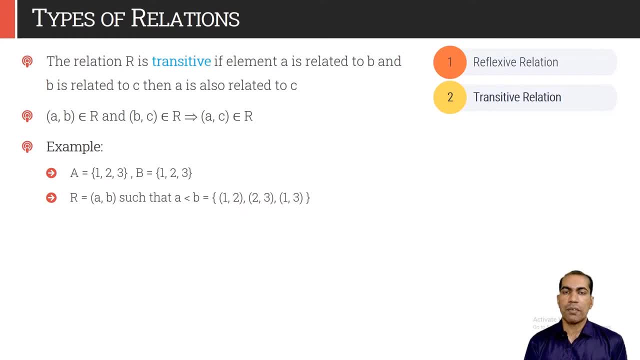 1, 3 comma 2, 3 comma 3.. Conditions are false for all three tuples, So none of the tuples starting with 3 will be added into the relation. So relation R ultimately would be 1 comma 2,. 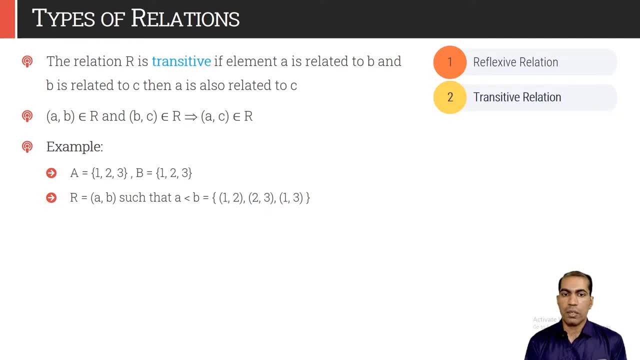 2 comma 3 and 1 comma 3.. 1 comma 2 is in R, 2 comma 3 is in R and 1 comma 3 is also in R. So this is a transitive relation. So AB is in R, BC is in R as well as AC is also in R. So 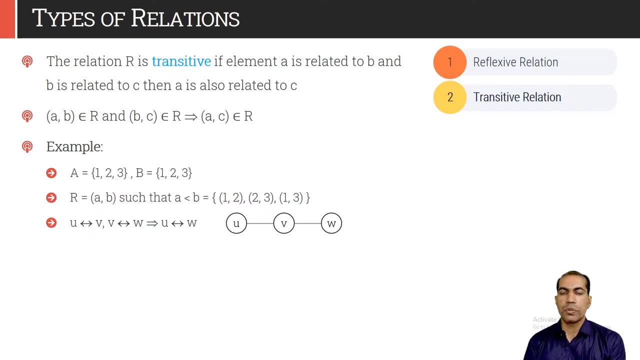 it is transitive. So if you are on vertex U and you can move to V and from V if you can move to W, then definitely you can reach from U to W. So this reachability is also transitive. Similarly, less than or equal to is equal to greater than or equal to less than greater than. 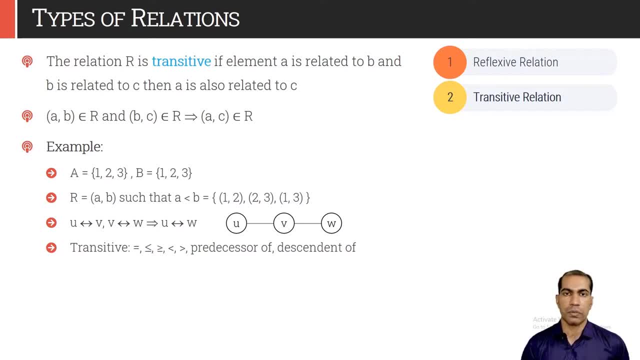 predecessor of descendant. of all these relations are transitive. 4 is less than 5,. 5 is less than 6.. So 4 is less than 6.. Fine, So these all are transitive relations, However not equal to. 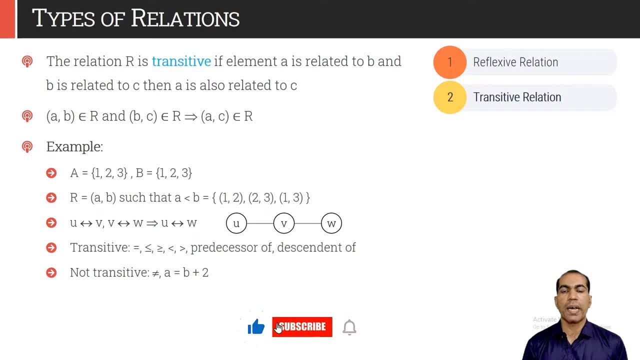 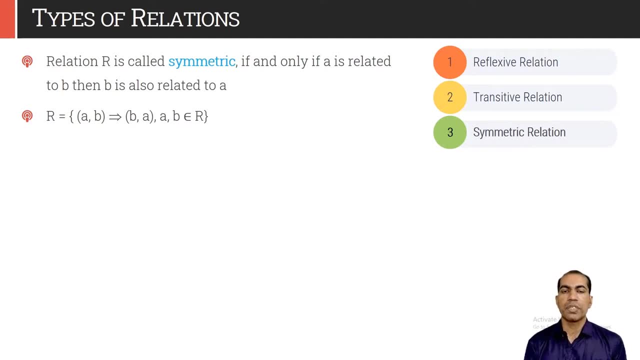 some functions A is equal to B plus 2, they are not transitive. Relation R is said to be symmetric. If A is related to B, then B must be related. It means if A comma B tuple is in relation R, then B comma A must be in R. Then we can say that R is. 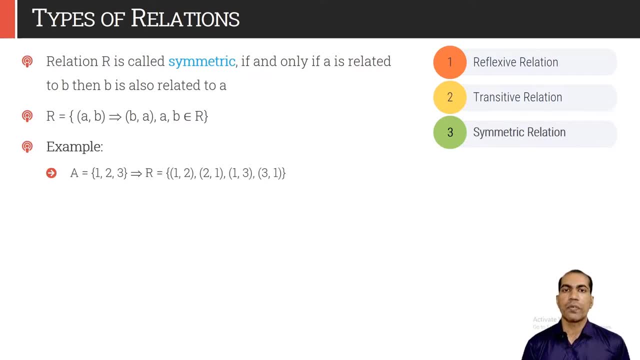 symmetric relation, For A is equal to 1,, 2, 3, if R is 1, 2, 2, 1, 1, 3,, 3, 1, then it is symmetric. If you pick up any tuple, say for example 2 comma 1.. So A is 2, B is 1.. So B comma A should be in. 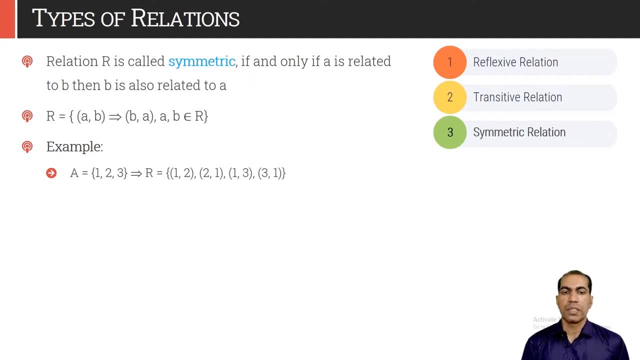 R, That is, 1 comma 2 should be in R and it is already there. Similarly, if I consider 1 comma 3.. So 3 comma 1 is also in R. Similarly if I consider 1 comma 3.. So 3 comma 1 is also in R. 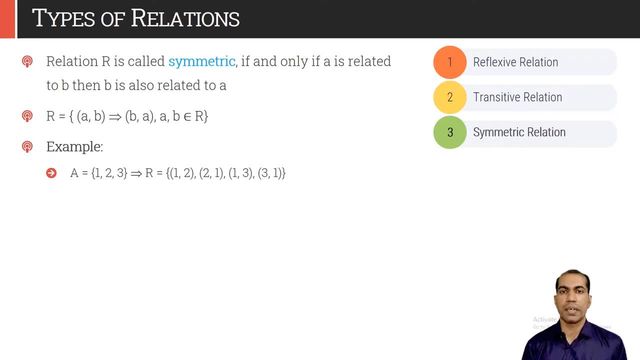 So this particular relation, R is symmetric relation. U is reachable from B, B is reachable from U, So reachable from is symmetric relation. Similarly is equal to being sibling. they all are symmetric relations. So I can say that Ram is sibling of Lakshmana, So Lakshmana is sibling. 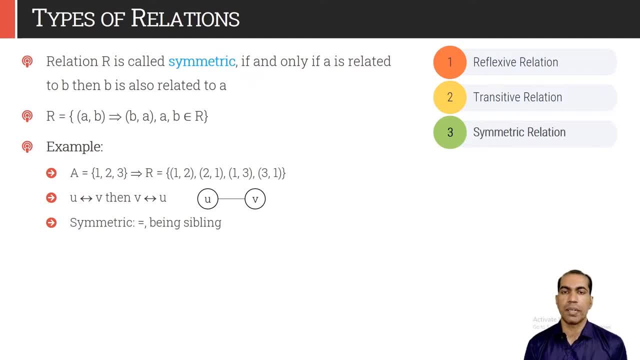 of Ram. that is true, So being sibling is also symmetric relation. However, less than less than or equal to greater than greater than or equal to these all are not symmetric. Relation R is said to be asymmetric. If A is related to B, then B must not be related. 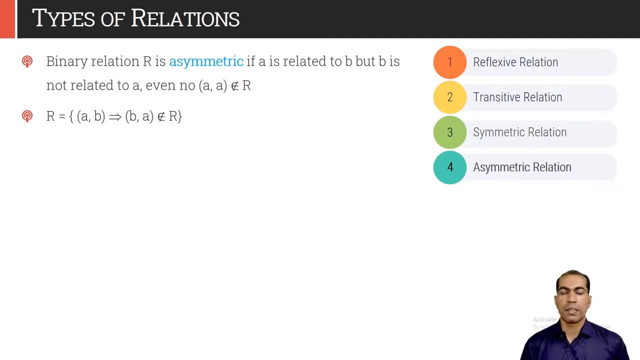 to A. Even A comma A should not be in R. That is, R is equal to tuple A. B implies B. A should not be in R. So if you take the example, R is equal to 1 comma 2, 2 comma 3, then this: 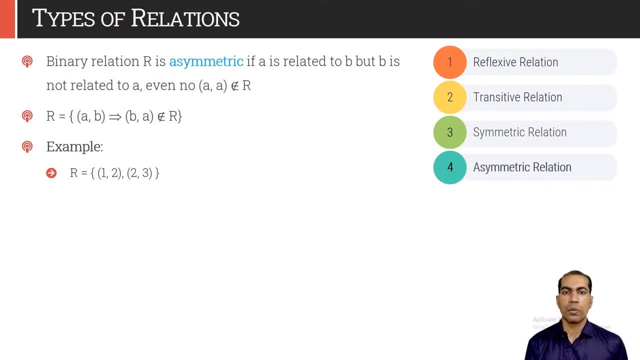 is asymmetric relation Because for tuple 1 comma 2, 2 comma 1 is not in R And for tuple 2 comma 3, 3 comma 2 is also not in R. So this is asymmetric relation. However, if you add one more tuple 1 comma 1, then it is no more asymmetric Because 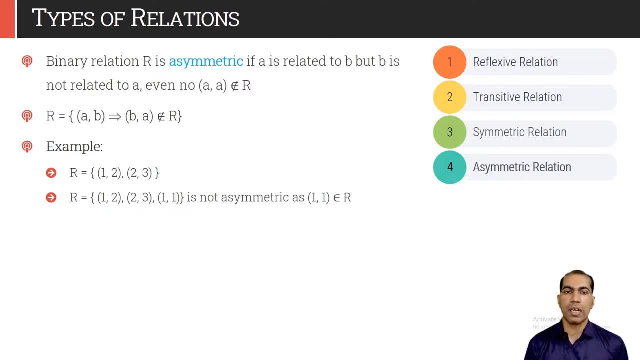 in asymmetric relation. A comma A is not allowed Less than greater than father of student. of all these are asymmetric relation. Dasharatha is father of Rama. That is the one relation. So Rama is father of Dasharatha is not true. It means A comma B is in R, but B comma A. 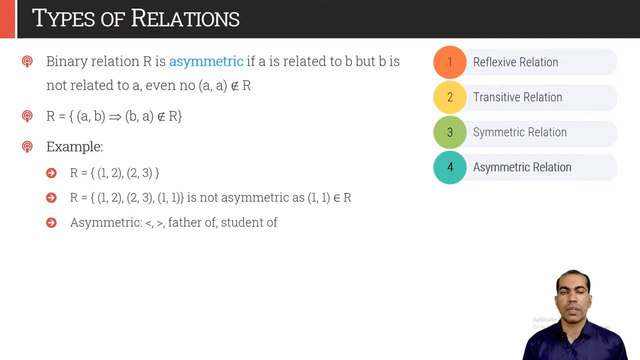 is not in relation. So father of student of mother of, they all are asymmetric relation, However, is equal to, is not asymmetric. Antisymmetric relation is same as asymmetric relation with minor difference. In case of antisymmetric relation, A comma A is also allowed Also. 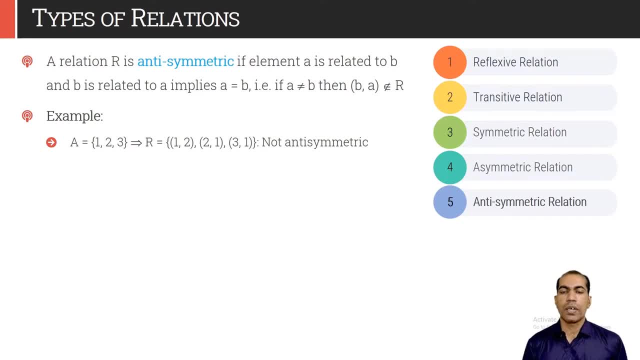 A can be related with A itself. So 1 comma 2 comma 3 is our set A And some relation on R is say, for example, 1 comma 2, 2 comma 1, 3 comma 1 is not antisymmetric Because 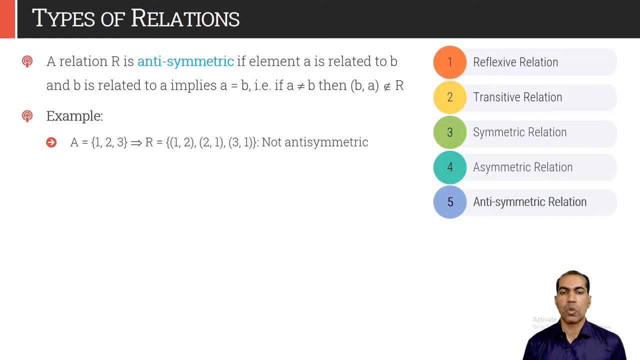 1, 2 is in R, So 2, 1 must not be there. But 2, 1 is present in R. So this is not antisymmetric relation: 1, 2, 2, 3 and 1, 1.. This is not asymmetric because 1, 1 is part of R. 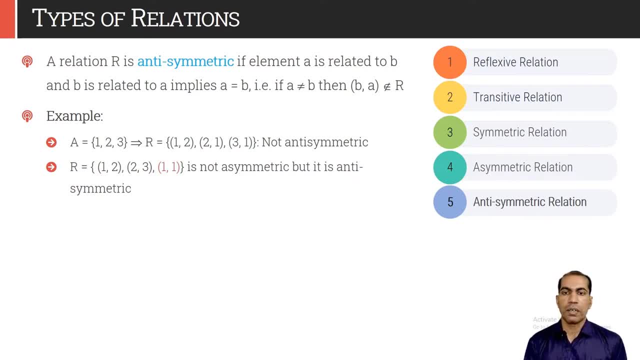 But it is antisymmetric. It is satisfying both the condition For 1, 2, 2, 1 is not present For 2, 3, 3, 2 is not present And a- a is allowed in antisymmetricity, So this one is. 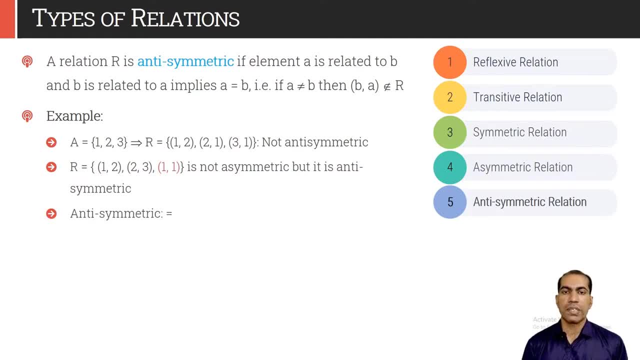 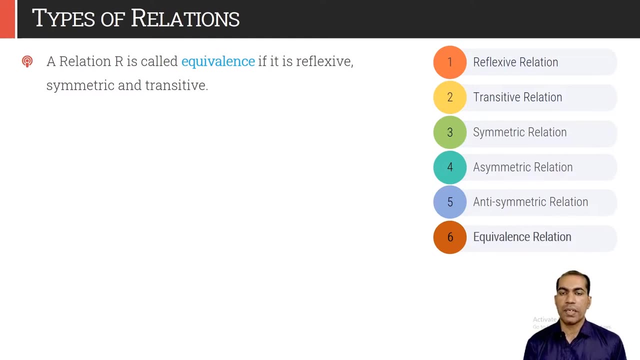 antisymmetric relation Is equal to. is antisymmetric relation less than greater than they are not antisymmetric relation. Relation R is said to be equivalence if it is reflexive, symmetric as well as transitive. So, given any relation, you can check whether it is reflexive or not symmetric. 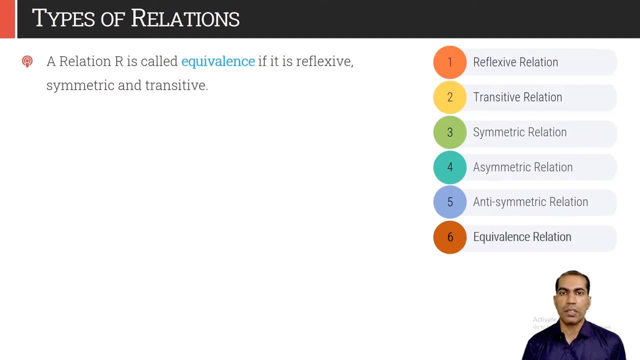 or not, transitive or not? If it is having all these three properties, then we will say that this is an equivalence relation. For example: is equal to, So is equal to, is reflexive or not? If it is having all these three properties, then we will say that this is an. equal to So, given any relation, you can check whether it is reflexive or not. If it is having all these three properties, then we will say that this is an equal to So, given any relation, you can check whether it is reflexive or not. If it is having all these three properties, then we will say that this is an. equal to So, given any relation, you can check whether it is reflexive or not. If it is having all these three properties, then we will say that this is an equal to So, given any relation, you can check whether it is reflexive or not. If it is having all these three properties, then we will say that this is an. 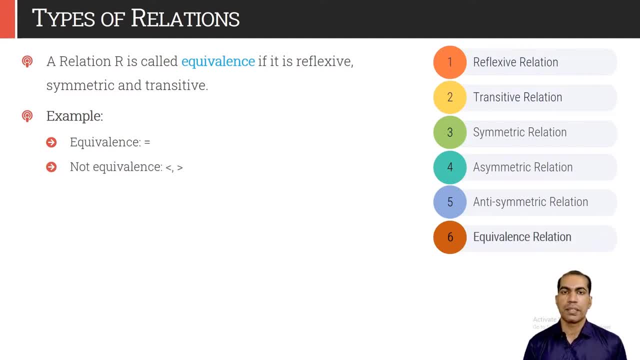 equal to. So, given any relation, you can check whether it is reflexive or not. If it is having all these three properties, then we will say that this is an transitive also and hence it is equivalence. Less than and greater than are obviously not. 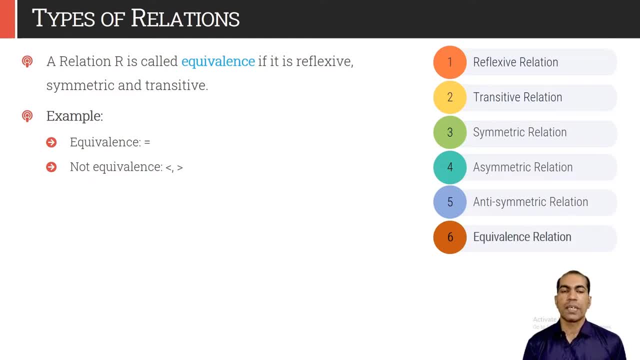 equivalence because less than is transitive, but it is not reflexive. Relation is said to be partial order if it is reflexive, antisymmetric and transitive And the set on which this relation is defined is known as a partial order set, or in short, 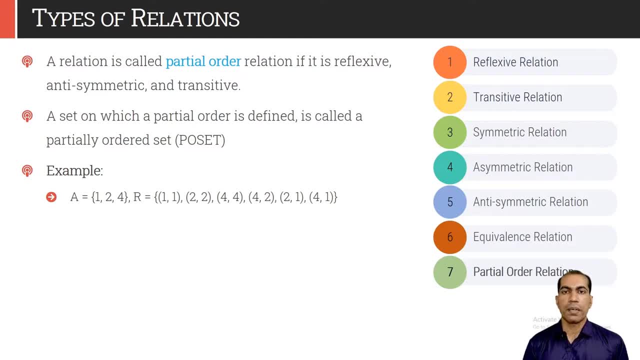 it is known as a poset. For example, let us consider: set A is equal to 1 to 4 and the relation R defined on set A is having these many elements. So we can check that 1, 1 is in R, 2, 2 is in R, 4, 4 is also in R. So this is a reflexive. 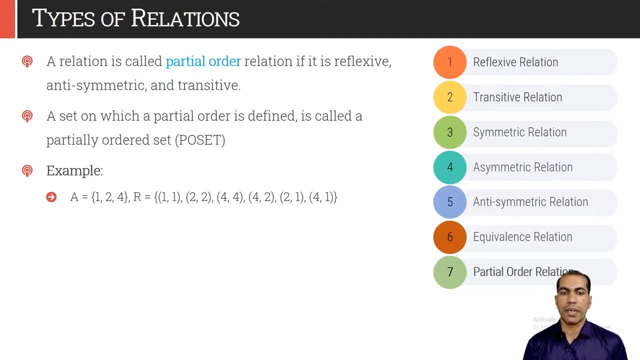 relation: 1, 1,, 2, 2, 4, 4 is allowed in antisymmetric. If 4, 2 is there, 2, 4 should not be in relation, which is true. 2, 1 is there, 1, 2 should not be in relation, that is fine. and 4, 1 is there, 1, 4 should. 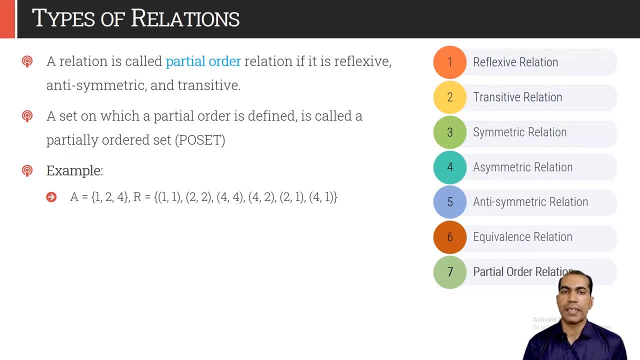 not be in relation. that is also true. So this relation is not in relation. 4, 1 is also antisymmetric As tuple 4, 2 and 2, 1 are there. 4, 1 must be in relation. 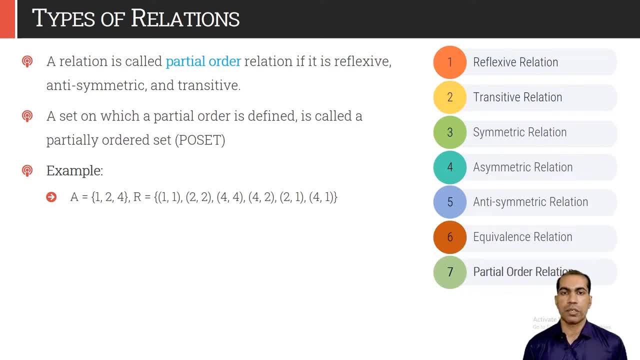 So 4, 1 is also there. So this relation is transitive relation also. So in short, it is partial order because it is satisfying all these three conditions. Divides over n. it is reflexive because number can divide itself, So A divided by A is true. so this is reflexive. 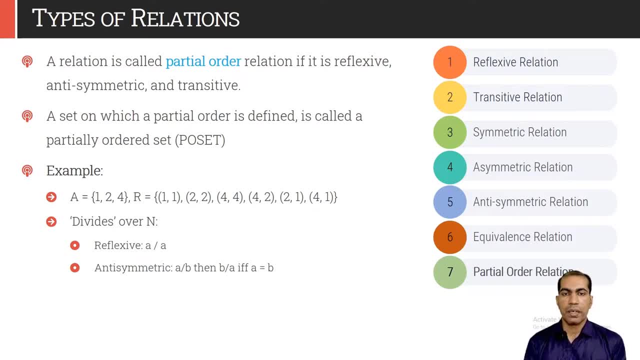 It is antisymmetric, because if A divides B, Then B divides. A is only true if A is equal to B, So A is related to A. then only A by B is possible. otherwise A- B is in relation, but B- A will not be in relation. 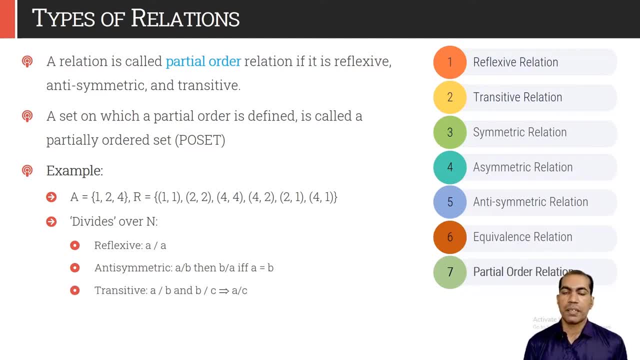 And it is also transitive, because if A divides B and B divides C, it implies A divides C. For example, 100 is divisible by 50 and 50 is divisible by 25. So 100 is also divisible by 25.. 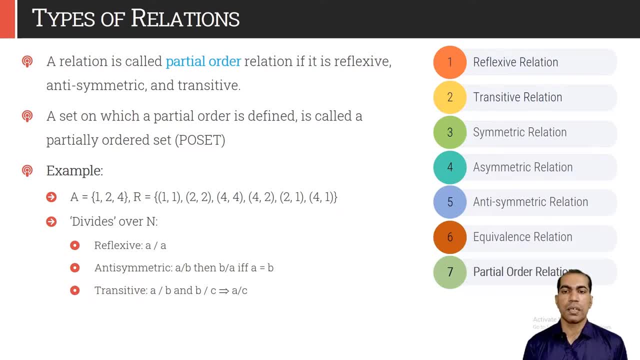 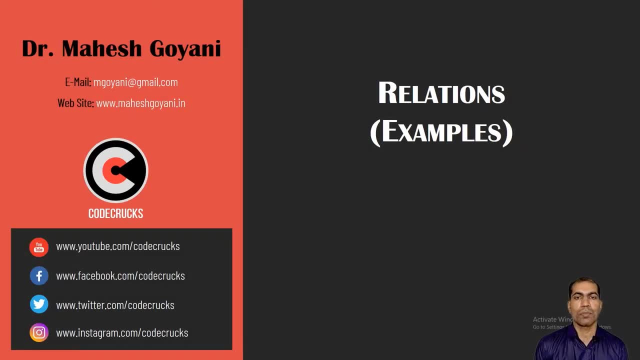 So it is transitive as well. So this relation is reflexive. This relation is reflexive relation, So this relation is partial order relation. Hello folks, welcome to Code Crux. This is Mahesh Guvani, and in this video I will be talking about relations and its example. 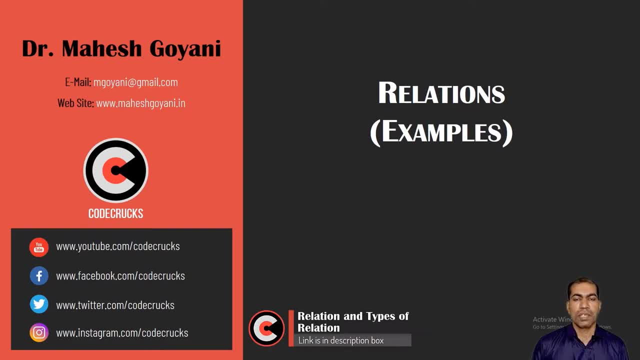 In previous video we have already talked about relation. We have introduced what is relation, which are the different types of relations, how to define relation and so on. So if you are not clear with the relation, I advise to watch that video. 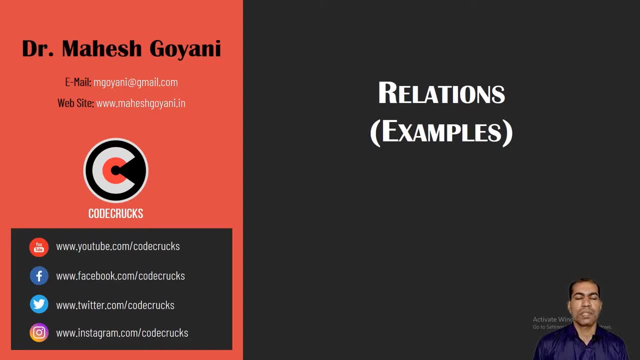 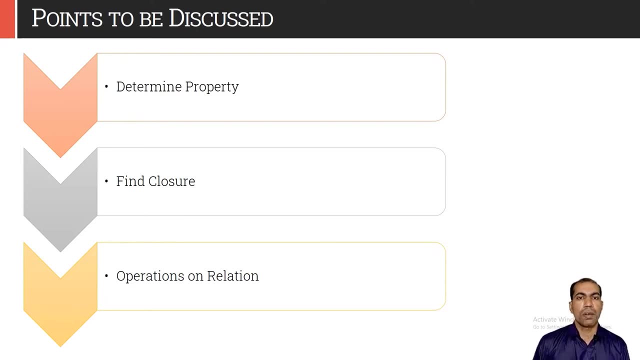 The link of that video is given in description box. In this particular video I will be talking about how to determine different properties of the given relation. We will also see how to compute the closure of any relation and we will talk on the various operations that we can perform on the relations. 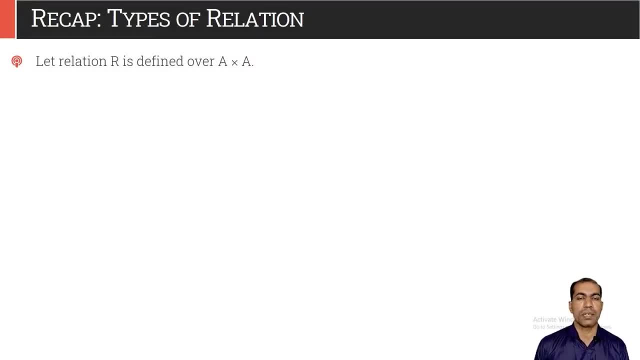 Let us recap the types of relations we have discussed in previous video tutorial. So I assume that capital R is a relation which is defined over a Cartesian product of A with itself. The relation R is said to be reflexive if for all the elements of capital A, A, A is. 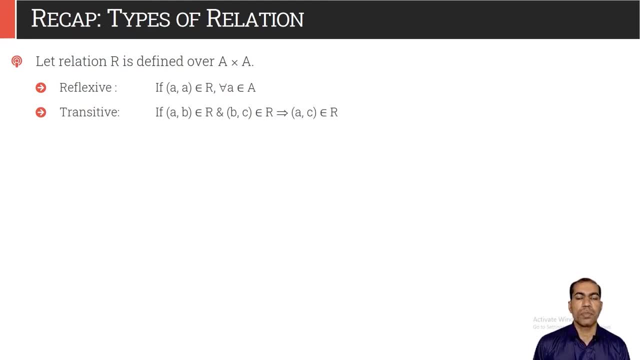 member of capital. R Relation is said to be transitive. if tuple AB belongs to R and BC belongs to R, then AC must be in R Relation. R is said to be symmetric. if A- B is in R, then B- A must be in R Relation. 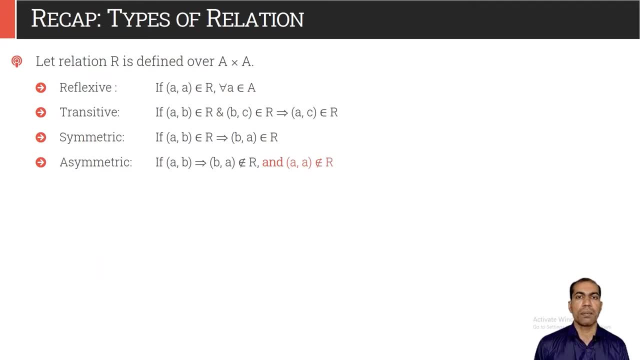 R is said to be asymmetric. if A- B is in R, then B? A must not be in R. even A? A is not allowed to be part of relation. R Relation is said to be antisymmetric. if A- B belongs to R, then B? A must not be in R. However, it is less restrictive compared to asymmetric. 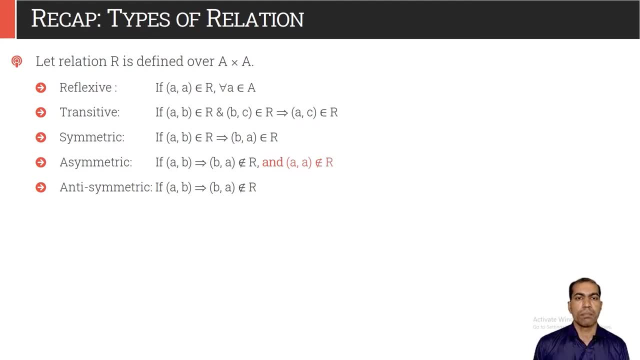 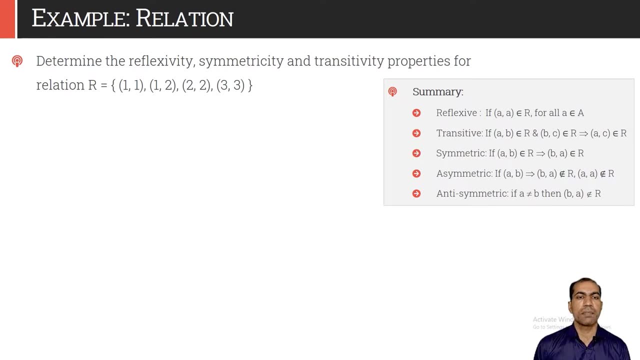 so A A can be part of antisymmetric relations Based on these properties- we will discuss few examples- Determine the reflexivity, symmetricity and transitivity property for the given relation. R is equal to 1, 1, 1, 2, 2, 2 and 3, 3.. 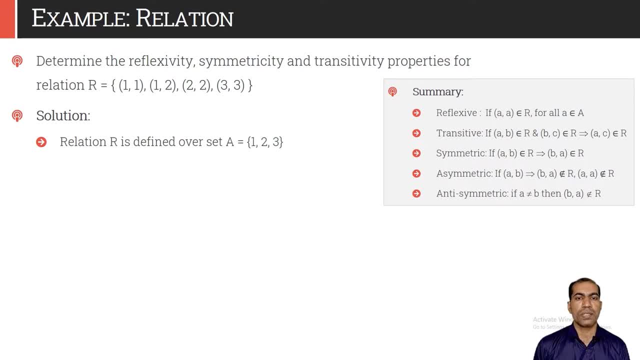 So, as we can see that this relation R is defined over set capital, A is equal to 1,, 2 and 3.. Relation is said to be reflexive if each element of A is related with itself in relation R. So 1, 1,, 2,, 2 and 3, 3 should be in R. 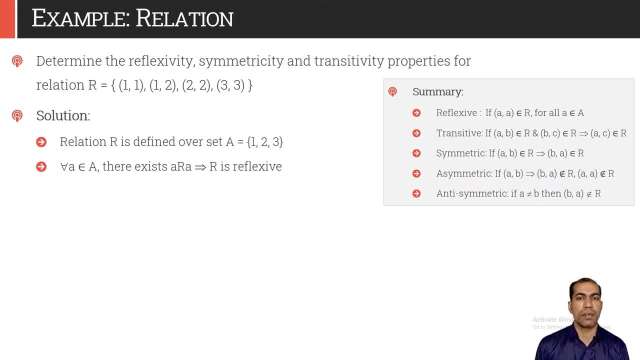 And as we can see that all 3 are present in R, it is reflexive relation. Relation is said to be symmetric. if A- B is in R, then B- A must be in R, But for given relation, R, 1, 2 belongs to R, but 2, 1 is not in R. 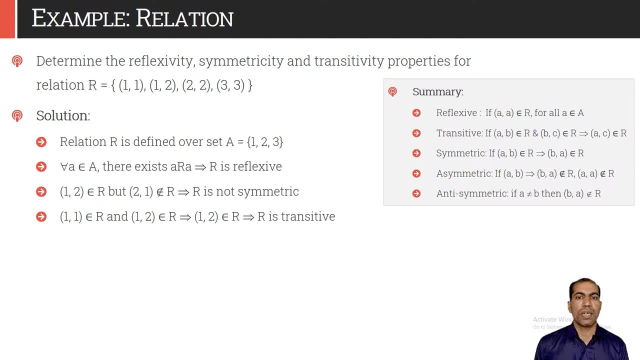 So this relation is not symmetric relation And for transitivity we have to check: if A, B is in R, B, C is in R, then A, C must be in R for all the tuples and hence this relation is transitive relation. Consider relation R is equal. 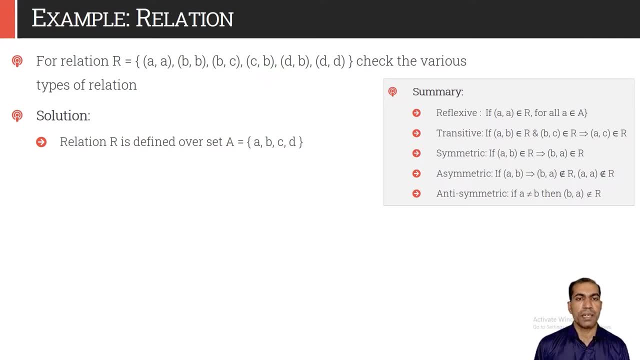 to AA, BB, BC, CB, DB and DD and we have to check various properties of the relations. So relation R is defined over set ABCD, as we can see from this relation R. R is not reflexive because tuple CC is not in R. R is not symmetric because DB belongs to capital R but BD is not in R. 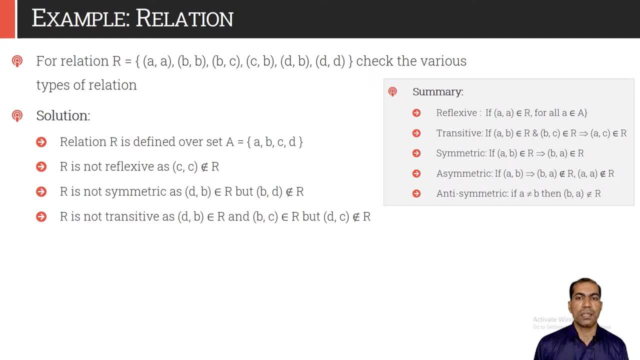 So this is not symmetric relation. R is also not transitive relation, because DB belongs to R and BC belongs to R, but DC is not in R. So this relation is not transitive. R is not asymmetric because BC belongs to R and CB is also in R, but B and C are not alike. 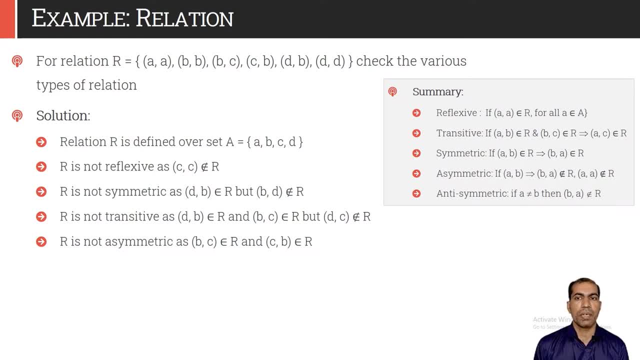 or we can say that AA, BB and DD are part of the relation and hence it is not asymmetric relation. Relation R is also not asymmetric due to the same reasons that B- C belongs to R as well as C. B is also R, which is not allowed in case of anti-symmetric relation. 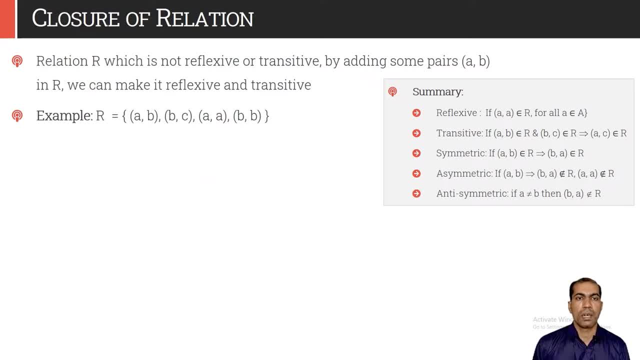 So this relation is not anti-symmetric as well. The closure of relation is computed by adding appropriate tuple into the relation, Relation R, which is not reflexive or transitive or symmetric. we can add few tuples into it and we can make that relation reflexive or transitive or symmetric. 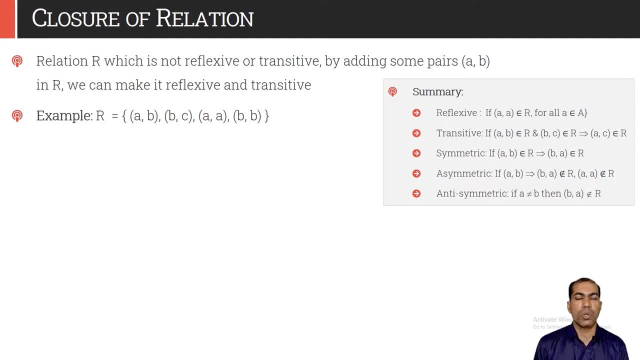 So that updated relation is known as closure of the relation. So assume that we have some relation. R is equal to AB, BC, AA and BB. To compute the transitive closure, we have to check the missing pairs, So as we can see that AB is in R, BC is in R but AC is not in R, So we have to add A. 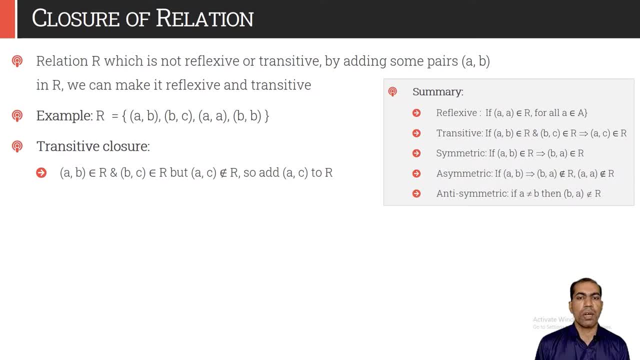 C into R. We have to check this for all possible tuples and if some tuple is missing, we can add that tuple into the relation. and finally, we can generate the transitive closure of R, which is represented as R star, So it contains all the tuples of R as well as newly. 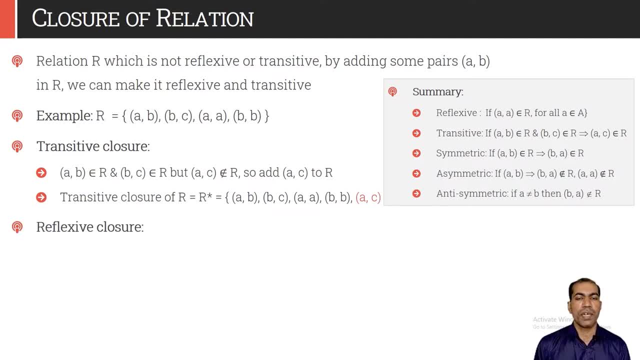 added tuple In same way to compute the reflective closure. the relation should always satisfy all the properties of reflexivity. That is, R is defined over set. So AA, BB and CC must be in R. then only we can say that R is reflexive. 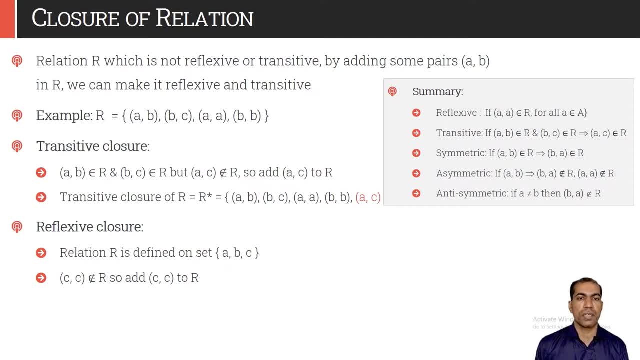 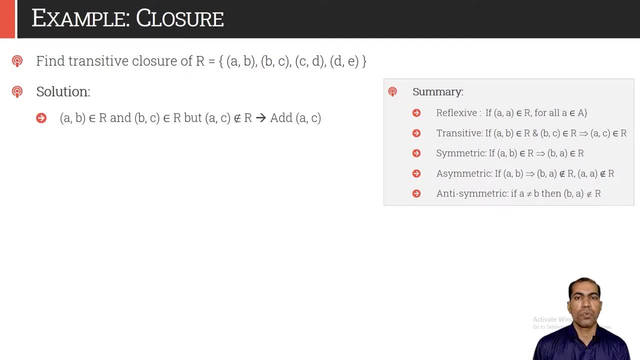 So we can say that R will be R star is equal to R star is equal to R star. so, for example, ADC is divided by the number of tuples of R, as well as newly added tuple C. C Find the transitive closure of relation R, defined as AB, BC, CD and DE. 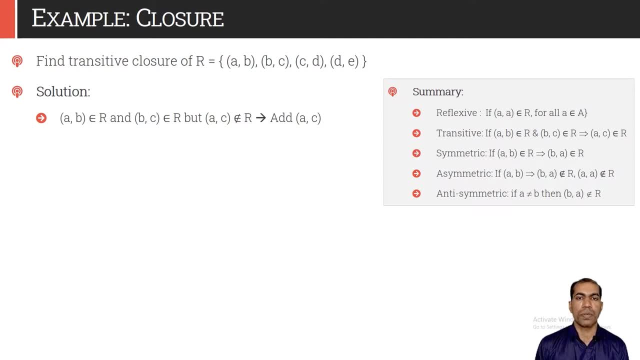 So again, we will check all the possible pairs and those pairs which are missing will add it into the closure of the R relation. AB is in R, BC is in R but AC is not in R, So we need to add AC into the relation. 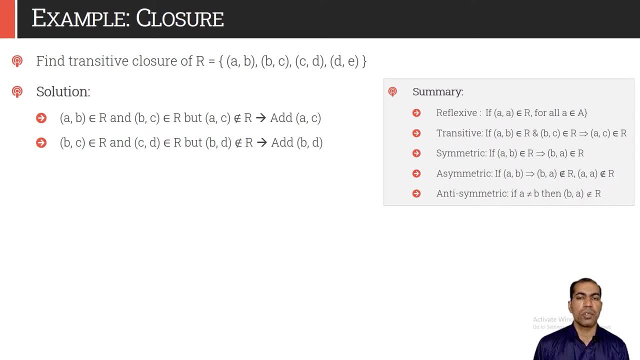 Similarly, BC belongs to C, So AB belongs to R. Here we need to add AC to the relation. Similarly, BC belongs to C, So here we need to add AC into the relation to r. cd belongs to r, but bd is not in r, so we shall add bd into the closure again. c, comma d. 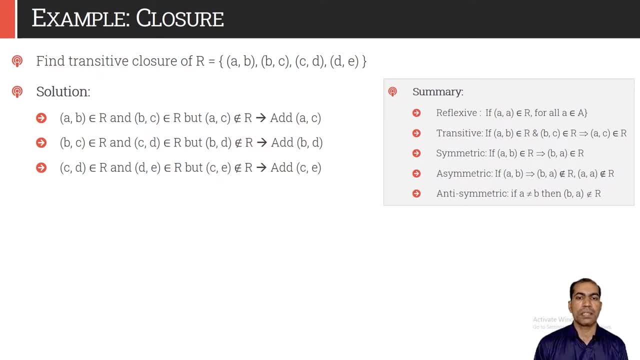 is in r, d comma e is in r, but c comma e is not in r, so we need to add that pair as well. so by adding these three pairs we can ensure that now r is a transitive relation, so the transitive closure of relation will be original tuples of r as well as newly added tuples a, c, bd and c e. now, if we make 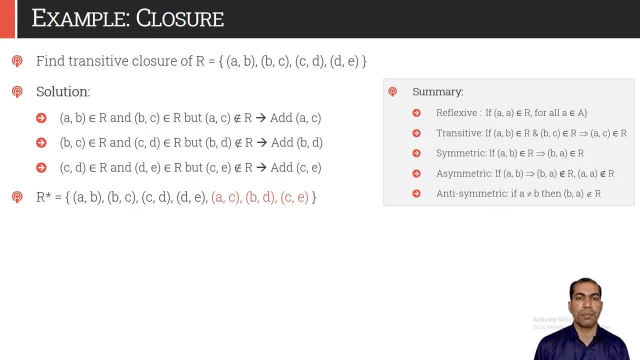 check for any two tuples, then the property of transitive will be definitely satisfied. so this is known as a transitive closure of relation r. find symmetric closure of relation r. that is defined as a, b, b, c, c, d and d? c. we know that symmetric closure means if a comma b is in r. 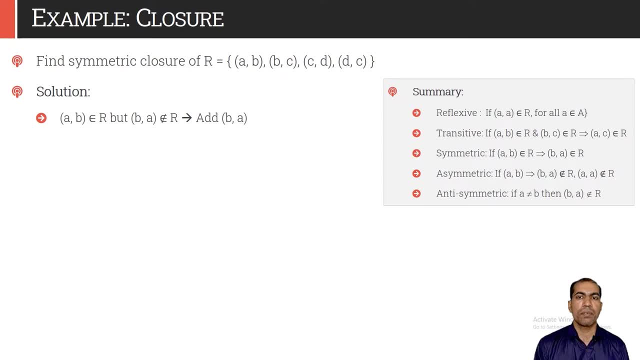 then b comma a must be in r. so that test we will make for each of the tuple and missing tuples will add into the relation. as we can see, a comma b is in r, but b comma e does not belongs to r, so we need to add b comma a. b comma c belongs to r, but c comma b is. 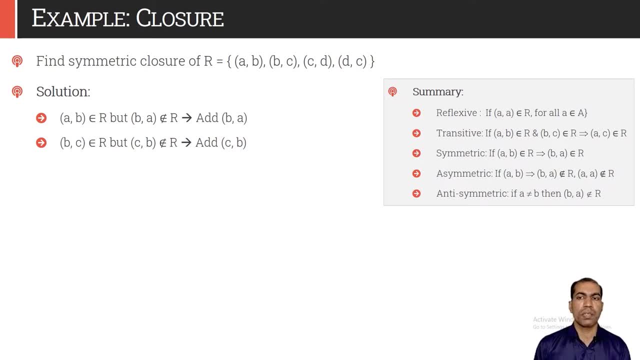 not in r. so again, we will add one more tuple, that is c, comma, b, c, d is in r. similarly d c is also in r. so we do not require to add any more tuple and hence the symmetric closure of relation. r would be all the original tuples as well as newly added. 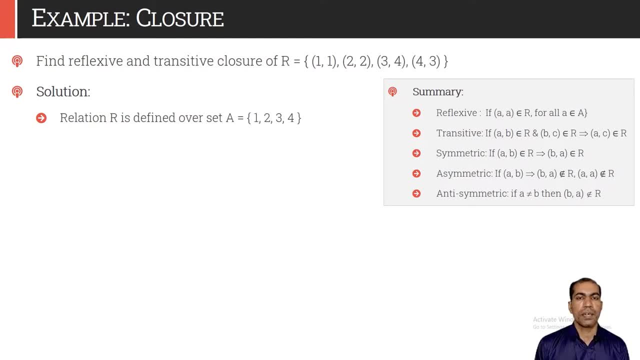 two tuples, b a and c. b find reflexive and transitive closure of relation r: 1, 1, 2, 2, 3, 4 and 4, 3. as we can see from the relation that it is defined over set 1, 2, 3, 4 for reflexivity. 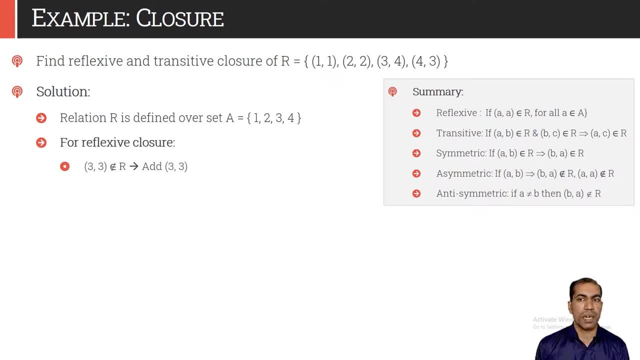 1, 1, 2, 2, 3, 3 and 4. 4 should be in r, but 3, 3 and 4: 4 are not in r, so we will add it and we'll create the reflexive closure of the relation that is given as like this: 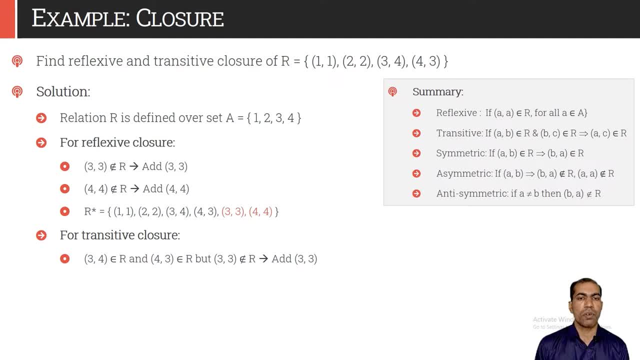 for computing the transitive closure. we will check that 3 comma 4 is in r. 4 comma 3 is in r, so 3 comma 3 should be in r. so just by adding this one element we can create a transitive closure of. 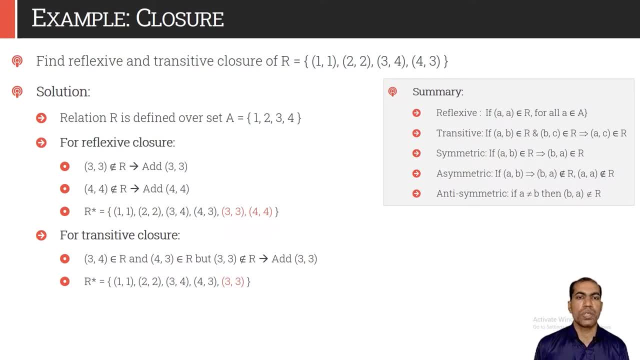 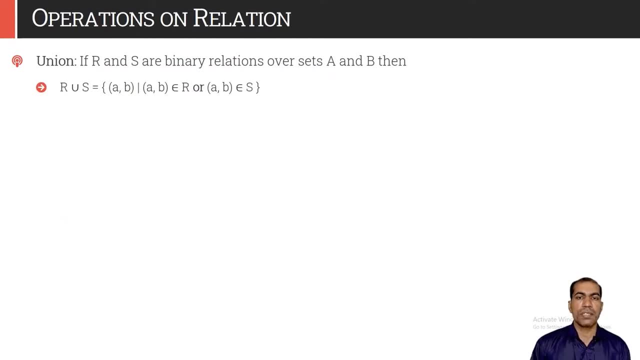 relation r. so this is how we can compute various closures of given relation, by adding the appropriate tuples into the relation. let us have a look at various operations on the relations of the union. operation is defined over two relations, let r and s. our binary relations are defined over sets a and b. so union of these two relation is 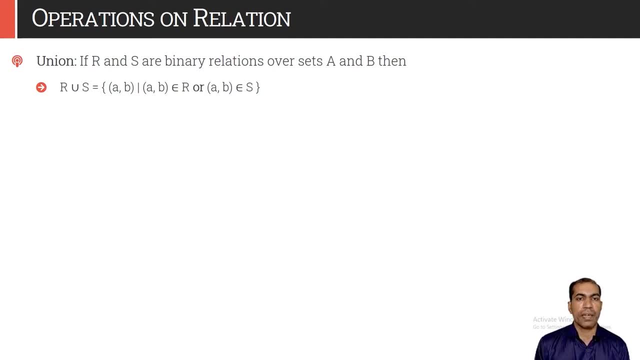 given as tuple a comma b, where a comma b should be in r or it should be in s. so it is something like a union of normal crisp set. so elements from set a and set b we are merging. similarly, to compute the union of relation we have to fetch the tuples from both the sets, both the. 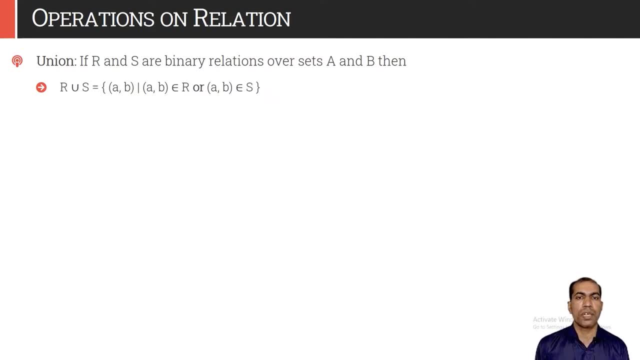 relations r and s. so this is the definition of union of two relations. consider: relation r is 1, 1, 2, 2, 3, 3 and relation s is 1, 1, 1, 2, 1, 3, 2, 2, 2, 3 and. 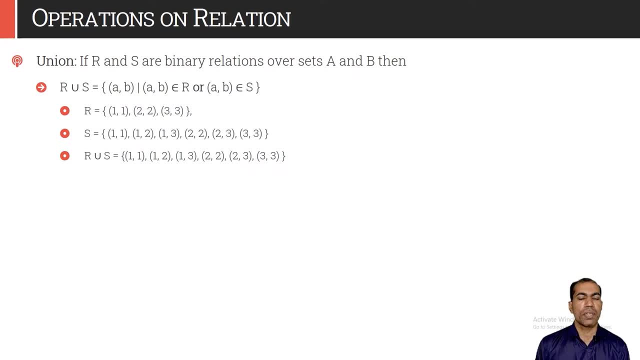 3, 3. so union of that would be: 1, 1, 1, 2, 1, 3, 2, 2, 2, 3 and 3, 3 greater than or equal to this relation is union of greater than, and is equal to and less than or equal to this relation. 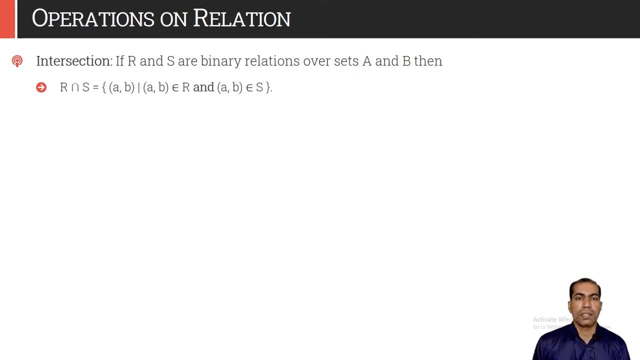 is union of less than and is equal to operator. just like union of relations, we can also define intersection of the relation. the only condition is that now the tuple should be common in both the relations. so r intersection s is collection of all the tuples, a comma b. 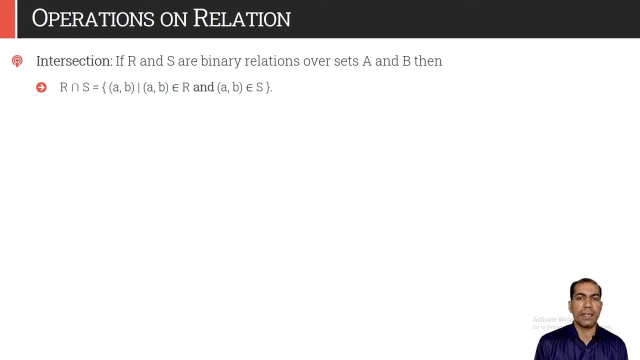 such that the tuple is present in relation r and it is present in relation s. so only common tuples from both the relations will be added to the intersection. so assume that r is having elements one, one, two, two, three, three and s is having elements as mentioned here. 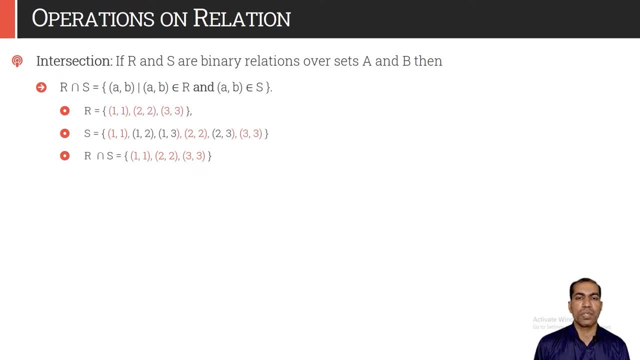 As we can see that elements highlighted in red are common in both the sets and hence that would be the output of intersection operation of these two relations, that is 1, 1, 2, 2 and 3, 3.. Is divisible by 10. this relation is intersection of: is divisible by 5 and is divisible by 2.. 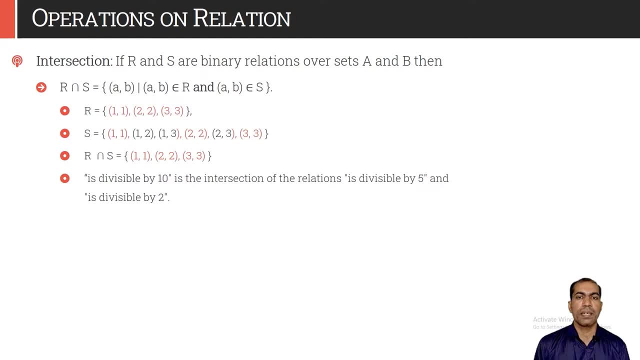 That's sure that if number is divisible by 10, then definitely it will be divisible by 5 as well as by 2.. So this is how we can formulate the intersection of the relations. Complement of the relation is defined as those tuples which are not in R, that is, R bar is. 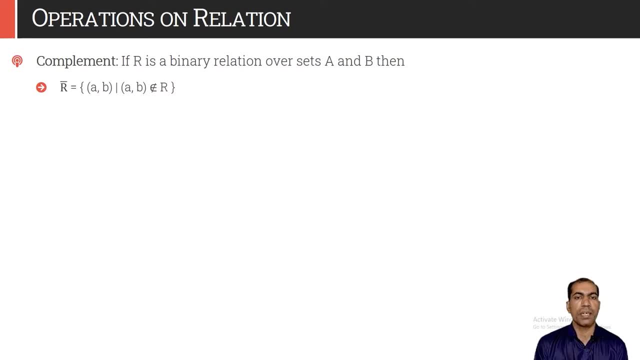 given as collection of tuple AB, such that AB does not belong to relation R. Let's set A is equal to 1, 2, 3 and we are defining the relation over Cartesian product A cross A. So A cross A would take 9 tuples and assume that we have some relation R. that is 1, 1, 2. 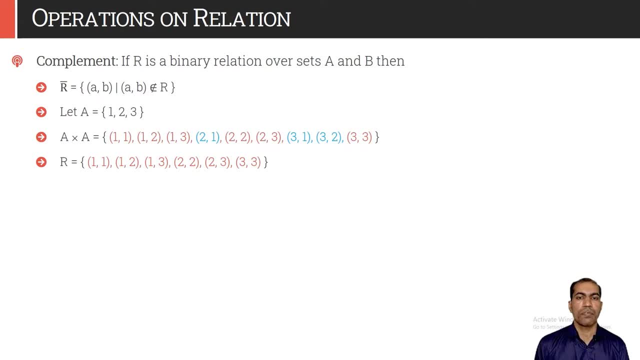 1, 3, 2, 2, 2, 3 and 3, 3.. So in fact, this relation is A less than or equal to B. So you can see that the first element of all the tuples is always less than or equal to. 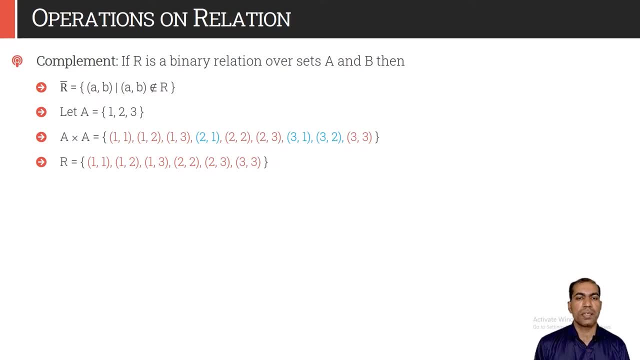 the second element. So R represents less than or equal to relation. Elements which are highlighted in red are in R and those are in blue in A cross A are not the part of R. So when we compute the R bar or the complement of R, it would take 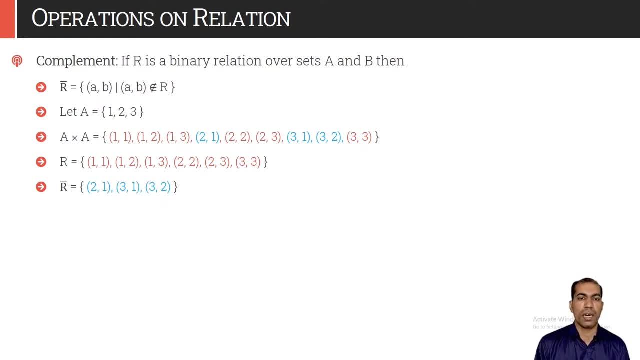 only those tuples highlighted in blue which are not in R, So R bar would be 2: 1, 3, 1 and 3: 2. Relations like is equal to and not equal to, are the complement of each other. Belongs to, does not belongs to less than greater than or equal to greater than less. 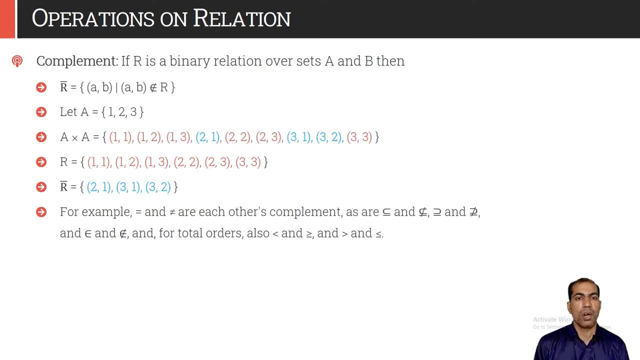 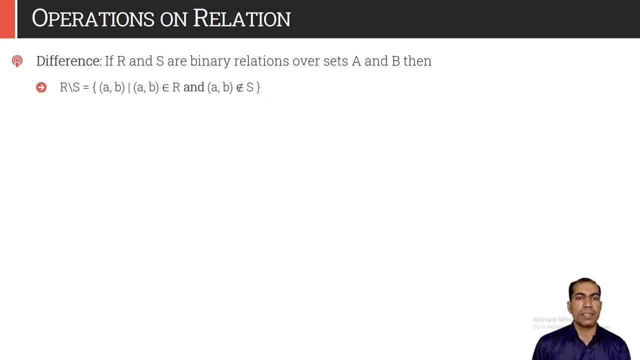 than or equal to subset, not subset. All these operators are complement operators. Difference of the relation: So let: R and S are the two relations Defined over sets A comma B. So difference of relation is given by R. difference S is equal to collection of all the tuples A comma B, such that AB is present in R, but it should. 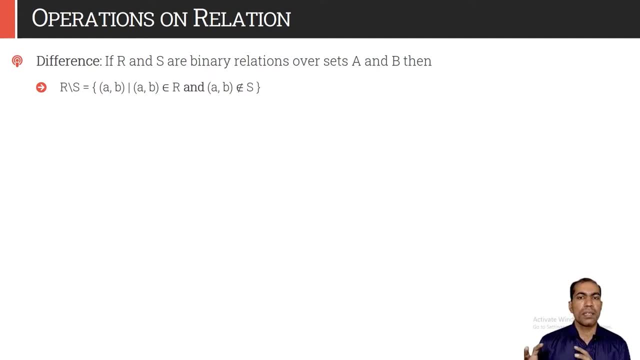 not be in S. So we shall subtract all the tuples of S from R. Similarly, S minus R or the S difference, R is given as collection of tuples AB, such that AB is not in R but it is in S. So that is quite simple. 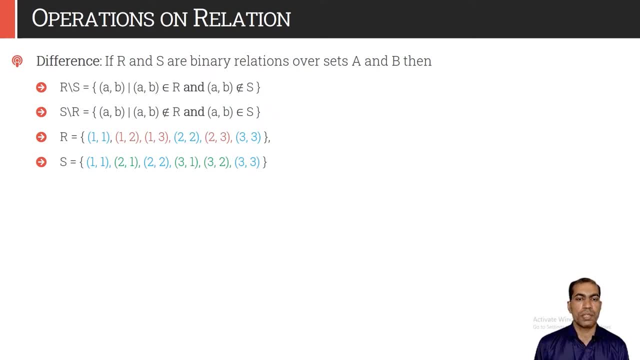 Let R is equal to: 1. 1, 1, 2, 1, 3, 2, 2, 2, 3, 3, 3.. So this is less than or equal to relation And capital: SB: 1, 1, 2, 1, 2, 2, 3, 1, 3, 2, 3, 3.. 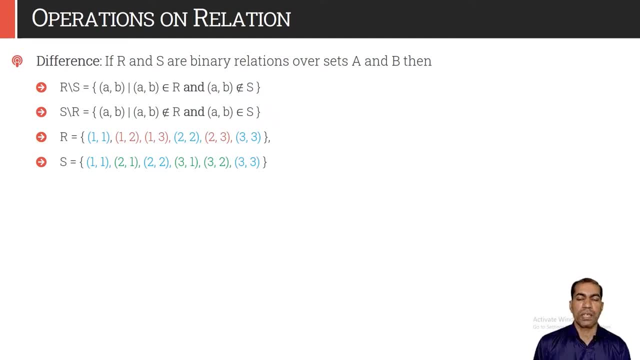 So this represents greater than or equal to relation. As you can see that in R first element is always less than or equal to second element. in all the tuples In S first tuple is always greater than or equal to the second tuple. So that is quite simple. 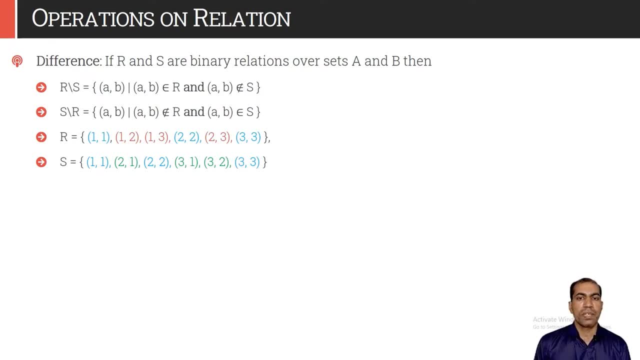 Now, elements highlighted in red are only present in R, elements highlighted in green are only present in C and elements highlighted in blue are common elements. they are in both. So when we compute R minus C or the R difference C, all the blue elements will be subtracted. 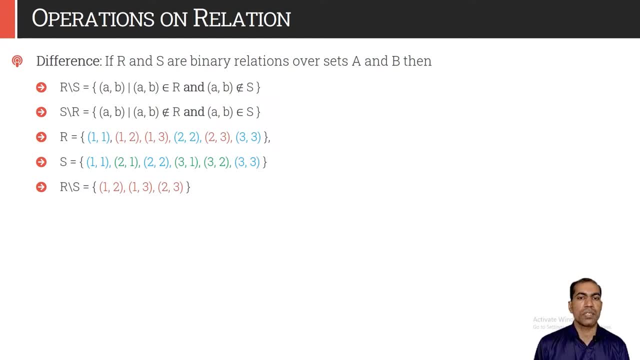 because they are common. So when we do R minus S, those elements will be cancelled out and we will be left only with the red colored element. those are 1, 2, 1, 3 and 2, 3.. 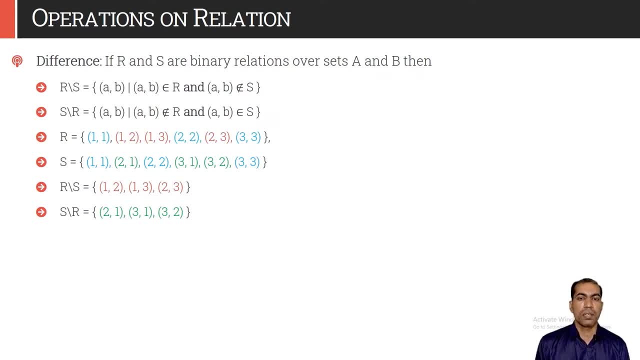 Similarly, when we compute S difference R, that is S minus R. so all the blue elements will be subtracted from the set S or relation S and we will be left with 2, 1, 3, 1 and 3, 2.. 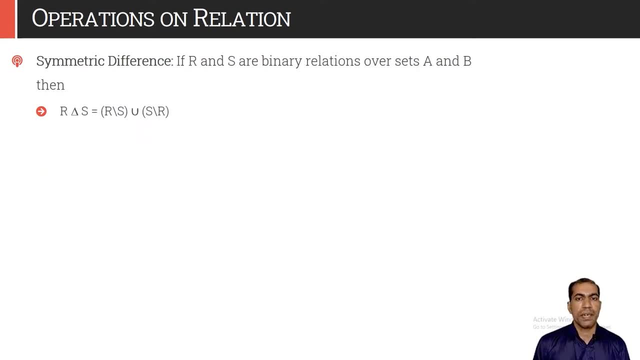 This is how we can compute the difference of the relation. Symmetric difference is given by R delta S. it is simply union of R difference S and S difference R. That is known as a symmetric difference. So on previous slide we have already seen these two relations, R and S. and if we compute 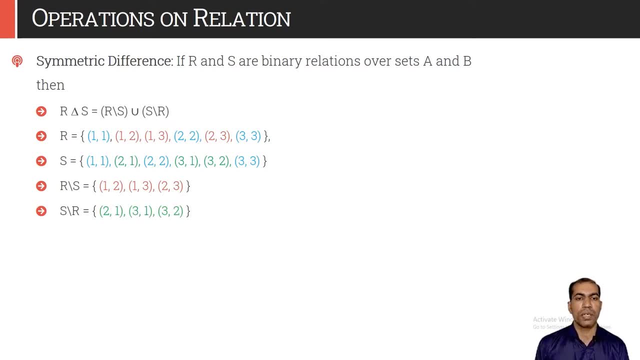 R difference S that was 1, 2, 1, 3, 2, 3, and the S difference R was 2, 1, 3, 1, 3, 2.. So R difference S contains red elements, S difference R contains green element and to: 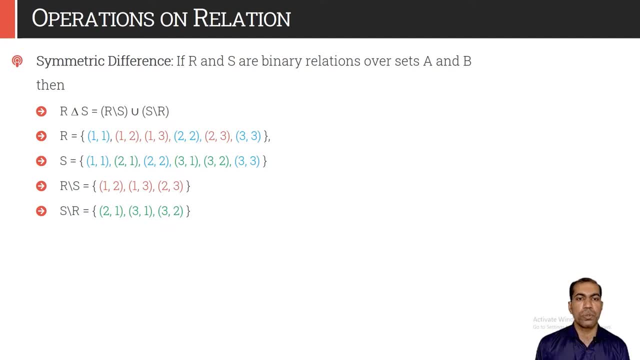 compute the symmetric difference, we need to take union of these two relations. So that would be the union of that. So it would contain red as well as green elements. Compositions of the relation Up till now, whatever operations we have discussed, all the relations, that is, relation R and S. 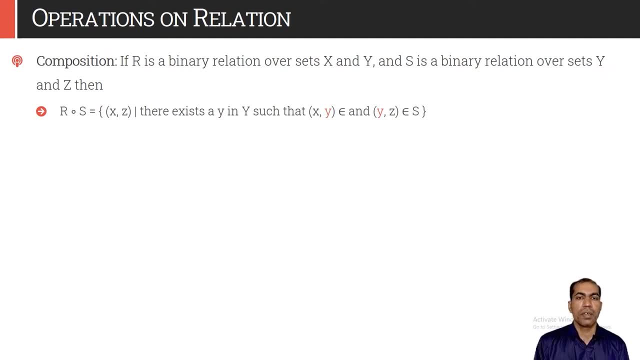 were described from the same universe, That is, R and B were described over A cross B. In case of composition, relation R is described over set X and Y and relation S is described over set Y and Z. So all the elements r will have form xy and all the elements in s will have form yz, because their universe. 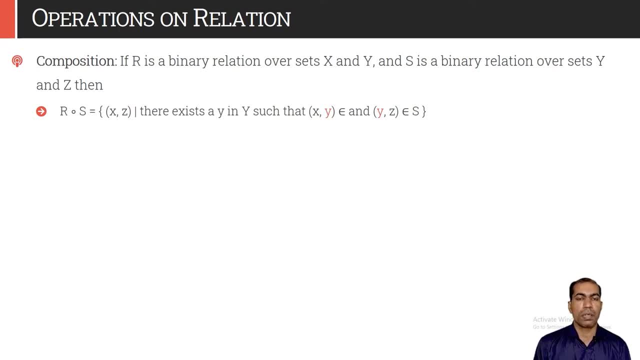 are different, So that now we need to find the composition of that Composition of relation r and s is represented by this notation. It is a collection of all the tuples xz, such that for y in capital Y, xy belongs to relation r and yz belongs to relation s, As we know. 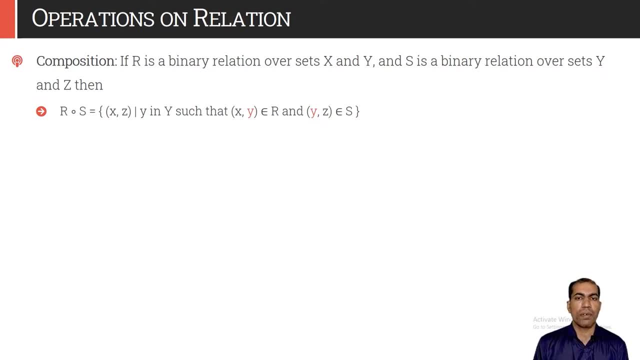 that universe of r is x, x, y and universe of s is y, x, z. so all the xy tuple will be in r and yz tuple in S. So xz tuples which are having y common between them, is mother of composition, is parent of will yield, is maternal, grand parent of. So we can find some. 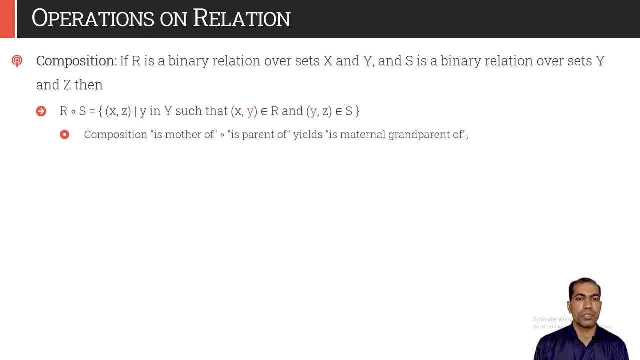 interaction between the two different relations by taking the compositions of that isfather of composition is mother of yield, the mother of, So based on that you will get, so we can already know that about representation, et cetera, grandmother, Let us take one example: Relation R is having tuples, AC, BD and CA, and relation 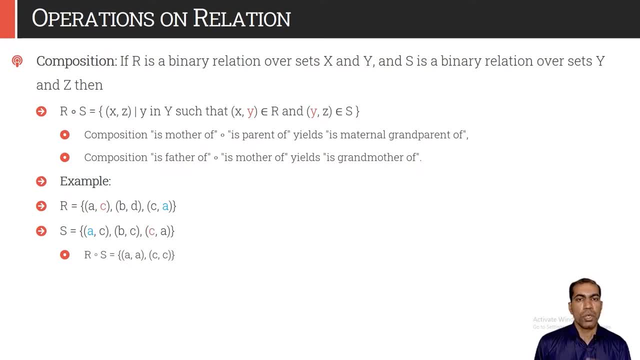 S is having tuple AC, BC and CA. To compute the composition of R over S or composition of R with S, we shall find out common Y between R and S. So Y is the second component in R and it is first component in S. So we have to find out such pairs And for those pairs. 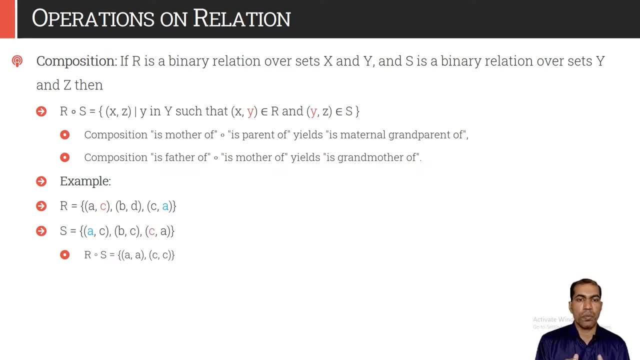 will be in R composition. S So is in R. So for this tuple, Y is equal to C, So we will check in relation S. Is there any tuple which is starting with C? Yes, is there, So that will be in composition. Similarly, another tuple is, So in this case, 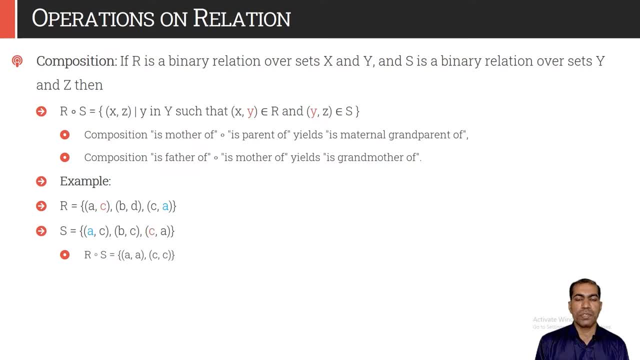 Y would be D, but there is no tuple in S which is starting with D, so we have to skip that tuple. the third tuple in R, which is C comma A. so in this case Y is equal to A. so we have to scan S and we have. 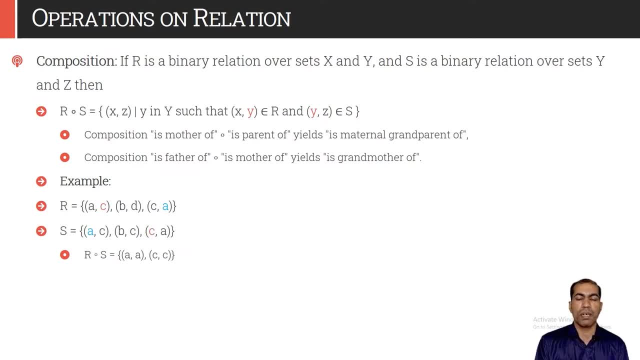 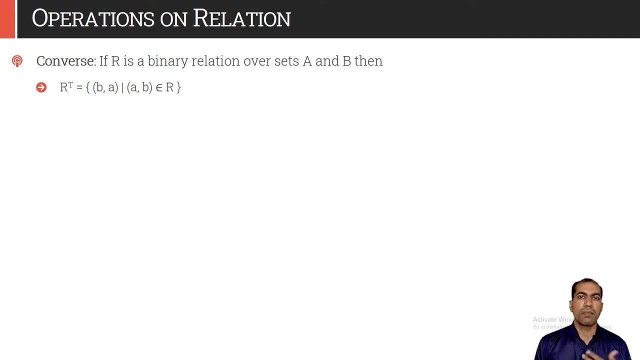 to find out all the tuples which are starting with A. so there is only one tuple which is A comma C. so the C comma C would be in composition of these two relations. Conversion of relation. if R is a binary relation over set A and B, then the converse or the transpose of the relation. 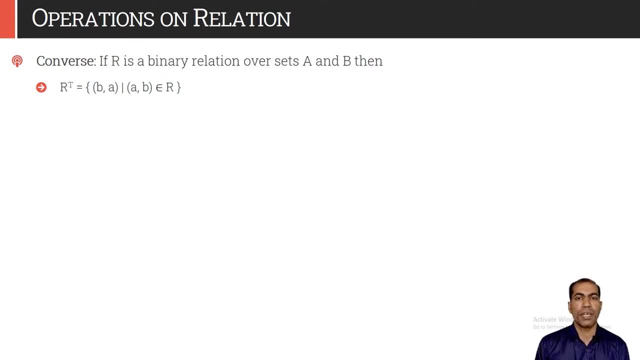 is given as R transpose is equal to B comma A where AB is in R. so if tuple AB is in R, then B comma A would be in the converse of that relation. let R is equal to 1, 2, 2, 3, 3, 1. 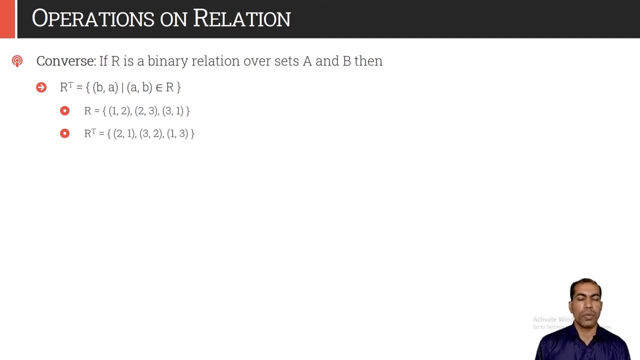 so R transpose would be: 1. 2 will become 2, 1, 2. 3 will become 3, 2 and 3, 1 will become 1. 3 is equal to, is converse of itself, and same is true for the not equal to greater than and less than. 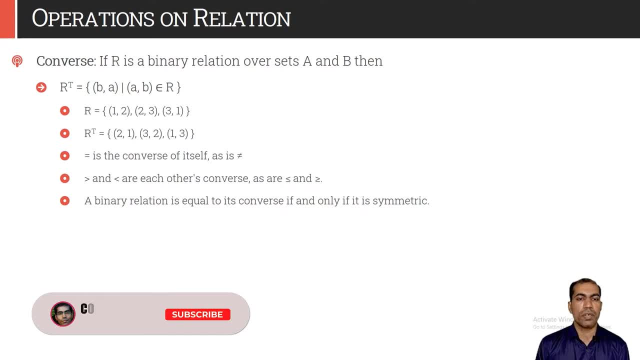 are converse of each other, and so are less than or equal to and greater than or equal to. from the definition of converse, it is very clear that you can find the converse of relation if it is a symmetric relation. these are the various properties of the operations we have performed. 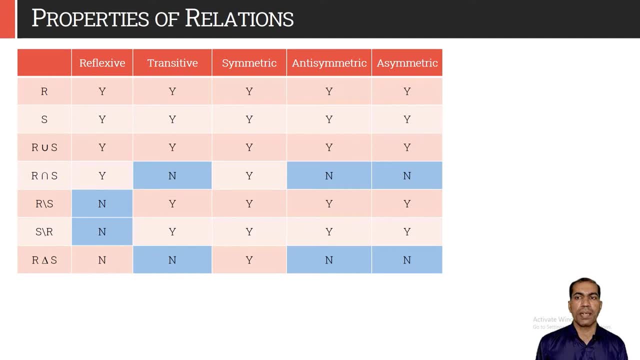 any relation could be reflexive, transitive, symmetric, anti-symmetric, asymmetric and so on, and the operations are the same. so we have to find out the converse of the relation. R intersection S is reflexive. if relation R and S are reflexive and R intersection S will, may not. 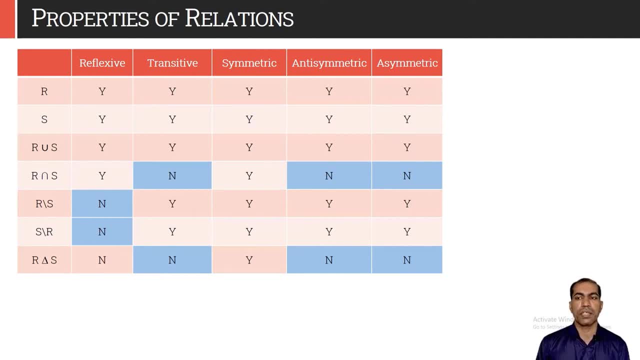 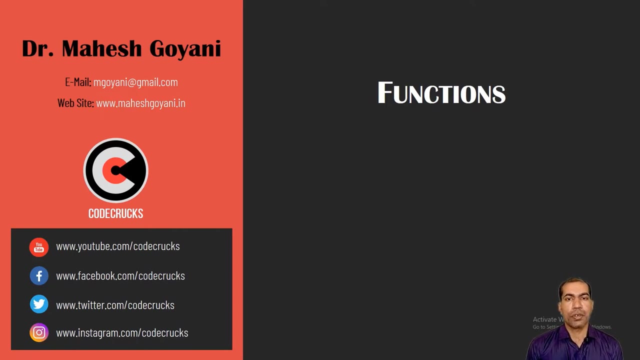 be transitive. always. similarly, it may not be anti-symmetric as well as asymmetric, so this table summarizes the various properties of the relations, as well as operations performed on the relations. hello folks, welcome to code crux. this is Mahesh Gujani, and in this video I am going to 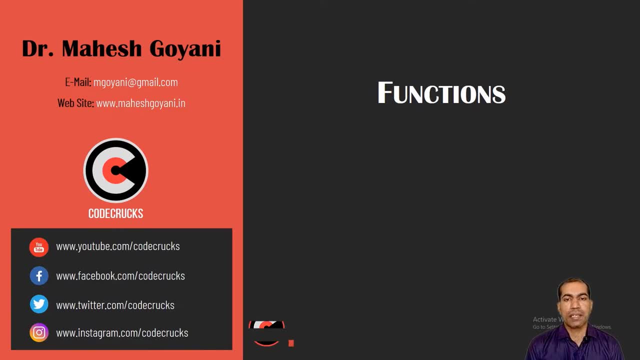 talk about functions. so functions are basically derived from the relations. so at top we have a set of Cartesian product from that we are deriving the relations. so Cartesian product is super set of relations and functions are derived from the relations. that is, functions are subset of relations. many natural phenomenons. 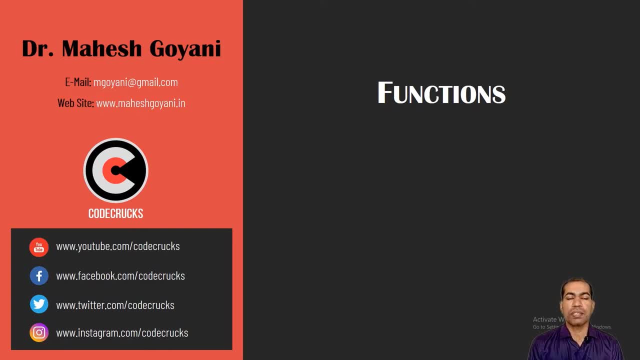 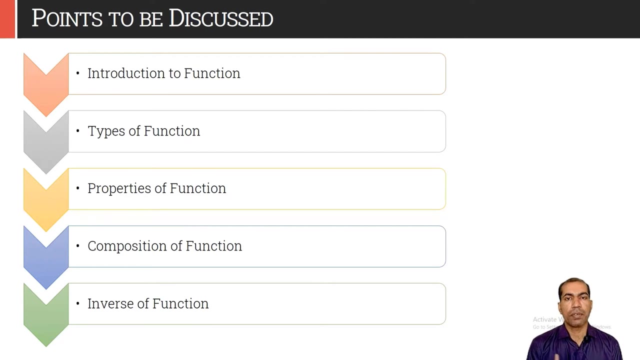 are effectively represented using the functions. so functions are basically a mathematical concept which maps one set with the another set by some relation. So we are going to talk about introduction of the function. we will discuss various types of functions, which are the properties of the functions. we will also talk about composition. 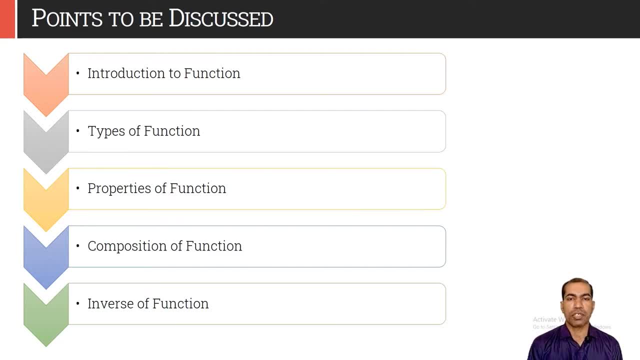 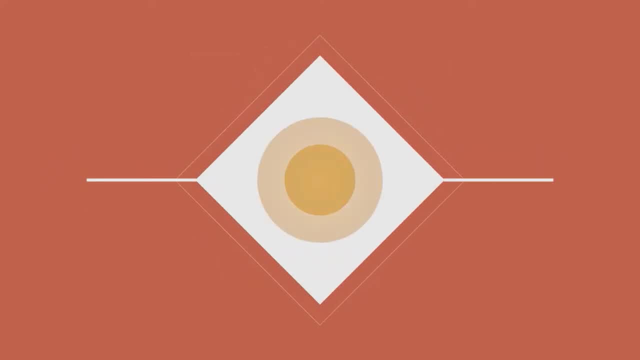 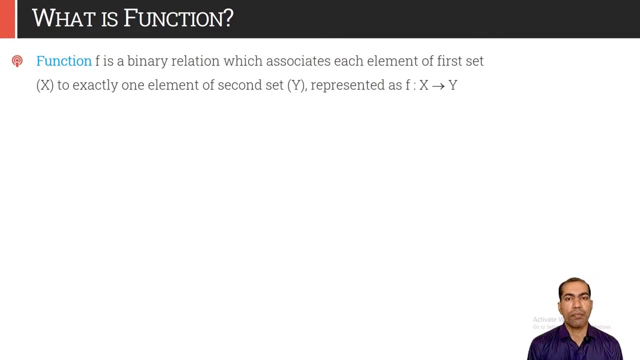 of the function, and we will conclude the video with the inverse function. so let's get started. Function F is a binary relation which associates the relation between the two functions. Function F is a binary relation which associates the relation between the two functions. Function F is a binary relation which associates the relation between the two functions. 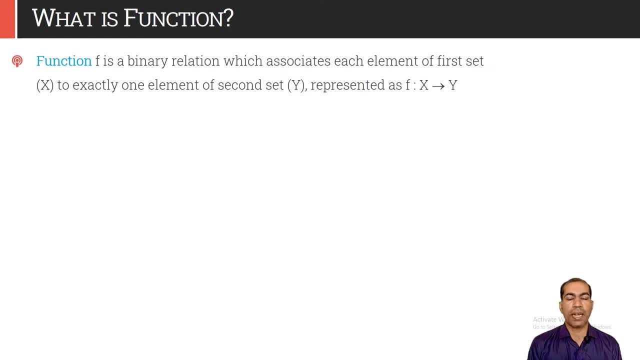 each element of first set X to exactly one element of second set Y and it is represented by F. colon X gives Y. it says that all the elements of first set capital X must be associated with exactly one element in second set Y. so none of the elements from set X should be left and none of the element of X. 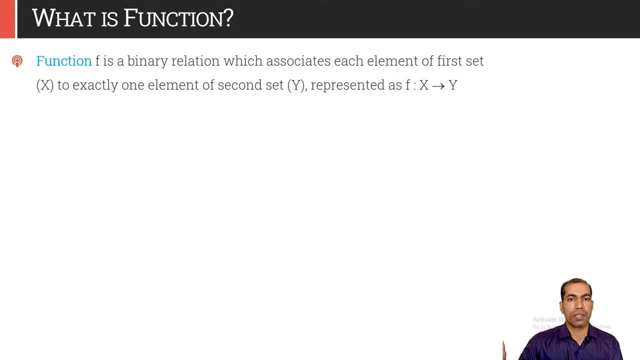 should be associated with multiple elements in Y. however, multiple different elements from set X may be connected with the identical element in Y, but one element should not have a. two different values in Y relation are, which is subset of Cartesian product of X cross. Y is a function if it satisfy. 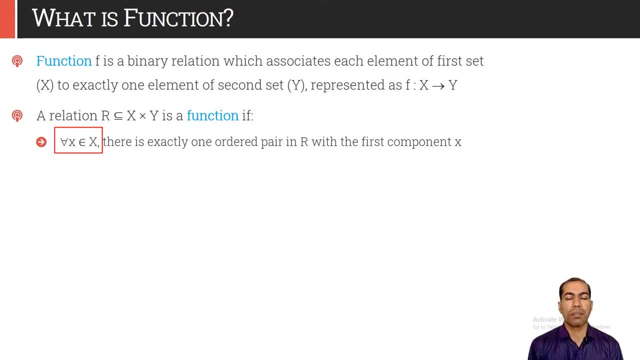 following condition: for all small x belongs to capital X. that means for each element of first set X should be associated with multiple elements. in element of set X there exists exactly one ordered pair in R, such that its first component is obviously small x, because it is a Cartesian product. So definitely first component should. 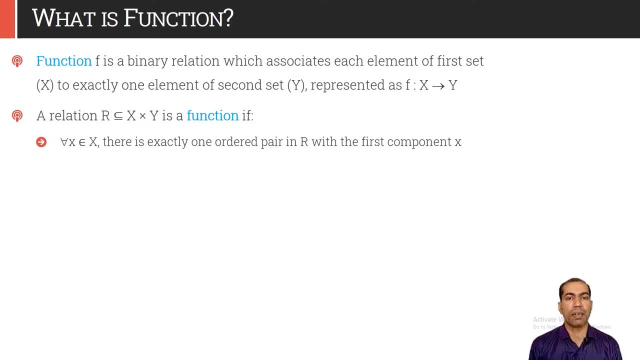 be from capital X and the second should be from capital Y set. However, it is not compulsory that all the elements of Y are connected to X. So there must be a connection from X to Y for all elements. but some of the elements in Y may not be connected. that is allowed, but element from X. 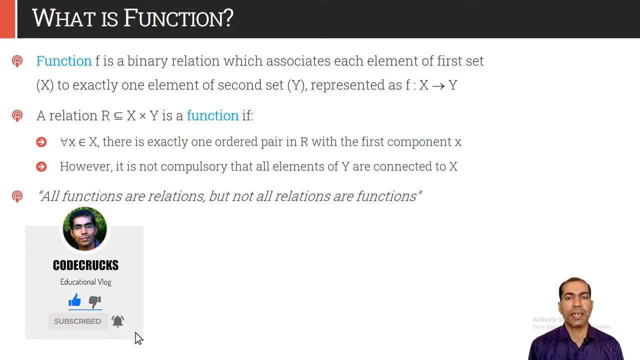 should not be left out With this discussion. we can claim that all the functions are relation, but not all the relations are function. that is very obvious. Have a look, this is not a function, because all the elements of X must be connected with some of the elements in Y. 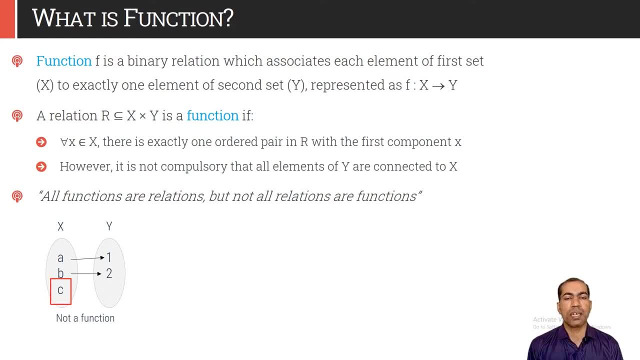 as per the definition. but here element C is not connected with any of the element in Y, So this is not a function. So this is not a function. So this is not a function. So this is is not a function. This is also not a function because all the elements of x are connected. 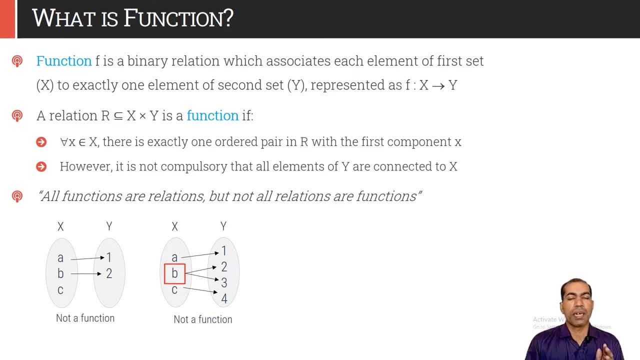 but element b is having two different values in y, and hence this is also not a valid function. This is function because all the elements of x are connected with at least one element in y and all the elements in x are having exactly one association If there would be multiple, as like. 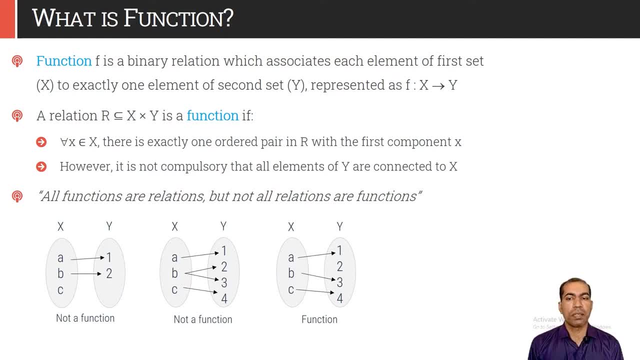 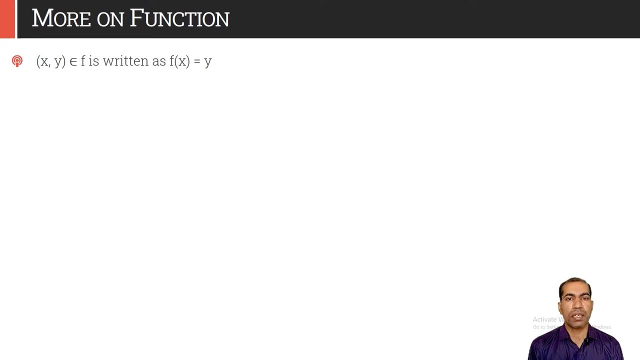 in the previous figure, then it would not be function. However, 2 in y is not connected, but that is allowed. Component in y can be skipped, but elements in x cannot be skipped. If a tuple x comma y is member of function, then typically we are writing it as f of x is equal to y, or? 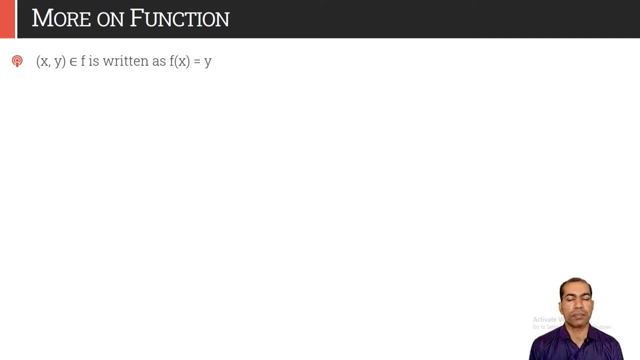 sometimes we are also writing it as a y is equal to f of x. In this case x is known as independent variable Set of all first elements of member of function. f forms domain of f and it is denoted by dom of f. So we are typically selecting x from some set and we are calculating y, So that input set is known. 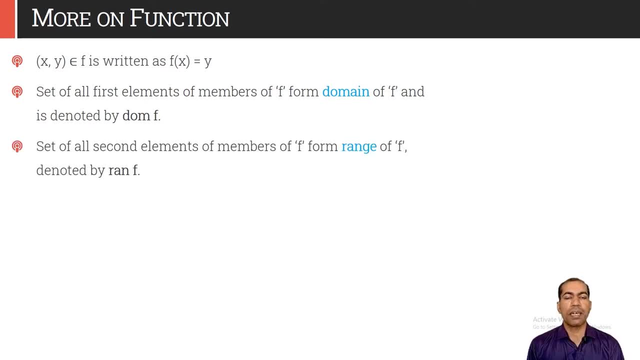 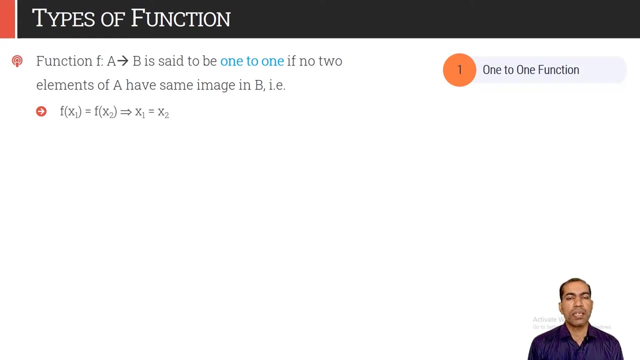 as a domain of the function and the output generated by this function is known as range or co-domain of the function. So that would form the second argument into the tuple x, comma y. So that is nothing, But it is an output of the function. Let us discuss various types of function. Function f from a to b. 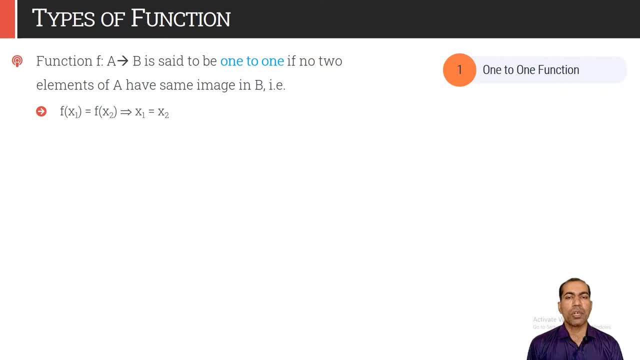 is said to be one to one if no two elements of a have same image in b. That is, if you put different arguments into the function, that is, x1 and x2, and function results same output. That is, if f of x1 is equal to f of x2, then x1 and x2 must be same. Then only function can have a same output. Otherwise 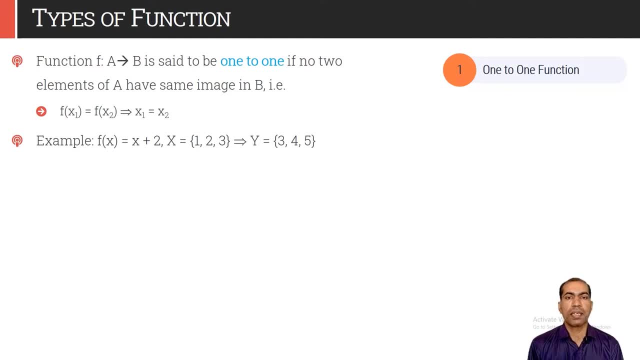 it will generate different output. For example, let us consider the function f of x is equal to x plus 2.. If our domain capital X is 1 to 3, then by putting the x is equal to 1 into f of x will generate output 3.. For x is equal to 2, it will produce output 4, and for x is equal to 3, it will 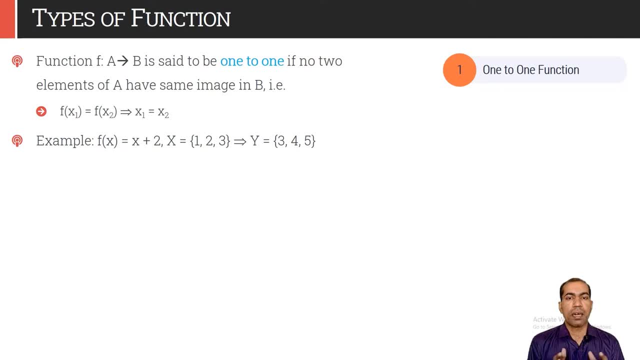 output: 5.. As we can see that x is equal to 1 to 3, set is associated with. y is equal to 3, 4, 5.. No two elements of a have same image in b, So that is why we are calculating y from a to b. 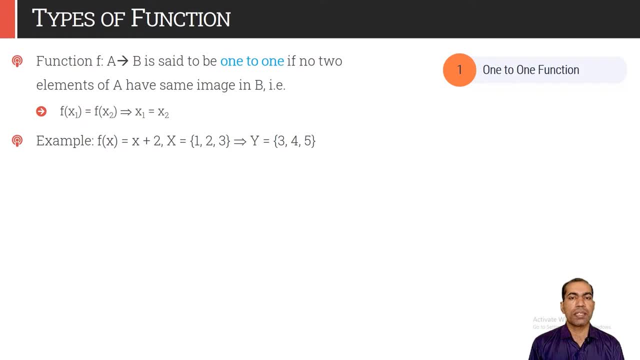 So elements in x have identical image in y, and that is why this is one to one function, And this is true for all the x. Such functions are also referred as injective functions, So another name of this function is injective function. Let us have a look at some examples. This is not a 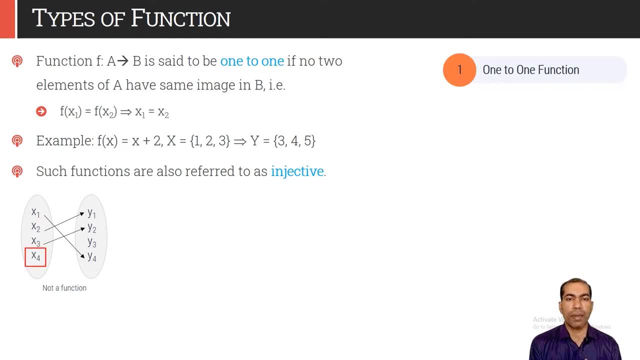 function at all, because element x4 from x is not connected with any element in set y, So this is not a function. This is also not a function because now x4 is connected with any element in set y, So this is also not a function, because now x4 is connected with any element in set y, So this is. 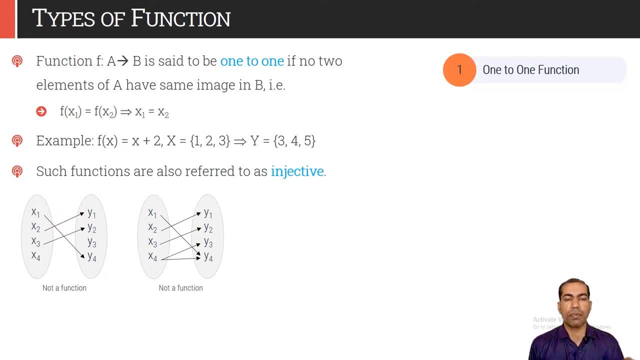 having a multiple connection. So that is not possible, that you will put one element into function and it will generate two different answer. That is not possible. This is function because all the elements of x are connected and they have a unique arrow or unique association. 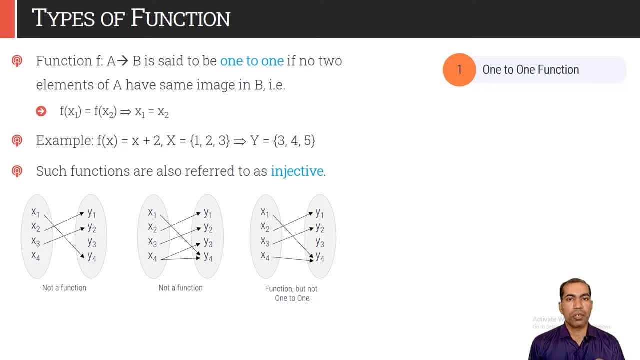 However, it is not one to one function, because x1 and x4 elements are associated with y4, but x1 and x4 are not same. That is, f of x1 is equal to 1 to 3.. So this is not a function. So this is. 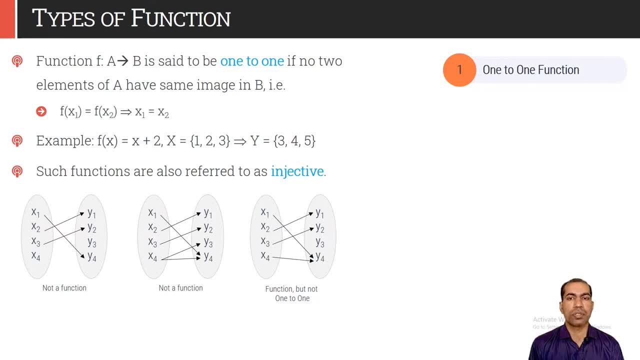 f of x4, but x1 and x4 are not same, So this is not a one to one function. This is definitely one to one function. First we will check whether it is function or not. So all the elements of x are connected with y. None of the element from x has multiple connection in y and no two elements in x. 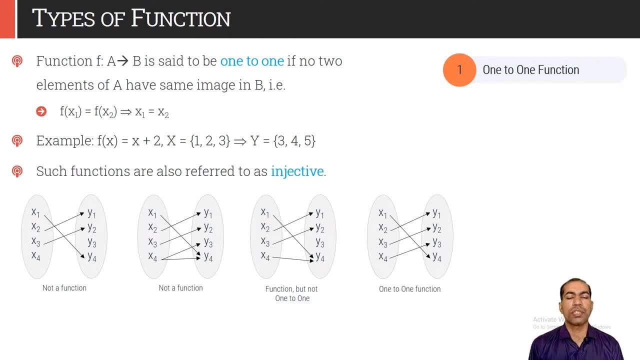 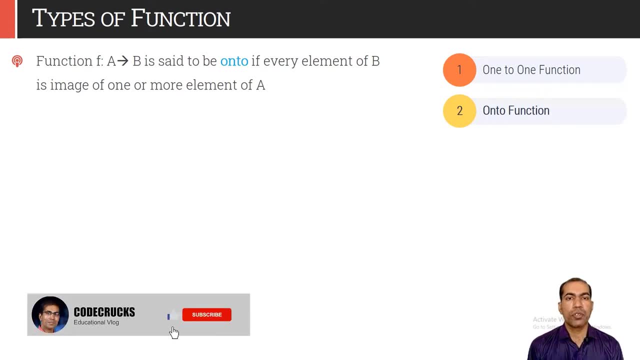 have a unique image in set y. So this is function as well as it is a one to one function. So this is function as well as it is a one to one function. A to b is said to be onto function if every element of b is image of one or more elements of a. 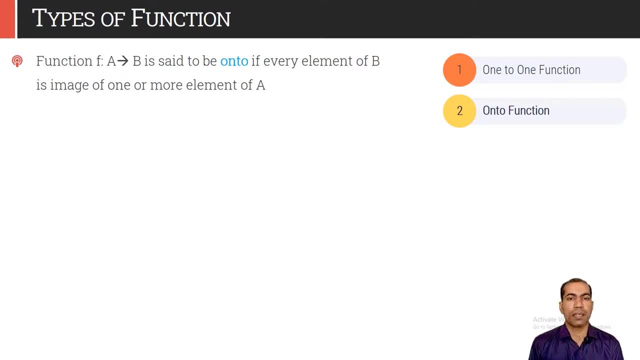 So what it says. none of the element from y should be disconnected. It must have some association with one or more variables into the set x or in the domain Onto. functions are also known as surjective function. Consider: the function f of x is equal to mode 3.. We know that when we compute. the mode of any function, we know that f of x is equal to mode 3.. So we know that f of x is equal to mode 3.. We know that when we compute the mode of any function, we know that f of x is equal to mode 3.. 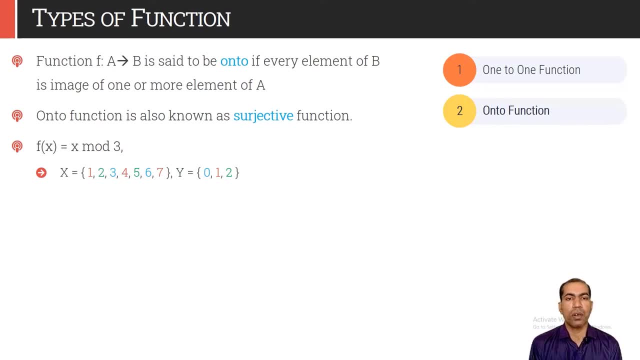 Any number with 3,, then output would be either 0 or 1 or 2.. So consider that our domain x is 1 to 7.. So when we compute 1 mode 3, that will be 1.. 2 mode 3 will be 2.. 3 mode 3 will be 0.. 4 mode 3. 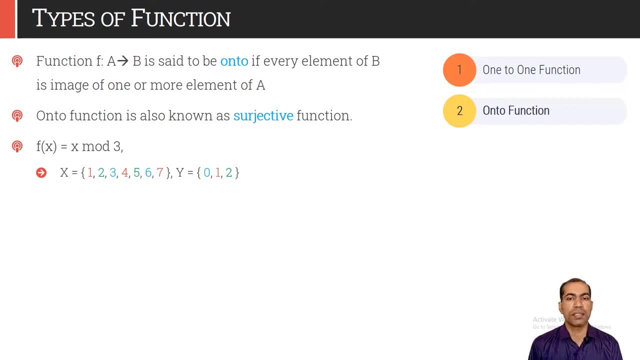 will be 1.. 5 mode 3 is 2.. 6 mode 3 is again 0. So output is always contained within 0,1 and 2.. For simplicity I have color coded the elements. The elements of the macro function are called. 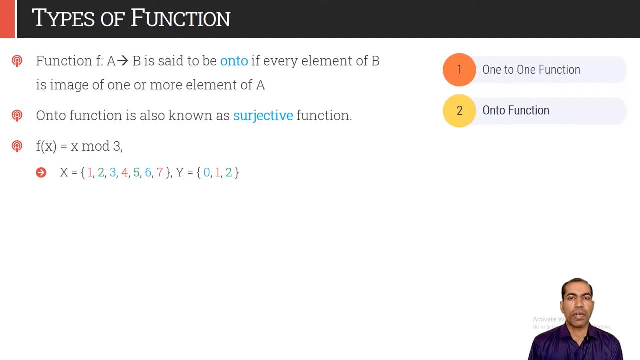 in red color in X will have output 1.. When we take modular of those numbers with 3, then it generates output 1. that is again shown in red color in Y. Similarly, component 2 and 5 highlighted in green in X are generating mode 2 and components shown in blue color. 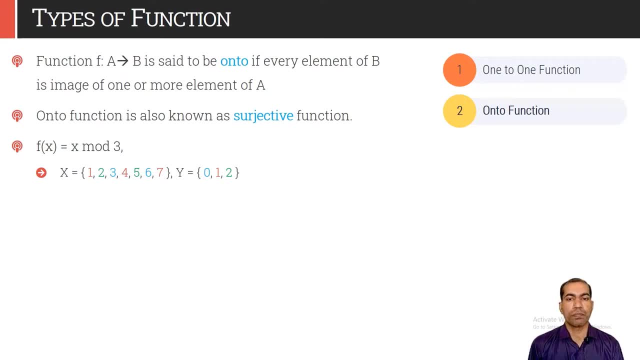 in X that is 3 and 6 will generate a mode 0. So all the elements of Y are connected with multiple elements in X. that is allowed and none of the elements from Y is skipped. all elements are having some association in X. some is connected with two elements, some. 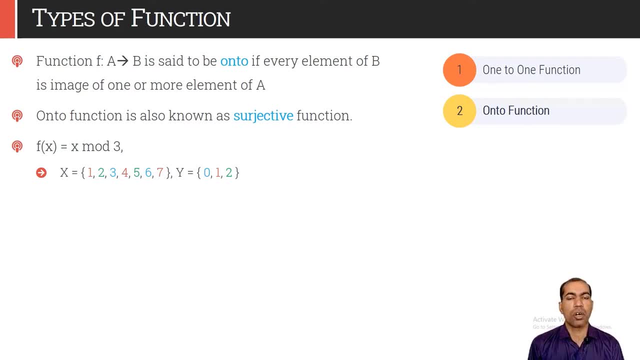 are connected with three elements in X, So this is onto function. this is valid function, but it is not onto function. by the definition we know that all element of X must be connected, connected. they are connected and there should not be multiple association from x to y and 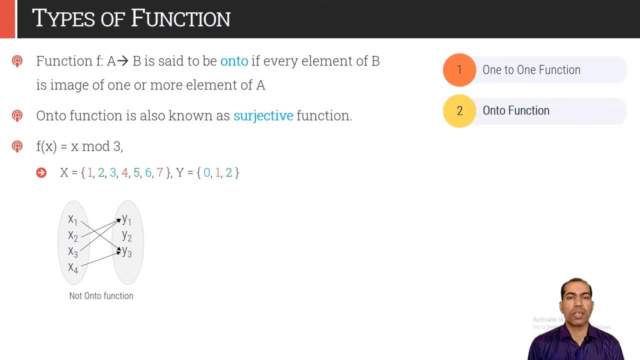 it is not there. So this is function. but this is not onto function because element y2 is not having any association with its domain, So this is not onto function. This is onto function because all the elements of y are connected with x. It is allowed that one element of y may be connected with multiple elements of x. 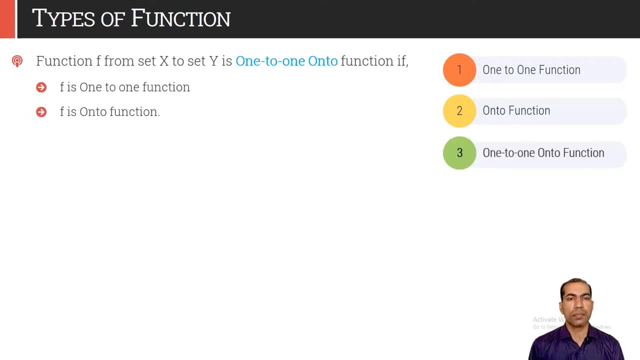 So this is an example of onto function. Function is said to be 1 to 1 if it is both, that is, if it is, it should be 1 to 1 as well, it should be onto functions. Such functions are called 1 to 1 onto function, and such functions are popularly known as. 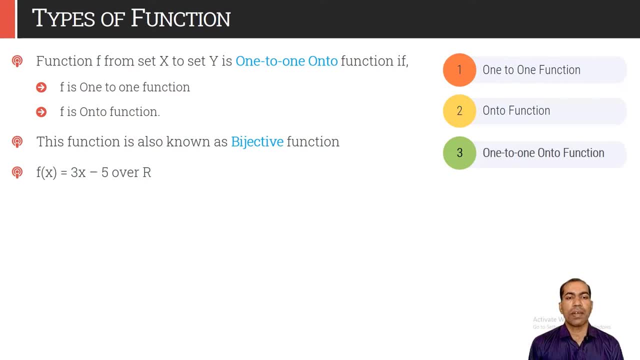 bijective function. Consider: the function f of x is equal to 3x minus 5 over the set R. So by putting different values of x We can always verify That it is 1 to 1 function also, as well as it is onto function also. 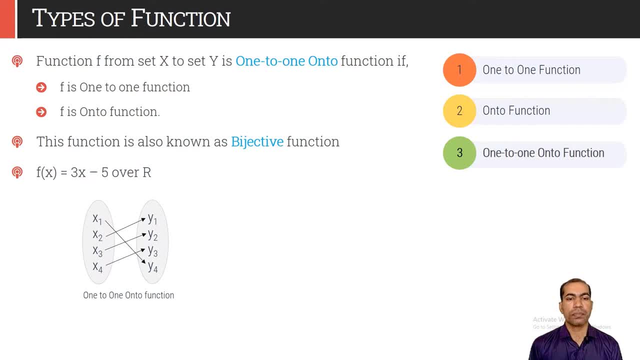 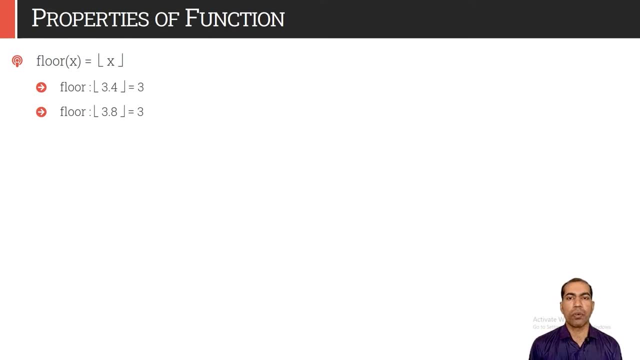 So ultimately this function is bijective function. This function is 1 to 1, as well as onto function. will discuss some of the popular functions like a floor, ceiling and round the floor of the variable x is represented by this notation. floor function will always return integer less than or equal to given number. 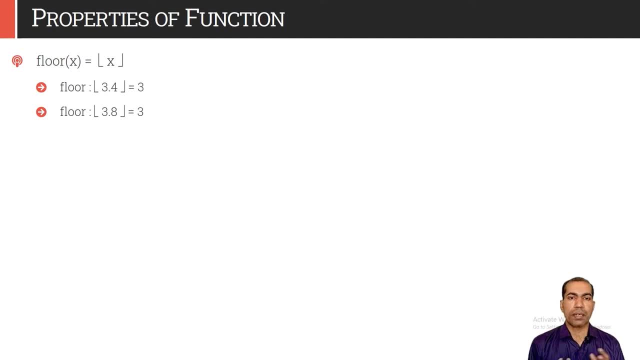 So if we compute floor of 3.4. That would be 3 and floor of 3.8. That would also be 3, because it will always find integer which is less than or equal to given number. Sale function will always compute or it will always return integer greater than or equal. 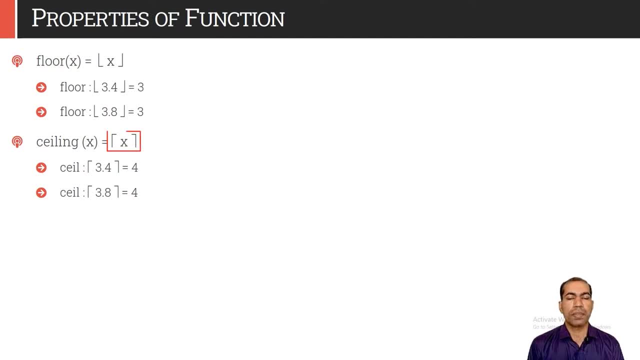 to given number and the ceiling operation is represented by this notation. So sale of 3.4 will be the next higher integer, that is, 4. similarly, sale of 3.8 will also be 4.. However, round function will return the nearest possible integer on either side. 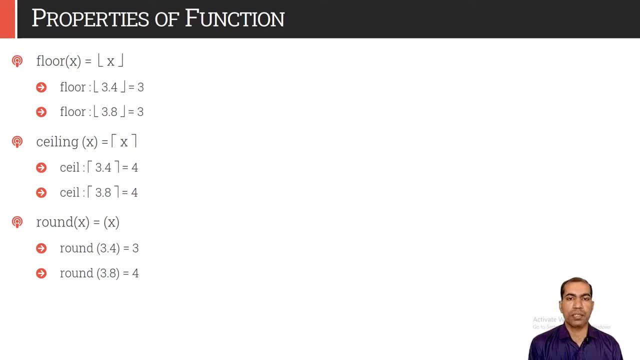 So round of 3.4 would be 3 because 3 is the nearest to 3.4, and round of 3.8 will be 4 because 4 is near to 3.8. floor and ceiling returns always one value, irrespective of what is the. 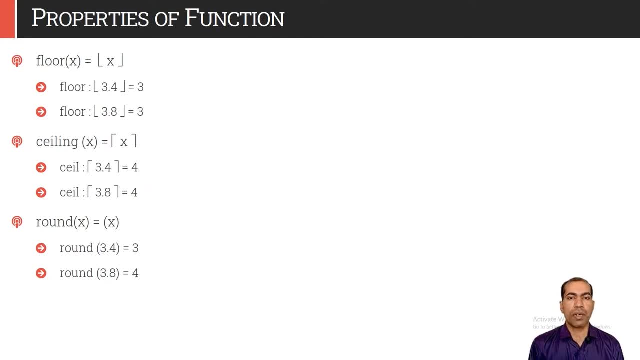 decimal value. But in case of round, if decimal value is greater than or equal to point 5, it will return next higher integer value and if it is less than 0.5, then it will return the previous integer value. For any variable x. this condition would be always satisfied. x minus y is less than floor. 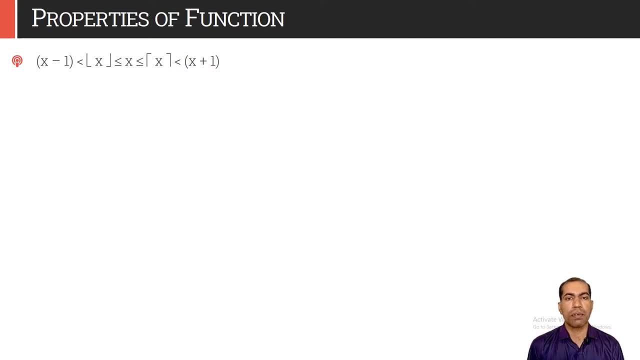 of x, which is less than or equal to number itself. again, it is less than or equal to sale of x, and it is less than x plus 1.. Now x could take any value. it may be integer or it may be any real number. So assume that x is equal to 3.4. so floor of this number would be definitely 3 and ceiling 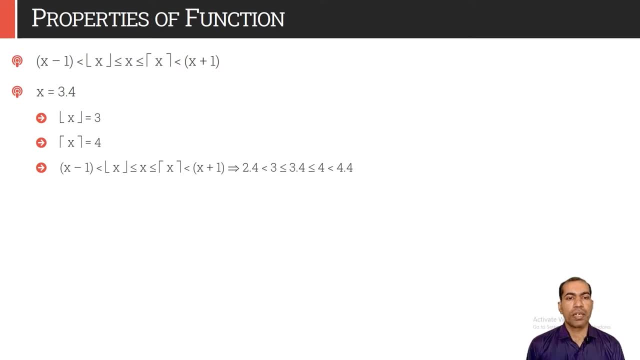 of that would be 4.. If you put these values in the given equation, then it would look like 2.4. less than 3, less than or equal to 3.4, less than or equal to 4, less than 4.4.. 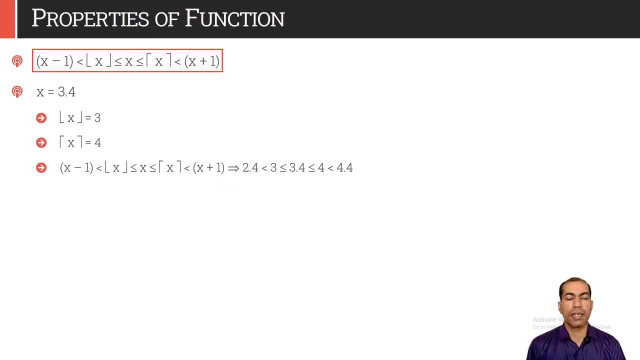 So, as you can see that this condition or this inequality is being satisfied, The another property is that for any integer number- x, Now x must be integer, Now x must be integer. If you take floor of x by 2 plus ceiling of x by 2, it will always return you the x. 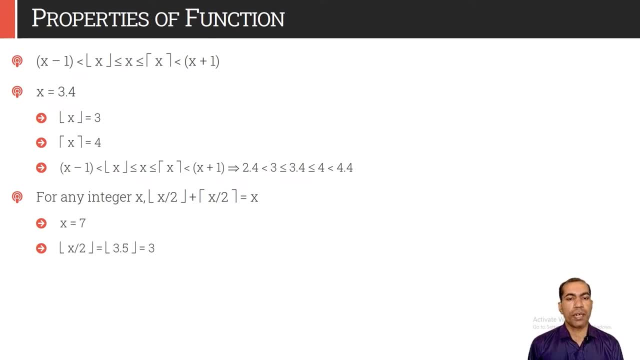 Consider x is equal to 7, its floor of x by 2, that is floor of 3.5, would be 3 and the ceiling of that would be 4.. So addition of floor of x by 2 plus ceiling of x by 2 will yield 3 plus 4 is equal to. 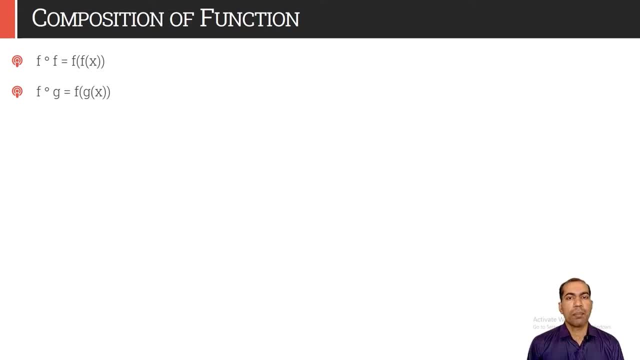 7. that is nothing, but it's a x Composition of function, That is function as an argument of another function, And composition is represented by this circle. notation F composition f is given as f of f of x, and f composition g is written as f of g of x. 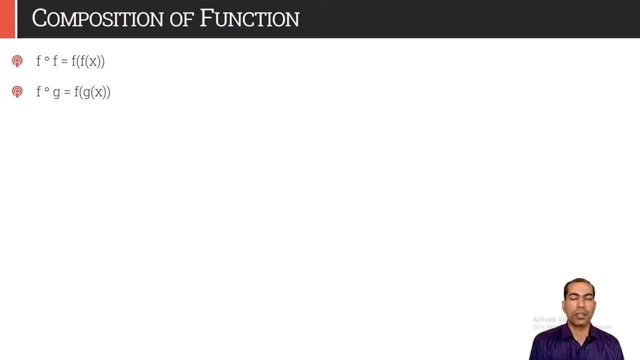 So this second function we are passing as an argument to the first function And that will form the composition. Consider that we are given two functions: f of x is equal to x square and g of x is equal to x cube. Let us find out various compositions of these functions. 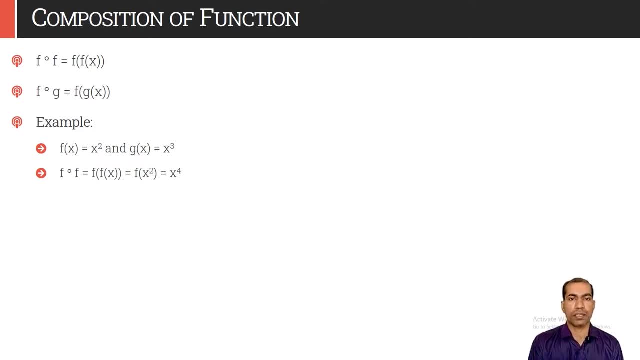 So f composition, f as we know, it is given as f of f of x, and f of x is x square. So now our function f will take x square as an argument. So when we execute it, f of x itself is x square. So x is replaced by x square and hence it would be x raise to 4.. 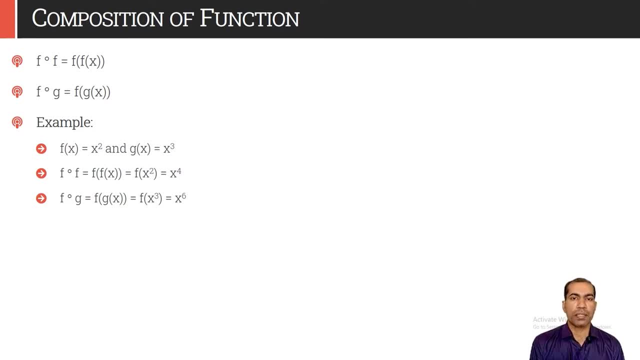 f, composition g, that would be f of g of x. So argument of f would be now g function, that is x cube, and function f is what x square. So it will simply take the square of this input argument: x cube. So that would be x raise to 6.. 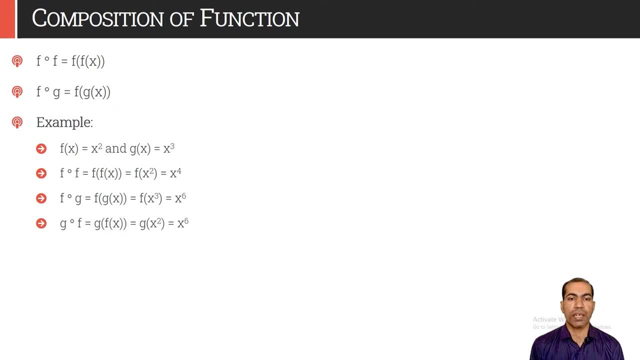 Same is true for g composition f. that would be g of f of x. Now we are passing f as argument to g. f of x is x square, So this would be g of x square and function g is simply computing cube of the input argument. 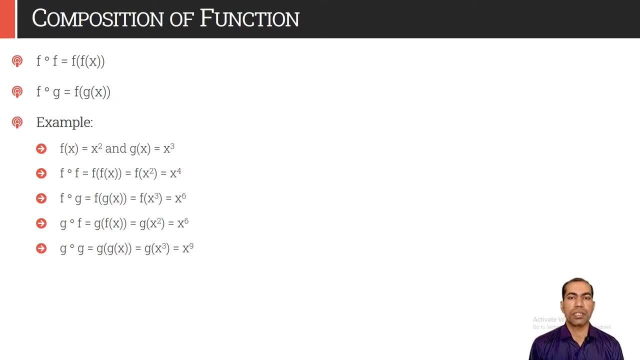 So that would be x, g, composition g. so we are passing function g as argument to g itself. So this function would look like g of g of x. by replacing the inner values, function would become g of x cube. We know that function g is simply again computing the cube of the input argument. 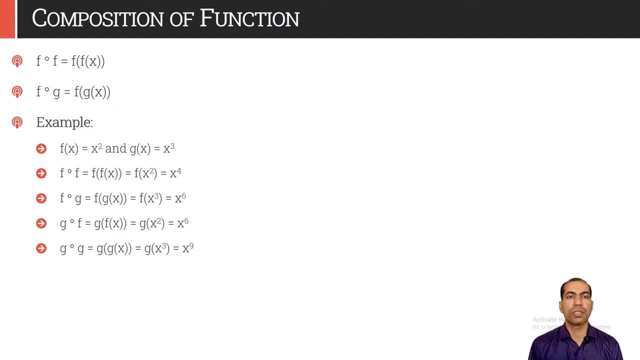 So x cube will become now x raise to 9.. So this is how we can compute the composition. Let us take one more example, where f of x is x square plus 9 and g of x is equal to 4x plus 5.. 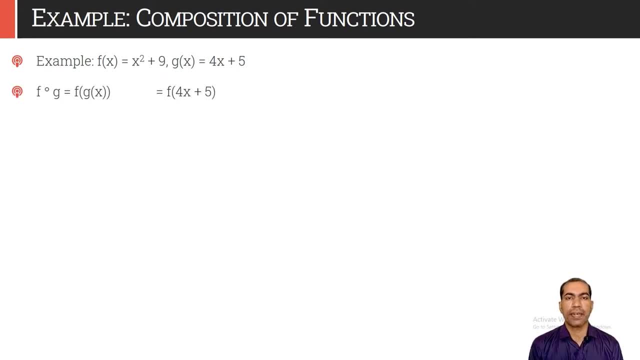 So first we will compute the composition of f with g. that would be f of g of x. So function g of x is passed as an input argument to function f, so it would be f of 4x plus 5.. We know that function f is squaring the x and adding 9 into that. 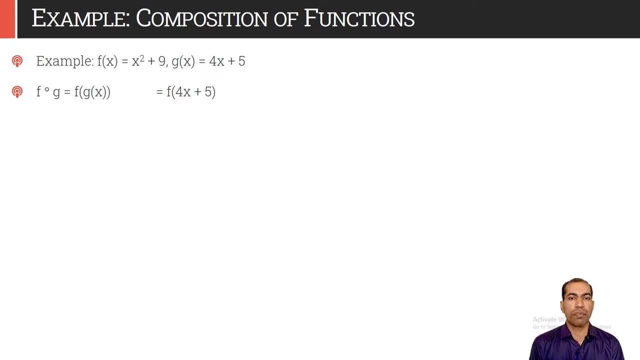 So by putting or by replacing 4x plus 5 into the x square plus 9, we will get 4x plus 5, whole square plus 9.. Let us simplify this. So this would be 16x square plus 40x plus 25 plus 9 and ultimately it would be 16x square. 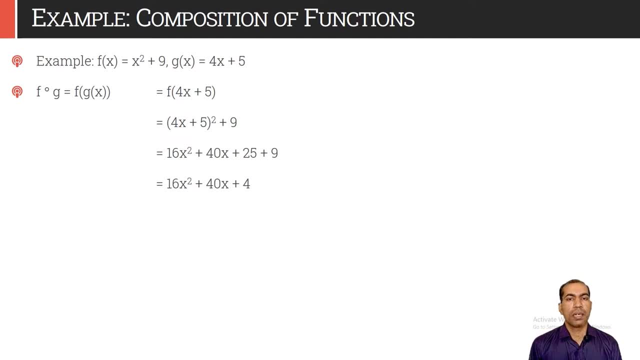 plus 40x plus 4.. Let us compute g composition f, that is g of f of x. So now we are passing function f as an argument to function g. That would look like g of x square plus 9, and by looking at the definition of function, 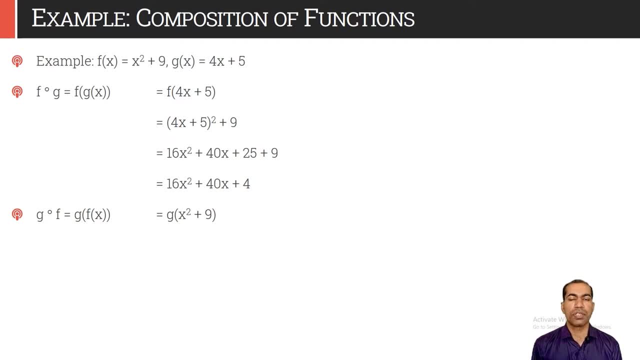 g of x. We know that Whatever argument g takes, it will simply multiply it by 4 and it will add 5 into that. So this will be converted as 4 into x square plus 9 plus 5. and let us simplify this. 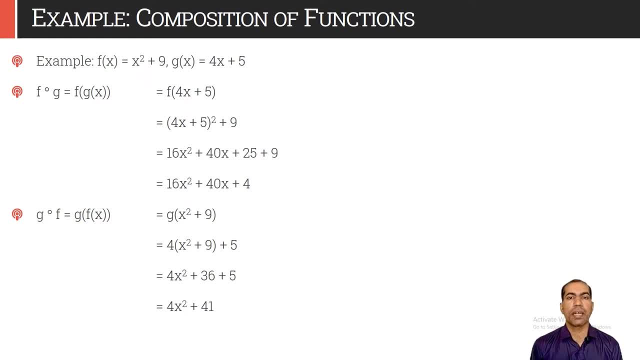 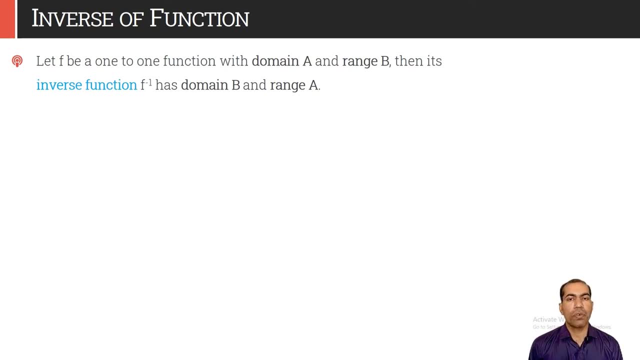 So this would be 4x square plus 41.. So this is how we can compute the compositions of the functions. Inverse of the function. Let f be a one to one function with domain a and range b, then its inverse function, which is represented by f of inverse. 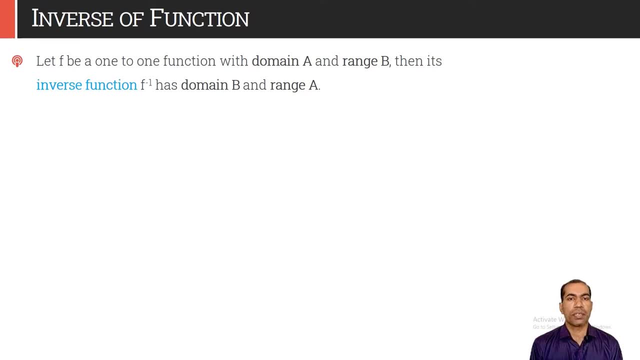 This f of inverse will have domain b and range a. So whatever was the domain will become range and range will become domain. in case of inverse function, The inverse of the binary relation is denoted as a r inverse. So r inverse is mathematically defined as b comma a if belongs to r. 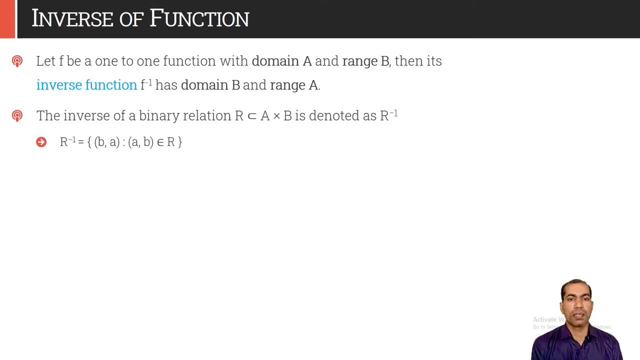 If tuple belongs to relation r, then b, a will be in the relation r into a inverse. So we are simply interchanging the role of domain and range. Normally we are writing f of x is equal to y or y is equal to f of x. When we compute the inverse of that it would be written: 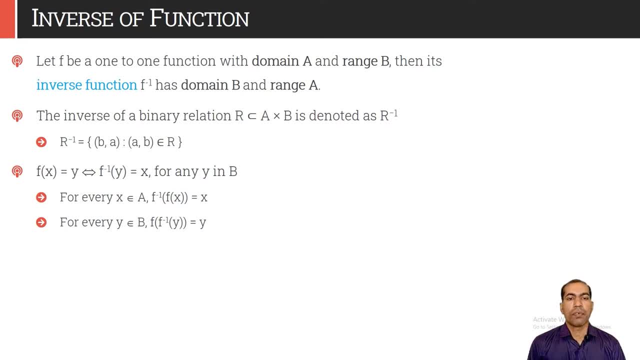 as f of f inverse of y is equal to x. For every x belongs to domain a, f inverse of f of x would be x itself. and for every y belongs to b, f of f inverse of y would be b. So that's a tautology. 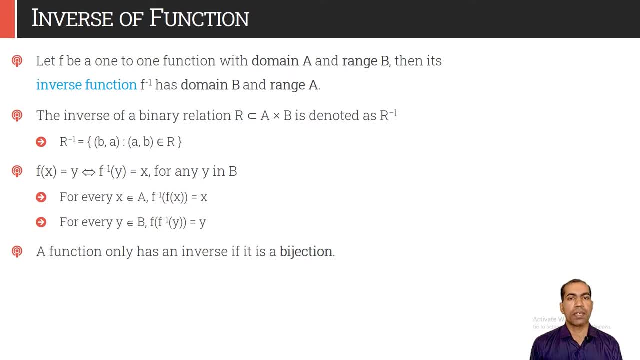 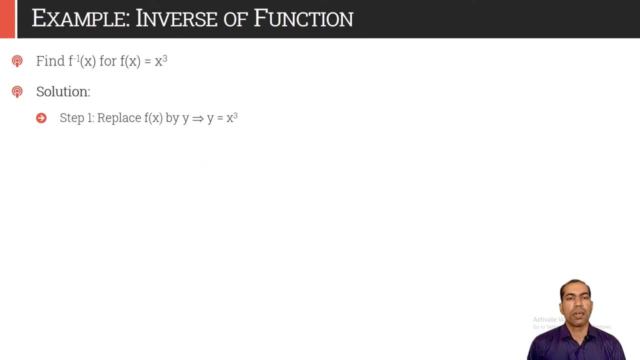 that's very obvious, and a function only has a inverse if it is a bijective function. Otherwise you may get, or you may not get, the inverse of the function. Let us see the examples. Compute inverse of function x. f of x is equal to x cube. So what we have to do is we have to. 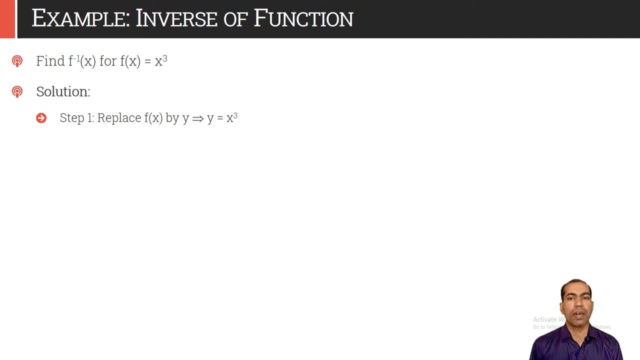 replace f of x by y, So our function would look like y is equal to x cube. In second step we have to solve this function For x, So y is equal to x cube would become x is equal to cube root of y And as we know that, 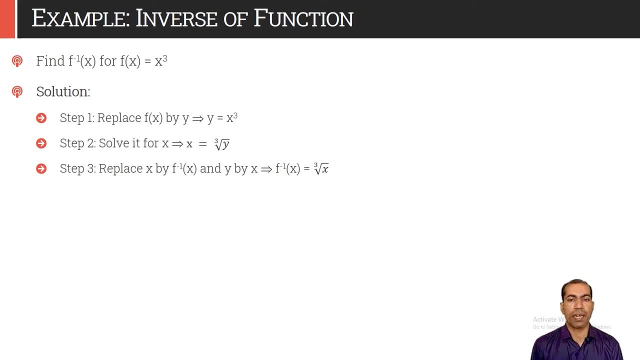 now we have to replace x by f inverse of x and y by x, So that domain will become range and range is represented by domain. So the f inverse of x would be cube root of x. Let us take one more example. We have to find the inverse of function f of x is equal to x plus 1 by x. So the first 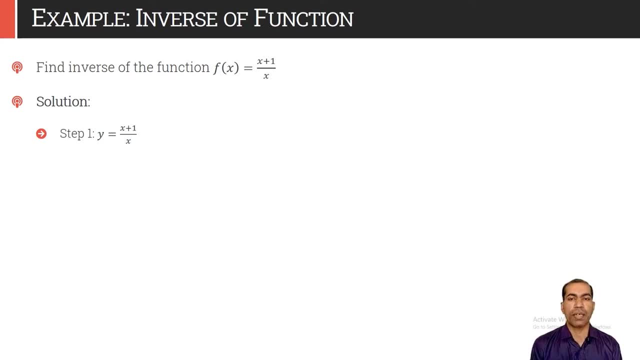 step is that we have to write down. it is in form of Y, So f of x is replaced by y, So y is equal to f of x plus 1 by x. We have to solve it for x. So we will take the x in denominator on left hand side. So x, y would be x plus 1.. We will take x on. 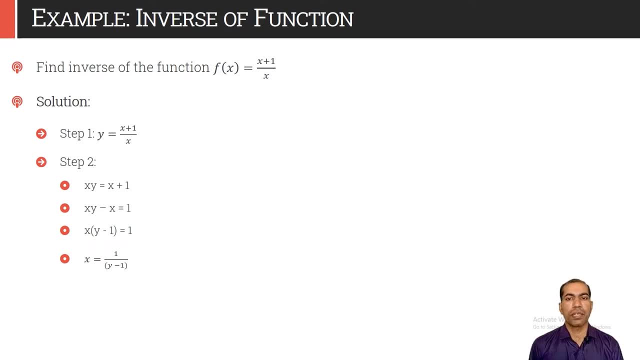 left hand side, and we will take x common And finally we will compute it in terms of x. So now it is x is equal to 1 by y minus 1.. And finally, to compute the inverse, we have to replace x by f, inverse of x, and y by x. 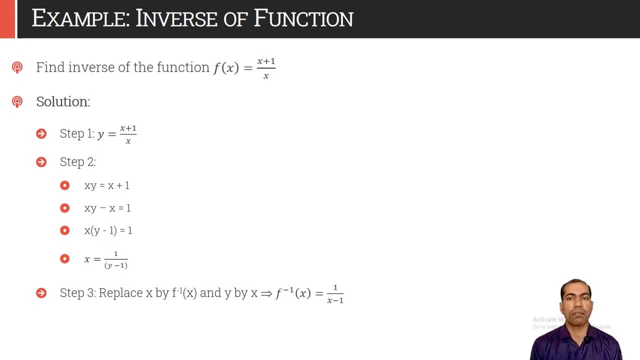 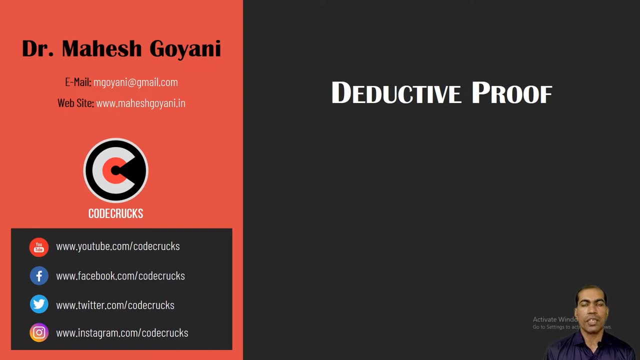 So the inverse of function x would be f. inverse of x is equal to 1 upon x minus 1.. Hello folks, Welcome to Code Crux. This is Mahesh Guyaani and in this video I'll be talking about deductive proof. Reasoning is the process of inferring something from the given statement. 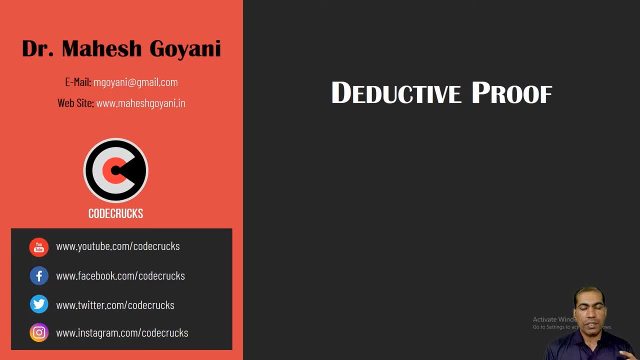 So if statement is given by some logical steps, we are coming to some conclusion. So the derivation- we are coming, we are reaching to some conclusion- is known as a proof or the reasoning process. there are two reasoning approaches: inductive approach as well as detective approach. in this, 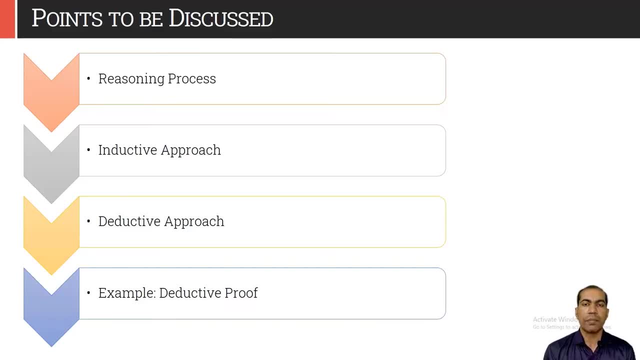 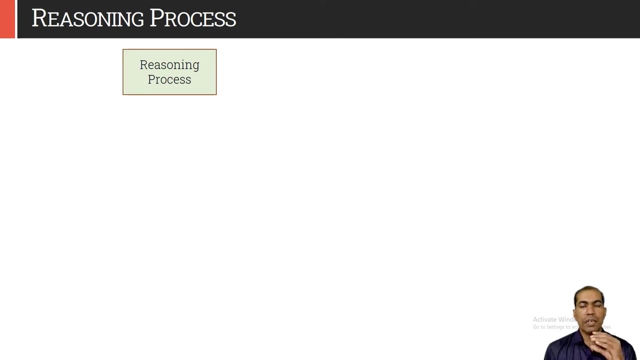 video. basically, i will be targeting what is the reasoning process, what are the different approaches for that, and i'll be discussing detective proof with the help of examples. as discussed, reasoning process will start with some assumption and it will try to prove it. so there are two different approaches. you can consider it as a bottom-up or the top-down. 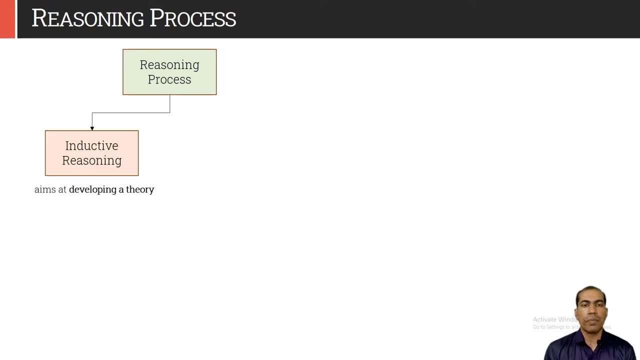 approach, or the forward or the backward approach. so the first approach is known as an inductive reasoning, in which we are aiming to develop some theory. so first we are observing some data and from that data we are finding the patterns, and from pattern we are trying to generalize it. 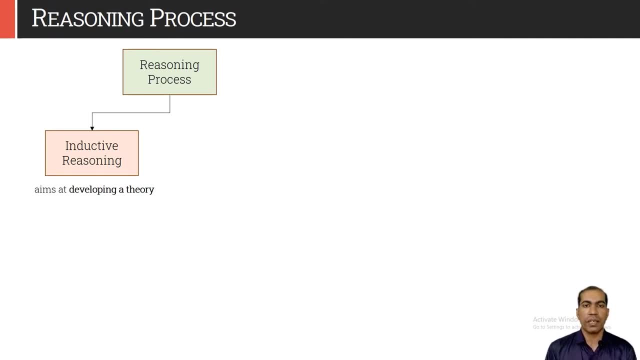 so we are moving from specific case to the general case, so we are developing the theory into that, whereas in case of deductive reasoning process we are doing the exactly reverse thing. we are trying to test the existing theory and we will check whether that theory what we were claiming. 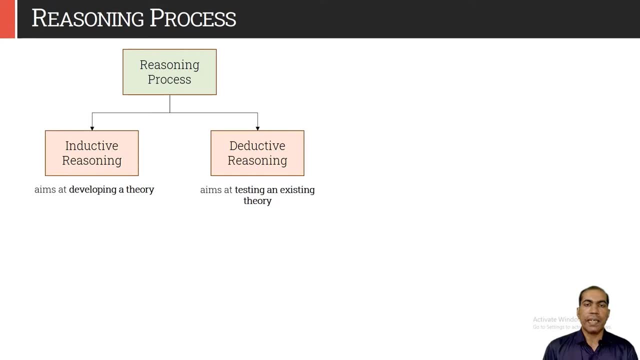 is true or not. so it takes exactly reverse steps compared to the inductive reasoning process. so in case of inductive reasoning we have a specific case and by observations we are trying to develop a general case for that. that is what inductive reasoning? whereas in case 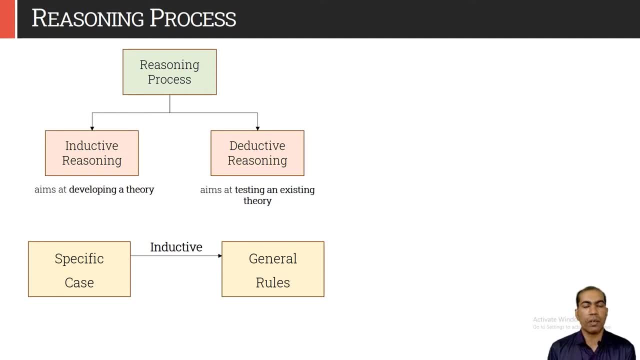 of deductive reasoning. we already have some developed theory or we already have generalized case and we are trying to narrow down it and we are going to the specific things and we will check whether it is true for given specific value or not. so they are totally contradictory ways of 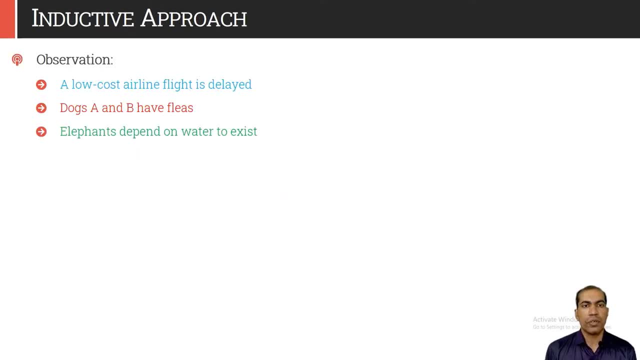 proving the same thing. let us try to understand what inductive approach with the help of this example. so in inductive approach we have first very little data, or we can say that we have just an observation of one or two samples. a low cost airline flight is delayed, so we have observed that. 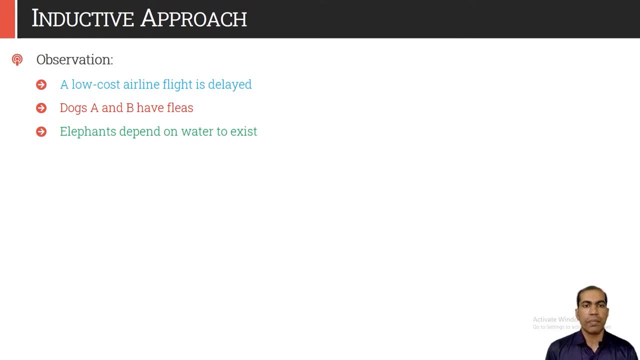 one low cost airline flight is delayed. we have also seen that dog a and b having fleas. so we have observed two dogs and we have also observed supposed elephants depends on water to exist. so these three are our observations and they are not very much generalized, they are very specific to one flight, two dog and an. 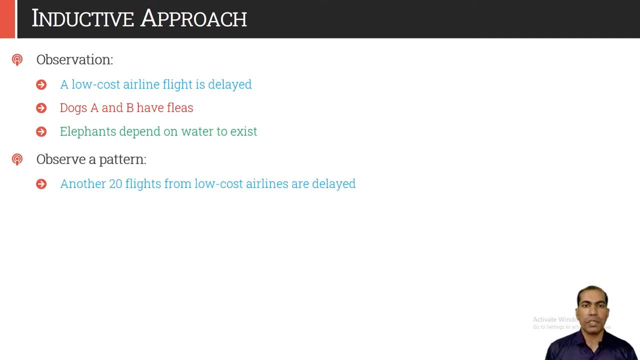 elephant from this specific observation. we will try to check whether this pattern is repeating or not, whether it was just an incident or it is actually happening. and after observing, we really we realize that another 20 flights from low cost airlines are delayed. so initially the observation was for one flight only. now we have looked at the two flights and we have seen that the two flights 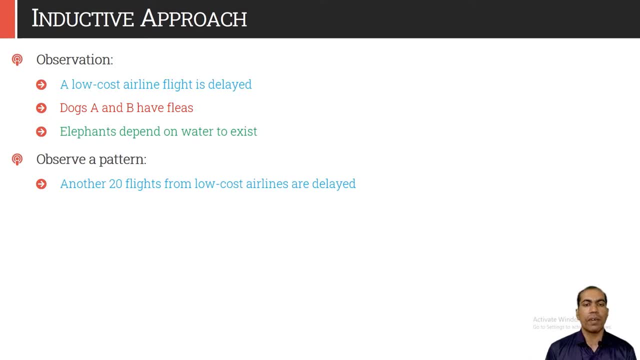 are delayed. we have also observed that all observed dogs have fleas. so we might be observing dogs in our colony, maybe in our society, maybe in our city, etc. and we found out that, okay, whatever dogs we have observed, they have fleas. and we have also observed that all animals, not only just 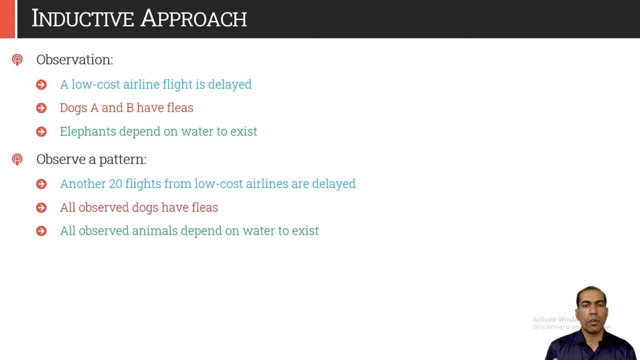 elephant, but maybe cow, buffalo, got dog and we have also observed that all dogs have fleas. and we have also observed that all dogs, cats, all animal depends on water to exist. so from this pattern, now we will generalize our observation that low-cost airlines always have delays. so this is the theory that if your airline is of 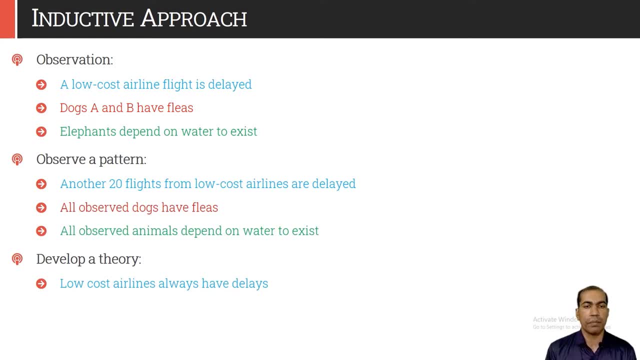 low cost, then it is going to be delayed every time. all dogs have fleas. so initially have our observation for two dogs, only then we observed in specific region, and from that we come to the conclusion that all the dogs are having fleas. And for the third statement we conclude that all biological life, not only elephant, not only just animals we have observed, but all the biological life depends on water to exist. 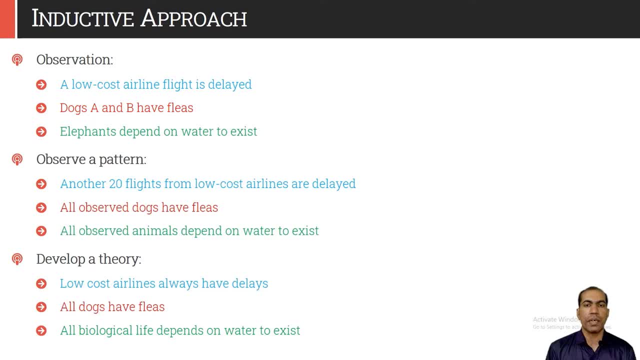 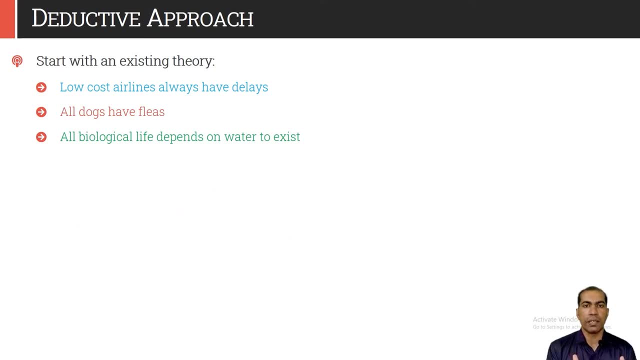 So, that is, we have moved from observation to the exact theory. In deductive approach the things go exactly in reverse order. We start with the theory. So these three statements we have derived into the last step of inductive approach. like low cost, airlines always delays, all dogs have fleas and all biological life depends on water to exist. 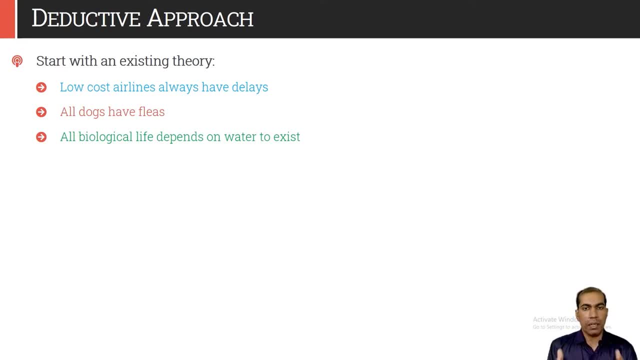 Now, deductive approach will try to minimize the scope of this and it will try to check whether it is true for each and every specific instance or not. So first we need to formulate hypothesis, in this case The hypothesis for the first statement. 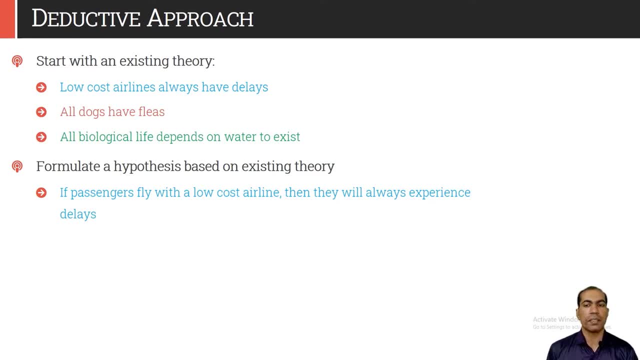 The first statement would be like: if passengers fly with low cost airline, then they will always experience delays. This is what our hypothesis. So we need to prove whether this hypothesis is true or not. Similarly, we can develop hypothesis for all dogs have fleas and all biological lives depends on water to exist, as shown. 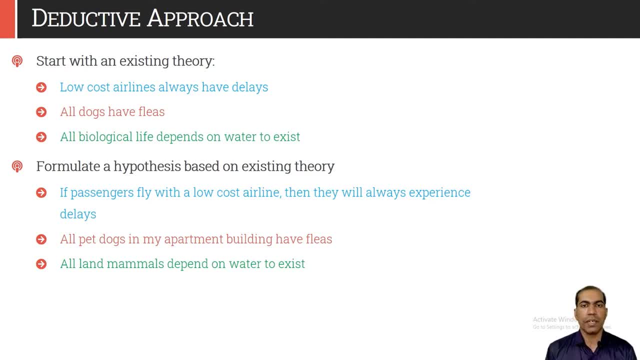 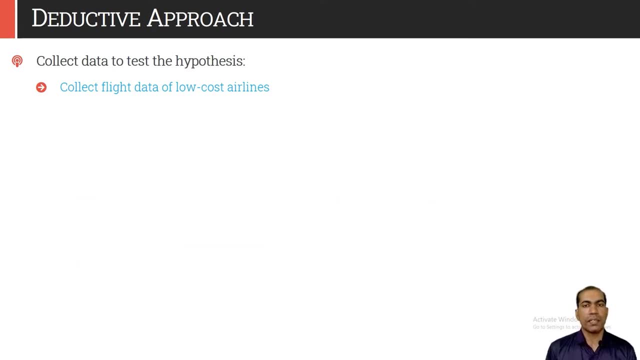 Now, to prove this hypothesis, we need some data, We need some statistical support for that. So we will collect the data. So assume that we have collected Fly Data of low cost airlines, because right now we are talking only about the flights of low cost. 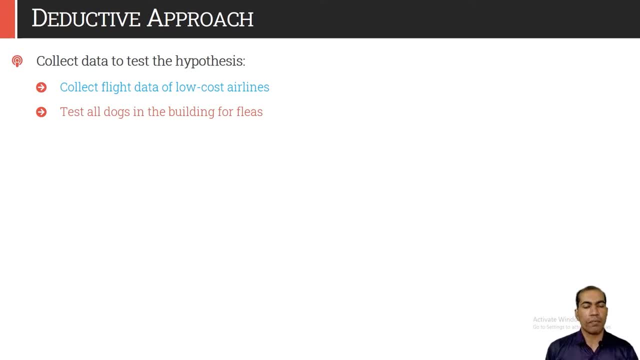 Then we test all the dogs in the building for the fleas. So we have reduced the scope of dog from universe to building only, and we study all the land mammals to see whether that depends on water or not. So instead of all the biological entities, we have reduced our scope to just land mammals. 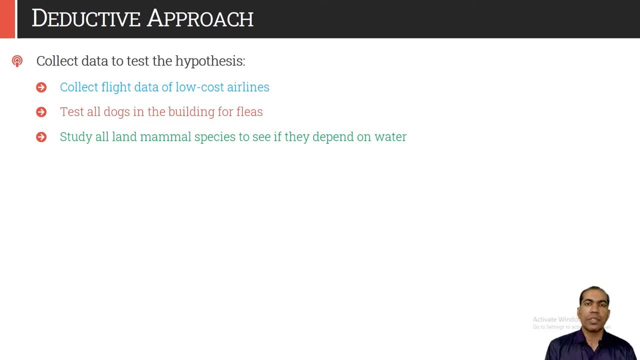 We will collect the data And we will check whether our hypothesis is true for collected data or not And based on that, either we will accept it or we will reject it and assume that five out of 100 flights which we have observed or for which we have collected the data of low cost airlines are not delayed. 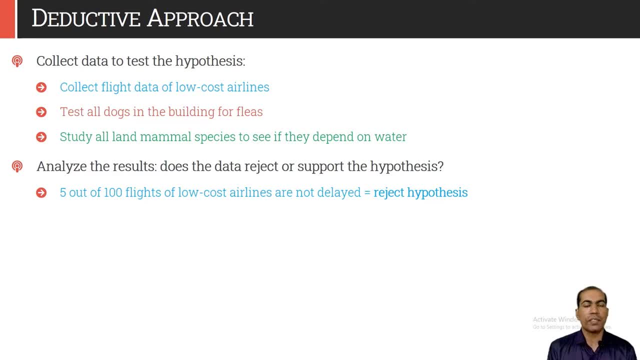 What was our hypothesis? that if flight is of low cost then it will be delayed. but out of 100, the statement or the hypothesis is true only for the flight. So we are rejecting our hypothesis. It means that is not true. As of that. we have tested the 20 dogs and out of 10 dogs didn't have fleas. 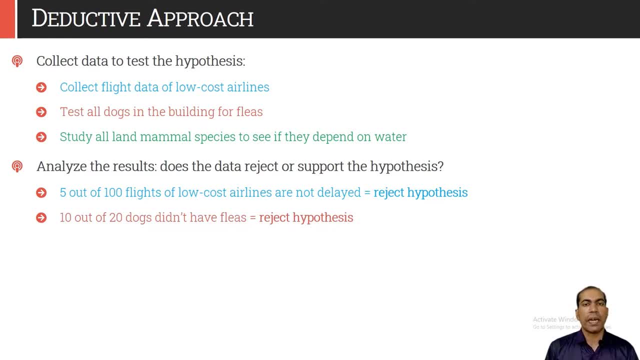 So only 50% data supports our hypothesis And based on just 50% data we cannot say that our hypothesis is always going to be true. So in this case also, we are rejecting our hypothesis. It means our claim was wrong. 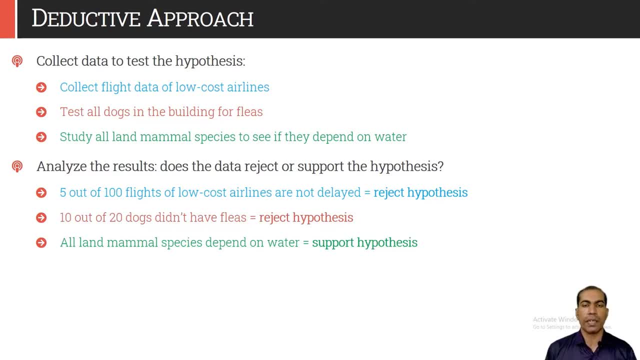 All land, mammals, Spaces, depends on water. That's proved, Okay, That is always true. So, whether I'll consider 100 people or 1000 or 10,000, the statement is always going to be true And hence that particular hypothesis will be accepted. out of this, three to are rejected. 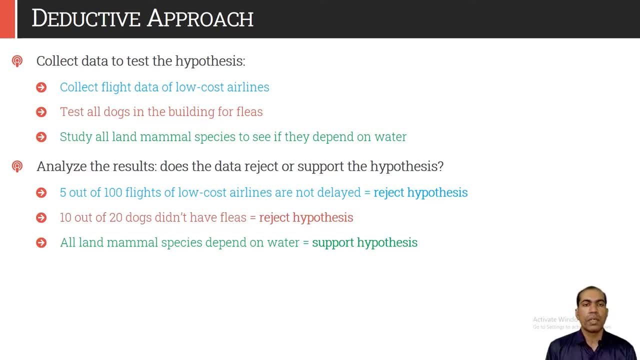 One is accepted. You should be clear by now. in inductive approach, We are starting with one observation. We are finding the patterns and we are generalizing the theory. We are coming to some specific theory. in case of deductive approach, We are starting with the theory. 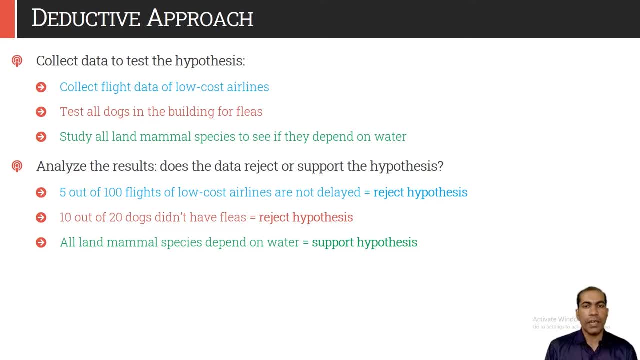 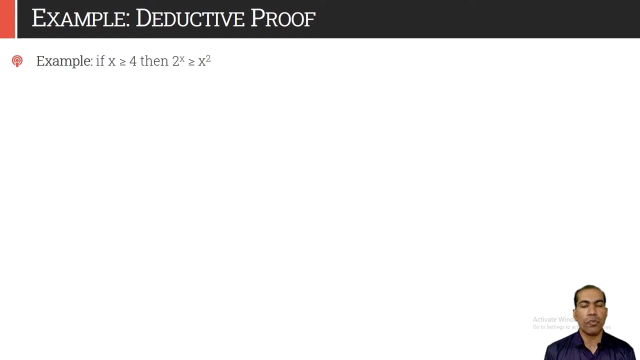 We are narrow down in the scope, We are formulating the hypothesis and, based onto the collected data, we will either accept the hypothesis or we will reject the claim. So let us try to understand how deductive proof works. It is given that if X is greater than or equal to four, then two power X is greater than or equal to X squared. 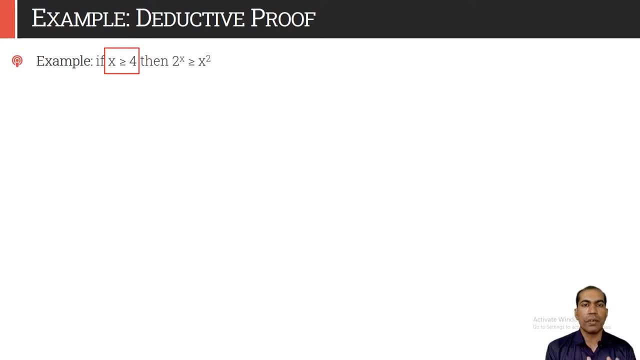 So the left hand side part formulates our hypothesis and the right hand side of this formulates the conclusion of this. If If hypothesis is true, then conclusion should also hold. Then only can say that this given claim is right or our statement is true. 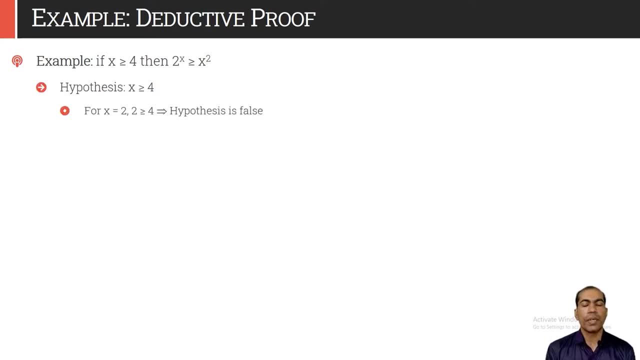 If we take X is equal to two, two greater than or equal to four, This condition is false. So our hypothesis is false for X is equal to two. For X is equal to three. also, hypothesis will be false For X is equal to four. 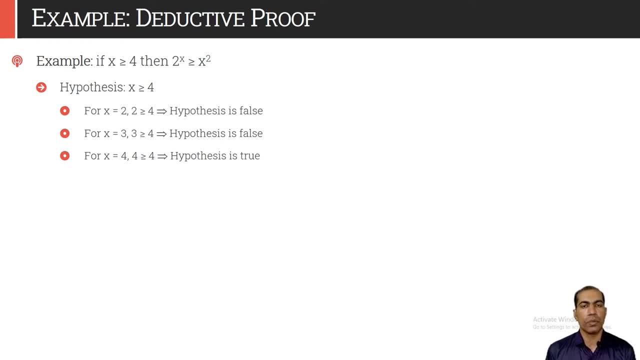 This would be true because four greater than or equal to four is true. So for that value, hypothesis is true And for any value greater than or equal to four, our hypothesis is true. So for whatever values of X, hypothesis is true. 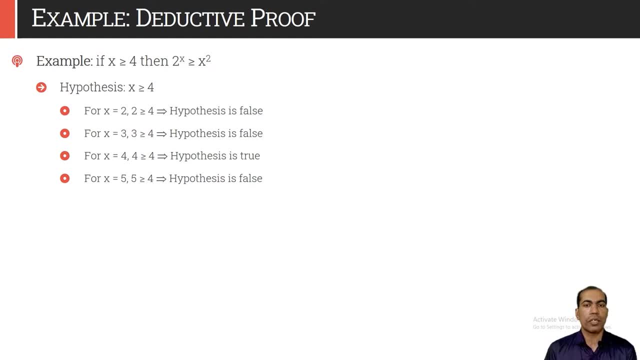 For all those values of X, our conclusion should also be true. So let us try to prove that two power X is greater than or equal to X squared, for X greater than or equal to four. So this is our conclusion: Two power X greater than or equal to X squared. 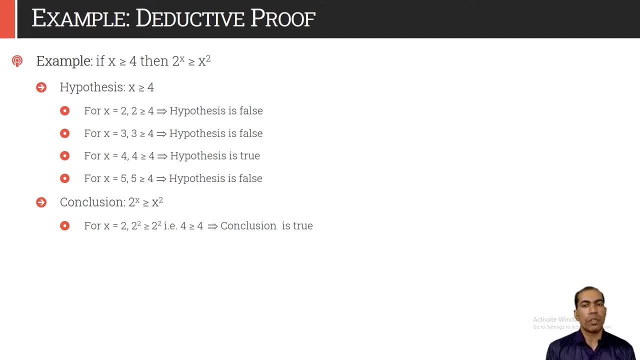 Let's consider: X is equal to two, So for two our hypothesis is false, But conclusion is true because two power X greater than or equal to X squared. If we replace X by two, then simply it would be four greater than or equal to four. 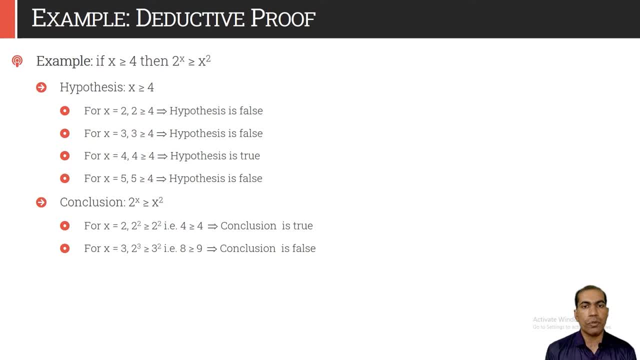 So our hypothesis is false. Conclusion is true for X is equal to three. Two power, X greater than or equal to X squared condition would be false because eight greater than or nine is not true, So conclusion is false. So you see that for some random value of hypothesis, conclusion may be true or may be false. 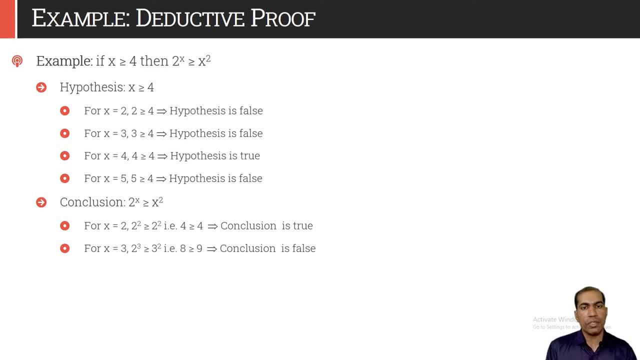 We are not worried about that. But once your hypothesis is true or it is accepted, your conclusion should always hold true. Then we can say that given statement is acceptable. So now we know that hypothesis is always true when X is greater than or equal to four. 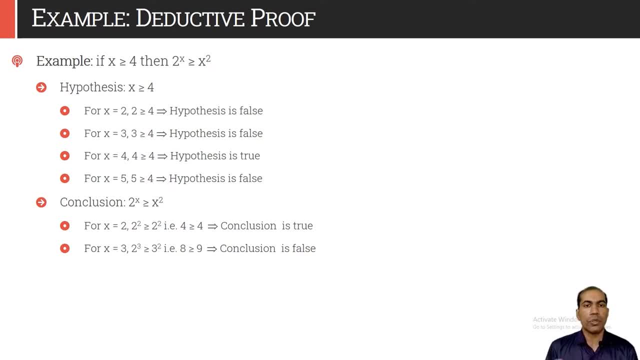 So we will make a test whether our conclusion is true for X greater than or equal to four or not. So for X is equal to four. it would be two power four greater than or equal to four squared, That is 16 greater than or equal to 16.. 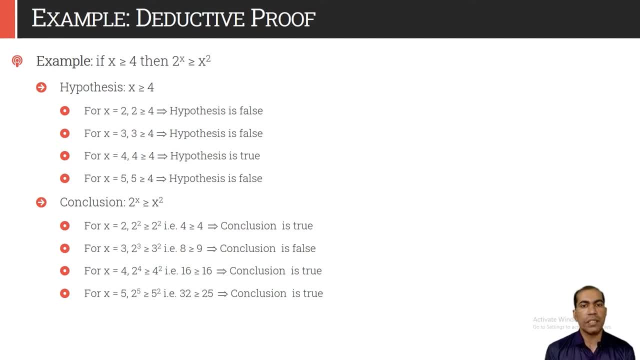 So conclusion is true for X is equal to five. It would be two power five greater than or equal to five. squared, That is 32 greater than or equal to 25.. Condition is true, So conclusion is accepted. for X is equal to six. 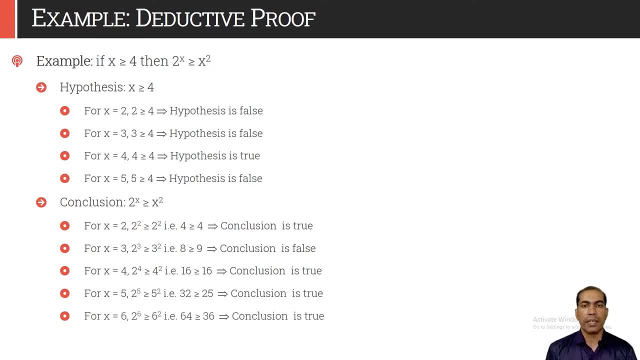 We know that our hypothesis is true And in conclusion it would be two power six greater than or equal to six squared, That is 64 greater than or equal to six greater than or equal to 36.. So conclusion is true. So now we are finding the pattern there. 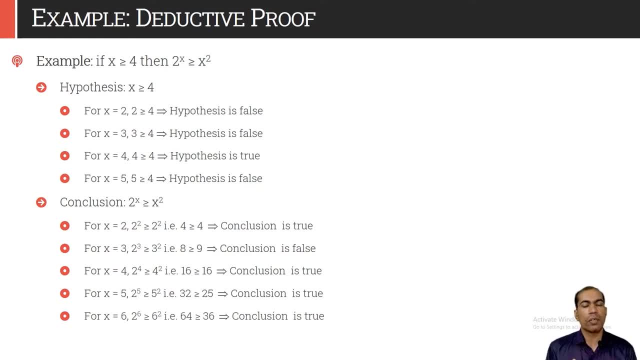 that, whatever may be the value of x now onwards conclusion is always going to remain true. If we observe carefully, when x is incremented by 1- the left hand side of the conclusion, that is, 2 power x- it is always going to be doubled. So for x is equal to 2, it was 4. for x is equal to 3 it. 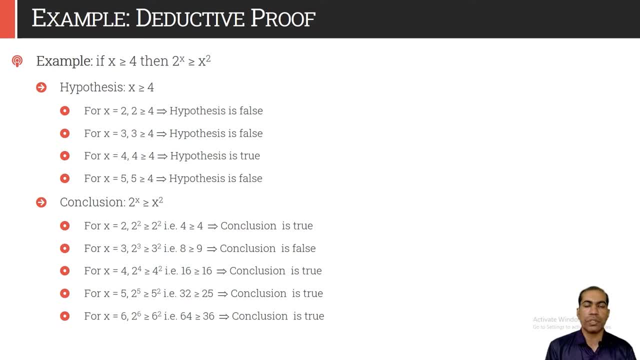 was 8, for x is equal to 4. it was 16, then 32, 64 and so on. So it is doubling with increment in x, whereas on right hand side of the conclusion is not increasing with that rate. Initially it was 4, then it is becoming 9.. So that rate is greater than 2, but after that 9 becoming 16.. So it has. 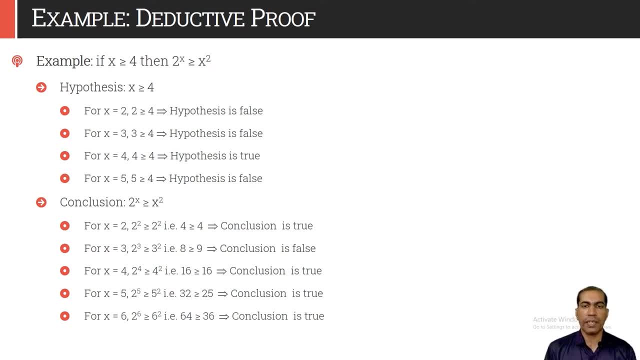 not doubled, then 16 has become 25.. So again, it has not doubled. So rate of increment on right hand side of this conclusion is always less than rate of increment on left hand side, and that's why, after 4, this condition is always going to be true, irrespective of any value of x. As x is increased by 1, the 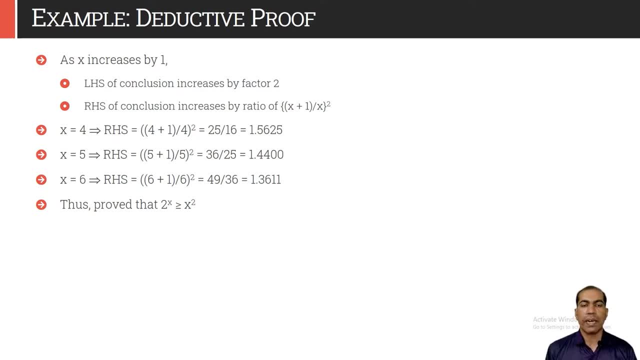 left hand side of conclusion increases by factor of 2 and right hand side of conclusion is increased by the ratio of x plus 1 upon x, whole square, which is always going to be less than 2.. Let's try to prove that x is equal to 4. then right hand side. 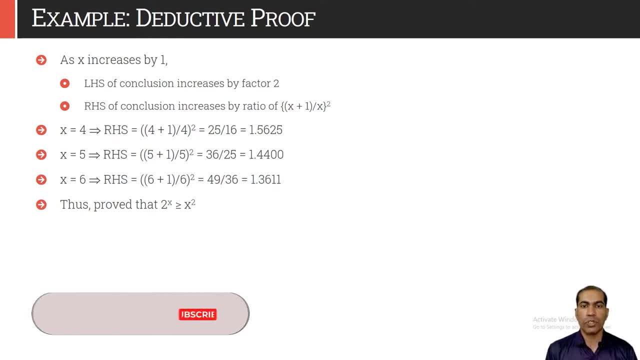 would be 4 plus 1 upon 4 whole square, that is 25 by 16.. So that ratio is 1.5625.. For x is equal to 5. the right hand side of conclusion would be 5 plus 1 divided by 5 whole square, that is 36 by 25.. 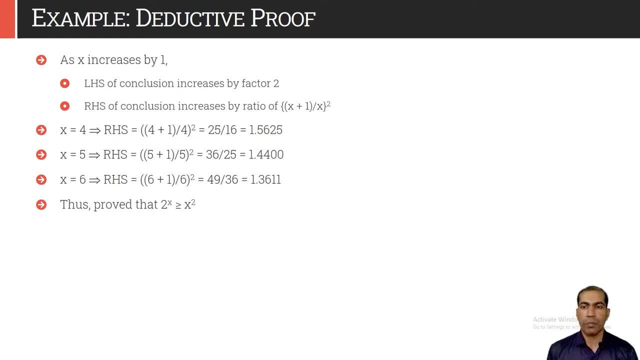 So that ratio is 1.44, then it becomes 1.36.. So, as you can see that, as x is increasing, this ratio is going down and down, down and down: 1.56 to 1.45.. 44, and from 1.44 to 1.36, and hence the left hand side of conclusion will always remain. 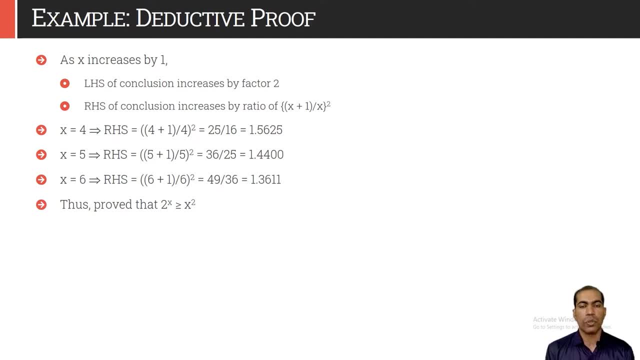 greater than or equal to the right hand side of the conclusion. So our assumption is proved, or whatever statement is given is always true that 2 raised to x is greater than or equal to x square when x is greater than or equal to 4.. 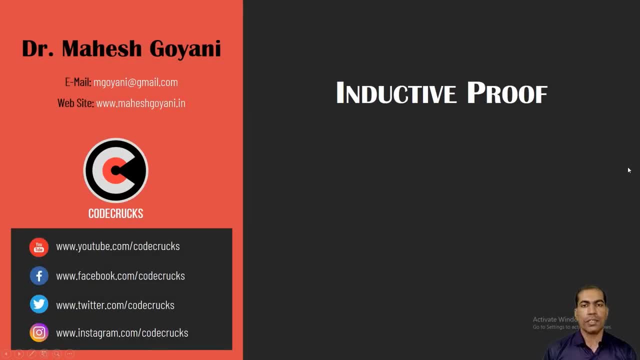 Hello folks, welcome to Code Crux. This is Mahesh Guyanee and in this video I am going to talk about inductive proof. In last video, we have talked about different reasoning approaches and we have discussed deductive proof method. In this video, we will be talking about inductive proof. As we know, 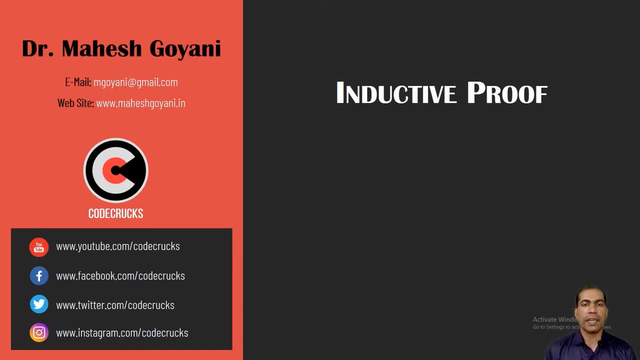 that inductive proof and deductive proof works exactly in reverse order. So inductive proof will start from specific observation and go up to the final theory, whereas deductive proof will start from the generalization and it will go up to the specific case and it will check whether the given hypothesis can. 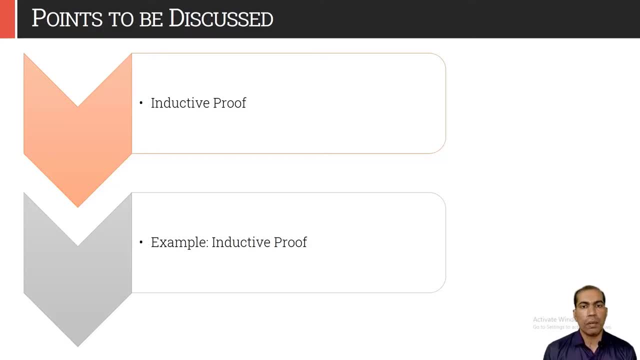 be accepted or not. So basically I will be talking about what inductive proof is. So I will recap some of the concepts we discussed in a previous video and will also discuss example of inductive proof. Reasoning means to infer something, So we are given the statement. by writing a logical steps, we can come to some conclusion. 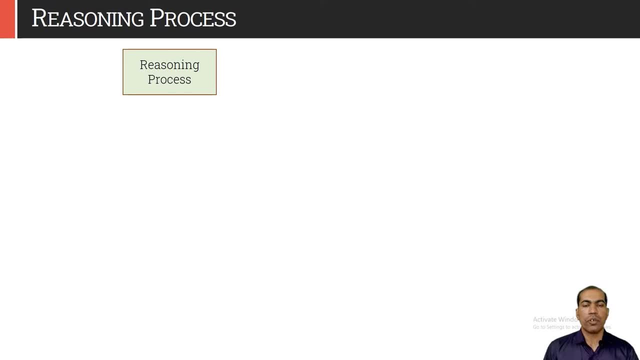 so that process is known as a reasoning process. That could be different ways for the reasoning something: in inductive way or in inductive reasoning. we are starting with the specific case and we are going to the generalized theory. So we are trying to develop some theory from the given data. 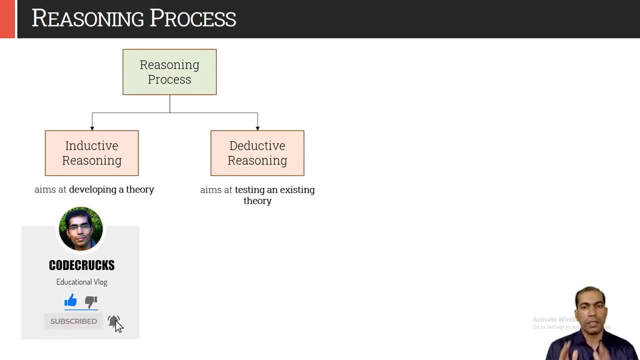 Whereas in case of deductive reasoning, theory itself is given and we are trying to prove that theory whether it is true or not. So first we are building the hypothesis and then we are testing it with the data. Inductive reasoning means specific case to generalized rule and deductive reasoning means 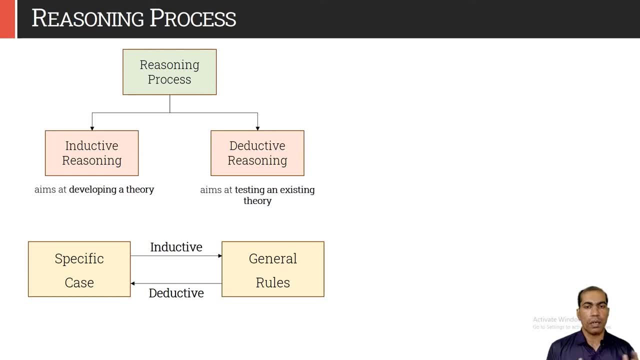 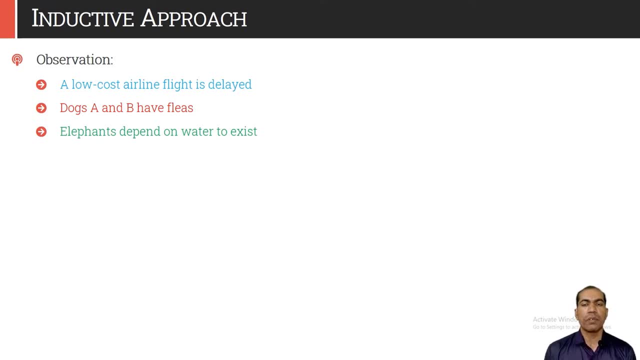 we are given the generalized rule and we are trying to make it true or false for the specific case. Let us recap: inductive approach, That in inductive approach We are always starting with the observations like: a low cost airline flight is delayed, Dogs A and B have fleas and elephants depend on water to exist. 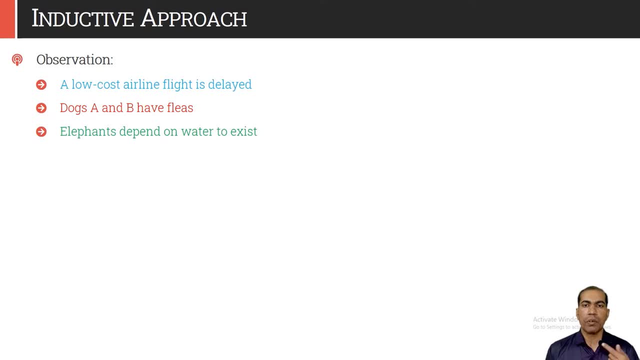 So right now we have very specific data, like we have observed only one flight and we think that a low cost airline flight is delayed, So that might be just an incident. it may or may not be true. Dog A and B- only two dogs we have observed. they might they have fleas, but it doesn't. 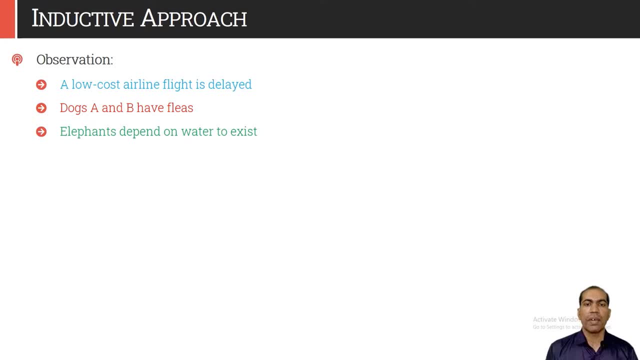 mean that all the dogs would have fleas And elephant depends on water to exist. it doesn't mean that all the animals would depend on to the water to exist. So we will check whether it is really true or not. So we will now observe the pattern, whether whatever we have observed for one incident. 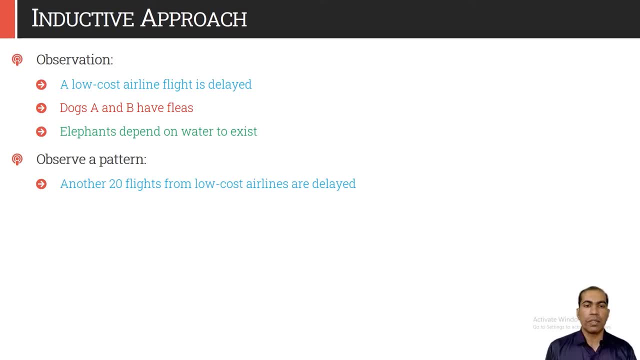 whether it is repeating or not. So we found out that another 20 flights from low cost airline are delayed. All the observed dogs have fleas. We might have observed more fleas. We might have observed more dogs, maybe in our apartment, maybe in colony, maybe in society. 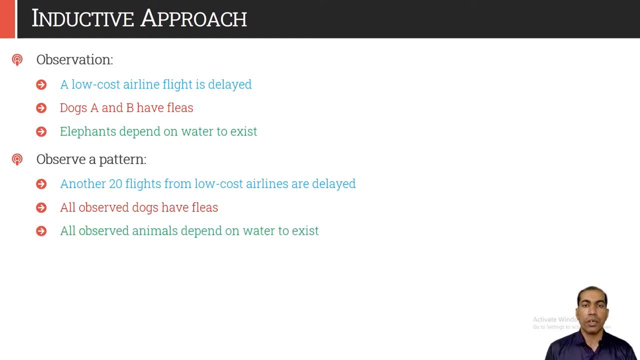 cities or anywhere, And we also observed that, not only elephant, but whatever animals we are observing around us- maybe cow, buffalo and cat, monkey, donkey, dogs- So they all depends on water to exist. So that was the pattern. it was repeating across different incidents or different instances. 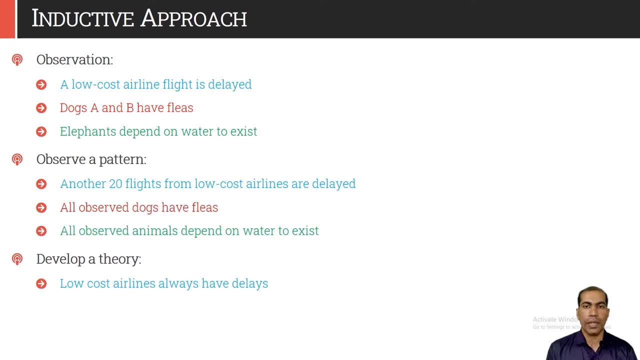 And from these two we are coming to the conclusion that, okay, All the low cost airlines always have delays, all the dogs have fleas and all biological life depends on water to exist. So these statements are now universal statements. they are true for all the inputs. 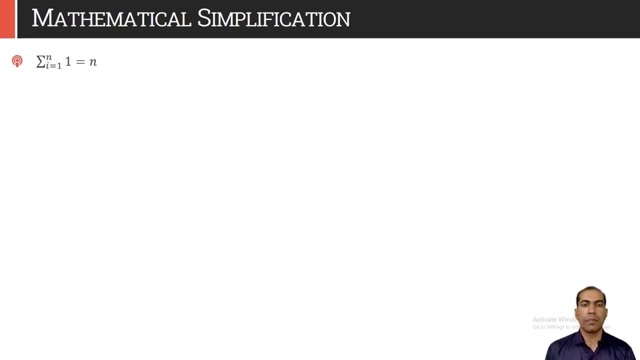 Let us try to see some mathematical simplifications which will be very much useful in case of inductive learning. So summation i is equal to 1 to n of 1 is n. This is a loop from 1 to n And we are summing 1 n times. 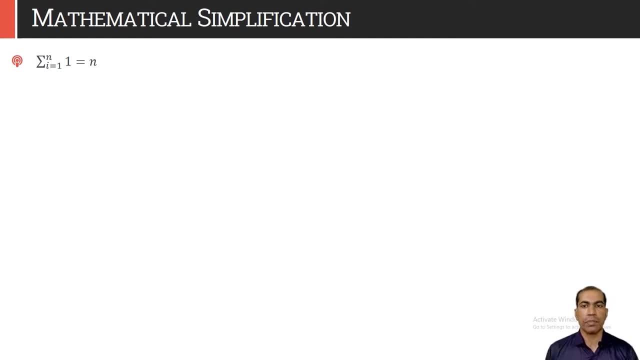 So that would be 1 plus 1 plus 1 plus 1 up to n times. So the summation final summation would be n. Summation i is equal to 1 to n, 2. So again, 2 is a constant. 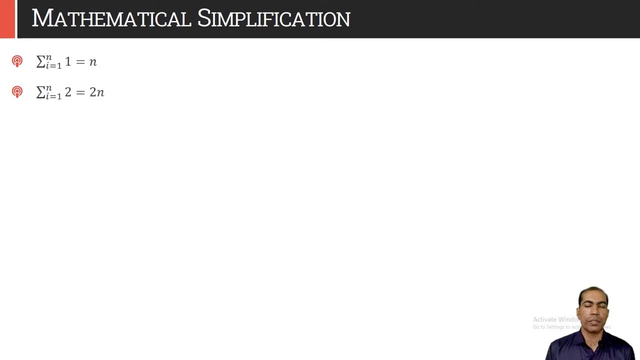 So we are adding 2 n times 2 plus 2 plus 2 up to n, So that summation would be 2 n i is equal to 1 to n i, So now i is a variable, So every time the value will be changing. 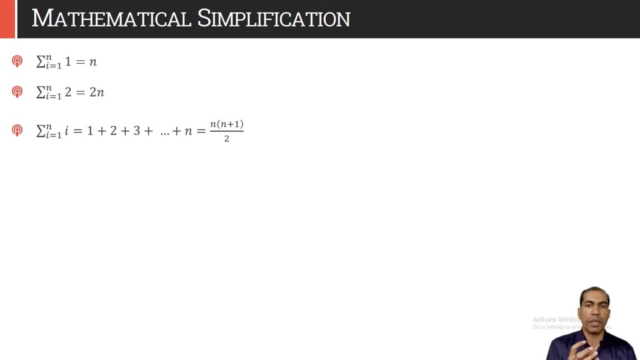 So initially it was only 1 plus 1 plus 1 plus 1 n times, Because argument was 1, which was constant. In second case it was 2, again it was constant. So we had 2 plus 2 plus 2 plus 2 n times. 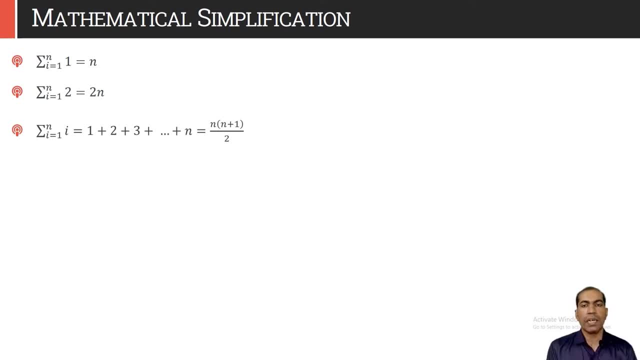 But now loop iterates with the variable i is equal to 1 to n and we are summing up i. So initially i will be 1, then 2, then 3, then 4, up to it goes up to n. So this formula would be expanded to 1 plus 2 plus 3, up to n. 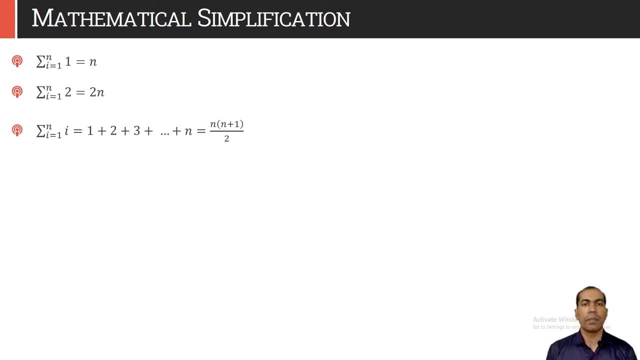 And we can simplify it just by writing n into n plus 1 by 2.. So this formula would be expanded to 1 plus 2 plus 3 up to n, And we can simplify it just by writing n into n plus 1 by 2.. 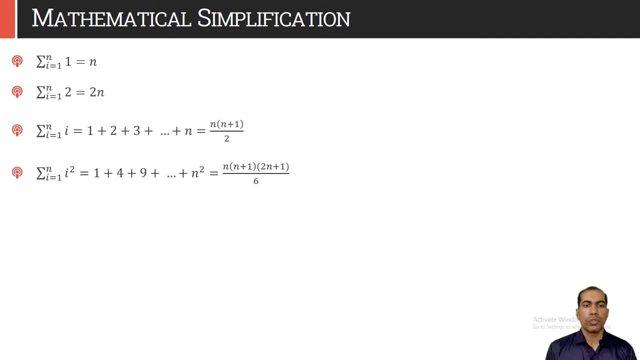 i is equal to 1 to n i square. So now we have to take square of the argument, So that would be 1 plus 4 plus 9 plus 16 and so on, And the simplification of that would be n? n plus 1 into 2, n plus 1 by 6.. 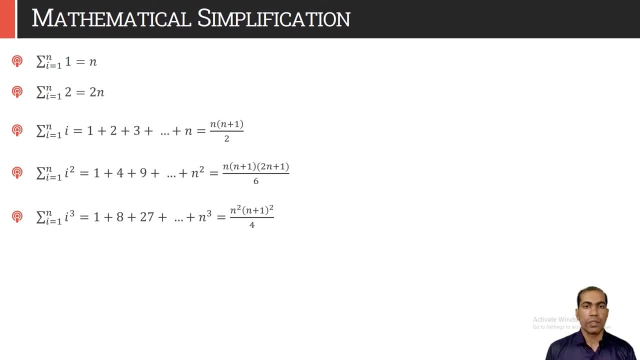 Summation i is equal to 1 to n i cube, So that would be 1 plus 8 plus 27 and so on Up to n cube. And the simplification of that series would be n square into n plus 1 whole square divided. 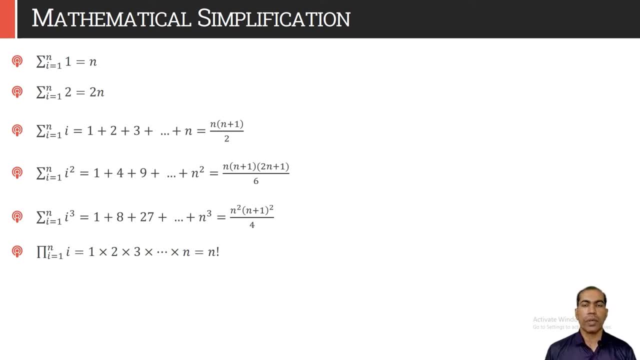 by 4.. And pi i is equal to 1 to n. sigma stands for summation, pi stands for the multiplication, So now we simply have to multiply all i's, So that is 1 into 2, into 3, up to n. 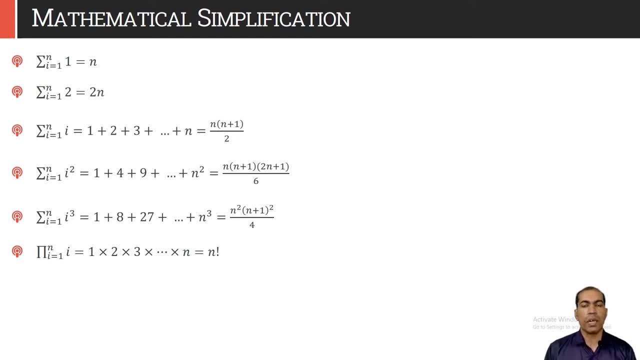 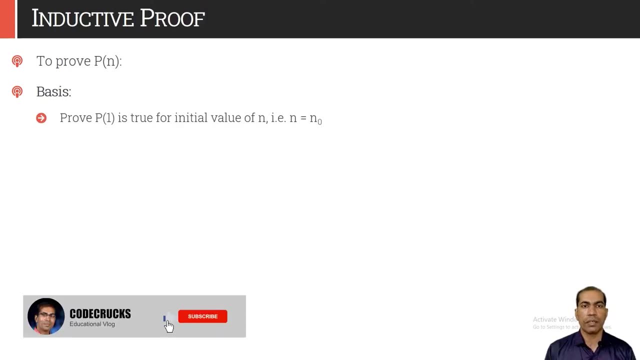 So that is nothing, but it's a n factorial. So with this we will see that how mathematical induction, or the inductive reasoning is going, is working. Inductive proof operates in two phases: basic step and the inductive step. So to prove that any given statement p of n is true for all the values of n first, we 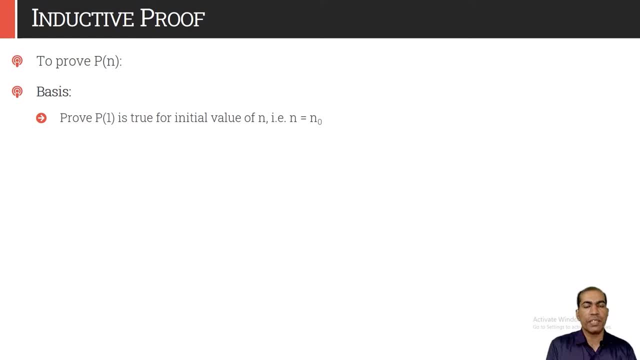 have to check whether it is a true for specific case or not, or particular incident or not, or the smallest possible value or not. So we have to prove that p of 1 is true for the initial values. Now, initial values may not be always 1.. 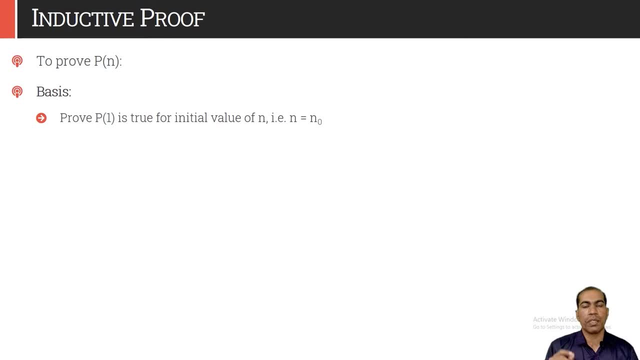 Okay, It depends. It depends whatever minimum or the starting point is given. So we have to check whether the given statement is true, for initial value n is equal to n 0 or not. So n 0 is some initial value from where we have to start. 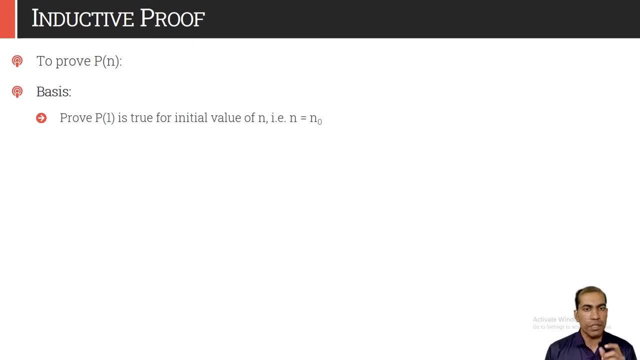 So if it is true, we can say that p of 1 is true. It means the specific case is true, as, like, dog A is having fleas or a particular flight is delayed, something like that very specific. Then we are going to the inductive step. 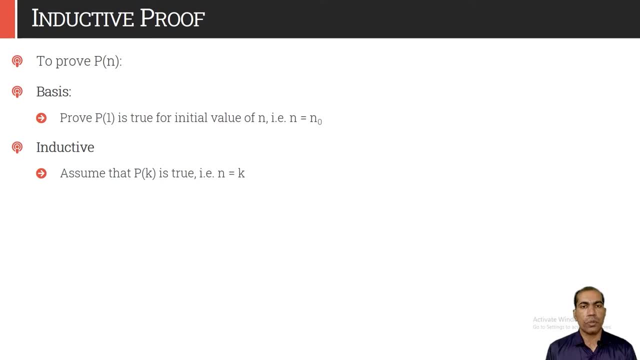 So first we will assume that p of k is also true. It means, for n is equal to k. also, whatever statement is given to us is true. So that is our assumption. And from this assumption, So this is nothing but finding the patterns, like 20 flights have been delayed. 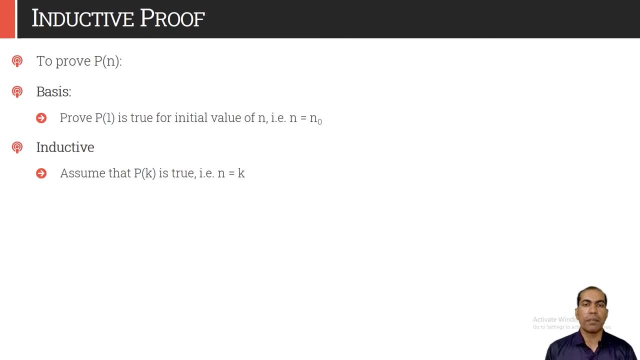 All the dogs we have observed. they are having the fleas and so on. So this is just a pattern And from this we have to generalize our observation. It means we have to prove that p of k plus 1 is also true. So now we have to consider: n is equal to k plus 1.. 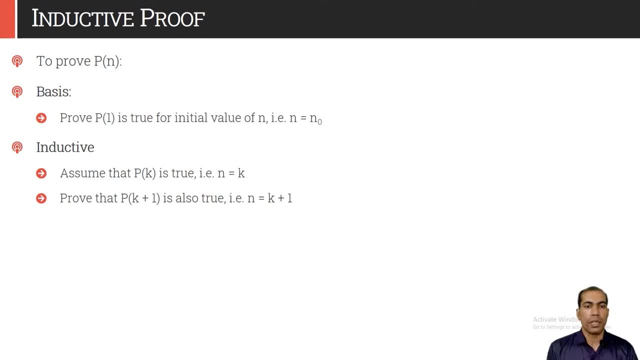 And from that we will try to prove that the statement is true. If it is true, then we can say that the given statement will be true for any value of n. So that is how inductive proof is working. Let us see one example. 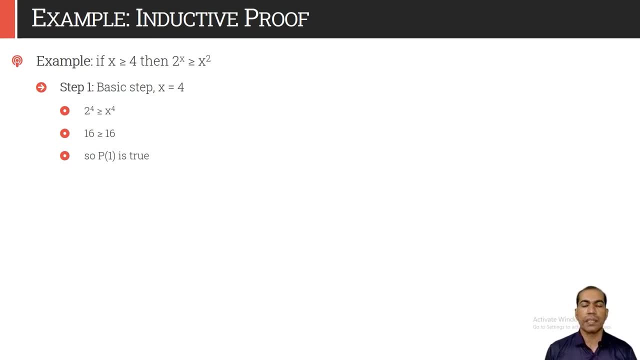 If x is greater than or equal to 4, then 2 power x greater than or equal to x square. We are considering the same example, what we have discussed in inductive proof, But the way of proving will be different. The step 1.. 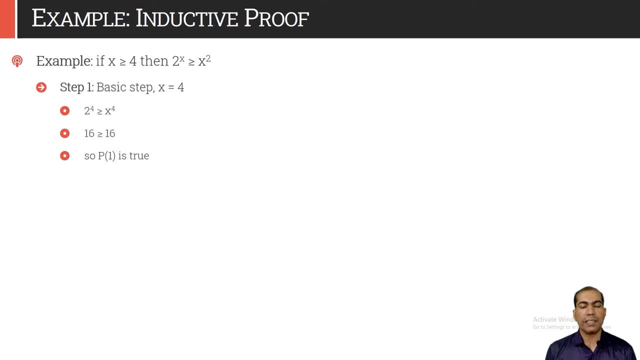 This is the basic step. So it is starting with x greater than or equal to 4.. So that would be our initial value. So when we take x is equal to 4, the claim is 2 power, x greater than or equal to x square. 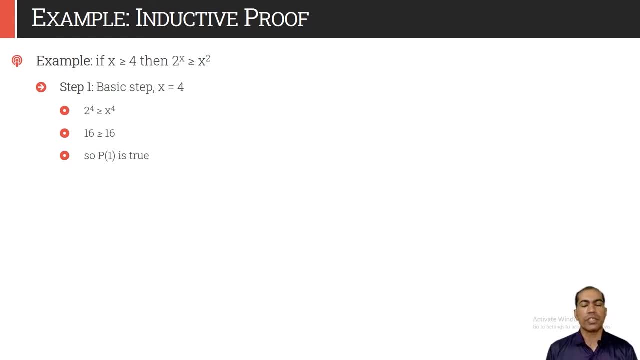 would be true because 2 power x is 16 and x square is also 16.. So 16 greater than or equal to 16 is true for the initial value of x. So we will say that p of 1 is true. We do not have to test it, for x is equal to 1.. 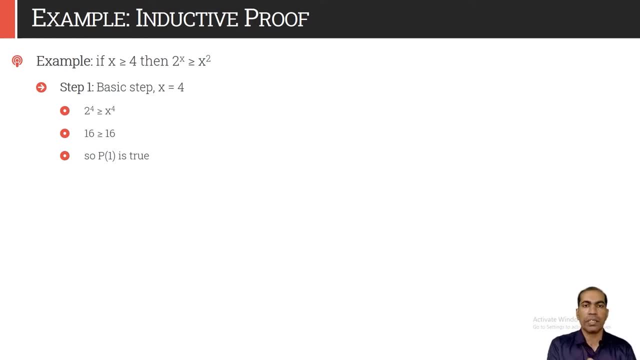 Rather we have to test it for the initial value. So our initial value or the hypothesis is what x should be greater than or equal to 4, then the given statement is true. So here n0 is 4.. Now we are moving towards induction step. 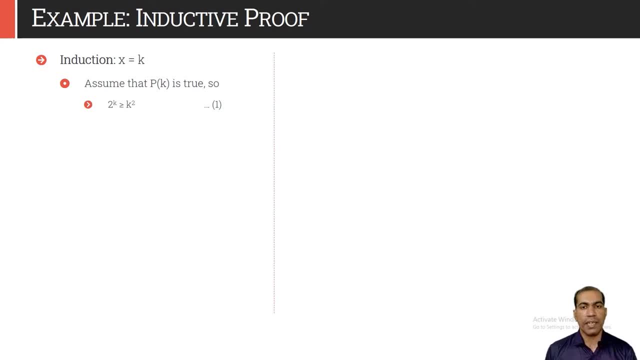 We are assuming that x is equal to k and for that k given statement is true. So we will assume that p of k is true and our claim would be: 2 power k is greater than or equal to k square. Let us call it as equation number 1.. 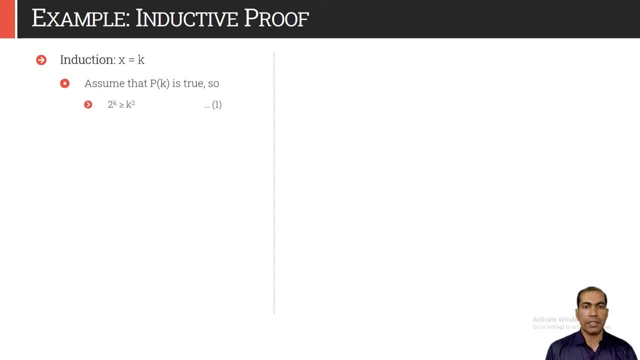 And we will assume that p of k is true And from this we will try to generalize it. So we will prove that the statement is true, for x is equal to k plus 1 as well. So k will be replaced by k plus 1 into the equation 1 or into the original claim that. 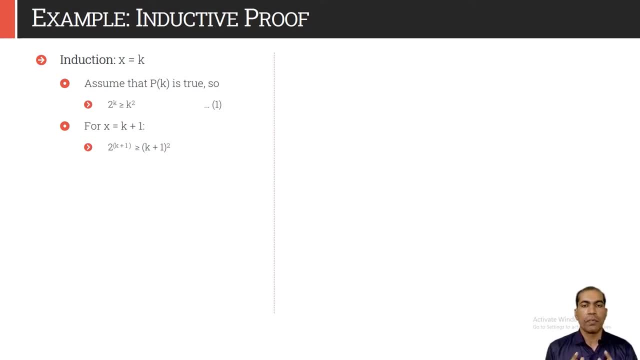 is 2 power x greater than or equal to x square. We are simply replacing x by k plus 1.. So it would look like 2 power k plus 1 is greater than or equal to k plus 1 whole square. We know that 2 power k plus 1 can be written as: 2 power k plus 1 is equal to k plus 1 whole. 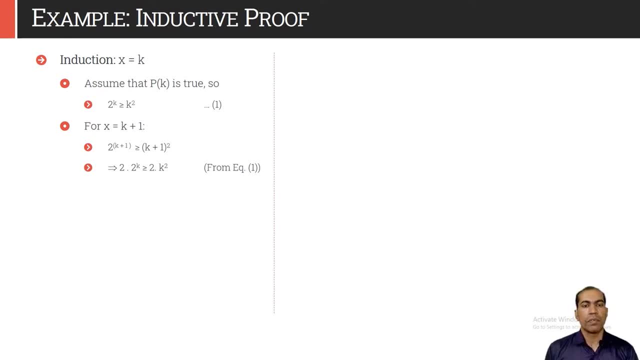 square. Then we can say that p of k is 2 times 2 into 2 power k, which is greater than or equal to k plus 1 whole square. It comes from the equation number 1, because 2 power k is greater than or equal to k square. 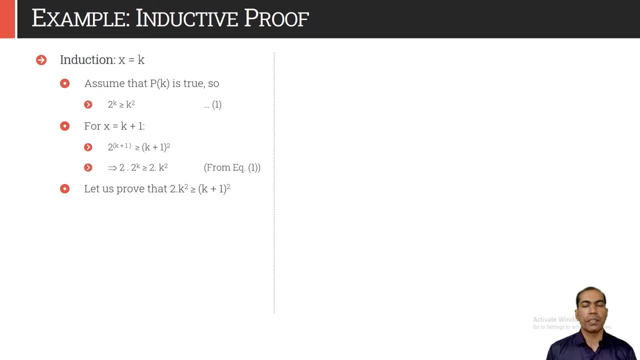 as per the equation 1.. If we can prove that 2 power k square is greater than or equal to k plus 1 whole square, then we can say that 2 power k plus 1 is greater than or equal to k plus 1 whole square by: 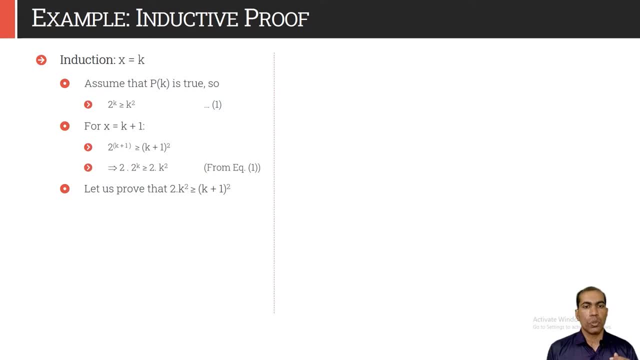 the property of transitivity. Why 2 power? k plus 1 whole square is greater than or equal to 2 into k square. And now we are trying to prove that 2 into k square is greater than or equal to k plus 1 whole square. So it implies: 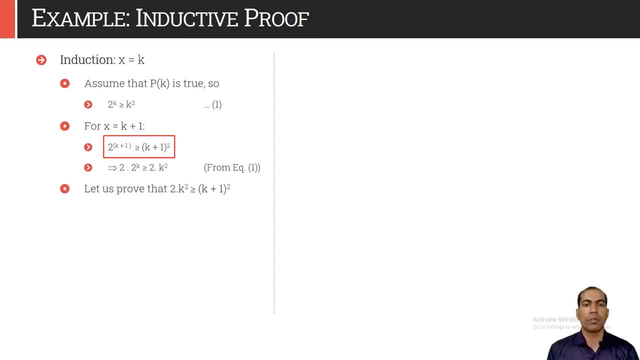 2 power, k plus 1 would be definitely greater than or equal to k plus 1 whole square. We are expanding k plus 1 square term just like this. So this would be 2 k square greater than or equal to k square plus 2 k plus 1.. By simplifying, it would be k square greater than 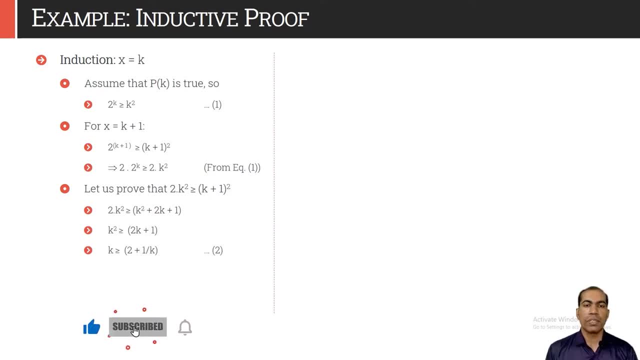 or equal to 2 k plus 1.. We are dividing on both the side by k, So we are left with k greater than or equal to 2 plus 1 by k. Let us call it as equation number 2.. So in equation, if we put 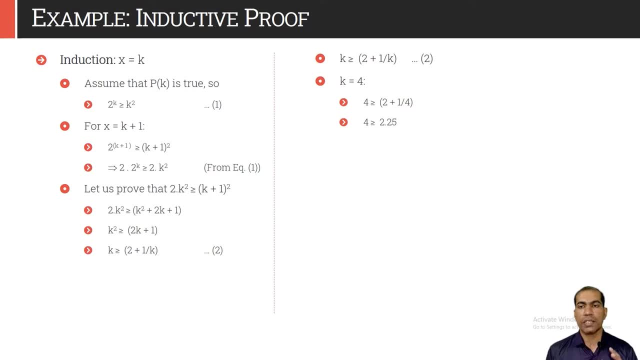 k is equal to 4, because that was our initial assumption- x is equal to 4.. So we are starting with that, for k is equal to 4.. Equation 2 would be 4 greater than or equal to 2 plus 1 by 4, and that is nothing but 4 greater than or equal. 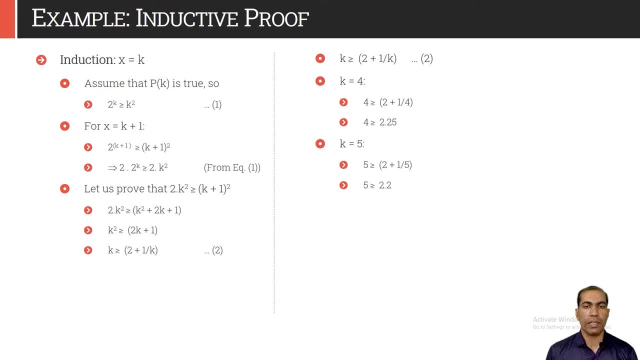 to 2.25.. For k is equal to 5, equation 2 will reduce to 5 greater than or equal to 2.2.. For k is equal to 6, equation 2 will reduce to 6 greater than or equal to 1.67.. So you see. 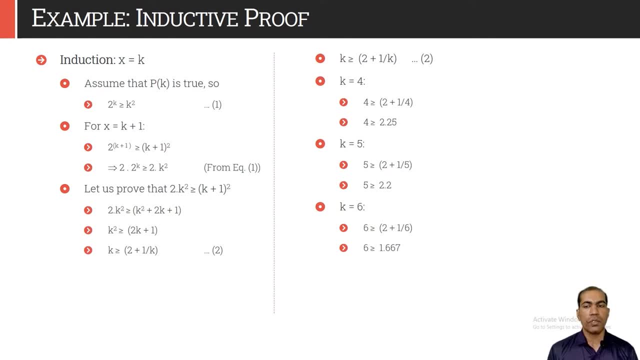 that whatever may be the value of k now onwards, it is always going to be remain greater than or equal to 1.67.. For right hand side: because right hand side is decreasing, left hand side is increasing, For k is 4, 5 and 6.. Right hand side is 2.25, 2.2 and 1.667 respectively. So as left hand, 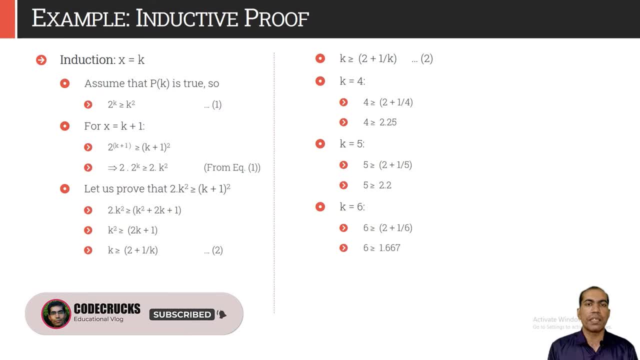 side is increasing. right hand side is decreasing, So that inequality is always going to be true. So we have proved that 2 k square is always greater than or equal to k plus 1 whole square, and we already know that 2 into 2 k is greater than or equal to 2 k plus 1 whole square. 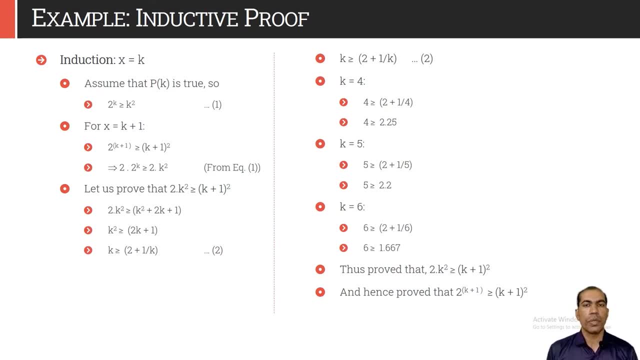 And 2 into 2 k is nothing but 2 power k plus 1.. So ultimately, we have come to the conclusion that statement 2 power k plus 1 is greater than or equal to k plus 1 whole square, and that means our claim is true, for x is equal to k plus 1, and hence the given statement. 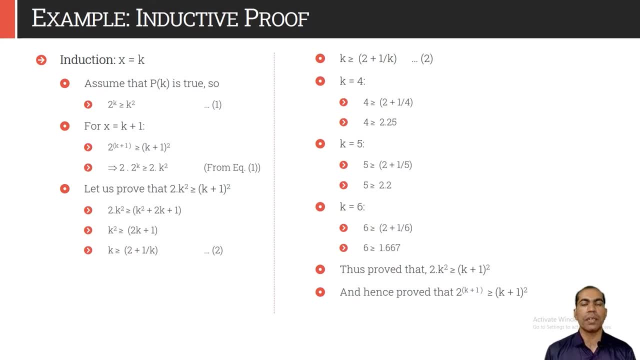 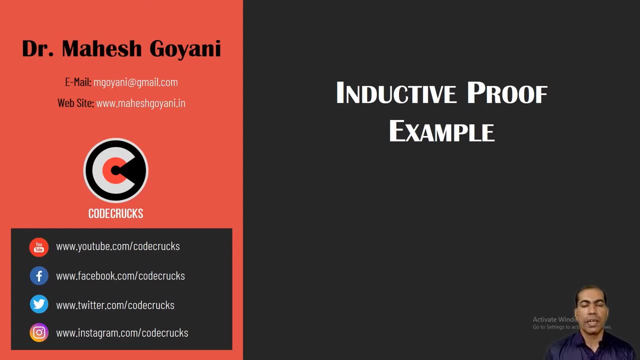 is true. So we have proved this with mathematical induction or by the inductive proof technique. Hello folks, welcome to Codecracks. This is Mahesh Gyani, and in this video I will be talking about inductive proof example. In previous video I have already discussed what do we mean by inductive proof and how. 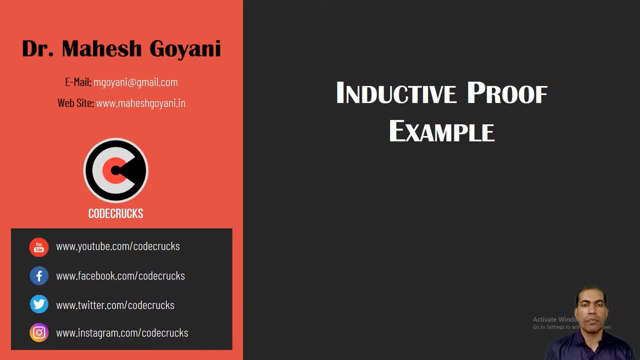 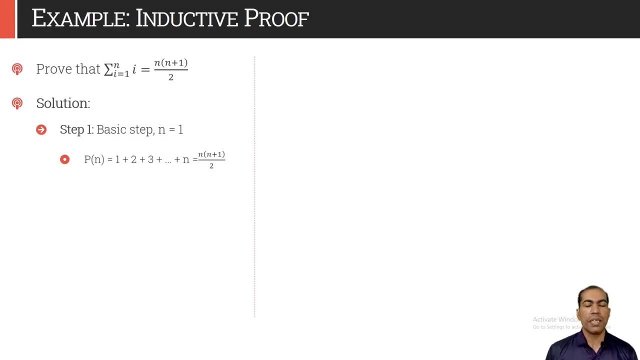 it works. We have also differentiated inductive proof from the deductive proof technique. Inductive proof starts from very specific case. It will find the pattern and it comes to the generalization of certain theory. We are given the statement that we have to prove summation. i is equal to 1 to n. i is equal to n into n plus 1 by 2.. 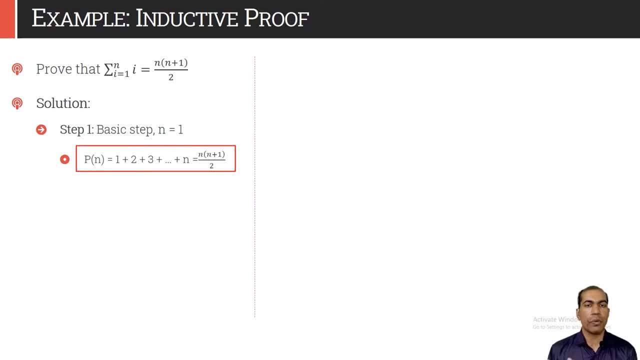 So the series 1 plus 2 plus 3 plus up to n is equal to n into n plus 1 by 2.. This is the claim. Now, by inductive proof or by the mathematical induction, we will prove that this statement is actually true. So, as we know that inductive proof operates in two, 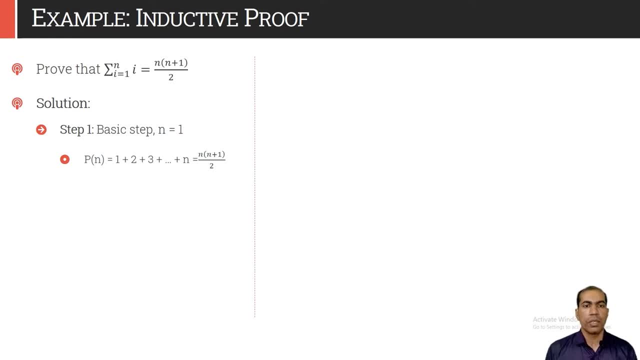 stages. One is a basic step and other one is the inductive step. So in basic step we will check whether a given statement is true for the initial value of n or not. So let us start with: n is equal to 1.. Let us put: n is equal to 1.. 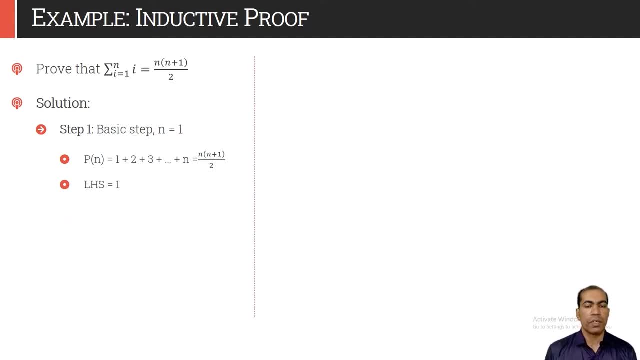 So on left hand side we will select the first entity, that is 1.. On right hand side, if we replace n by 1, then that would be 1 into 1 plus 1 divided by 2, that is again 1.. So as 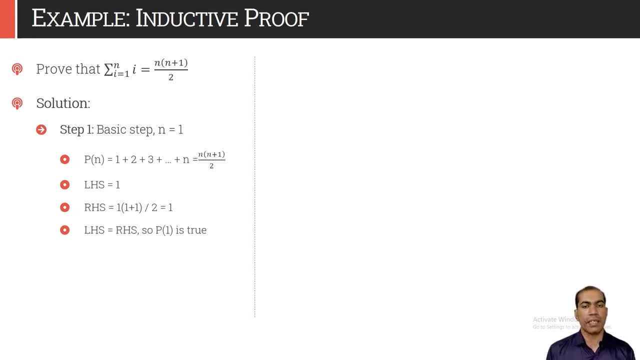 we can see that left hand side is equal to right hand side for n and right hand side for n is equal to 1.. So we can say that the given hypothesis or given statement is true for p of 1.. Now we will form the inductive hypothesis and we will assume that the given 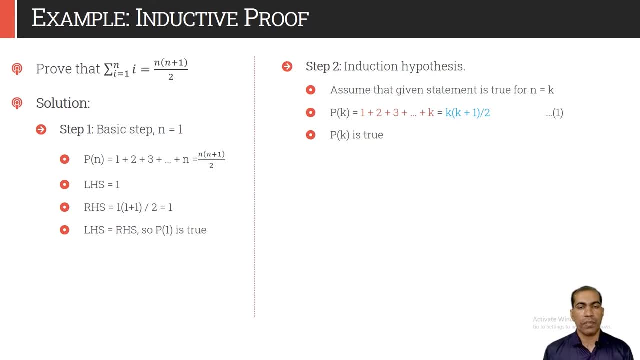 statement is also true for n is equal to k. So simply we will put: n is equal to k in this particular representation. So that would be: p of k is equal to 1 plus 2 plus 3 up to k. So we are summing up first: k values only Will be same as k into k plus 1 by 2.. So call. 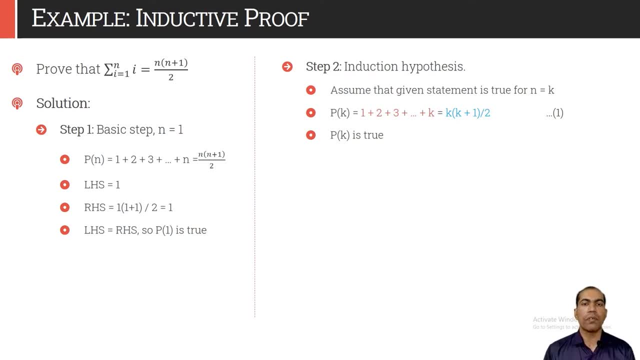 it as an equation number 1 and we are assuming that this p of k is true. Now we will try to prove that. if this statement is true, for n is equal to k plus 1, then our claim will be true. So we are selecting: n is equal to k plus 1 and we are putting that value into 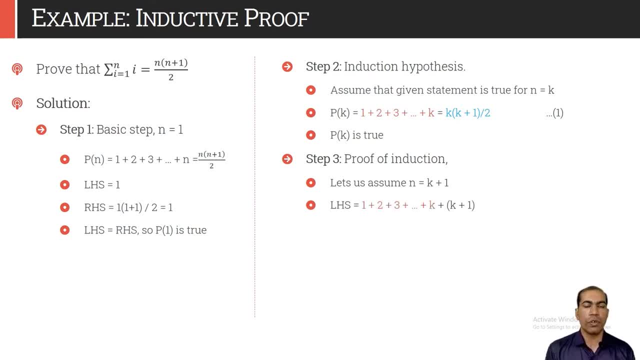 this equation, The left hand side of this statement, would be 1.. 1 plus 2 plus 3 up to k plus k plus 1, because now n is replaced by k plus 1, so it will go up to k plus 1.. As we can see in equation number 1, whatever red colored part is here: 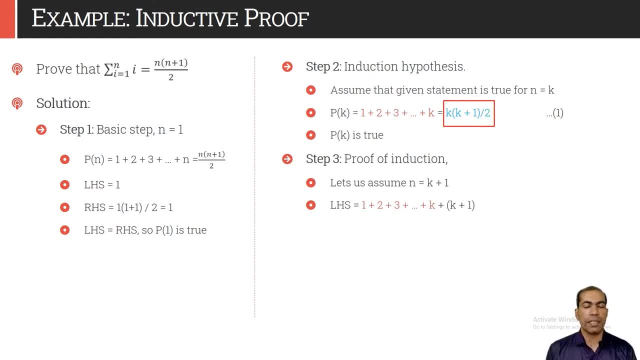 can be replaced by the blue component in equation 1, that is, k k plus 1 by 2.. By replacing this summation by k into k plus 1 by 2, we will get this one k into k plus 1 by 2 plus k. 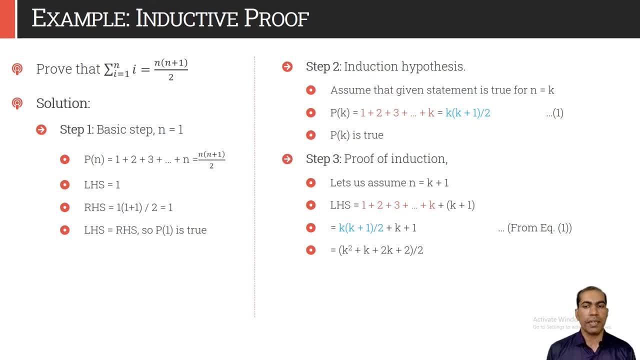 plus k plus 1.. Let us simplify this. So this would be k square plus k plus 2k plus 2 divided by 2. And we are taking the k common from the first two entities and we are taking 2 common from the second two. So this will reduce to k into k plus 1 plus 2, into k plus 1 divided. 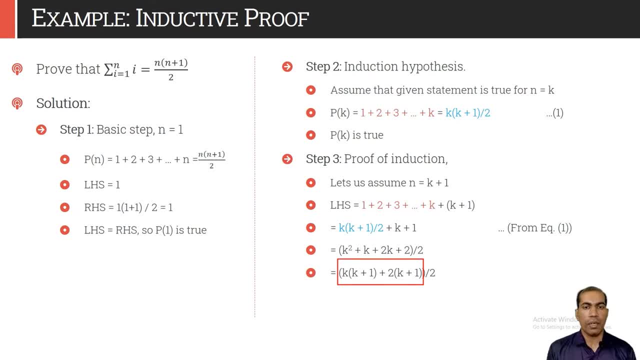 by 2.. Again, we can take k plus 1 common in this equation, So it will reduce to k plus 1.. So that is what we actually wanted to prove By putting n is equal to k plus 1. in this right hand side of this equation it would be k plus 1 into k plus 2 divided by 2.. And 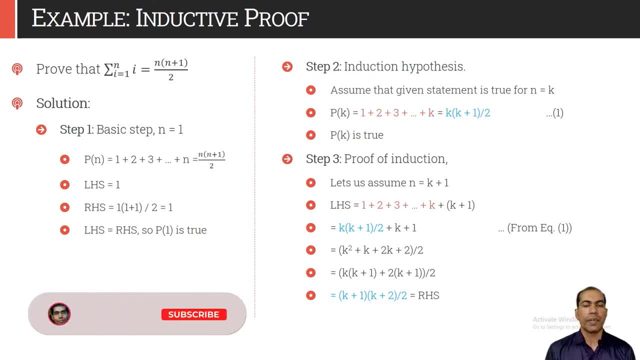 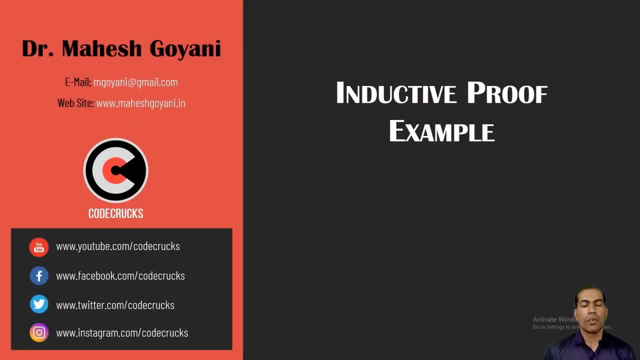 that is what we have just derived, So we can say that given statement is true, for n is equal to k plus 1 as well, And we can say that whatever claim we have made, that is acceptable and it is totally true. Hello folks, Welcome to Code Crux. This is Mahesh Guyani, And in this video I am going 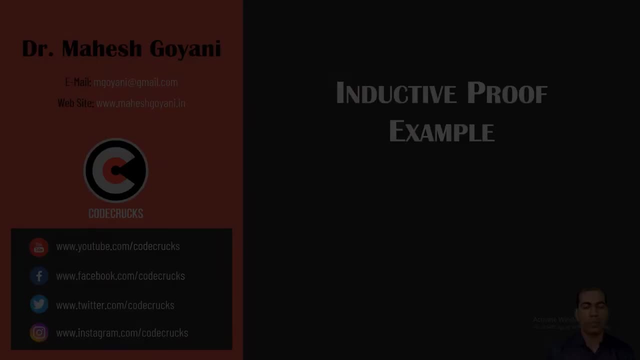 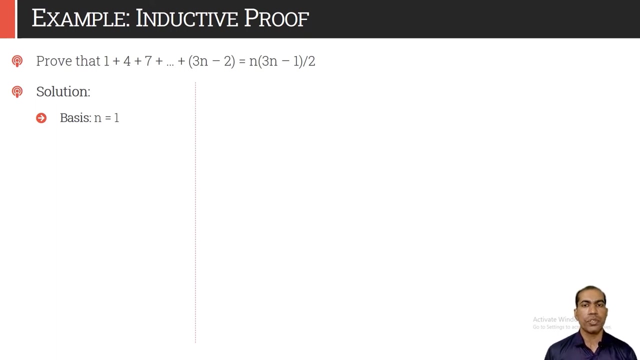 to talk about one more example on inductive proof. We have to prove that 1 plus 4 plus 7 up to 3. n minus 2 is equal to n into 3, n minus 1 by 2.. So first we will start with the basic step. So for n is equal to 1, the left hand. 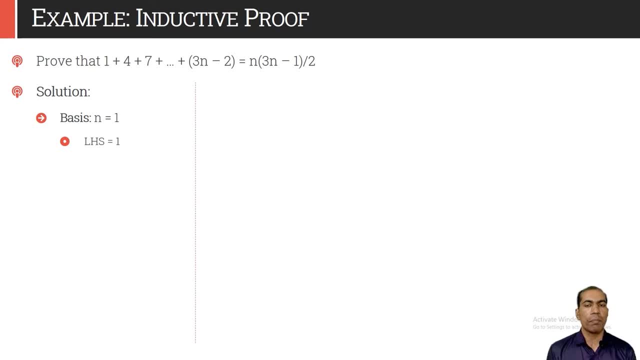 side of this equation would be 3 into 1 minus 2. so that is nothing, but it's a 1.. On right hand side, by replacing n by 1, the equation would be 1 into 3 into 1 minus 1 by 2. so ultimately, 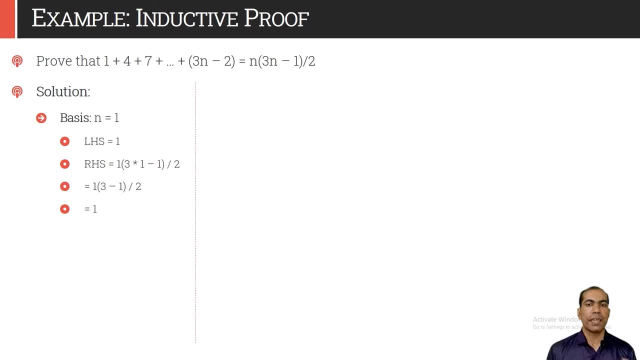 that will reduce to 1 only. So we can say that left hand side is equal to right hand side. so the given statement is true, for n is equal to 1 and hence we can say that p of 1 is true. Second stage is what? Induction stage? so we are assuming that the given statement 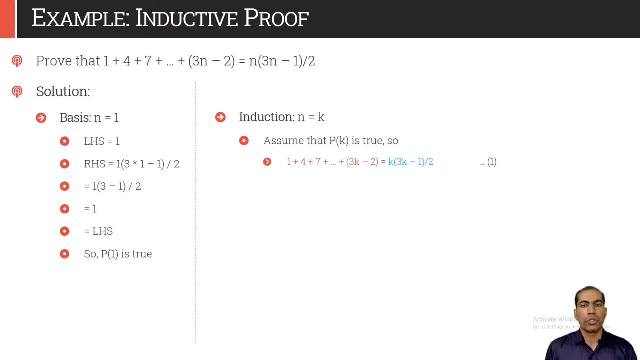 is true, for n is equal to k as well. so we are assuming that p of k is true. so simply we will replace n by k in given statement. so that would be one plus four plus seven up to 3k minus two is equal to k into 3k minus 1 by 2.. Call it as equation number one. so 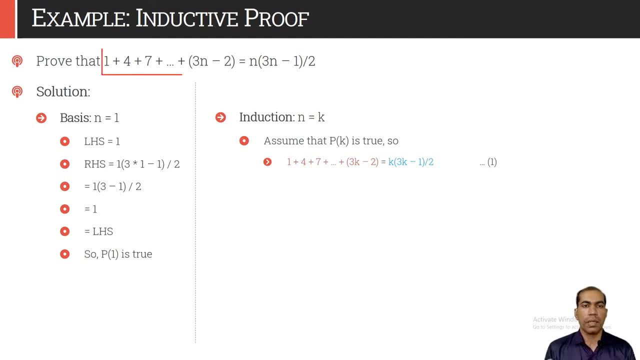 So simply, we have gone up to kth term into this equation. now we will try to prove it, for the n is equal to k plus 1, and if we can prove that left hand side of this statement is same as right hand side, for n is equal to k plus 1, then our claim will hold. 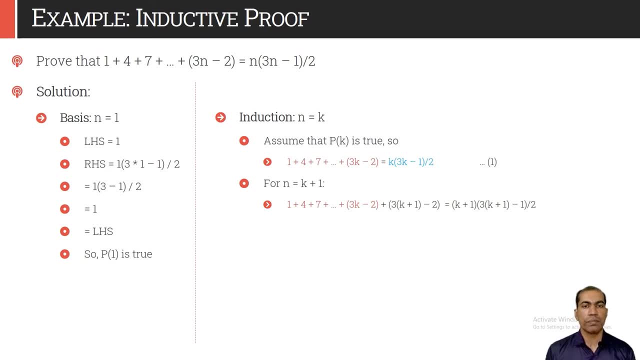 So let us put n is equal to k plus 1 into this, so this will be 1 plus 4 plus 7, up to 3k minus 2, and now we have to go one step forward. that is, now we have to go up to n. 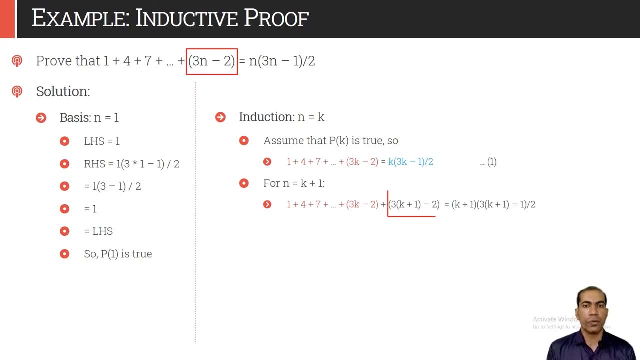 is equal to k plus 1, so this would be 3 into k plus 1 minus 2 is equal to k plus 1 into 3 k plus 1 minus 1 divided by 2.. So now we will try to simplify these things and, as you can see that from equation number, 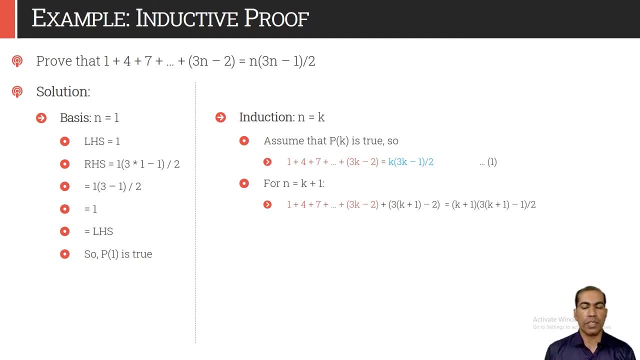 1, whatever red part are shown in both the equation. that can be replaced by the blue part, Because that is what our assumption is: that 1 plus 4 plus 7 up to 3k minus 2 is equal to k into 3k minus 1 by 2.. 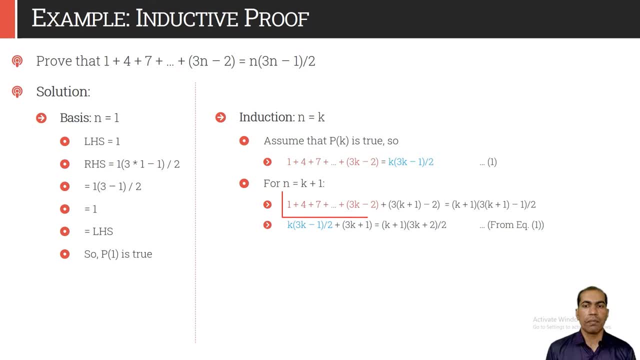 So we are replacing the blue part in equation 1 with this red part. so because both are equivalent, so that would be k into 3k minus 1, by 2 plus 3k plus 1, that is the simplification of this one is equal to k plus 1.. 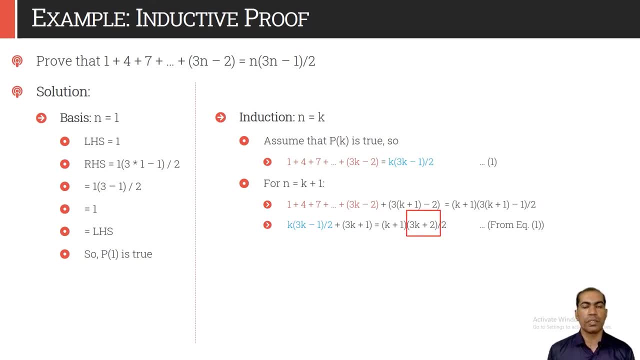 k plus 2 divided by 2, and 3k plus 2 is a simplification of 3 into k plus 1 minus 1 term. Let us keep simplifying these two statements and we will check whether both are reducing to identical values or not. 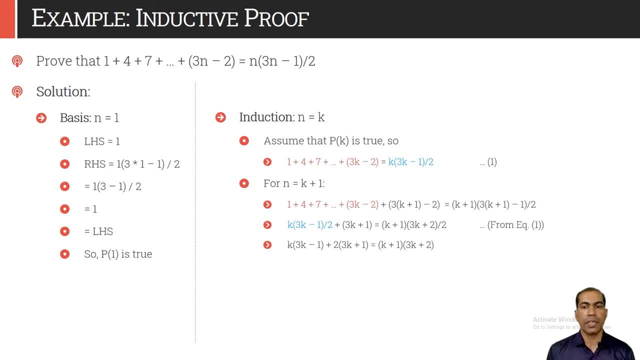 So this could be written as k into 3k minus 1, plus now this 2, which was in division that we have to multiply with this one to have, So that would be 2 into 3k plus 1, is equal to k plus 1 into 3k plus 2 divided by 2.. 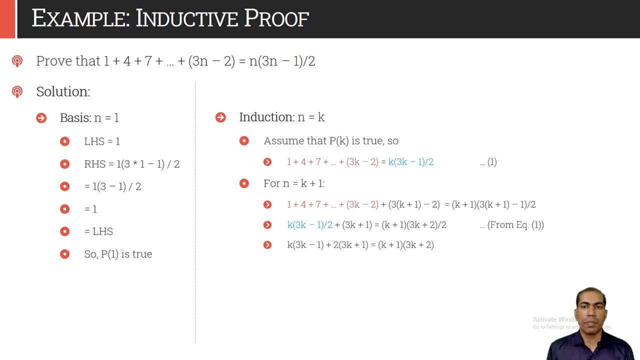 Now, 2 is in denominator on both the sides, so we can simply reject them. So this equation is without writing: 2 in denominator. we will multiply k inside, so this would be 3k square minus k plus. we will multiply 2 inside, so that would be 6k plus 2.. 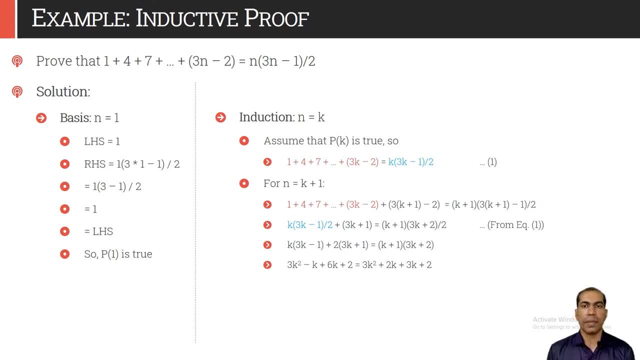 Again, we are simply multiplying k plus 1 with the 3k plus 2.. So that would be 3k square plus 2k plus 3k plus 2. we are simply rearranging the terms. so the left hand side would be 3k square minus k plus 6k, will be 5k plus 2 on right hand. 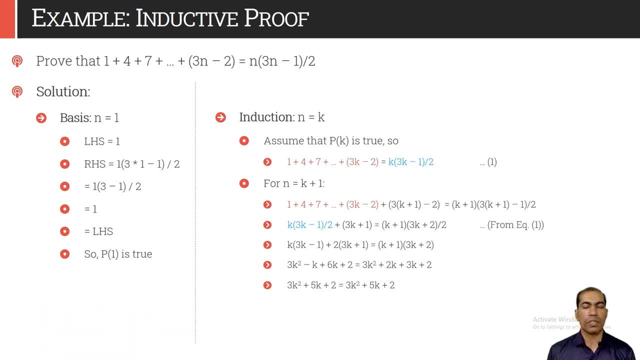 side also, we have 3k square plus 2k. plus 3k that would be 5k and plus 2.. So, as we can see that left hand side and right hand side are identical, So whatever claim we have made is true. that is statement is true for PK plus 1 as well. 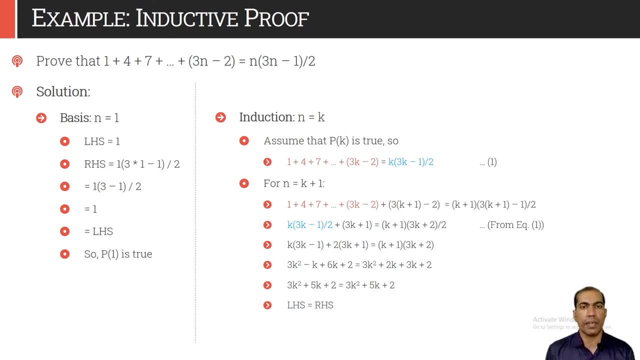 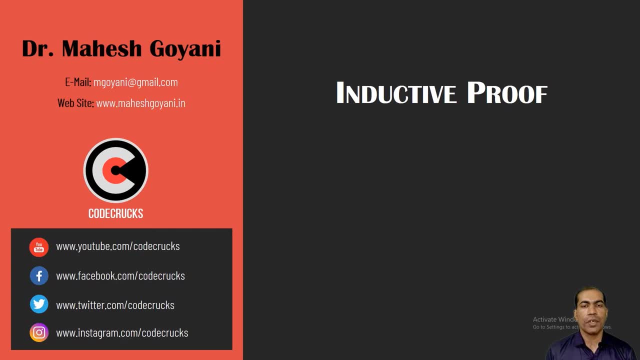 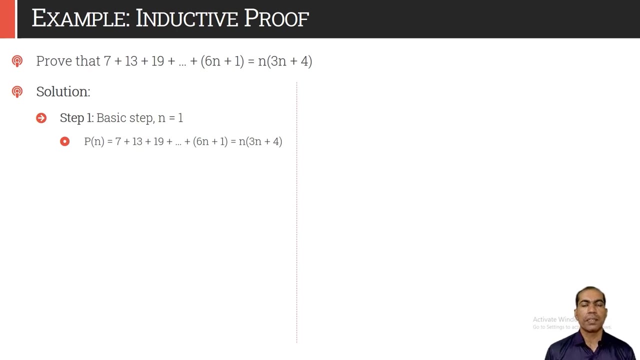 and hence it is universally true for any value of n. Hello folks, welcome to Codecracks. this is Mahesh Guvani, and in this we will be talking about one more example on inductive proof. We have to prove that the series is 7 plus 13 plus 19 plus up to 6, n letter plus 1 in. 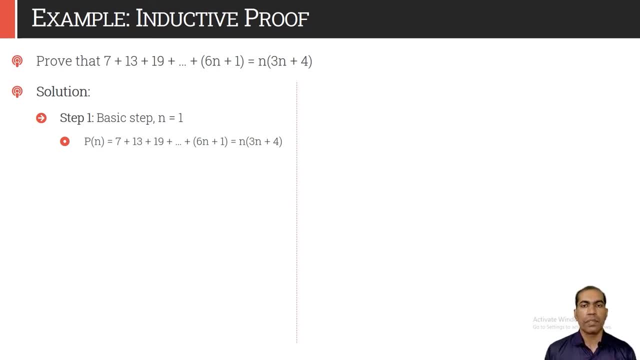 is same as n into 3n plus 4.. We are already familiar with how inductive proof is working. We need to first check that given statement is true, for n is equal to 1 or not. Then we will formulate our hypothesis and we will assume that it is true, for n is equal to k. Then we have to 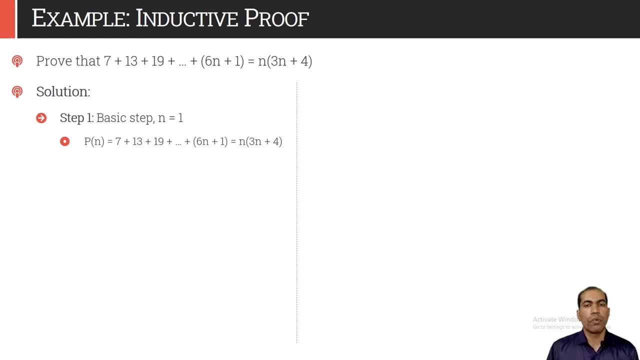 show that the assumed hypothesis is true, for n is equal to k plus 1 as well. If we can prove that, then we can say that the given statement will hold for any value of n. It means our claim is true. So let us start In basic step. we are assuming that n is equal to 1.. The p of n. 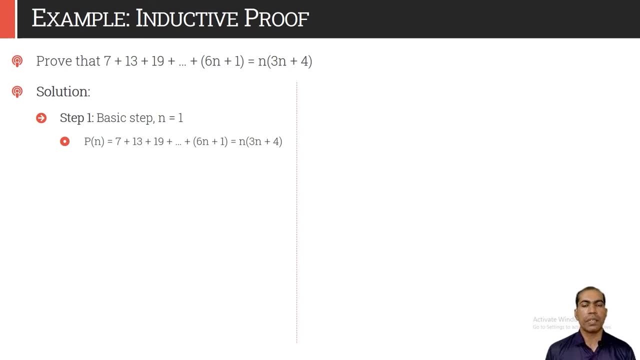 that means the given statement is 7 plus 13 plus 19, plus plus plus up to 6n plus 1 is equal to n into 3n plus 4.. Let us keep: n is equal to 1.. So on left hand side. 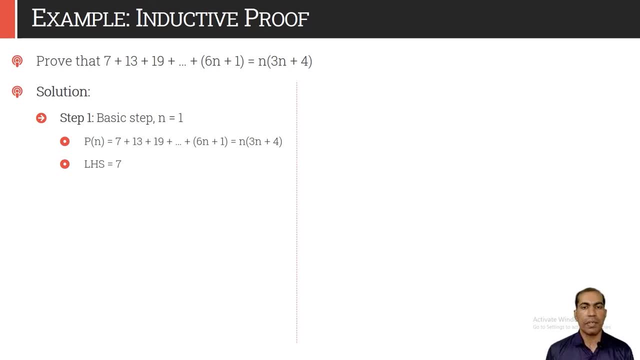 either we can select the very first entry, that is 7, or we can put n is equal to 1 into 6n plus 1.. So that is also 7.. So for n is equal to 1, left hand side is reducing to 7.. 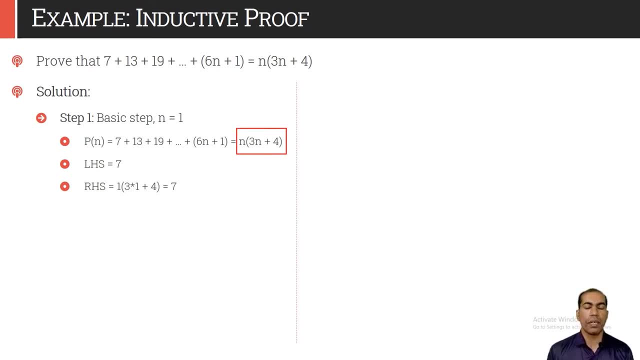 On right hand side it would be 1 into 3n, that is, 3 into 1 plus 4. So that is is also 7.. As we can see that left hand side is same as right hand side, We can say that: 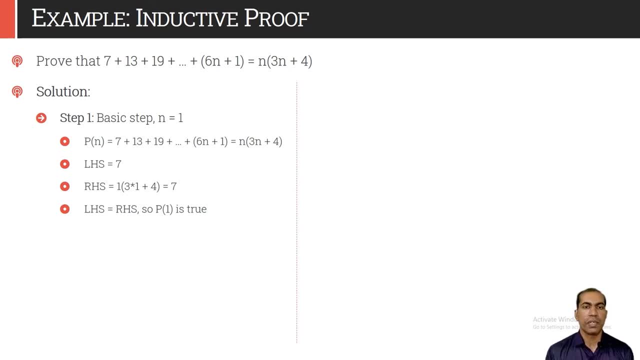 P of 1 is true for given series. Now we will move towards induction hypothesis, So we will assume that statement is true, for n is equal to k, So P of k would be 7 plus 13 plus 19, plus we have to expand it up to n is equal to k, So this would be simply 6k plus 1 is. 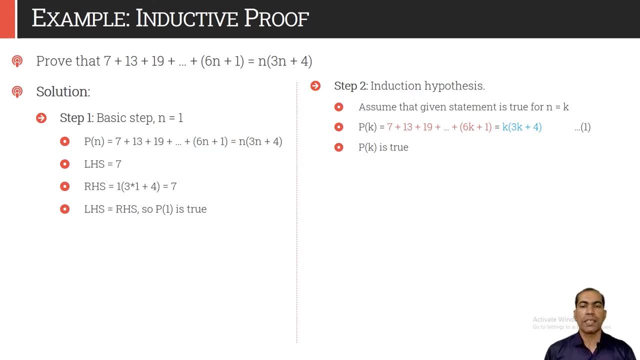 equal to k into 3k plus 4.. Call it as equation number 1.. Now I will try to generalize it by proving it, for n is equal to k plus 1 as well, So we will put: n is equal to k plus. 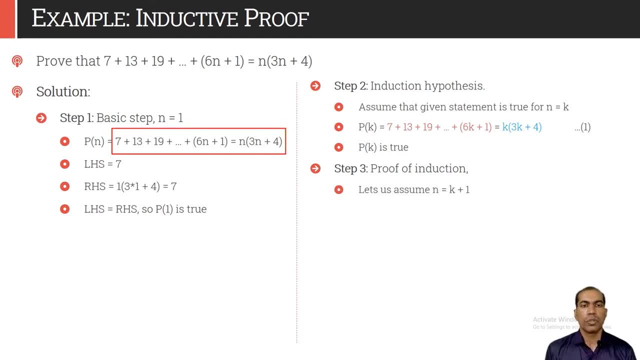 1 into this statement, So that would be 7 plus 13 plus 19.. Then we will go up to k-th step, that is, 6k plus 1.. Then we will go up to k plus 1 step, so that will be 6 into k. 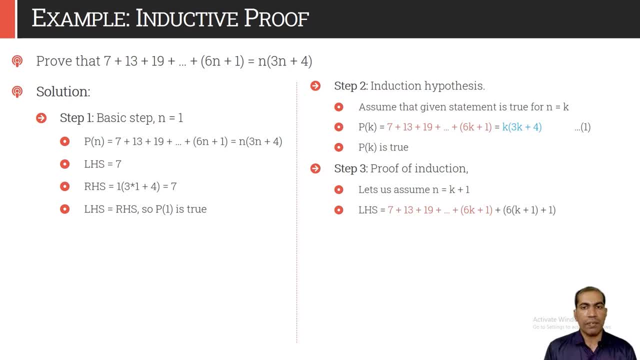 plus 1. plus 1.. So we'll start with the left hand side and we'll come to the right hand side. So there are two approaches: Either you start with left hand side and you derive the right hand side, or you directly start with left hand side is equal to right hand side and you keep reducing. 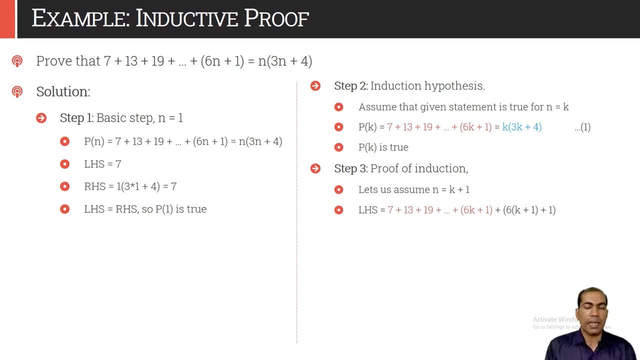 the equations and come to the identical values. Either way is the right one. So in left hand side we know that whatever is highlighted in red can be replaced by k into 3k plus 4, as per the equation number 1.. So let us replace it with that value, So we will have k into 3k plus 4. 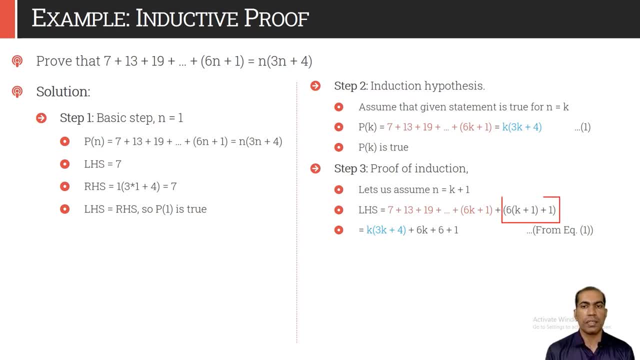 plus. Now we'll simplify this term, So that would be 6k plus 6 plus 1.. We are multiplying k within the parenthesis, So that would be 3k square plus 4k Plus 6k plus 7.. And by summing up k's we'll get 3k square plus 10k plus 7.. Let us rewrite this. 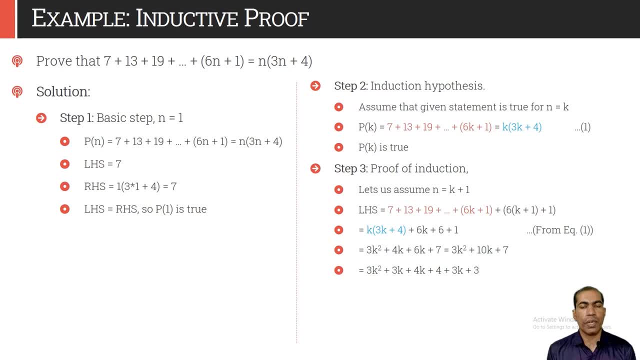 10k can be written as 3k plus 4k plus 3k and 7 can be written as 4 plus 3.. So by putting all these things together we can rewrite the previous equation as 3k square plus 3k plus 4k plus 4 plus. 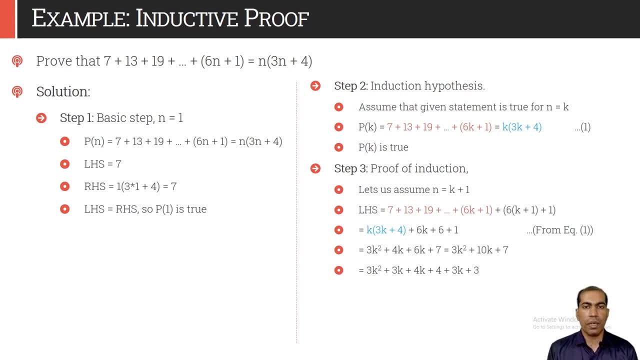 3k plus 3.. And by taking the common elements from two terms. So in first term 3k is common. In second two terms, 4 is common And last two terms, 3 is common. And after taking the entities common out of those, 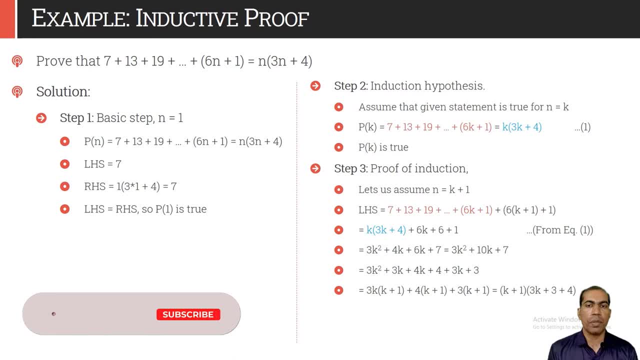 we can see that we can again take k plus 1 common from all of them. So we are left with k plus 1 into 3k plus 3 plus 4.. Let us rewrite it again So that would be: k plus 1 into 3k plus 3 can be written as 3. we are taking common, So that would. 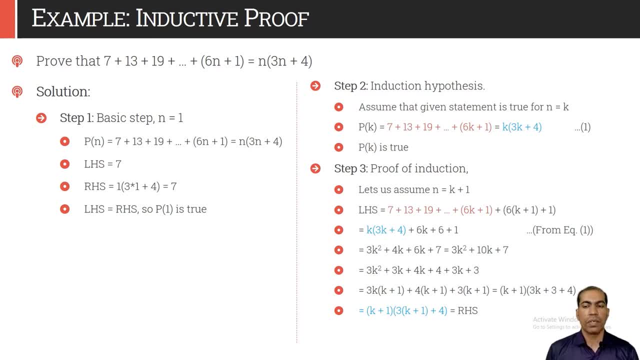 be 3 into k plus 1 plus 4.. And that's what we exactly wanted. Look at here: This is n into 3n plus 4.. So n should be replaced by k plus 1.. And when we replace this n by k plus 1, that would. 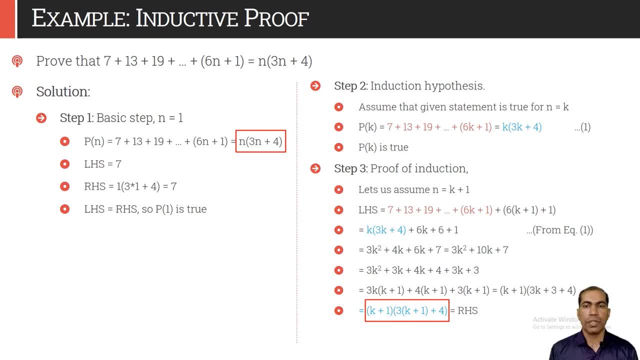 exactly. look like this: k plus 1 into 3 of k plus 1 plus 4. It means we have started with left hand side and we have come to the conclusion. It means we have come to the right hand side as well. So this given hypothesis holds true, for n is equal to k plus 1 as well. 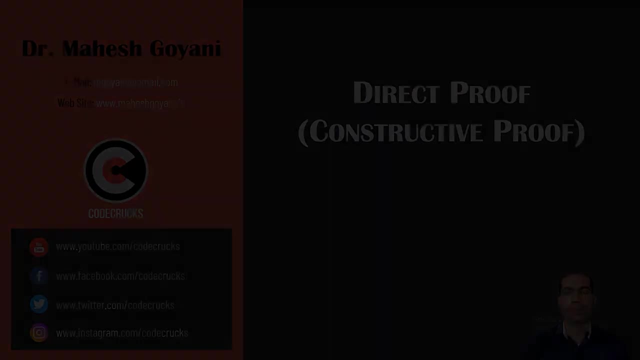 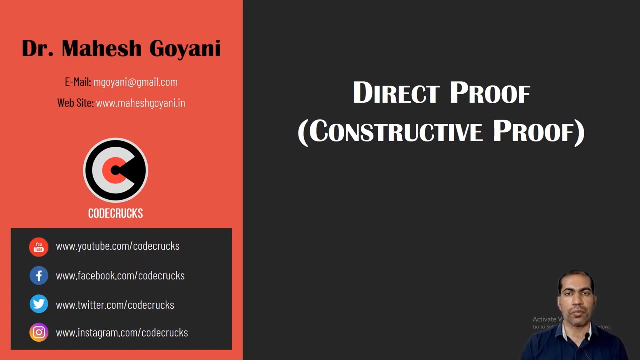 And hence a given statement is true. Hello folks, Welcome to Code Crux. This is Mahesh Gujani, And in this video I will be talking about constructive proof. Constructive proof is the type of direct proof And it tries to prove the given statement by help of examples. 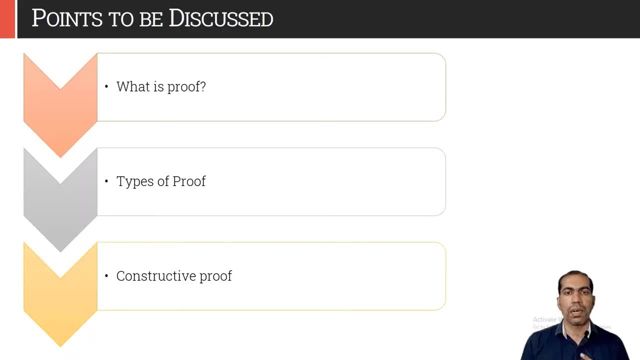 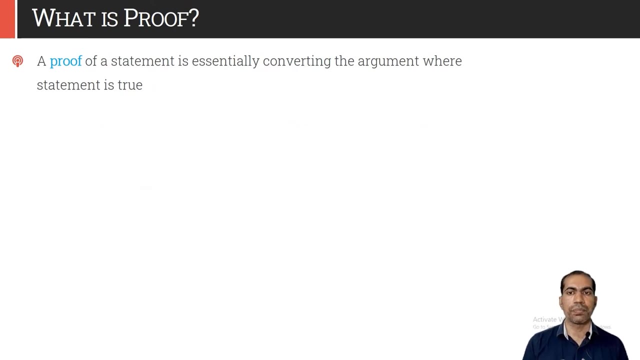 So this is very simplistic way of proving something I will be targeting. what is proof, What are the different types of proof And, at last, I will be talking about constructive proof And we will discuss few examples of that. A proof of a statement is basically converting. 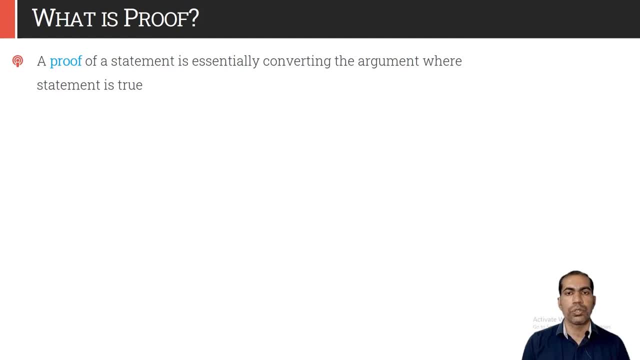 the argument where the statement will stand true. So, whatever statement is given, we are making some logical arguments And we think that and we prove that the given statement is true. So the sequence of arguments is called a proof, So the statement could be proved. 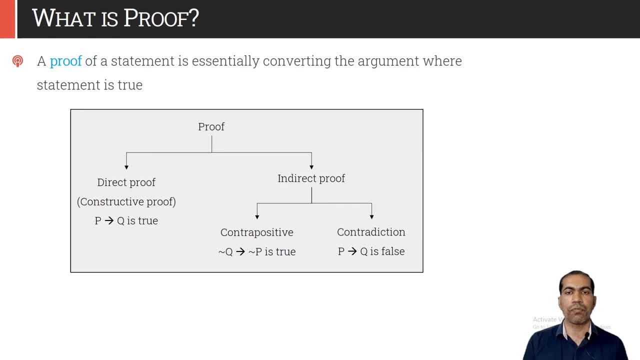 in many different ways. There are two basic types of proof, which is known as direct proof or indirect proof. Constructive proof comes under the direct proof Cont depositive and the contradiction comes under the indirect proof. Proof statements are typically in the form: If hypothesis is true, then conclusion is true, So we can write it as like if statement. 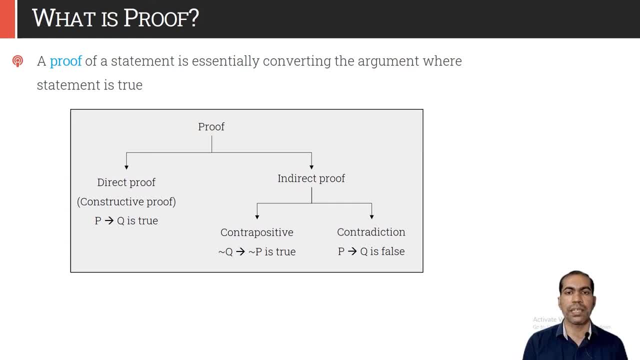 P, then Ah a Q. or we say that if proposition P is true, then some proposition Q is true, and this is represented as P implies Q or P implication Q. So in direct proof we are assuming that proposition P is true and from that we are giving some. 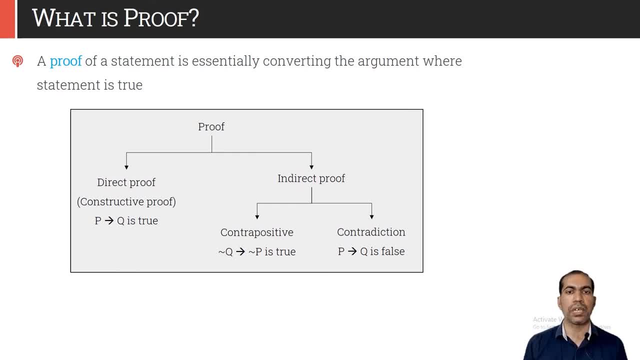 examples and will prove that the proposition Q is also true. So a constructive proof is a proof that directly provides a specific example to prove the given statement. In contrapositive, we are negating the given, both the propositions P and Q, and we are also 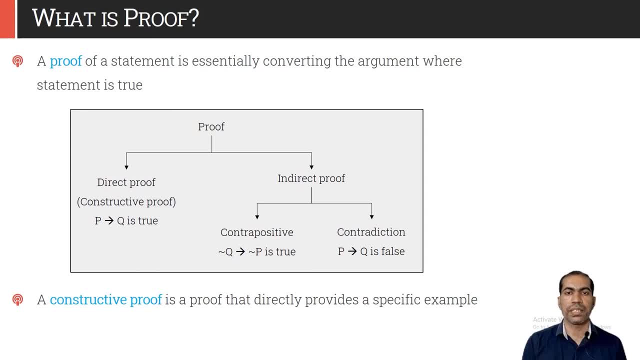 reversing the sign of implication. So basically we are trying to prove negation Q implies negation P is true. The contrapositive of a given statement is same as the statement itself. So if negation Q implies negation P is true, Then we can say that P implies Q is also true. 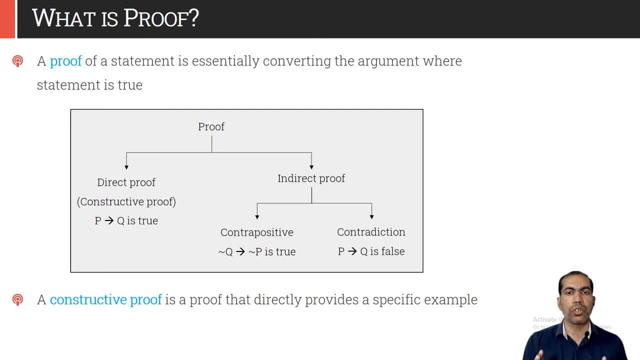 In contradiction method, the statement that we want to prove or the hypothesis, we will assume that it is wrong and we will try to prove its consequences, or we will try to come to the conclusion- which would not be possible, and hence it will be proved- that, whatever assumption we have made initially that our hypothesis is false, the statement itself is: 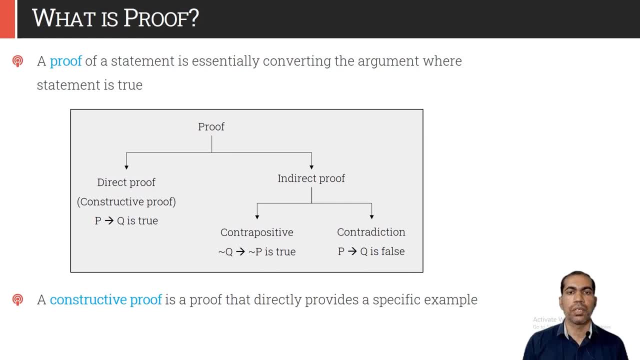 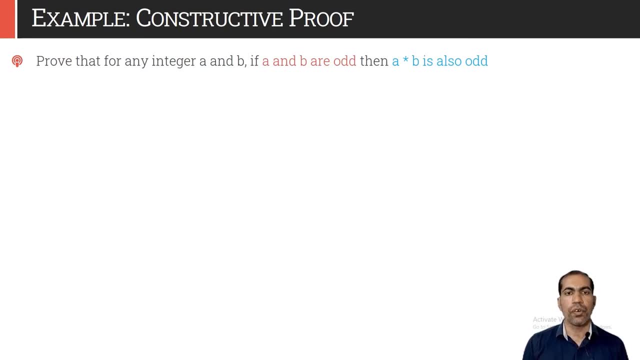 contradicting and hence the given statement would be true. So in this particular video we will be talking about constructive proof. Consider the example. prove that for any integers a and b, if a and b are odd, then a into b is also odd, As we can see that the statement is in the form of: if something, then something. 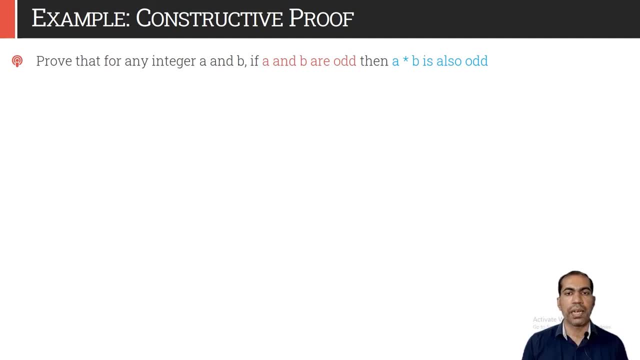 So the if and the condition is known as the hypothesis and the latter part is known as a conclusion or the consequences. So If the proposition P we have is a and b are odd, we will assume that P is true and based on that we will try to prove the conclusion, or we will try to prove that statement Q is. 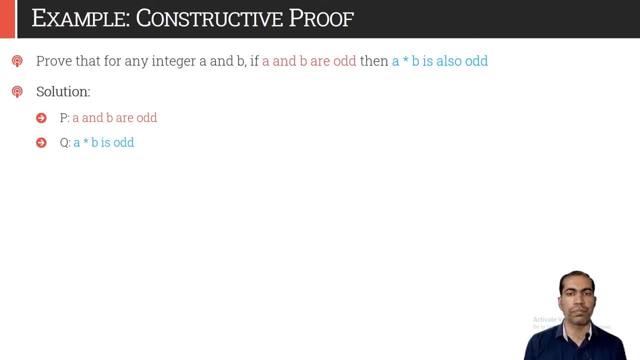 also true, or the proposition Q is also true. So let us start with the P. P says a and b are odd, so we can consider that a is equal to 2x plus 1. if we multiply any integer x with 2, then that would be definitely even. 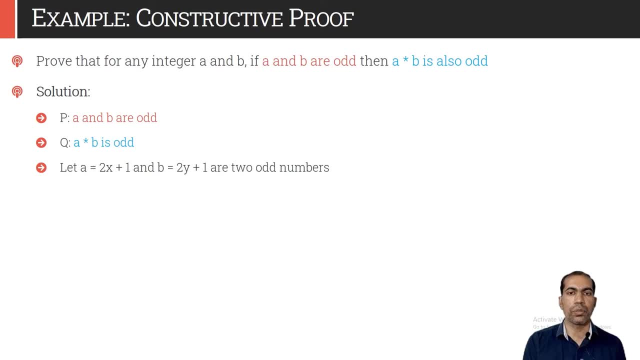 number. So 3 into 2 will be 6, 4 into 2 will be 8, 5 into 2 will be 10. so whatever may be the value of x, if we multiply it with 2 that will definitely be even number and plus 1 will make it odd. 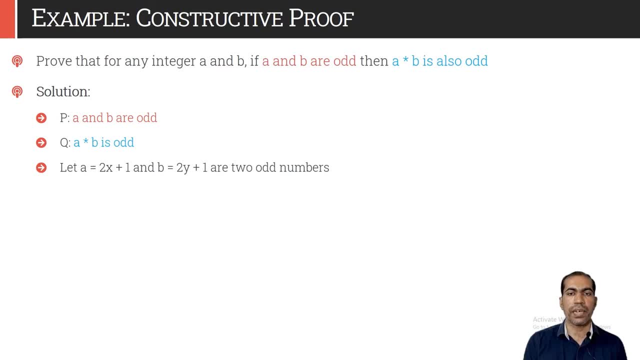 P says that a and b are odd. so we are considering: a is equal to 2x plus 1, so definitely it is odd, and b is equal to 2y plus 1.. Now with this We will try to prove the conclusion. 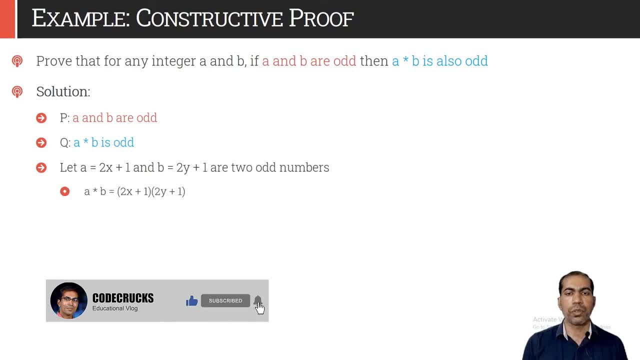 So We will try to prove that Q is also odd because we will put this value into our conclusion part. that is a into b. so a into b would be 2x plus 1 into 2y plus 1.. Let us multiply these two entities so we will get 4xy plus 2x plus 2y plus 1. 2 is common. 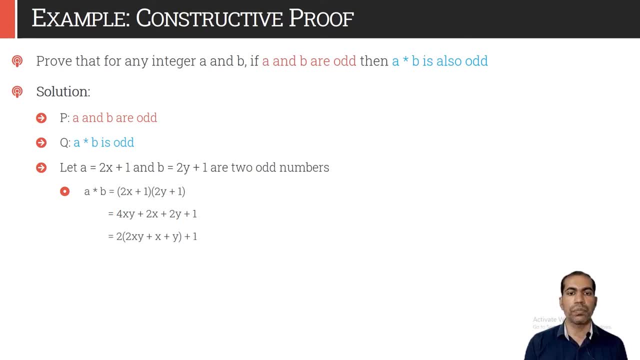 in first three terms, so we can rewrite it as a 2 into 2xy plus x plus y plus 1.. The inner term 2xy plus x plus y would be some value. let us call it as a capital M, so that would be 2 into M plus 1. anything which is multiple of 2 is obviously even number. 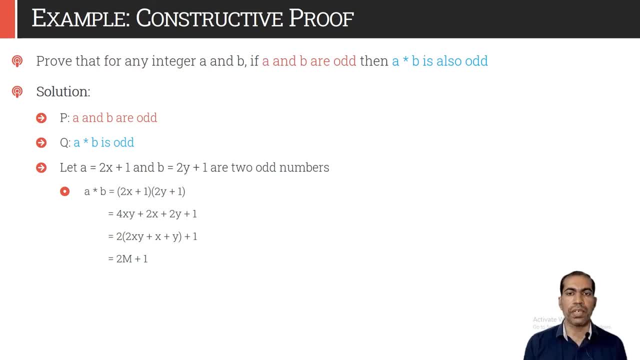 and plus 1 will make it odd. so ultimately, 2m plus 1 is odd and hence a into b is odd, because we have started with that a into b. so our claim or the statement is true that if a and b are odd, Then a into b is also odd. so this is how constructive proof is working. 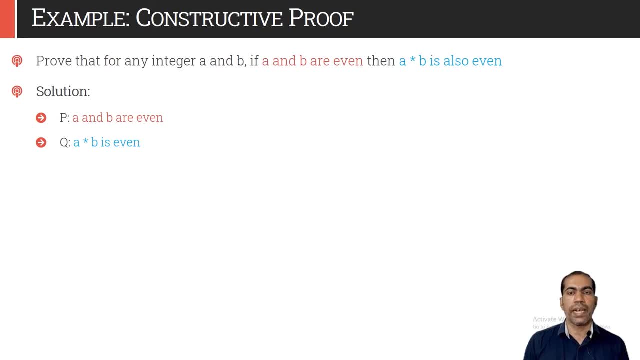 Let us take one more example. prove that for any integer a and b, if a and b are even, then a into b is also even. so here our proposition: P is what the hypothesis part, that is, a and b are even, and the conclusion is Q, that is, a into b, is even. 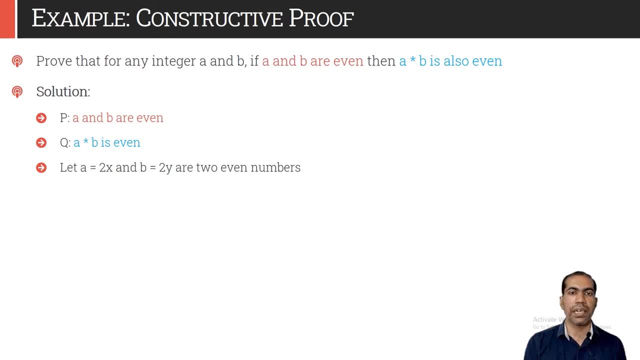 So If a and b are even, they are definitely multiple of 2. so we are assuming that a is 2 into x. so irrespective of any value of x, a is always going to be even as it is a 2x and similarly b is equal to 2y is also even. so we have assumed that P is true, that is, a and b are even with. 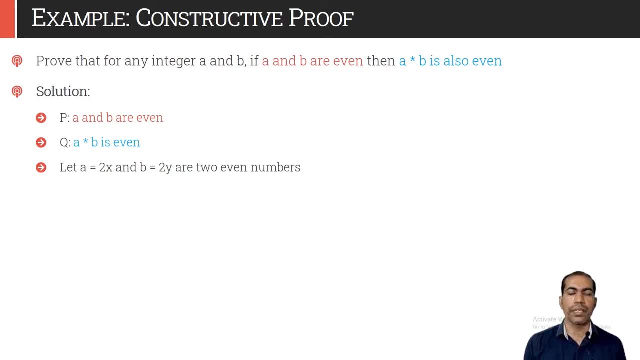 that assumption we are starting. now we try to prove that Q is also true. that is, a into b should be even. So let us put those values of a and b in the equation a into b, so that would be 2x into 2y. 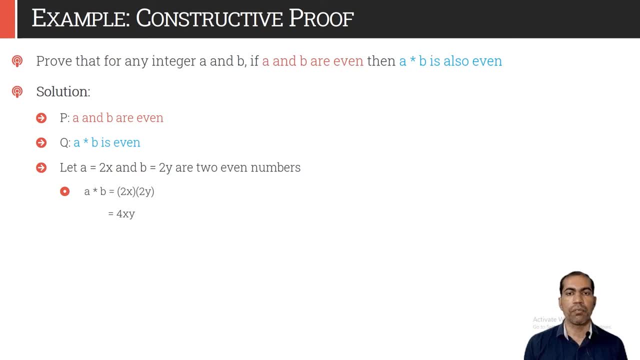 Multiply them and it will make it 4xy. we can rewrite it as a 2 into 2xy. 2xy will be some number, so we are replacing it by M, so this term would become 2M. Now anything multiple of 2, that is definitely even and hence a into b would be even. 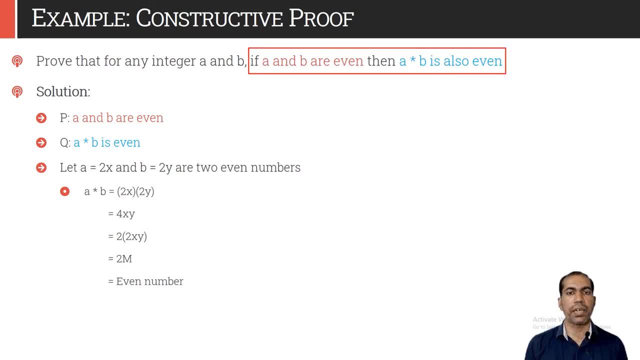 So our statement- if a and b are even, then a into b is also even- has been proved. consider that for any x which belongs to set capital z, if 7x plus 9 is even, then x is odd. so the statement is of the form: if p then q, it means p implies q. so if p is true, then q should be true, that is, if 7x plus. 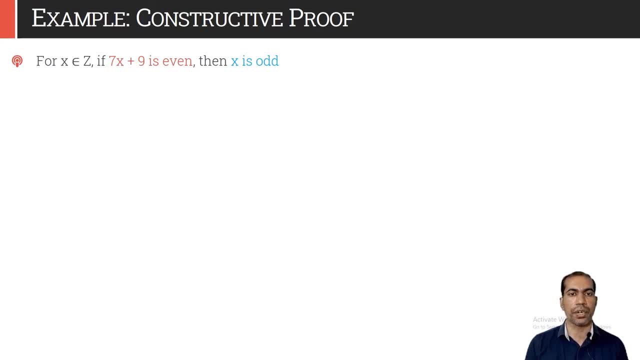 9 is even then, definitely x is odd, that we need to prove. so our proposition p is what? 7x plus 9, which is even so as it is, even that will be equivalent to 2a, multiple of 2, some number multiple of 2. so we are assuming that 7x plus 9 is equal to 2a. we want to calculate what is the. 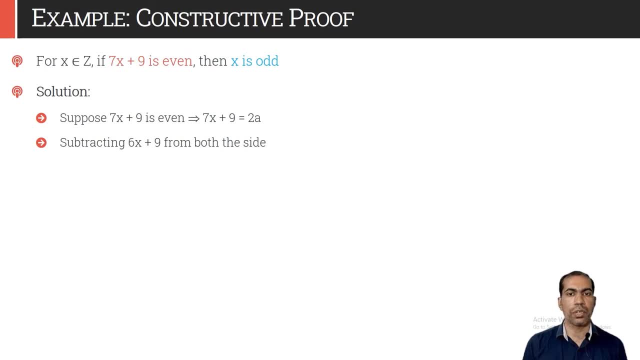 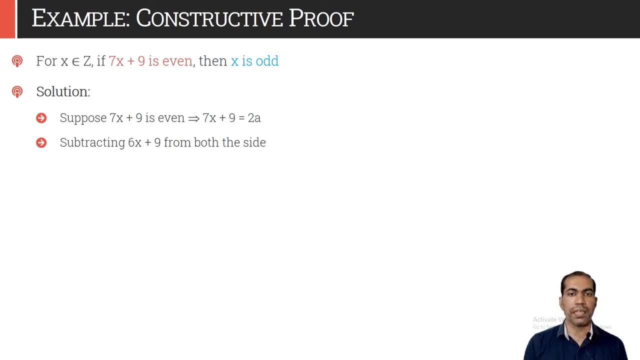 9 is equal to 2a. we will simply subtract 6x plus 9 from both the side. so 7x plus 9 is equal to 2a will be 7x plus 9 minus 6x minus 9 is equal to 2a minus 6x minus 9, from both the side we are. 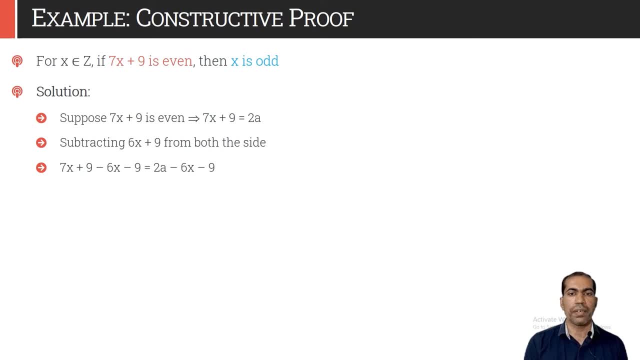 subtracting 6x plus 9. so on left hand side this 9 and this 9 will be cancelled out. 7x minus 6x would be x, so we will be left with x is equal to 2a minus 6x minus 9. minus 9 we can rewrite as minus 10 plus 1, so entire. 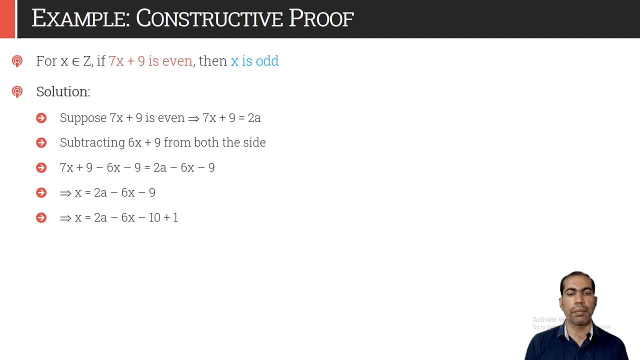 equation would be: x is equal to 2a minus 6x minus 10 plus 1. first three term in this equation are even, so we can take two common out of them. so it will reduce to: x is equal to 2 into a minus 3x. 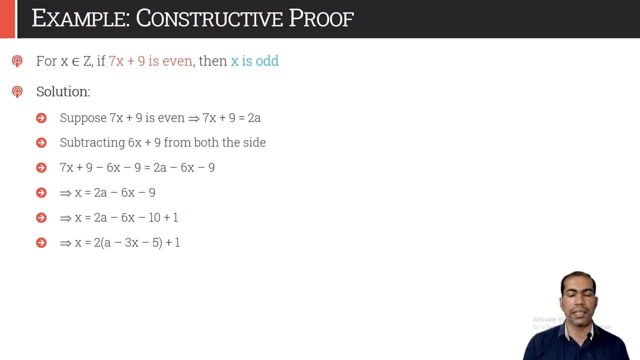 minus 5 plus 1.. the inner entity a minus 3x minus 5 will reduce to some number. let us call it as a m, so we will have: x is equal to 2m plus 1. 2m is obviously even because it's a m is multiple of 2 and plus 1 will. 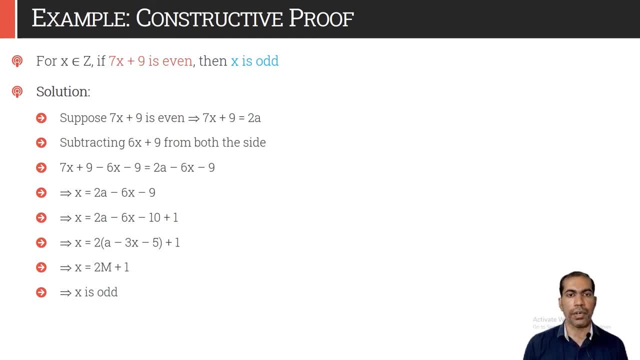 make it odd. so you can see that x is equal to odd. so we have started with the assumption that 7x plus 9 is true. that means p is true and we have proved that x is odd. that is q is also true. So that's how constructive proof goes. 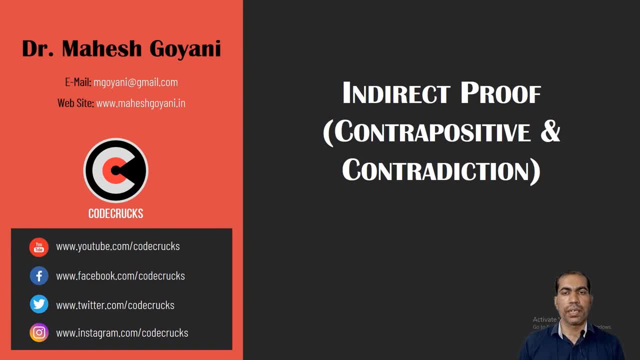 Hello folks, welcome to Code Crux. This is Mahesh Guhani, and in this video I'll be talking about indirect proof techniques. In previous video I have talked about direct proof techniques, under which we have discussed constructive proof method. The link of that video is given in description box. 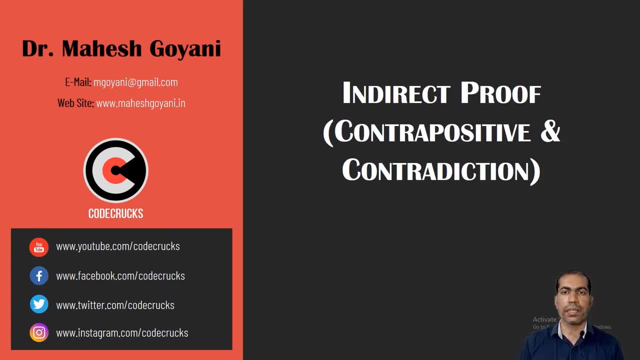 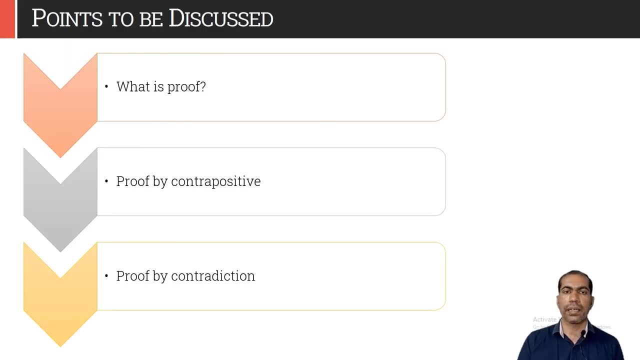 So if you have any doubt regarding direct proof method, then please go and watch that video first. In this particular video, I'll be targeting, or I'll recap, what is the proof, what are the different types of proof techniques and, specifically, I'll be talking two methods of indirect proof. 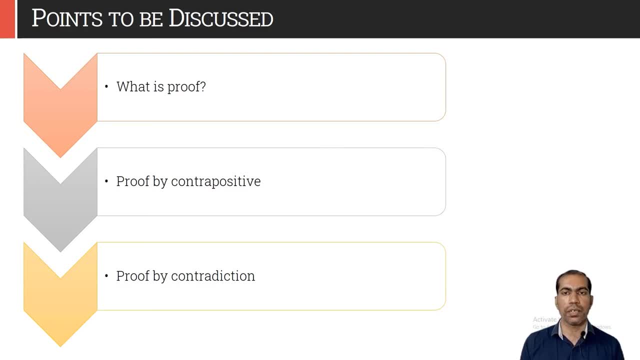 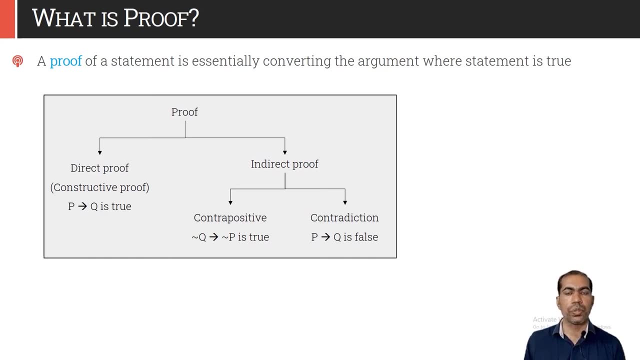 that is contrapositive proof and the contradiction method of the proof. A proof of statement is essentially converting the arguments where statement is true. A statement is given and we will make some logical steps to prove that given statement is true, So that sequence of logical statement is known as the proof. 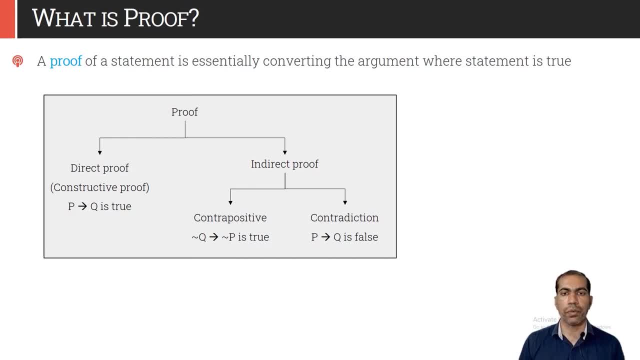 So the proof could be either direct proof or it could be indirect proof. Under direct proof, we have already discussed constructive proof method and in indirect proof we are going to talk about contrapositive method and the contradiction method. Proof statements are normally in form of: if hypothesis, then conclusion. 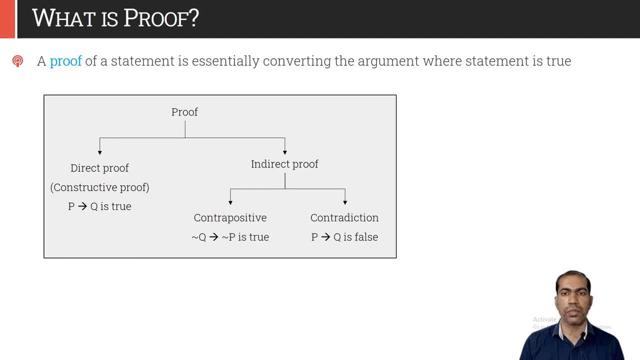 So, hypothesis: we are writing as a P and conclusion: we are writing as a Q. then it would be: if P, then Q. Such statements are represented by the implication, that is, P implies Q and it means that if P is true, then Q is also true. then we can say that given statement is true. 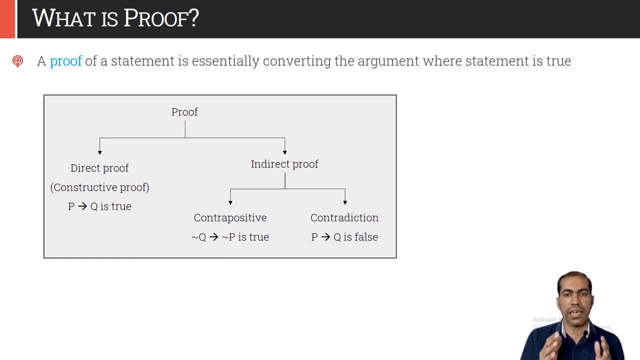 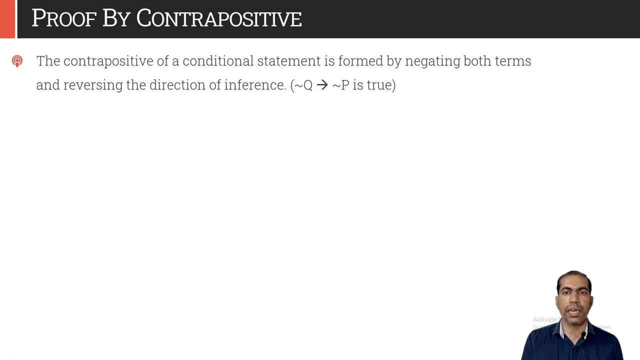 In direct proof or in constructive proof method. we were starting with the assumption that P is true and we are coming to the conclusion that Q is also true. In case of contrapositive method, we are simply negating both the proposition, P and Q, And we are even changing the sign of the implication or direction of the implication. 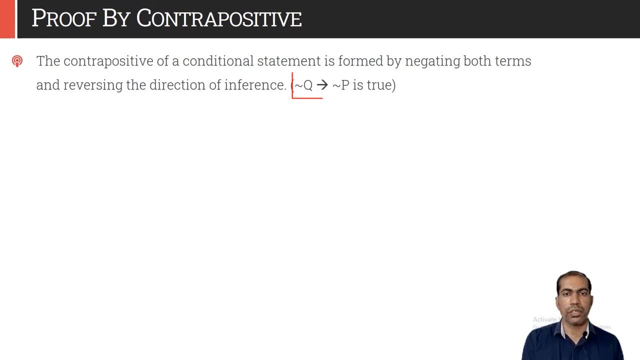 and our new proposition would be now: negation Q implies negation P, and if this is hold, then we can say that the given statement has been proved or the given statement is true. A statement and its contrapositive are logically equivalent. that means P implies Q is same. 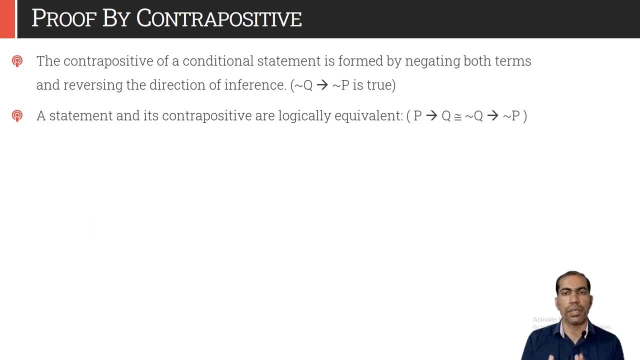 as negation Q implies negation P. So even if we are proving That Negation Q implies negation Q, that means that we have proved P implies Q. Propositions are often in the form of: if P, then Q. In case of contrapositive, we will start with negation Q and we will assume that negation. 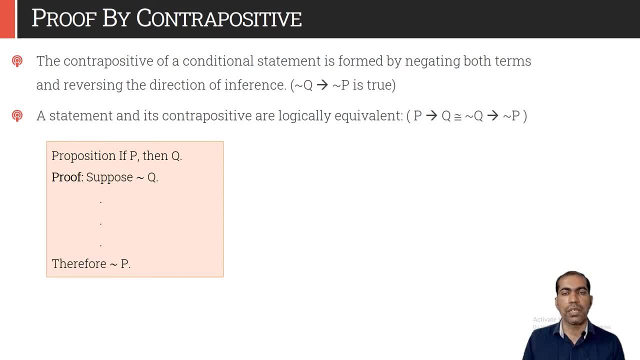 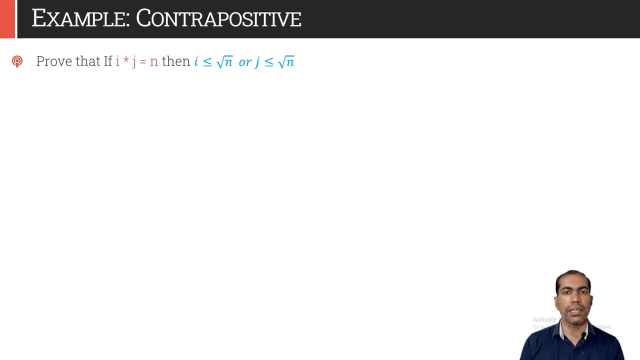 Q is true and by certain logical steps we will prove that negation P is also true. Consider the example. prove that if I into J is equal to N, then I is less than or equal to root N, or J is less than or equal to root N. 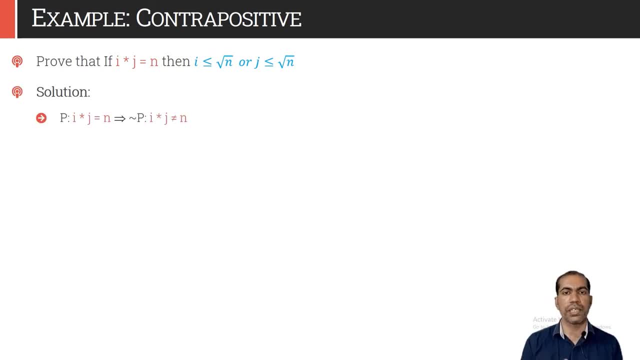 So we have: proposition P is equal to I into J is equal to N, and the negation of that would be: I into J is not equal to N. Similarly, the proposition Q is I less than or equal to root N or J less than or equal. 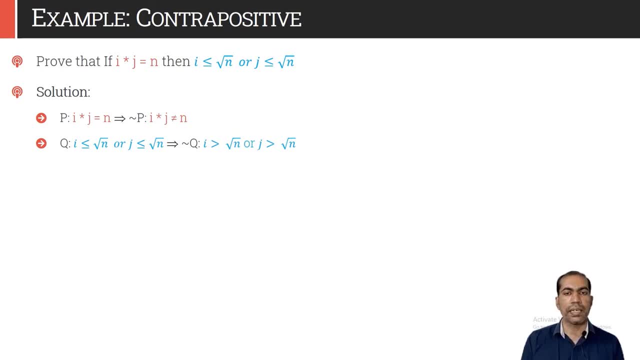 to root N. So the negation of that would be: I greater than root N or J greater than root N, because the contrapositive operation Of Is Equal to, Would be Not equal to, and for less than or equal to, it would be greater than we have to prove. 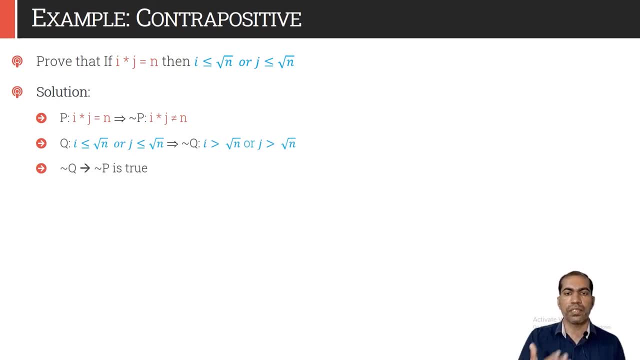 that negation Q implies negation P is true. So we will start with negation Q. Negation Q is having a two part: I greater than root N and J is greater than root N. So first we'll start with I greater than root N. 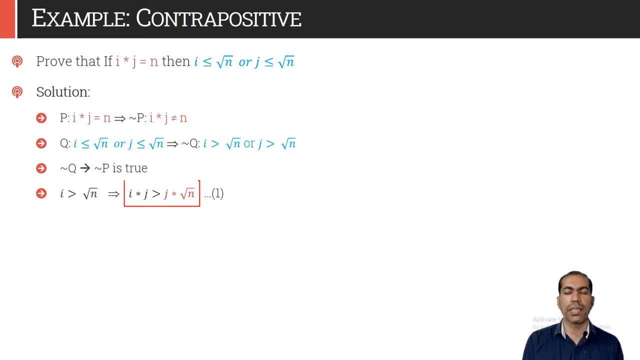 Let us multiply both the sides with J, so we will get I into J is greater than J into root N. Let us call it as a equation number one. The other part of negation Q was J greater than root N, So let us start with that and we will multiply on both the side by root N. 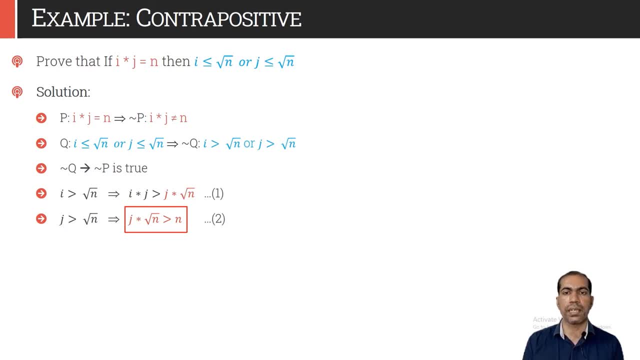 So we will get J into root. N is greater than N. We already know that greater than operation or the greater than relation is having a transitive property. That means if eight is greater than five and five is greater than three, then it implies that eight is greater. 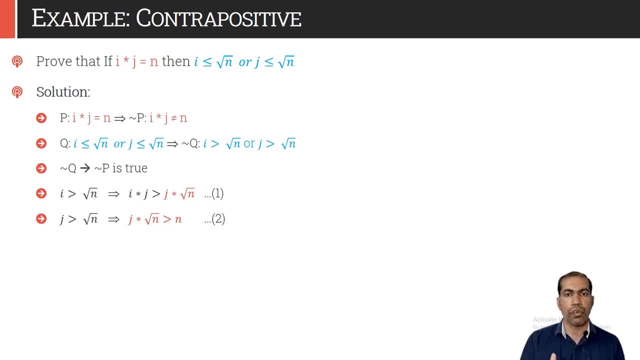 Than three because it is having the transitivity property. So from equation one and two it is easy to derive that I into J is greater than N. from equation one we can say that I into J is greater than J into root N, and from equation two we 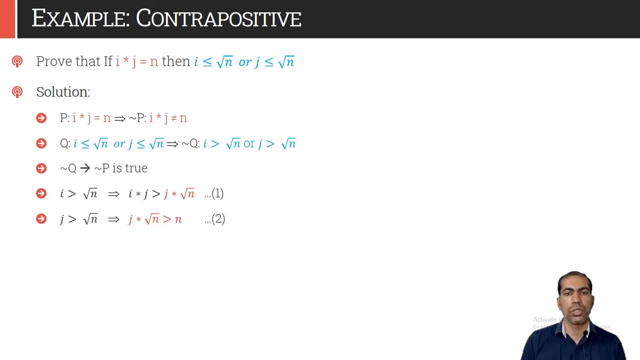 have J into root N greater than N. So by the property of transitivity we can say that I into J is greater than N. So as I into J is greater than N, I into J cannot be N. That means I into J is not equal to N. and 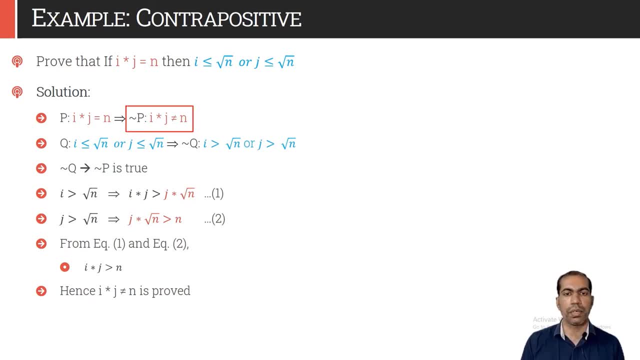 that is what we wanted to prove, That is, the negation P. I into J is not equal to N. So, as you can see that we have started with the negation Q and we have proved the negation P as well, That means the given statement is true or it is proved. 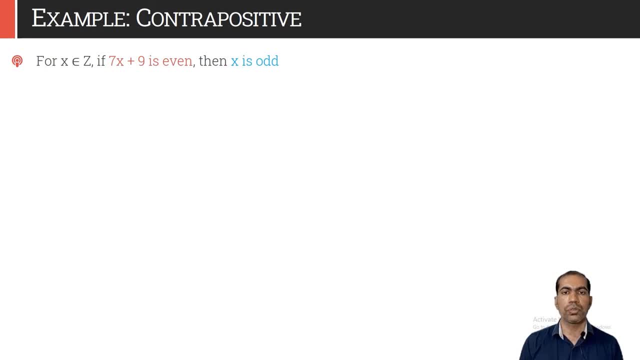 Consider another example, For X belongs to set capital Z. if seven X plus nine is even, then X is odd. So it says that if for any value of X which is odd, seven X plus nine should be always even. So this we want to prove. 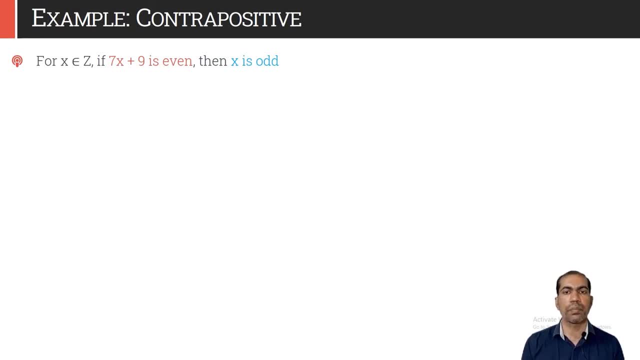 So our statement P would be seven X plus nine and Q would be X is odd. So for P: seven X plus nine is even, its negation would be seven X plus nine is not even. And for the proposition Q, X is odd, Its negation would be: X is not odd. 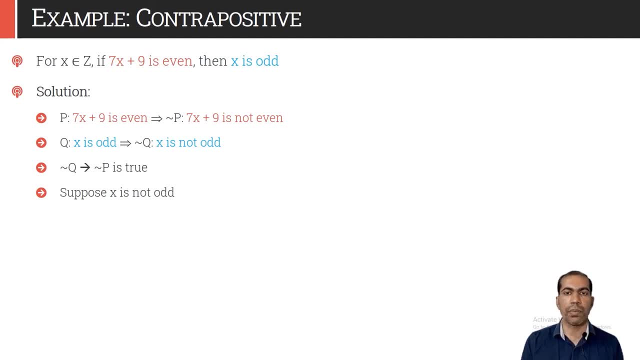 As X is not odd, obviously it is even. there is no other possibility. And if X is even, it will be definitely multiple of two of some number. So X we can consider as a two. A- Let us put this value into our proposition. P, seven, X. 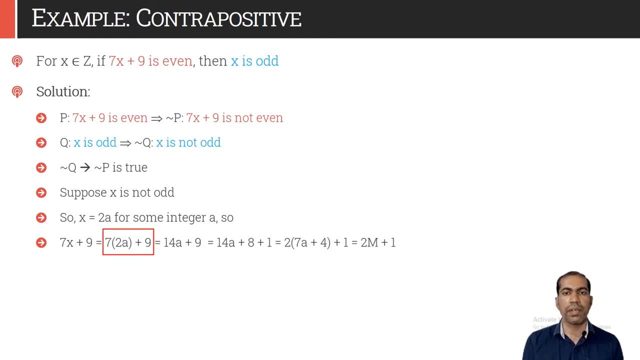 plus nine. So seven X plus nine would be seven, into two A plus nine. by multiplying seven with two A, It will be fourteen A plus nine. We can rewrite nine as eight plus one, So this will become fourteen A plus eight plus one. 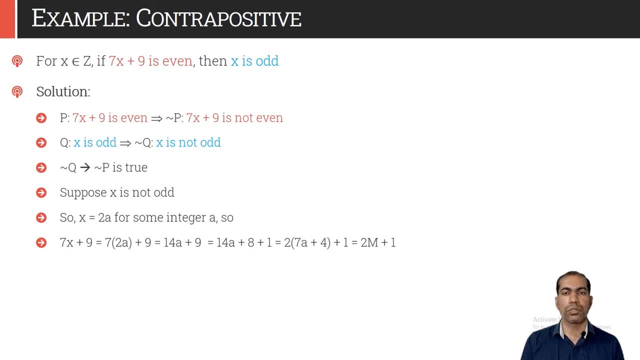 From the first two terms we can take two common out. So that would be two into seven A plus four plus one. Seven A plus four will reduce to some number. Let us call it as a M. So we will have a two M plus one, and M is a multiple of two. 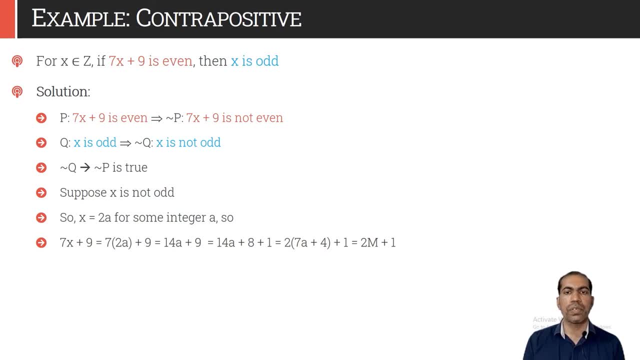 So this two M Will be definitely even and plus one will make it as a odd. So that says that seven X plus nine is odd, and seven X plus nine is odd. It implies seven X plus nine is not even, And that's what we wanted to prove. 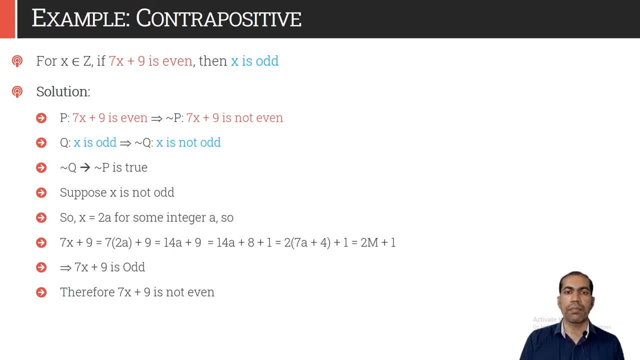 That is our negation P statement. So, as you can see, that we have started with X is not odd, and we have proved that in that case, seven X plus nine is not even. So, negation Q implies negation P is true, And hence the original statement. 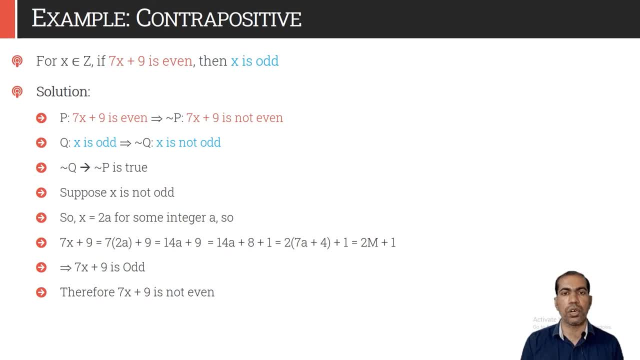 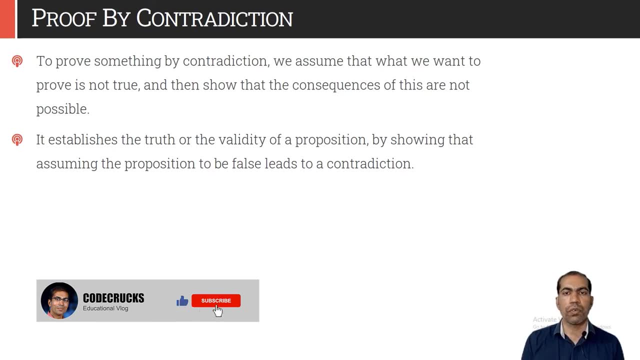 Seven, X plus nine is even then X is odd is also true In contradiction method. to prove something by this method, we are assuming that whatever we want to prove is not true and we will try to prove the consequences. but that would not be possible and hence our original assumption would be false. 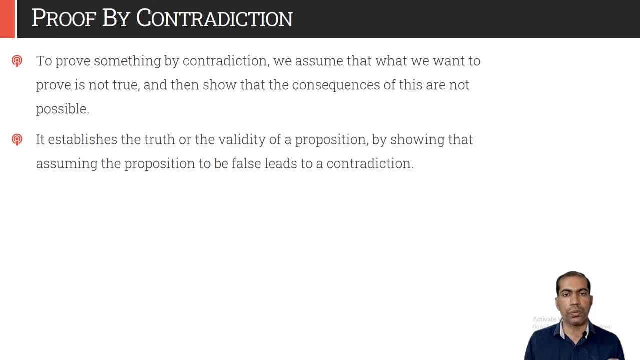 So we will assume that P is not true and we will try to prove the Q, but that would not be possible and hence we will assume that P is also Q. It establishes the truth or the validity of a proposition by showing that assuming the proposition to be false leads to the contradiction. 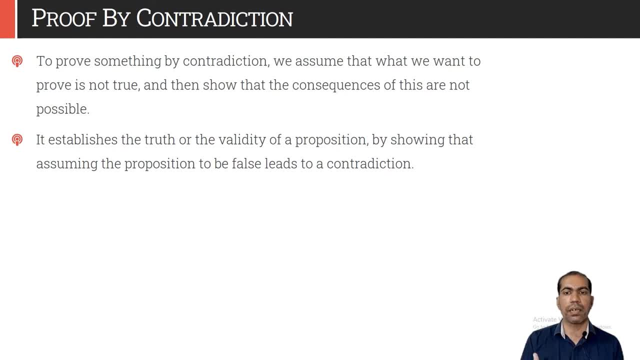 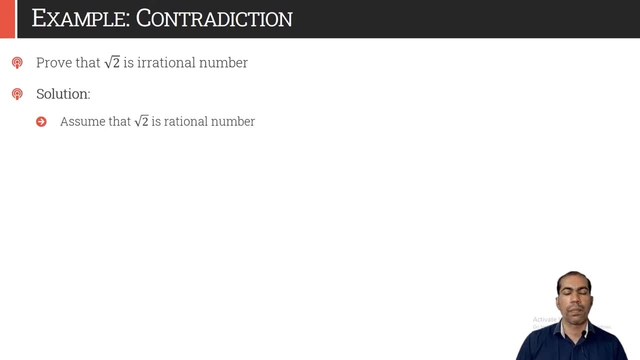 So whatever assumption we are making initially, that our hypothesis is false, will definitely not be the true. It will be contradicting with our assumption. Let us take the example: prove that root two is irrational number. Rational number is a number which can be represented by X. 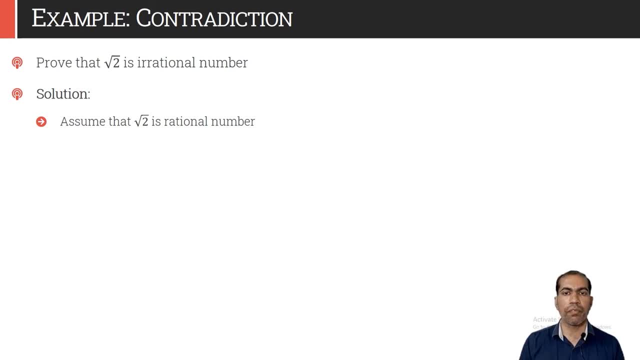 Upon Y, where X and Y do not have any common factor. So if I consider twelve, then twelve is equal to twenty four by two. So this is not a rational number, because twenty four and two has common factor two. So twelve is not a rational number. 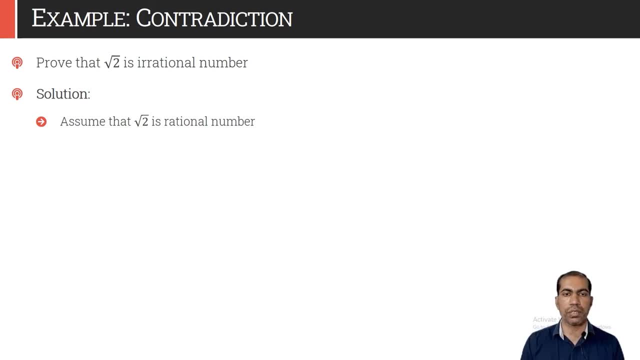 So, in contradiction, we will start with the inverse assumption. The statement we want to prove is what root two is irrational number. So we will start with the contradiction of that- That root two is rational number- and we will try to prove that this assumption is actually. 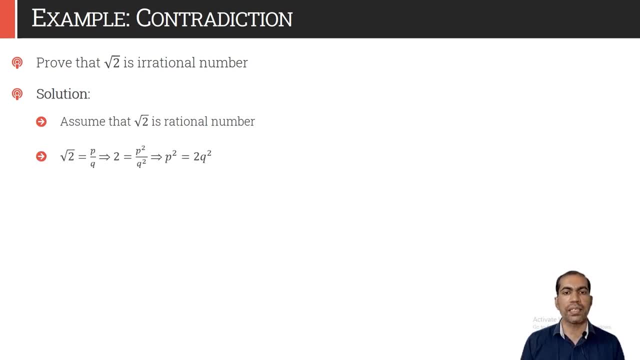 wrong and hence our claim is true. So, as it is a rational number, we can always write it as a P by Q, where P and Q will not have any common factor. By squaring on both the side we will get: two is equal to P square by Q square. 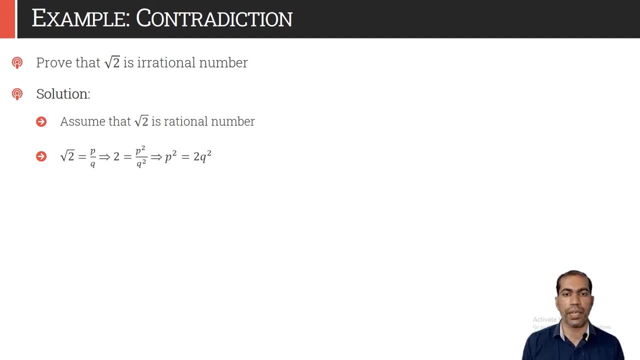 Simplifying it, we will get: P square is equal to two Q square. As P square is multiple of two Q square, We can say that P is even and, as it is even, we can assume it as a two K, because it's an even number. 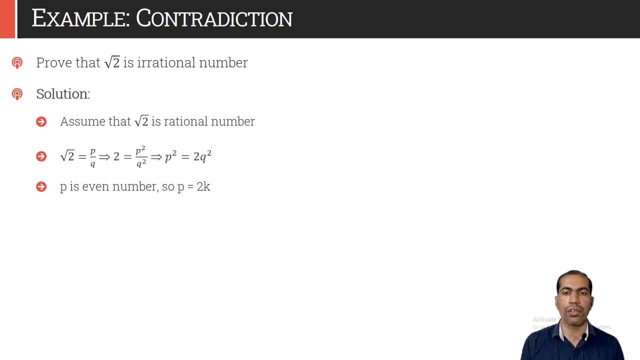 So multiple of two would be even, irrespective of any value of K. So let us put: P is equal to two K in this equation, So we will get: two K square is equal to two Q square. By squaring this term we will get four K square is equal to two K square and that will imply: 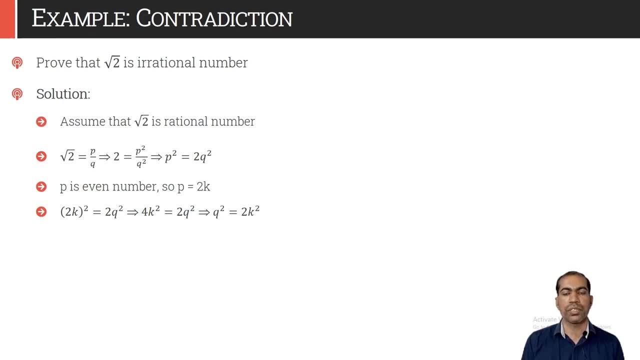 that Q square is equal to two K square. So this statement will tell us that Q is also even Because Q is equal to two K square, Because Q square is multiple of two, So Q is also even number, So P is even. 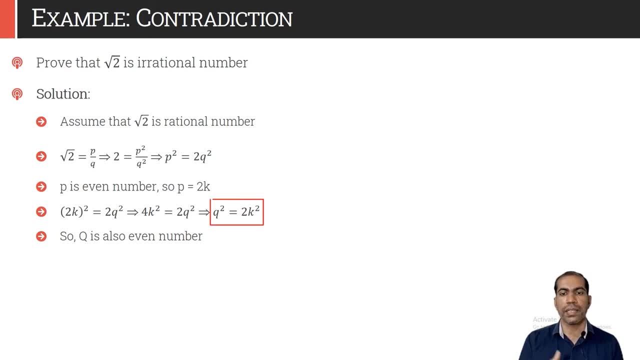 That we have proved from this statement. Q is even. That we have proved from this statement. Thus, P and Q, both are even numbers, So they have common factor, and which contradicts to our assumption that root two is a rational number. If root two would be rational number, then it won't be possible to write it in the form. 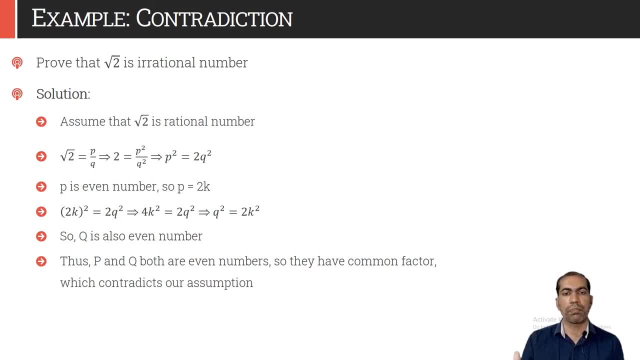 of P by Q, Such that P and Q Both have common factors. So our assumption is false that root two is a rational number and hence our claim will hold that root two is irrational number. Let us consider another example: Prove that P union Q is same as Q union P. So we will start with the contradiction of. 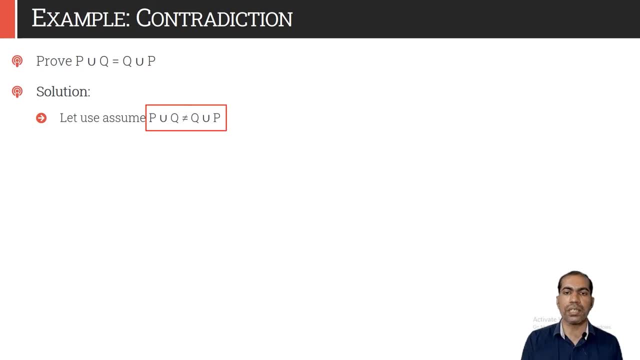 that and we will assume that P union Q is not same as Q union P. It means the elements which are present in P union Q Are Not same as all the elements which are in Q union P. If we consider one by one all the, 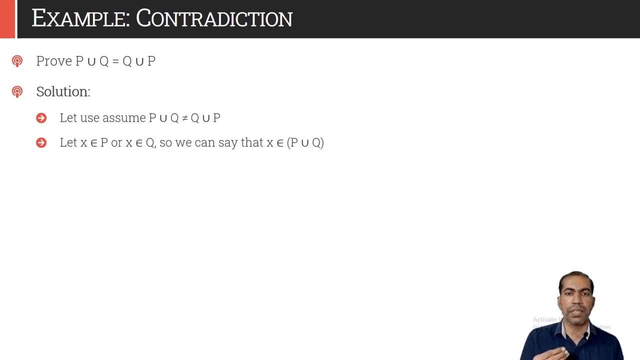 elements from P union Q and if we test the membership of that element, X, So that X would be definitely either in P or in Q and then we can say that X is a member of P union Q. If we select Q union P and if we test all the element, then definitely again the X would. 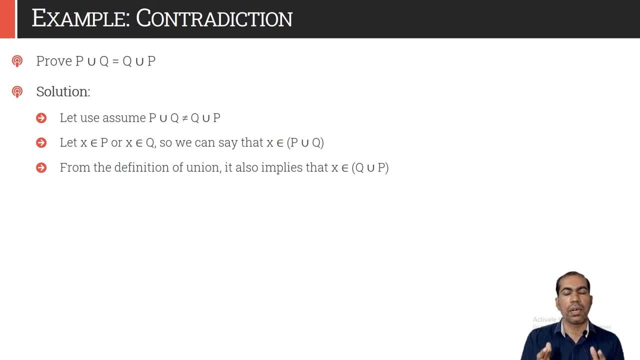 be either in P or in Q, And hence By the definition of union itself, it has been proved that all the elements of P union Q are same as elements in Q union P, And hence our assumption is wrong that P union Q is not same as Q union P. Fine. 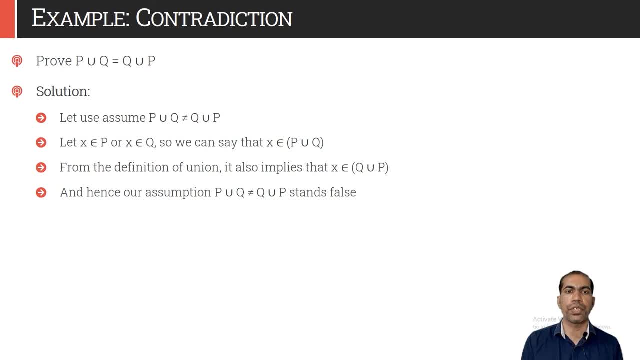 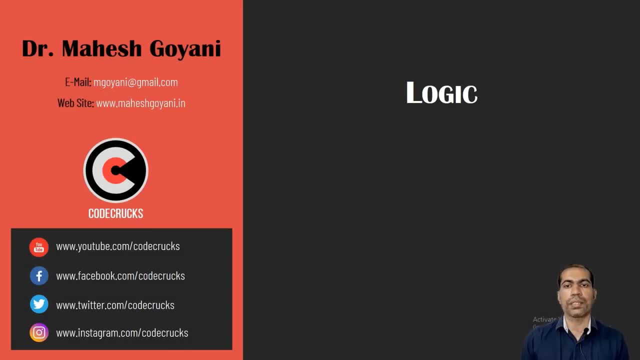 This assumption is wrong. It means our original claim is true, That is, P union Q is equal to Q. union P has been proved. Hello folks, Welcome to Code Crux. This is Mahesh Guyani, And in this video I will be talking about logic. 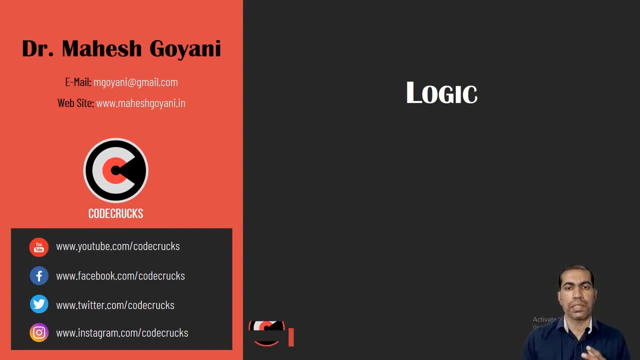 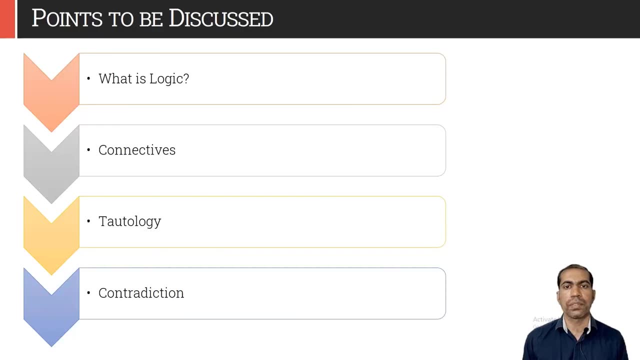 In previous two videos we have talked about proof techniques: The direct proof method and the indirect proof method. The link of those videos are given in the description box. In this video I will be talking about what is logic. We will also talk about various connectives to join different propositions and to make 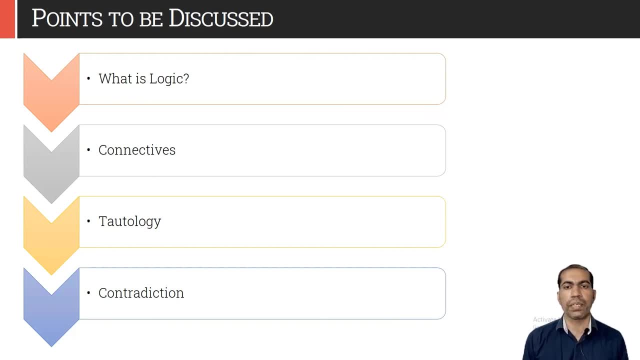 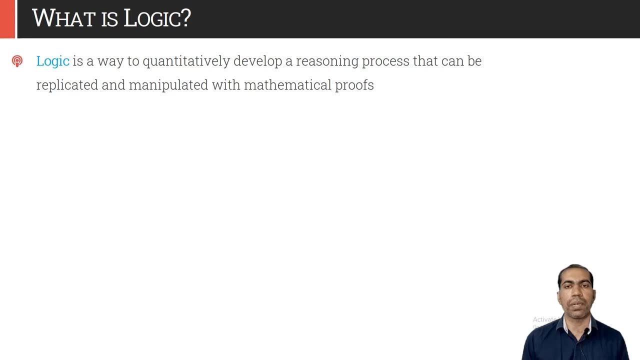 a compositional proposition That will be followed by the concepts of tautologic and the contract logic. So let us get started. Let us begin. Logic is a way to quantitatively develop a reasoning process that can be replicated and manipulated with mathematical proof. 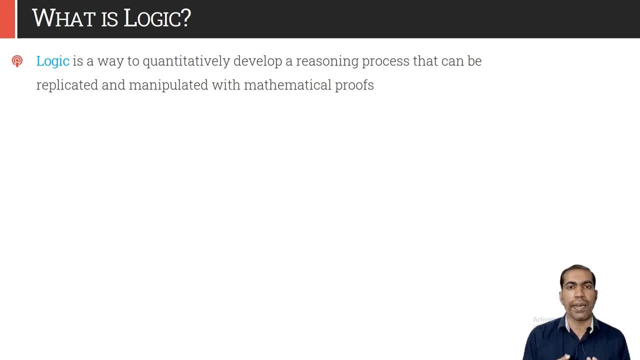 So logic is a sound inferring method where we are writing some mathematical steps to infer something And we can prove that whatever logic we have developed, that will be true for all the valid inputs. So this logic is a framework for the n factorial. So human brain will start thinking that what steps we should follow to compute the n factorial? 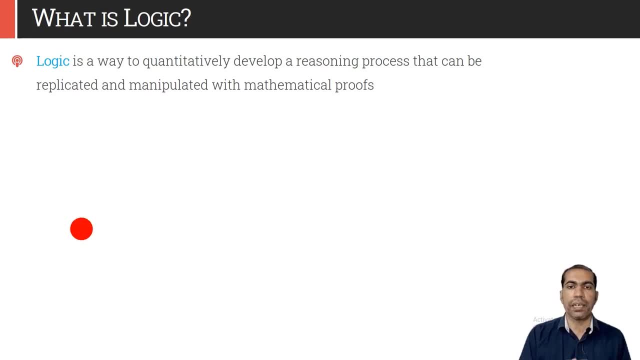 So first we are initializing variable f is equal to one. Then we are iterating a loop from i is equal to 1 to n. Within that loop we are writing that f is equal to f into i. So this thinking process, that how particular problem can be solved, is known as the logic. 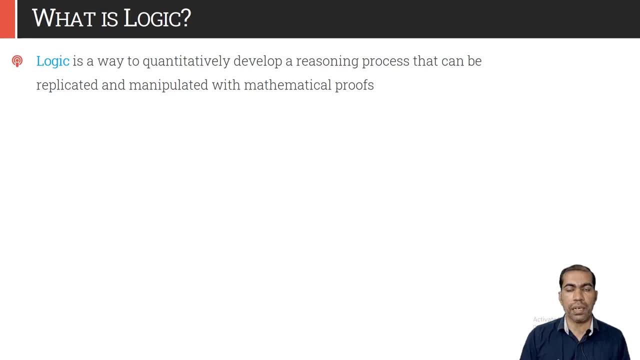 given. by writing the mathematical steps, we can come to the expected output. that process is called the logic. from the perspective of human. the logic is the ability of human to reasonably think about something with the help of proper proofs and the inferences whenever an incident happens. human 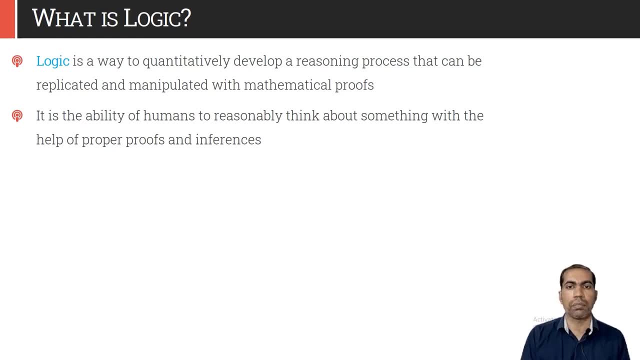 brain will start thinking on the causes of that. that. what could have caused this particular incident? so logically, human brain starts thinking or working on what has happened and what could be the possible cause for that. so that is what the logic is. proposition is a declarative statement. 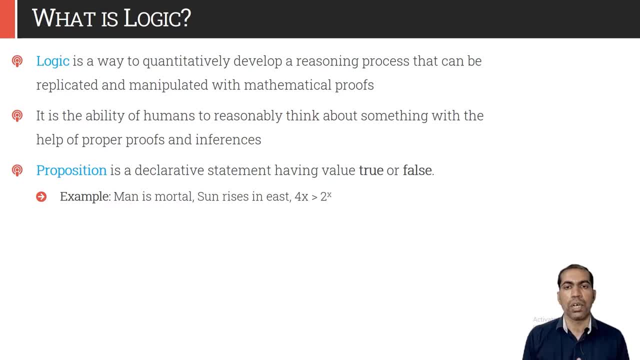 that can either take value, true or the false. no other values are possible for the proposition. it's a simple statement with value- true or the false, and these values are also known as the truth value of the proposition. for example, man is mortal, so this proposition is always true. Sun rises in east, so that proposition is also always true. 4x greater than 2 power. 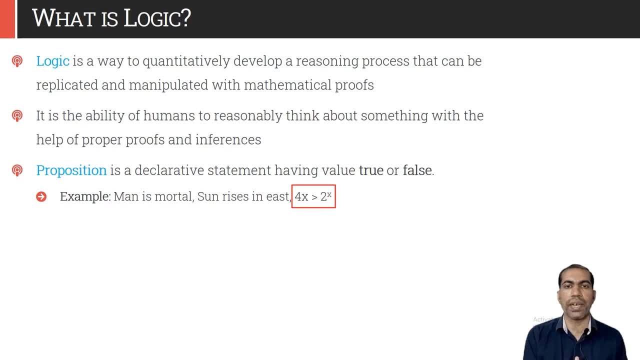 x. so this proposition would be true for certain values of x and would be false for the rest of the values. Answer of propositions depend on the variables involved into that. Such variables are known as the free variables. For example, 4x greater than 2 power x. so this: 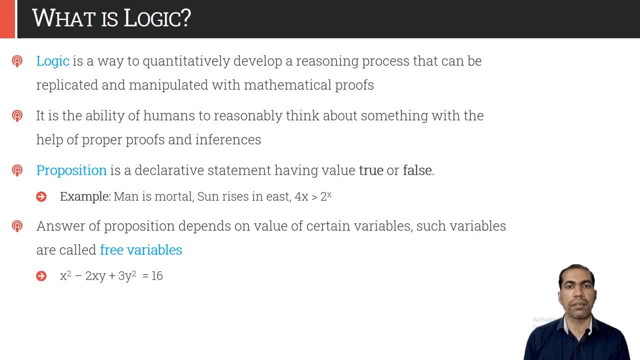 proposition will hold when x is greater than 4.. For x is equal to 2, it would be 8 greater than 4. that is false. For x is equal to 3: it would be 12 greater than 8. that is again false. For x is equal to 4: it would be 16 greater than 16. that is also false. But now, 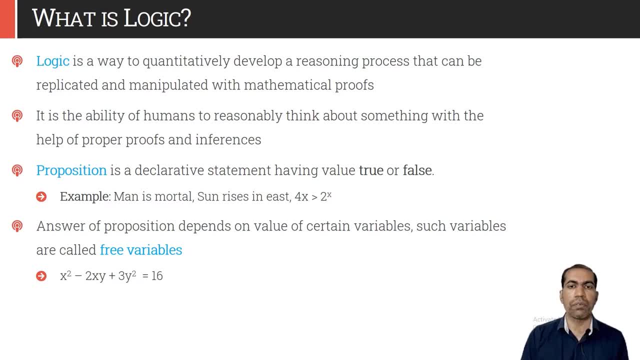 for any value of x greater than or equal to 5, this proposition is going to be true. So x is called free variable 5.. For this proposition, which will determine the truthness of the given statement, Consider another example: x square minus 2xy plus 3y square is equal to 16.. So the truthness of 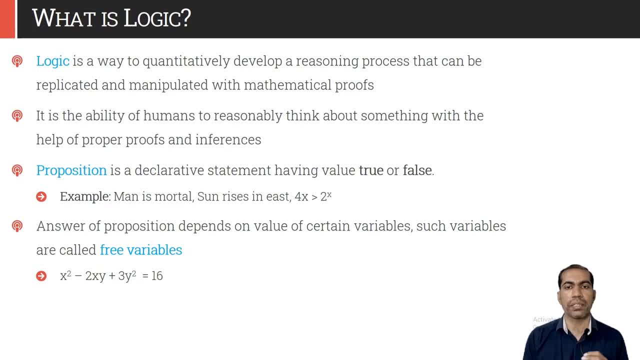 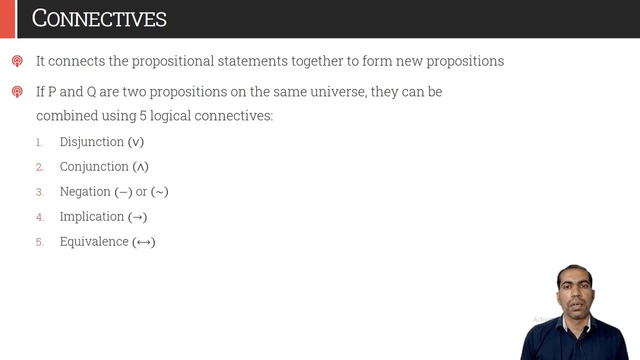 this statement depends on values of the variables x and y. So x and y are the free variables for this particular statement. Given two propositions, p and q, we can combine them with the help of different connectives and we can form a compound proposition. So compound proposition is a combination of individual propositions and these two individual 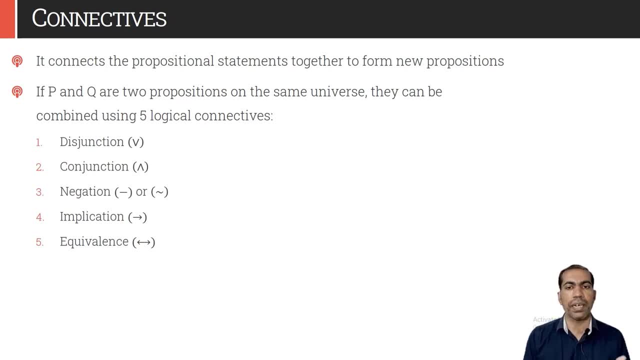 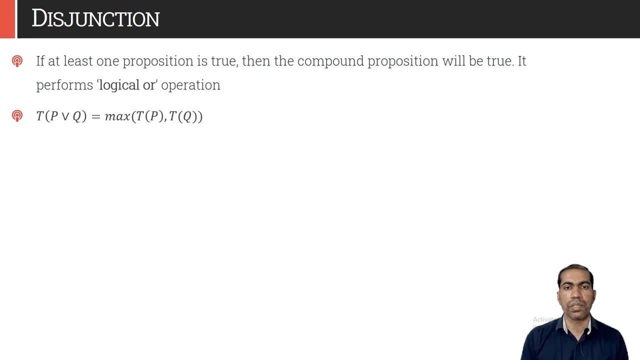 propositions can be connected with the help of different connectives like disjunction, conjunction, negation, implication and equivalence. Let us discuss all of them one by one. When we connect two propositions with the help of disjunction, then the compound statement will have truth value: true. 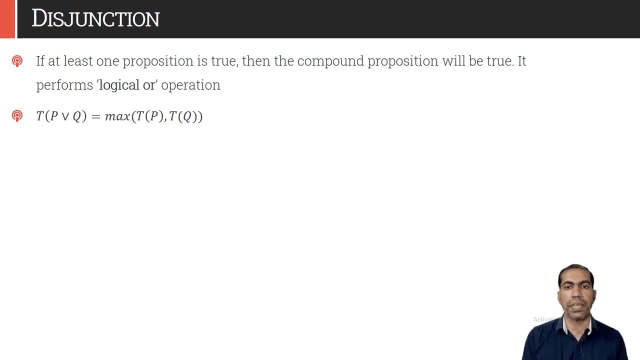 If any one of the proposition is true, assume that p and q are the two propositions and we are connecting them with the help of disjunction, which is represented as p disjunction q. So the truth value of this disjunction or the compound statement is given as max of truth. 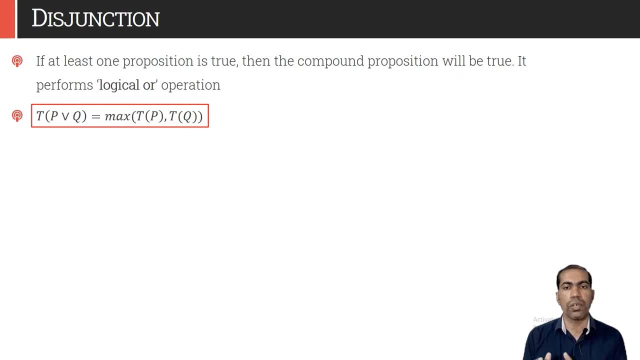 value of proposition p, comma. truth value of proposition q. So basically the disjunction is forming logical OR operation and it says that if one of the proposition is true, then disjunction will have value true. So the truth table for disjunction operation would look like this, where p and q are the two propositions. So there would 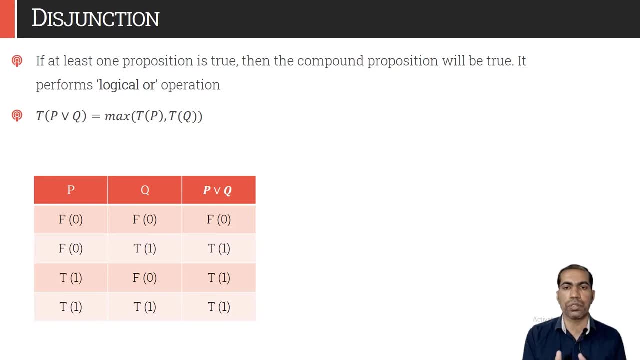 be four different combinations of their truth values: 00,, 01,, 10 and 11.. As disjunction forms the union operation or the logical OR operation when both the propositions are false or they have truth value zero. In that case only p disjunction q is true. So this is a combination. 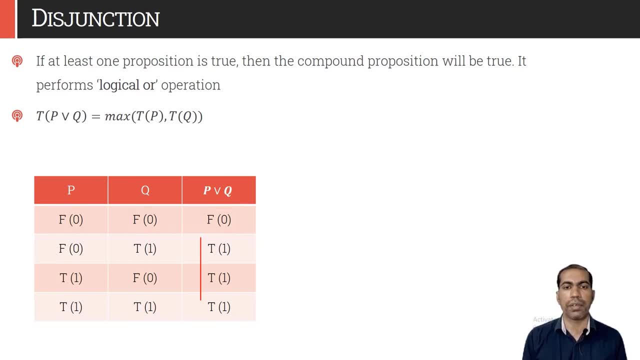 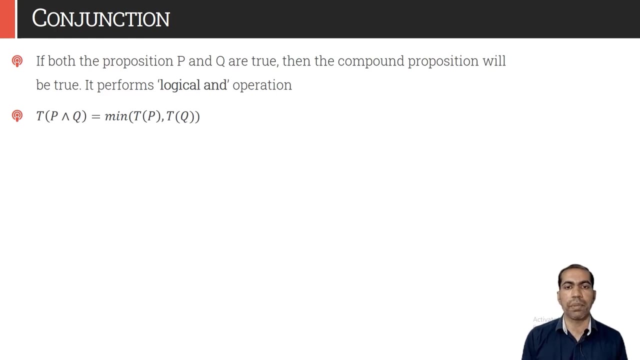 of the two propositions, We will take value zero. otherwise it will have truth value, one that can be easily verified from the table. If we connect two propositions, p and q, with the help of conjunction, then it will form logical AND operation and it is represented by p conjuction q. notation: The truth value of conjunction is given as minimum of truth. 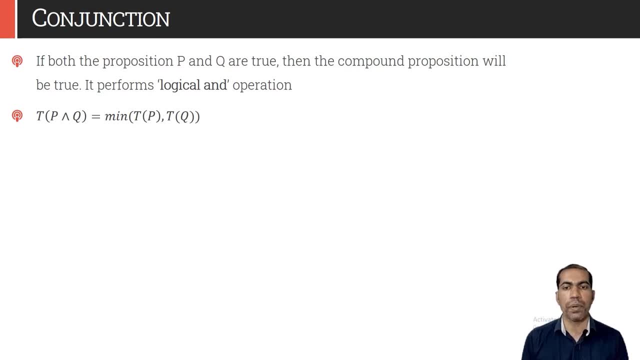 value of proposition p, comma, the truth value of proposition q. Or simply we can say that whenever both the propositions are true, then only this composition will have value. true. If one of the proposition is false or have value zero, minimum of this function would be zero and that would be the truth value of p conjuction q, The truth value. 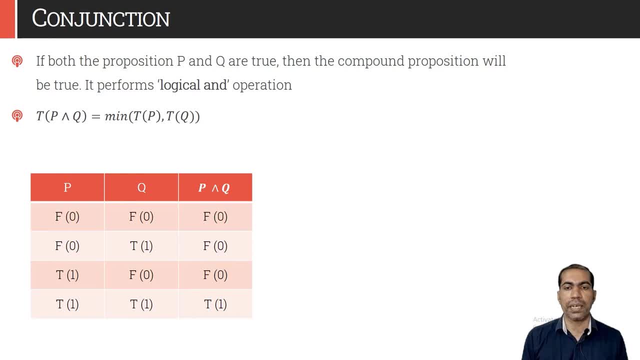 of this operation is as shown below, As you can see, that if any of the proposition has value zero, If any of the proposition is false, the p conjuction q will take zero value and if both are true, in that case only the minimum of t of p comma t of q would be one, because truth value of 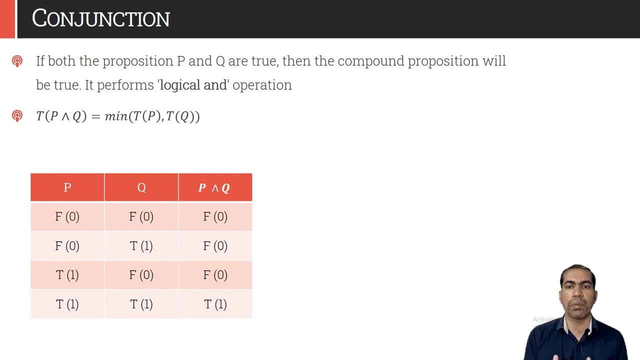 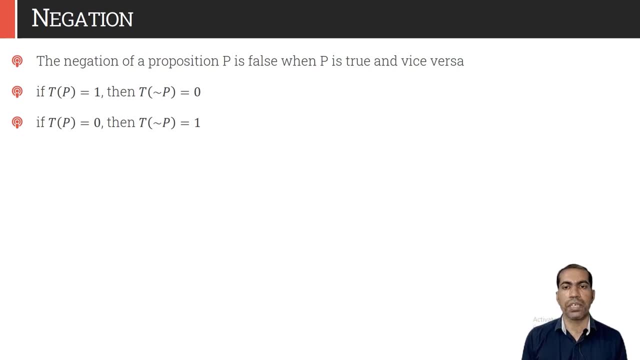 p is also one and t of q is also one, So minimum of that would be one. So this is simply a logical AND operation. The negation of the proposition p is false when p is true, and vice versa, And negation of p is represented by this notation. 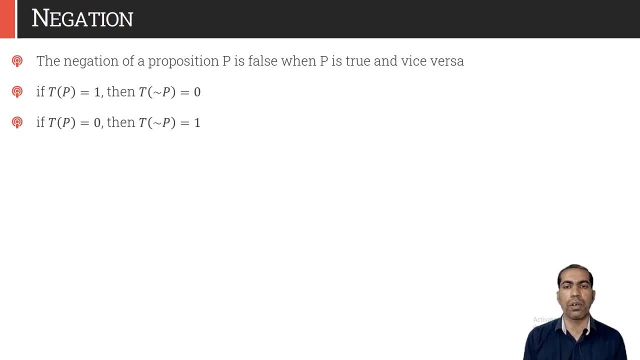 Truth value of p is one implies that truth value of negation p would be zero. and if truth value of proposition p is zero, then truth value of negation p would be one. So that's quite simple. We are simply taking the complement of the truth values of given proposition. 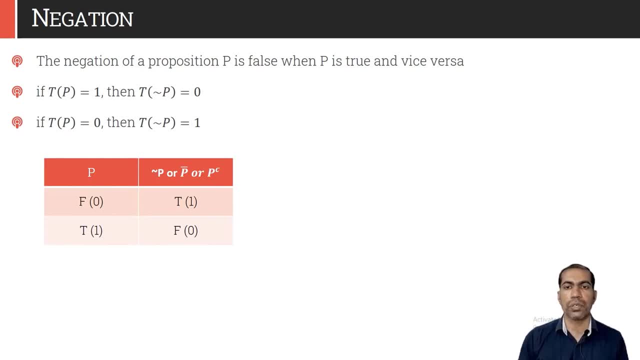 So if p is false, then the negation of p is true. The negation is represented by either hyphen p or p bar or p complement, or sometimes by p dash as well. De Morgan's law is a very good example of the negation. The first law says negation. 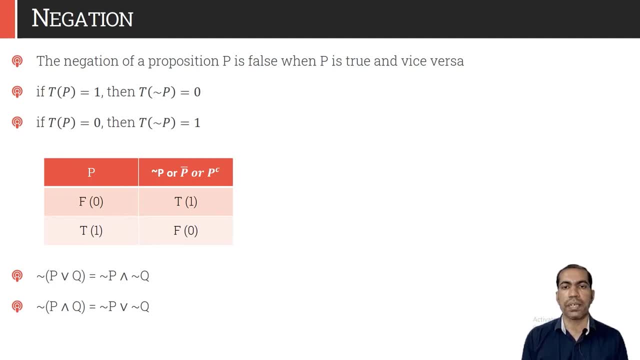 of p disjunction q is same as negation p conjuction negation q. And second law says negation of p conjuction q is same as negation of p disjunction with negation of q. So that simple De Morgan's law that we have already proved with the sets. If you have any doubt regarding de Morgan's, 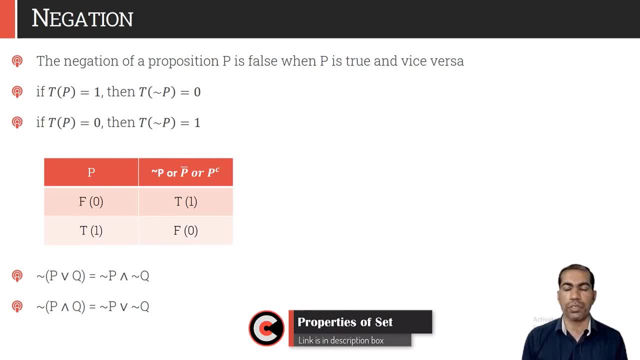 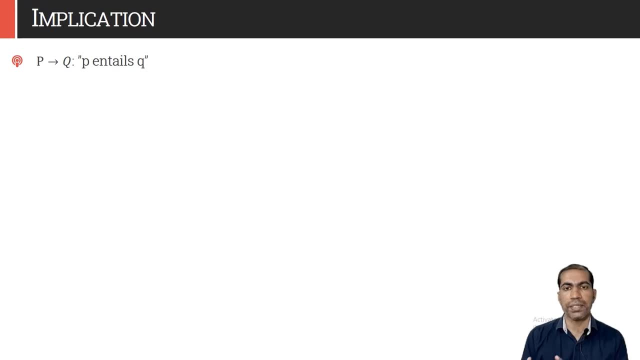 law. then you can watch the previous videos. The link of that video is given in the description box, Implication. it is represented by p implies q and it is read out as p entails q. It is also written as if p, then q. So such kind of rules are typically represented by the 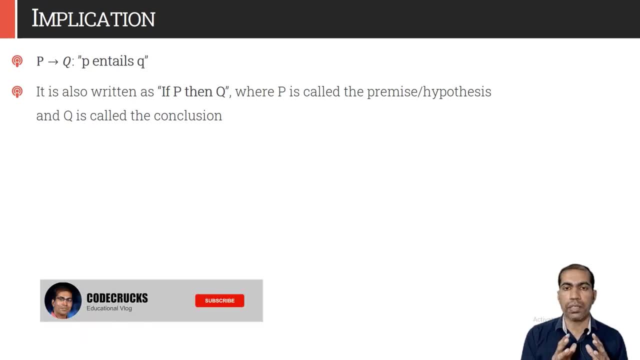 implication operator, where the component or the proposition p is known as a premise or the hypothesis And the proposition q is known as conclusion or the consequences. For example, if you score 90% or above in the subject, then you will get a grade. So here the proposition p or 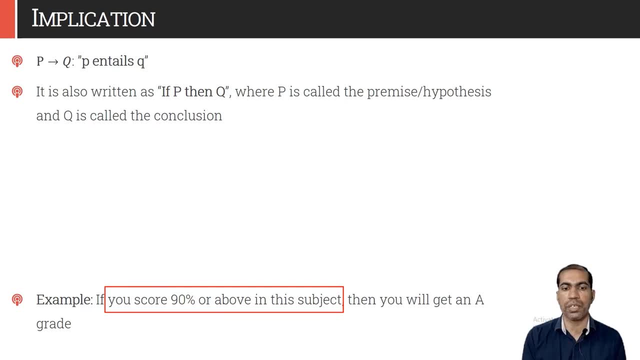 the hypothesis or the premise for this compound proposition is: you score 90% or above. The conclusion or the consequence of that would be that you will get a grade. So this kind of if, then kind of statements are are represented using implication: P entails Q is same as negation of P, disjunction Q and the. 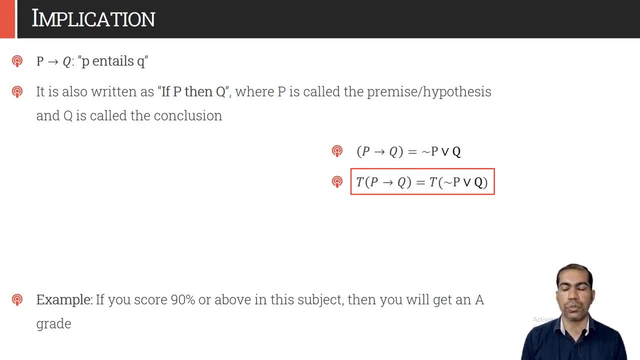 truth value of P entails Q or the P implies Q is given as truth value of negation P, disjunction negation Q. The other way to find out the truth value for P implies Q is this function that that value would be 1 if truth value of proposition P is less than or equal to truth value of proposition. 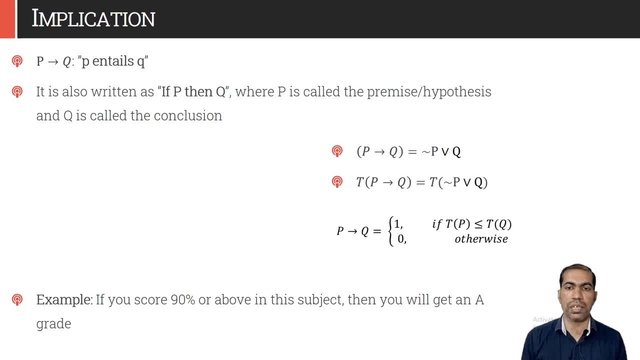 Q and it would be 0 otherwise. So this is just another representation of finding the truth value. Let us look at the table. So, as you can see, for the first row, the truth value of P is less than or equal to truth value of Q and hence the truth value of the proposition- P implies Q- is 1.. 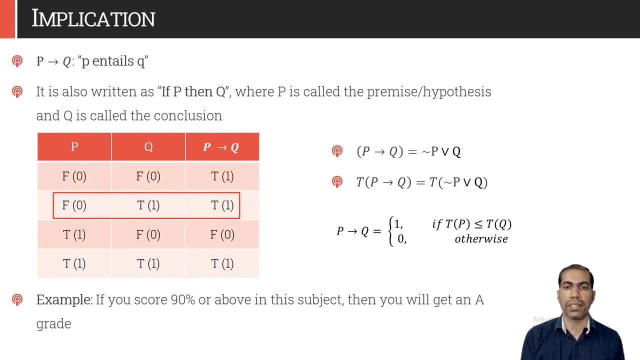 In second row, the truth value of P is again less than or equal to truth value of Q. So the truth value of compound proposition P entails Q is 1.. For third row, the proposition P has value 1, proposition Q has value 0 and for this particular case, P truth value of P less than or equal to truth value of Q. 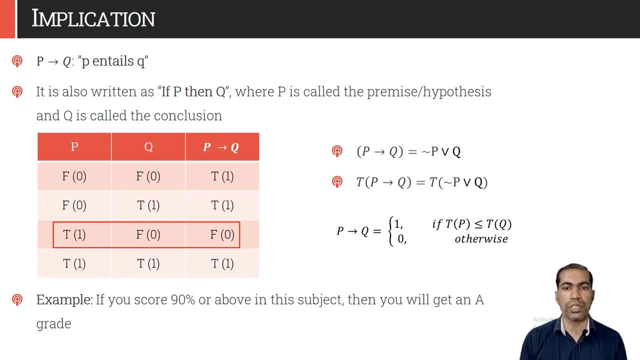 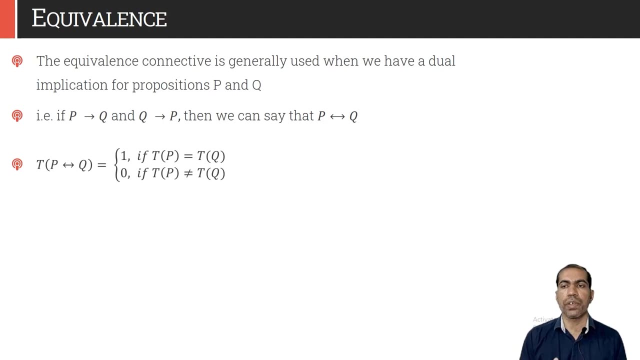 statement is false, So the compound proposition will take value 0 and for the last case again, truth value of P. P is less than or equal to truth value of Q and hence the compound proposition will stand true. The equivalence connective is generally used when we have a dual implication for the propositions P. 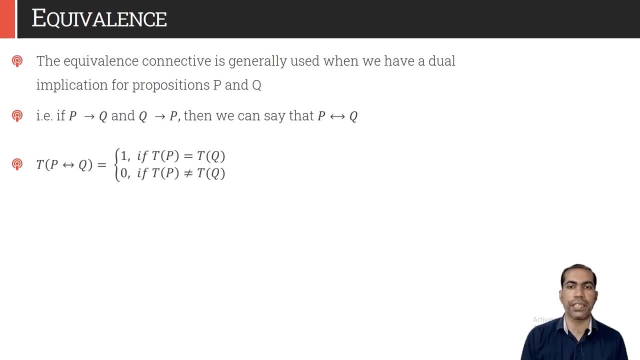 and Q. that means P entails Q as well as Q entails P. In that case we can write P equivalence Q, So P and Q are having the identical truth values and we can say that truth value of P equivalence Q would be 1. If both P and Q propositions have identical truth value and it would be 0 otherwise. So if we form 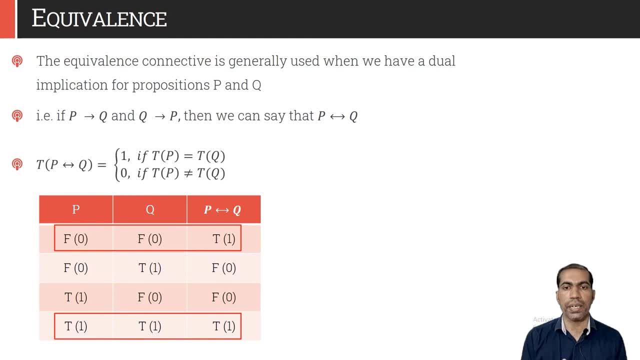 the truth table for that and we can say that for the first row and the last row, truth value of proposition. P and Q are identical. In first row both have 0 value. in last row both have value 1 and for those cases P equivalence Q would take value 1.. For remaining two cases, one proposition. 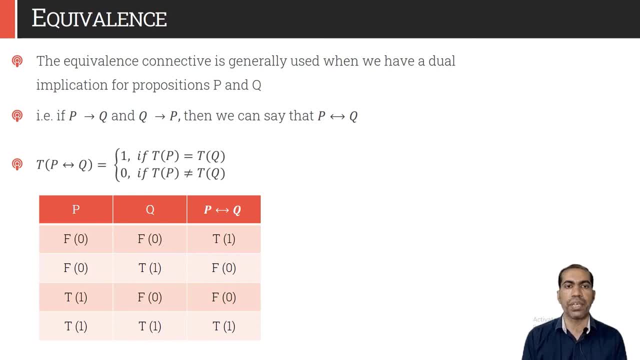 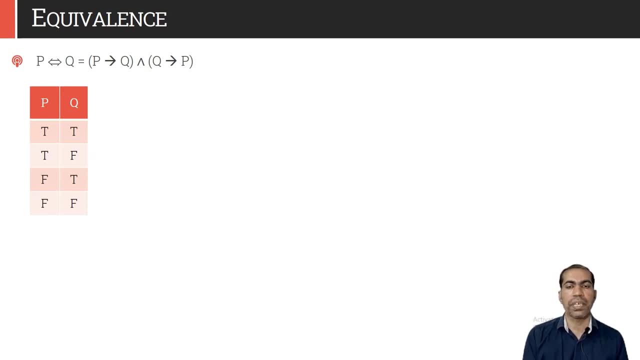 has value true, other has false and hence P equivalence. Q would take value 0. as we discussed on previous slide that we can say that P is equivalent to Q when we have a dual proposition, that means P entails Q is true as well as Q entails. 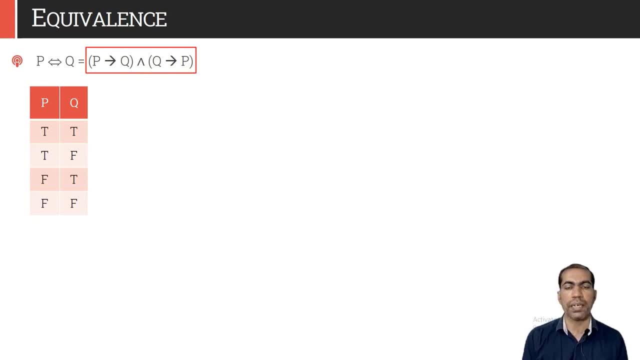 P is true. So these two propositions are connected by conjunction connectives. from previous slide We know that P entails Q is negation of P disjunction with Q. So first we'll compute negation of P. that would be as follows: F, F, T, T and P entails Q. that is negation, P disjunction with Q. So if one of the proposition either 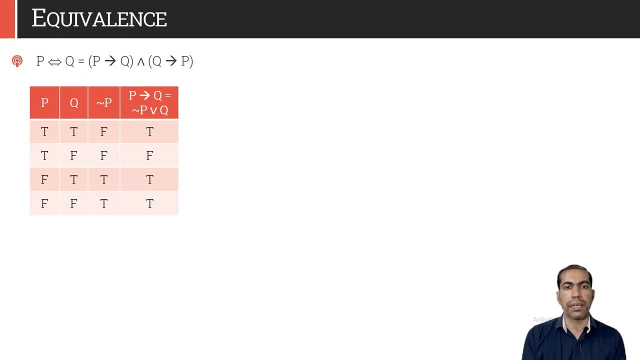 negation P or Q is true, then P entails Q will take the true value. otherwise it will have false value. So from the these two columns we can easily verify that for second row Q and negation P, both are false. So the P entails Q will be false. for rest of other cases it would be true. 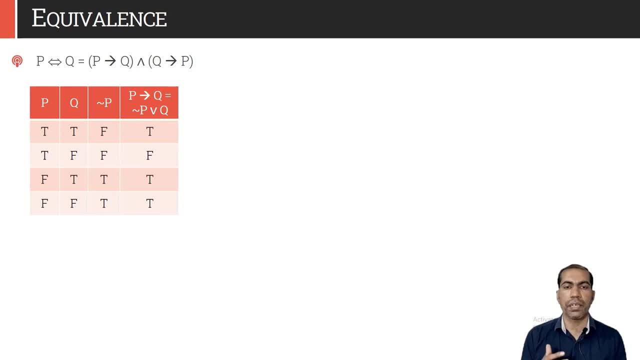 To compute Q entails P. we need negation of Q because Q entails P is same as negation Q disjunction P. So negation of Q would be F, T, F, T and Q entails P. that is same as negation P disjunction P. 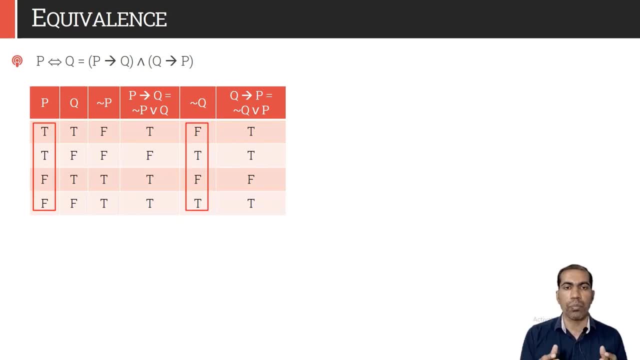 So we will consider these two columns and wherever both the values are false, in that case only Q entails P would be false, Otherwise it will be true. So for the third row, The proposition P and proposition negation Q has value F and for rest of other values at least one. 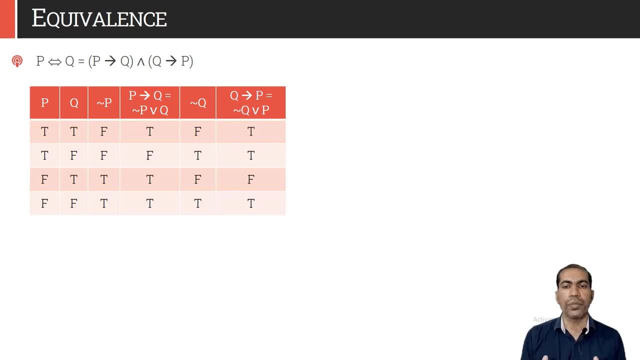 of them is true. And finally, to compute the equivalence, we have to take the conjunction of these two propositions: P entails Q, conjunction with Q entails P, and we already know that conjunction implies end operation, logical end operation. So whenever both of these propositions has value, 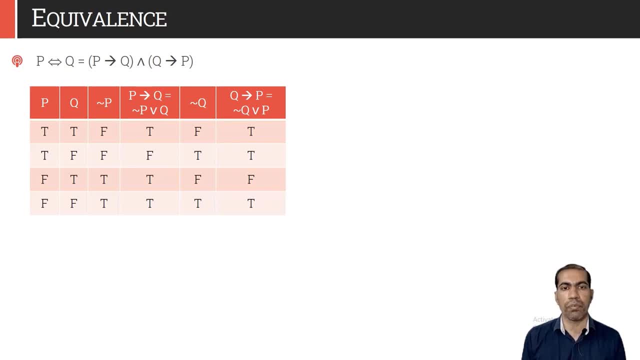 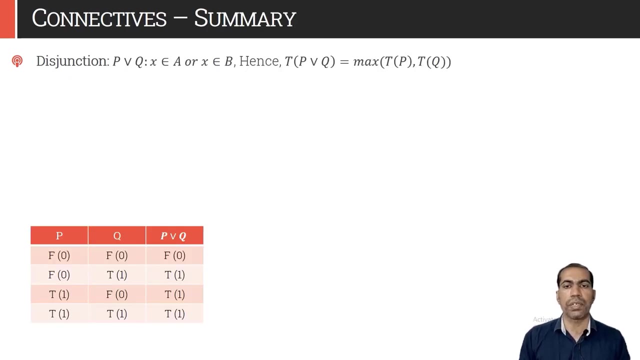 True P equivalence Q would be true, otherwise it will be false. So by observing these two columns and taking the logical end operation between them, we will derive P equivalence of Q as T, F, F, T. This is summary of all the connectives we have discussed so far. 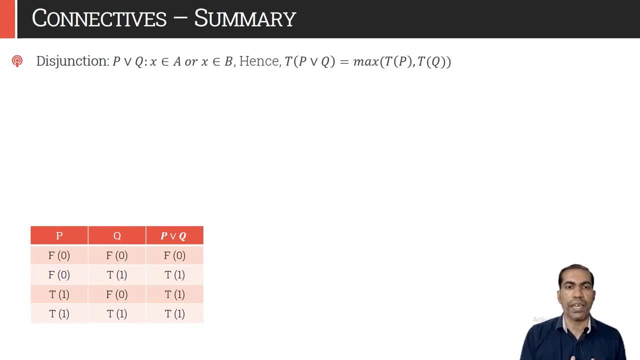 So disjunction forms logical or operation. So whenever proposition P and Q both have value false, in that case only disjunction will take false value, As we have seen. otherwise it will be true Conjunction forms logical and operation whenever P and Q both. 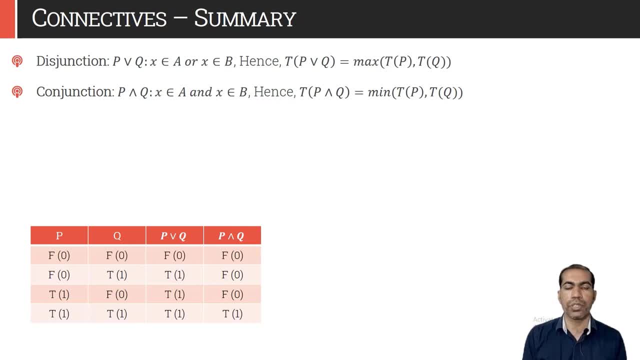 propositions are true, then only the compound proposition P conjunction Q will have value 1, otherwise it will be 0. The negation is simply complement of the truth value of given proposition. So if proposition is true, the complement or the negation of that will be 0, and if proposition is, 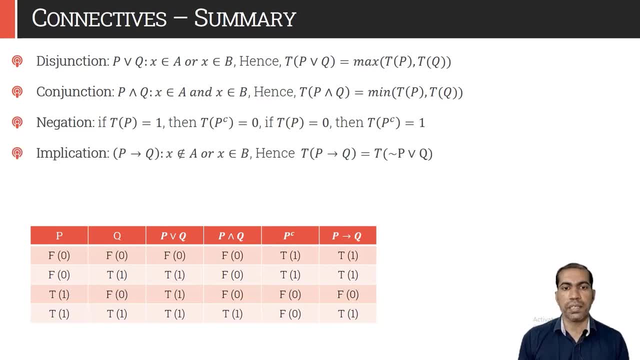 false, the complement would be true, Implication is represented as P entails Q and the truth value would be same as negation of P, disjunction, negation of Q and, finally, equivalence is given as P, double implication, Q, that is, P entails Q, is true, as well as Q entails P is also true and this compound. 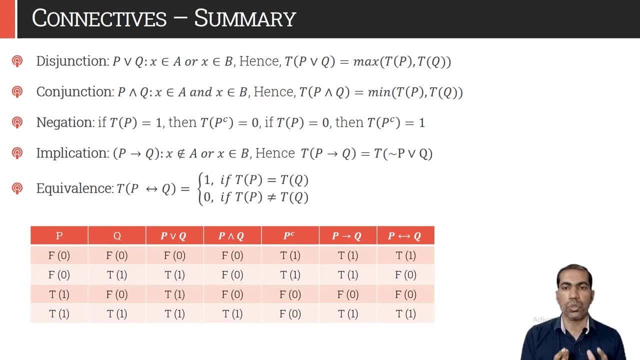 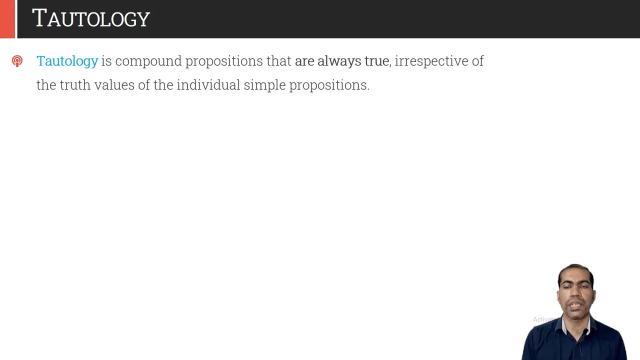 statement: compound proposition has truth value 1. if the truth value of P entails P is true. Truth value of Q, both are identical and 0. otherwise Tautology is compound propositions that are always true irrespective of the truth value of the individual simple propositions. So if we have formed some proposition with the help of two, 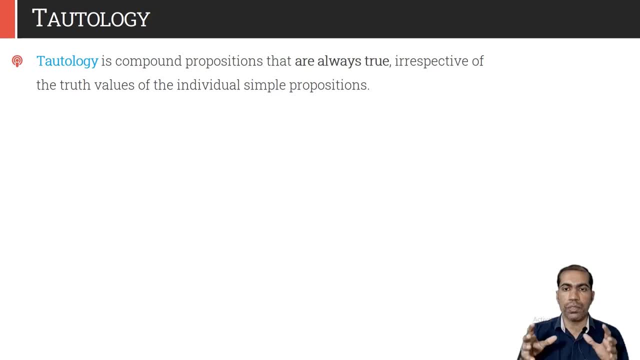 different propositions. so, irrespective of values of this P and Q, the compound statement will always take value. true, Such compositions or the such proposition are known as tautology. The tautologies are very useful for deductive reasoning, for proving the theorems and for making 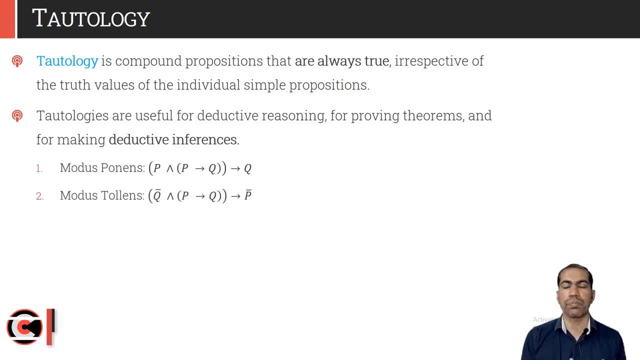 the deductive inferences. The modus ponens is defined as P conjunction P entails Q entails Q and modus tollens is Q bar. conjunction P entails Q entails P bar. So whenever we try to prove this, two that will be always true. That's a tautology and they are very frequently used in simplifying. 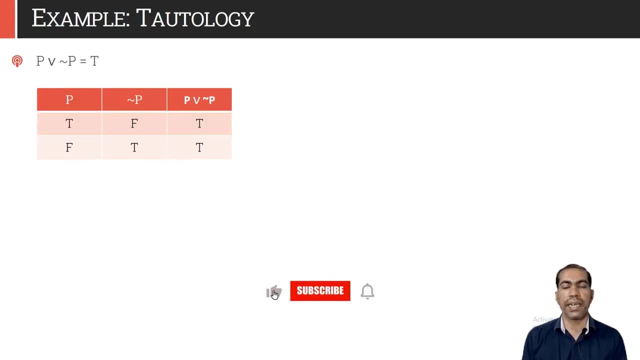 the deductive inferences: P- disjunction, negation P will be always true. Whenever P is false, negation P will be true. and whenever P is true, negation P will be false and the disjunction of that would be always true. So this statement is a tautology. Consider the example. we have to show that P entails Q, disjunction Q. 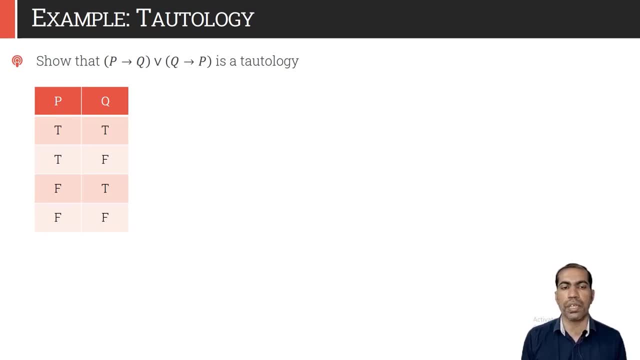 entails P is tautology. It means it is always true, irrespective of any value of P and Q. So first we will compute P entails Q, So that value will be t f, t, t. We have already computed this value on previous slides. 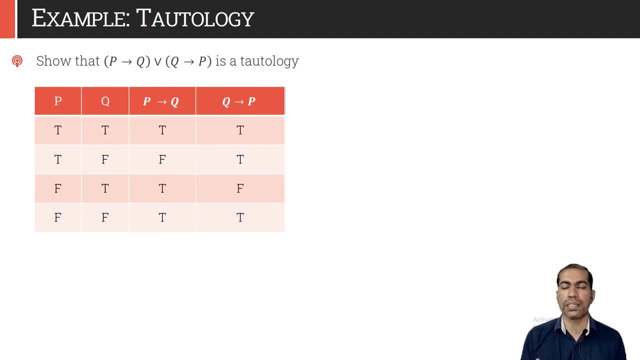 And Q entails P. also, we have already derived, when we were discussing equivalence, connective. So that is t, t, f, t. And if we take disjunction of these two, or the logical OR operation, that would be t, t, t, t, and that's why it is tautology. Now see, whatever may be the value of P and Q may be true, true, true. 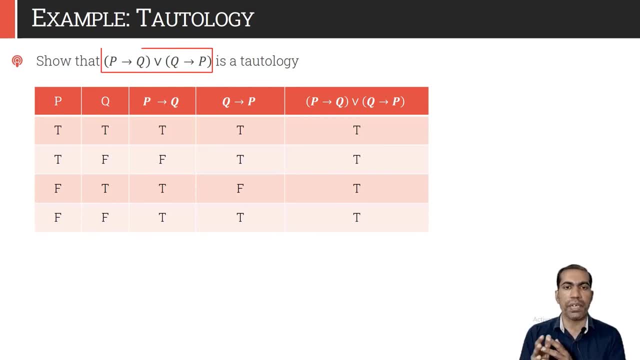 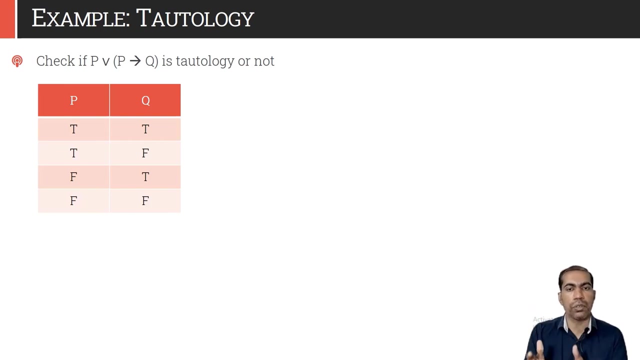 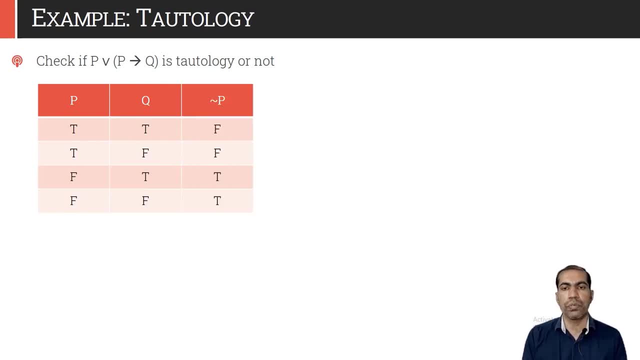 it is not. So to compute the p entails q, we will be needing negation p, because p entails q is same as negation p disjunction q. So negation p is computed, q is already available. we will find out logical or between them that will give us p entails q. So that is true, false, true, true and 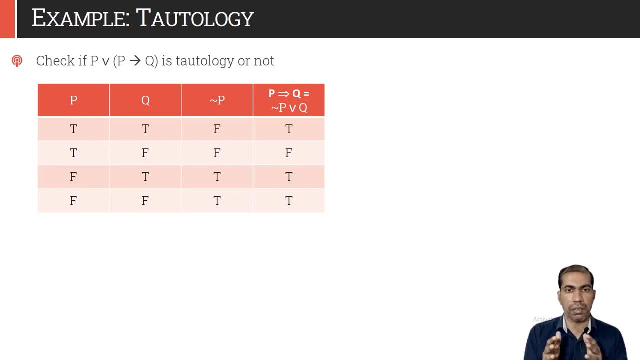 we have to take the disjunction of this proposition with proposition p, So we will simply take logical or between these two columns and the output of that is true, true, true, true. irrespective of truth values of individual propositions p and q, This proposition is always returning value. true. 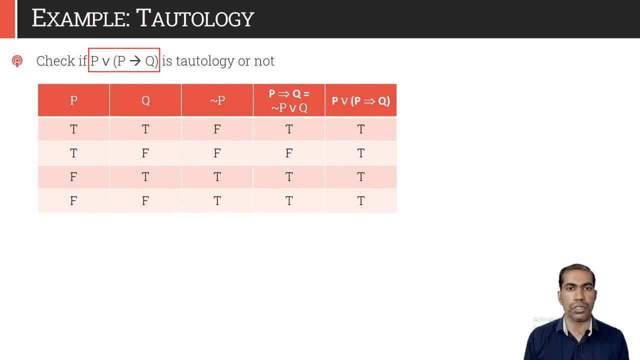 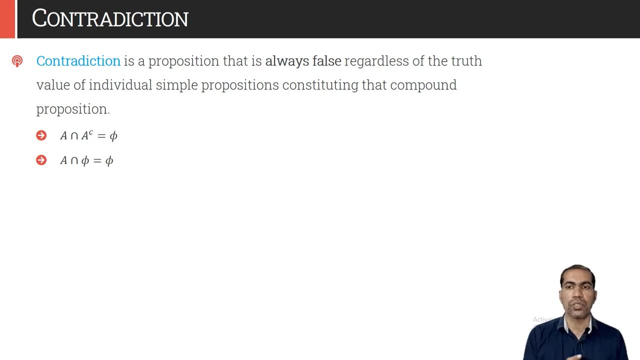 and hence this statement is the tautology Contradiction is a proposition that is always false. so this is exactly reverse of the tautology: It is always false, regardless of the truth values of the individual simple propositions. In case of set theory, we already know that a intersection, a complement, is phi. that is always. 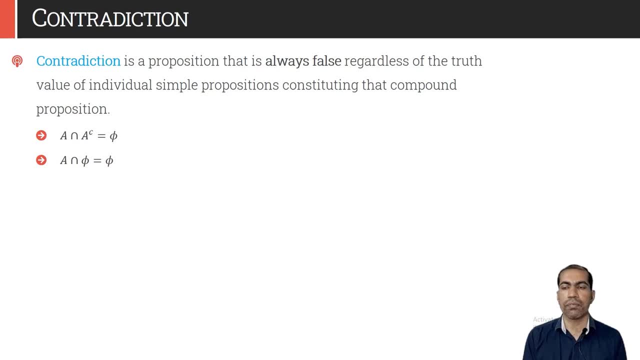 going to be false, or a intersection phi that is also always going to be phi. So these are the well known contradiction statements: P conjunction, negation p, that will be always f. So this is known as a contradiction. So p is true, negation p would be false. p is false, negation p would be true. and. 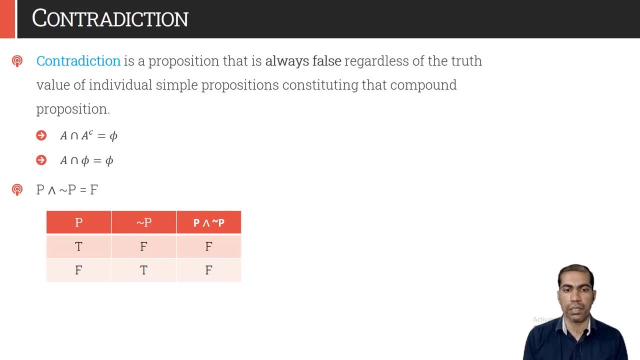 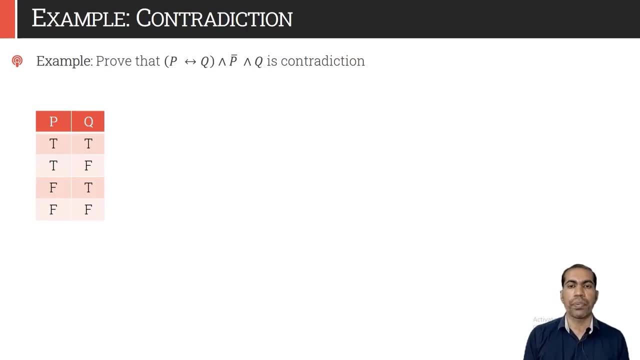 then conjunction is simply a logical and operation. So if both statements are true, then only conjunction will be true, otherwise it will be false. Let us check if p equivalence, q conjunction, p bar conjunction q is contradiction or not. So to prove that, we will build a truth table and we will find. 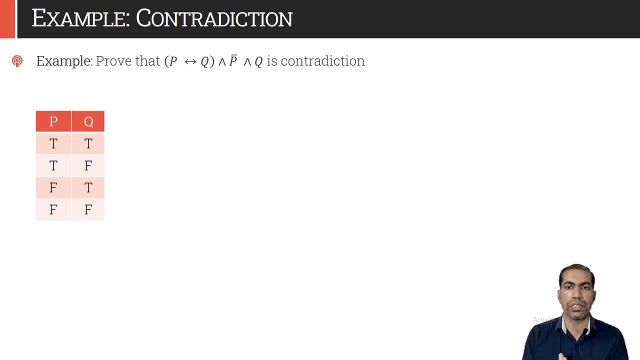 out whether the truth values of this compound statement is false. for all possible p and q, we need p bar, so that will be f f, t, t. so simply, that is the negation of the p? p equivalence. q is t, f, f t, because that would be true whenever p and q both are having the identical values. So for the first, 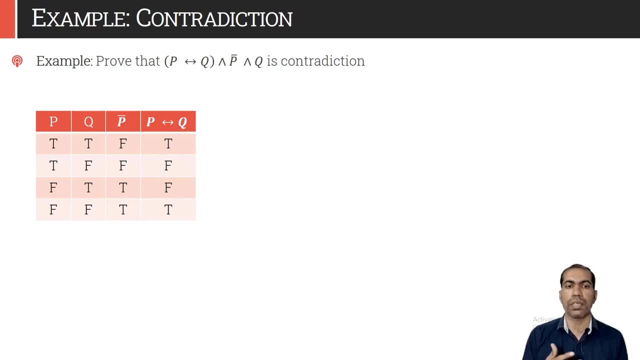 and the last rows, p and q, takes the identical value for other. one is true, other is false. So p equivalence q would be t, f, f, t. Now we will compute p bar conjunction q. So if p, bar and q both are true, then only p bar conjunction q will take value true. otherwise it will be false. 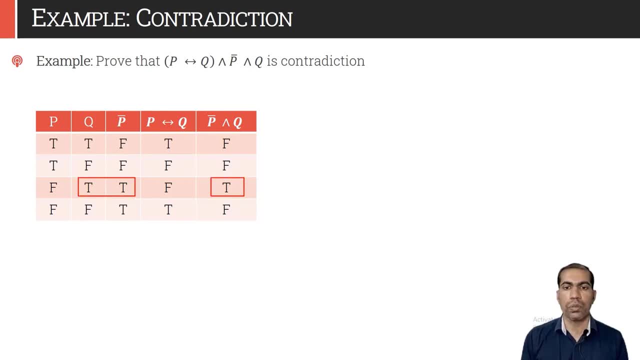 because it is a conjunction operation. So for only third row this proposition will take value t. for rest of all it is false. Now we will take conjunction of p, equivalence q with p bar conjunction q. that will give us the truth value of entire given propositional statement and when. 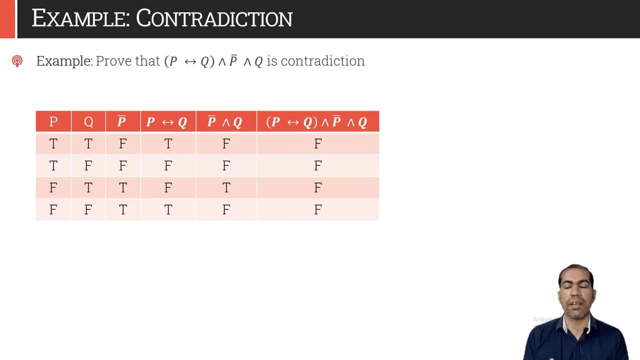 we take the logical and operation between them, Then it is f, f, f, f that says that given statement is a contradiction, because, whatever may be the value of individual propositions p and q, the output is always false and that's why it is considered as a contradiction. Thank you.